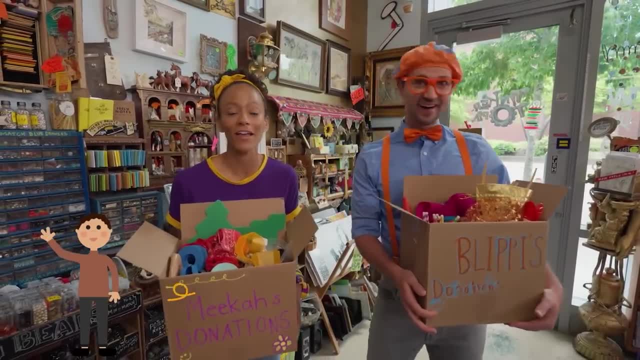 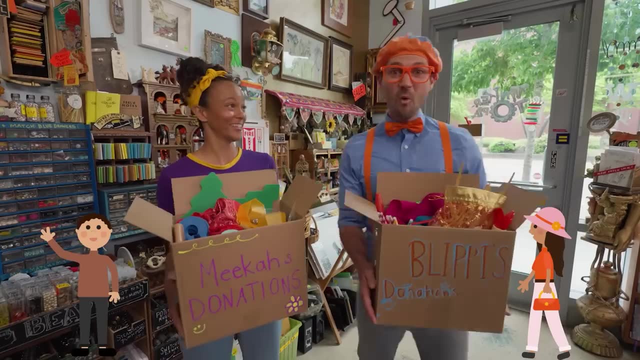 Well, that's when you have something that maybe you don't want anymore, You can donate it. and when you upcycle it, it's when somebody uses those items to make something brand new, Wow, cool, Hey. so today we're gonna upcycle these items, Yep. 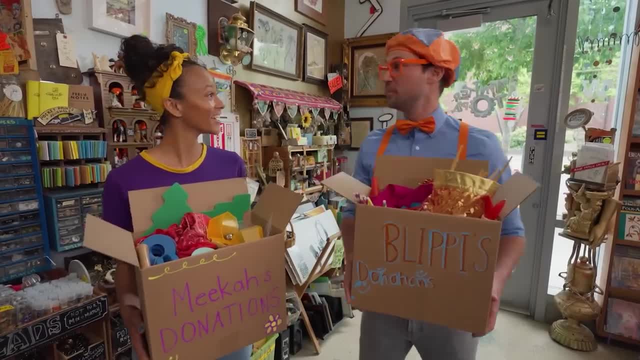 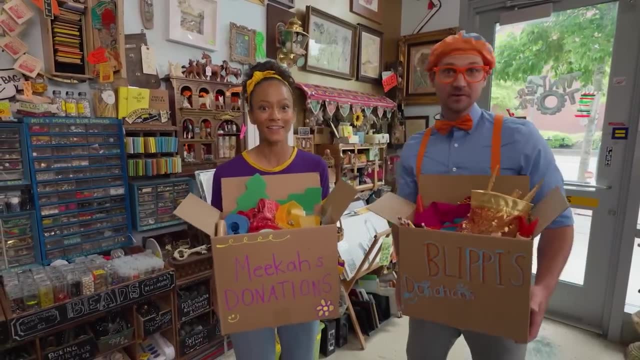 We're gonna donate them and then someone else at some other time will make a really cool craft. Yeah, hey, let's craft up a plan. We can donate our items, then collect new items to make a craft Cool, that sounds like fun, Yeah. 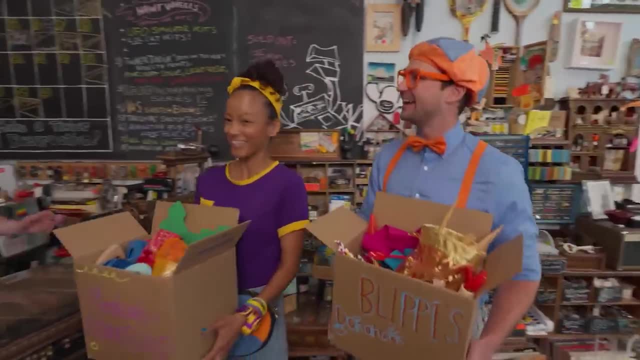 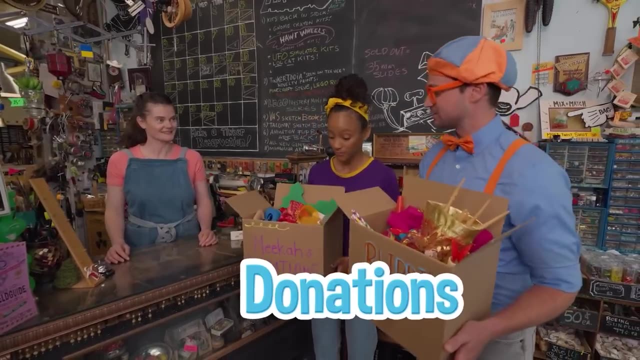 Oh, there's someone over there, Hello, Hey, Hello, welcome. Oh, what's your name? Um, I'm Ms Darcy. Welcome to Tinkertopia. Hi, Nice to meet you. We brought some donations for you, Yep. 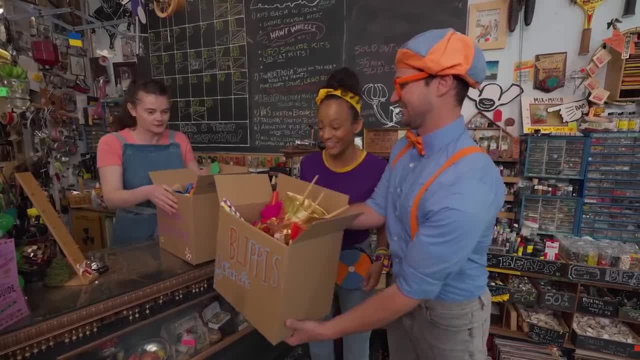 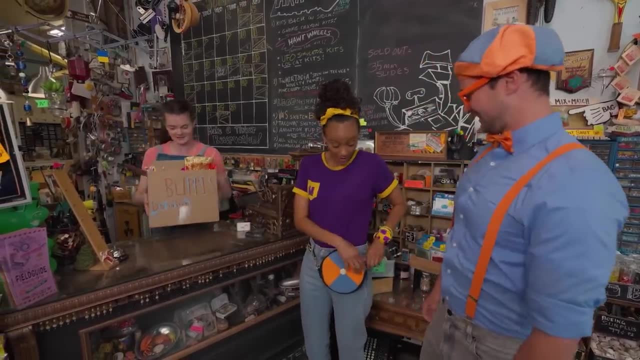 Wow, those look like some good goodies. Yeah, Nice and colorful. Do you think people will be able to use those? I definitely think that people will use these for their crafts, for sure. Thanks, I actually have two more things right here in my jam pack. 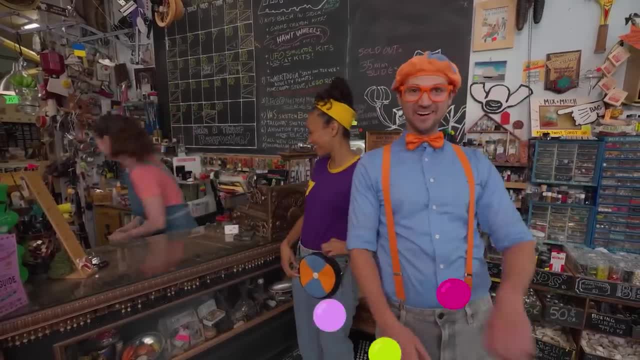 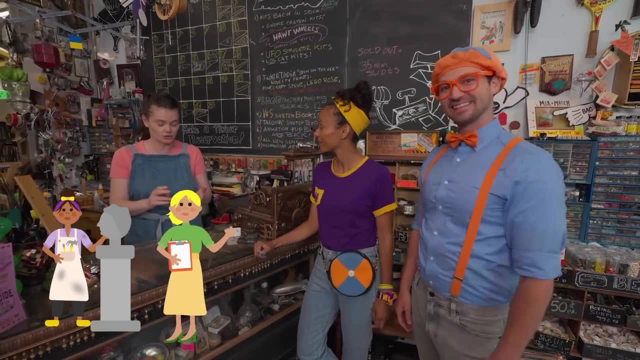 You can take these too. Awesome bouncy balls, Cool, Wow. so why is it called Tinkertopia? Well, we wanted to create a place where crafters, teachers, inventors, all kinds of folks that like to upcycle and repurpose things. 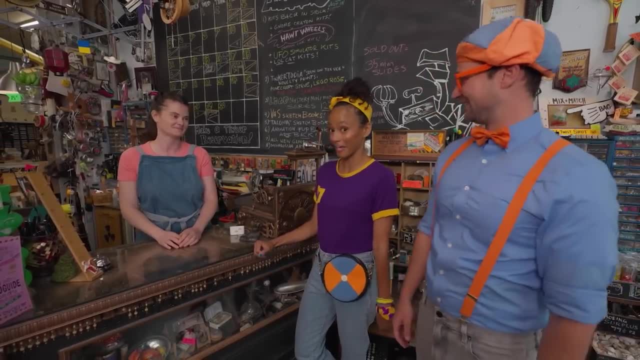 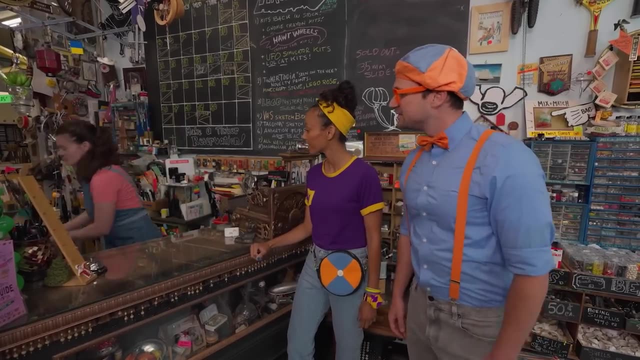 a place where they can find those perfect pieces. Oh cool, and they can tinker. That sounds like fun. How do we get started? Well, we have a session for you today and I have these humongous bags. You two can go and fill up with your own perfect pieces. 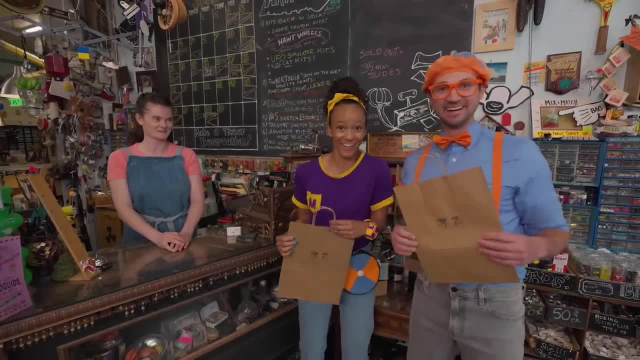 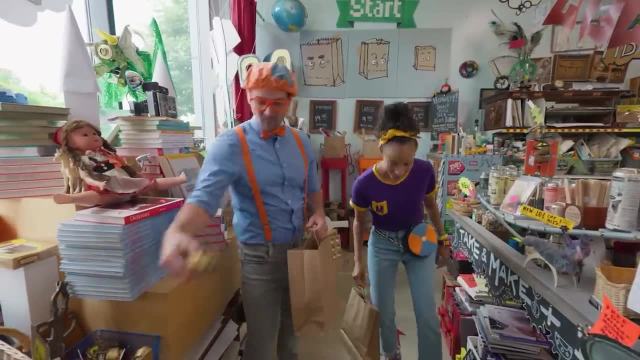 Oh, thank you. Yeah, Are you excited? Yeah, let's go. Thanks, Thanks, Wow, cool, There's so many cool things here. Yeah, Whoa, look at this, Mika. Oh, what is that? 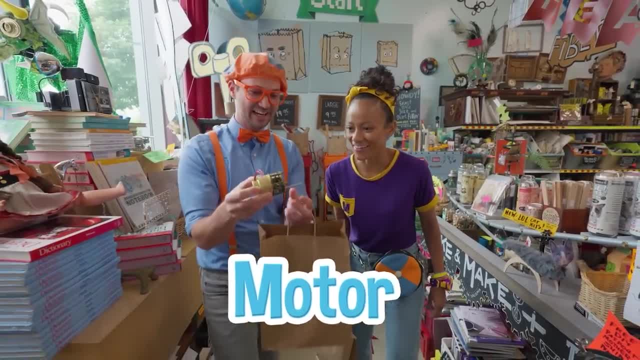 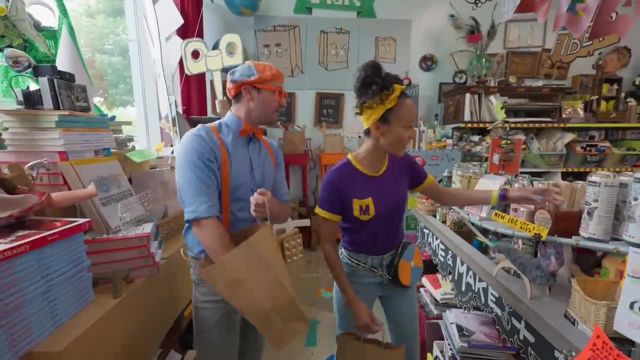 It looks like a motor Ring ring. Whoa, Yeah, you can attach it to some wheels and then go super fast. That is really neat. Yeah, Hey, what is this? I don't know. A cat? I think we can make our very own cat. 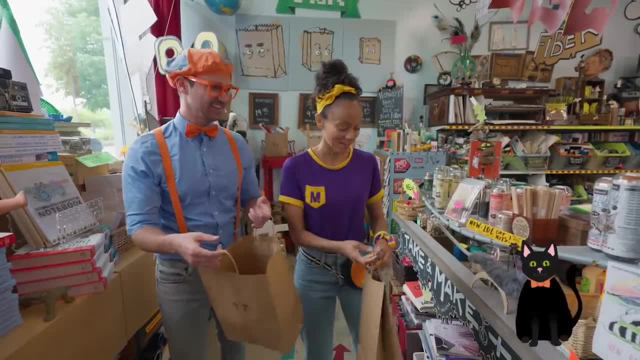 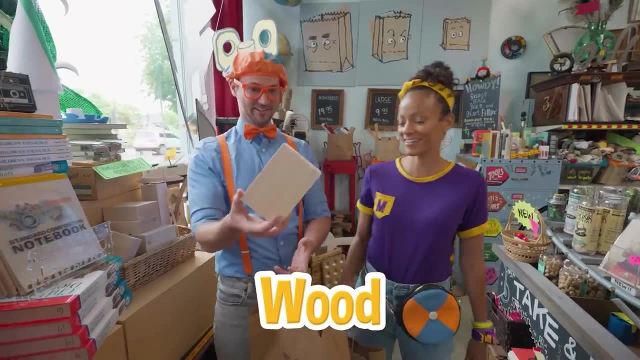 Oh, that sounds like fun. Here you go. Oh, thank you, I'll get one for me too. Meow, Hey, Mika, check it out. Oh, A big block of wood. You can do a lot of things with that. 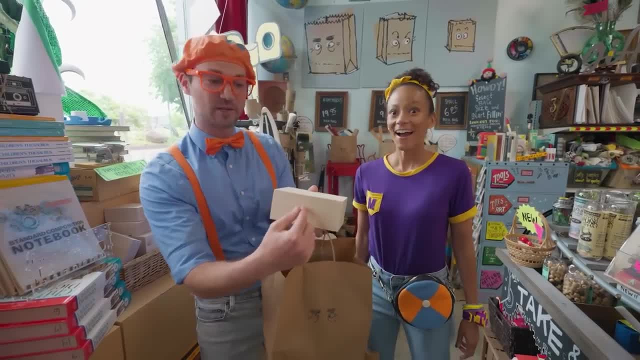 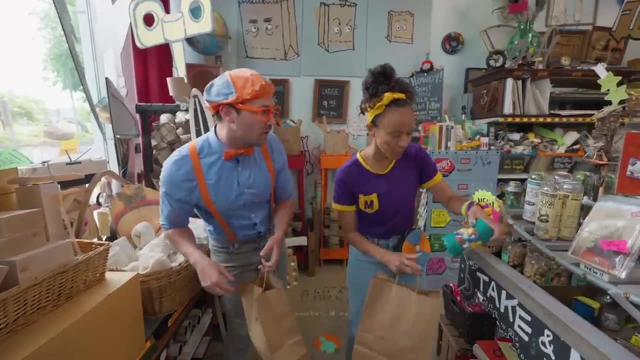 Oh yeah, We can make a pedestal for a cat. Yeah, and we can write first place on it. Yeah, that's a great idea. Yeah, Oh, what's in here? Oh, look, a bunch of tacks. 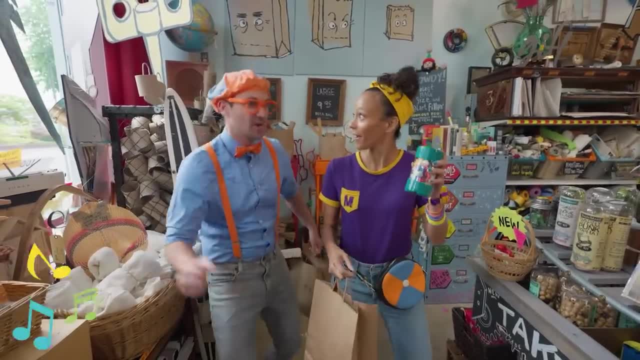 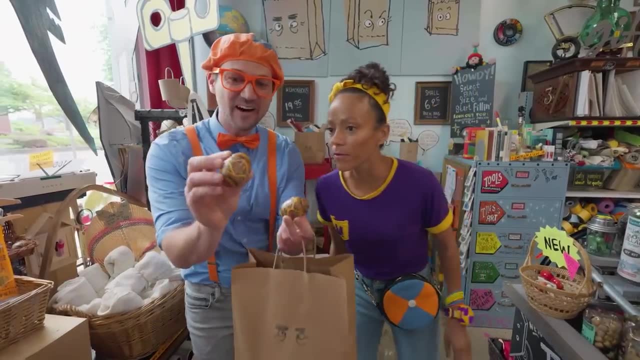 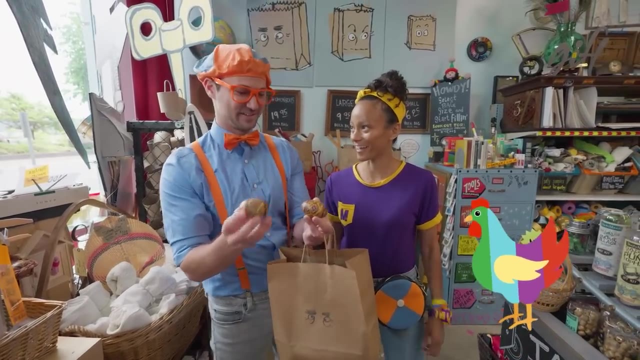 Whoa. you can tack things up with that, Yeah. or you could use it as a shaker, Whoa. and look at these, Wow, Colorful eggs. Yeah, they're really pretty. Yeah, they are. I bet that chicken was very colorful. 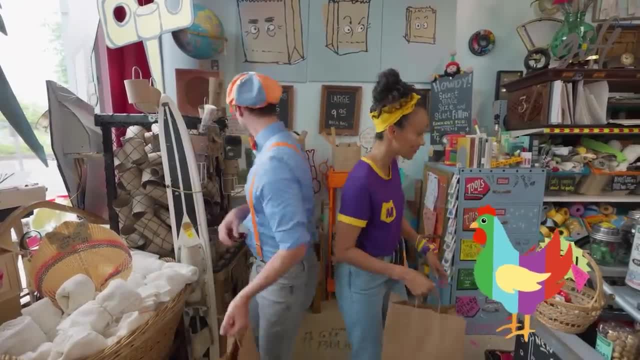 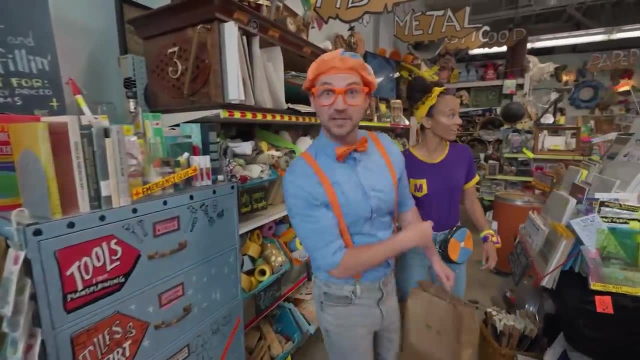 You want one Sure thanks, All right, you're welcome. Wow cool, So many cool things, Yeah, Whoa. Okay, I'll see you later. I see something cool. Okay, Let's see what else is here. 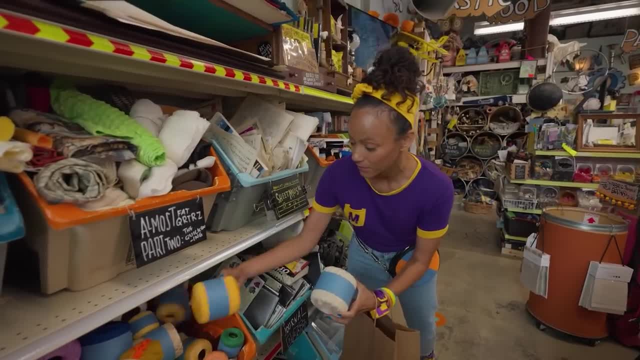 Oh, look at all this colorful string. Hmm, Maybe I could use something for my cat. Cats like to play with string and yarn. Ooh, and a journal. Hmm, I don't think I'm going to use that, Ooh. 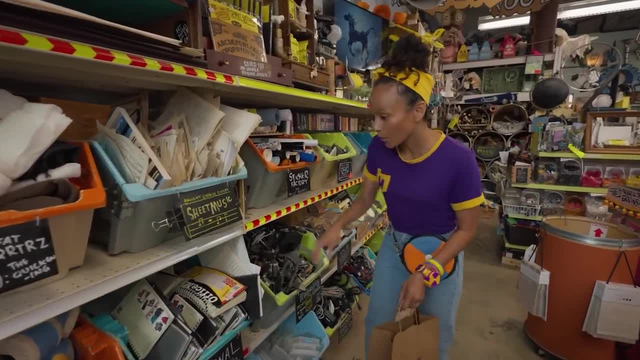 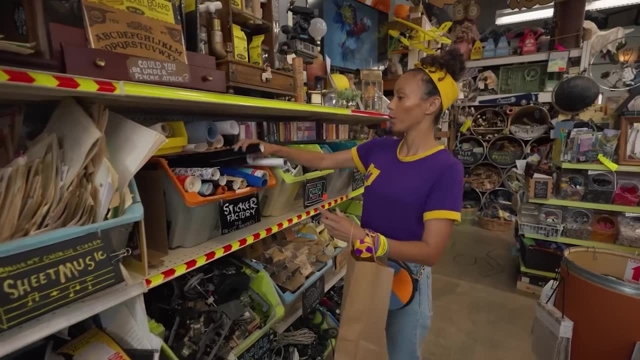 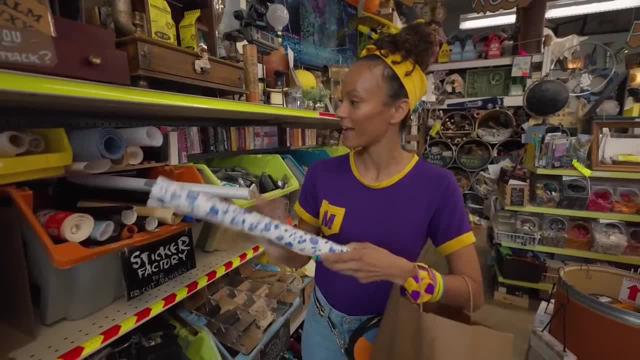 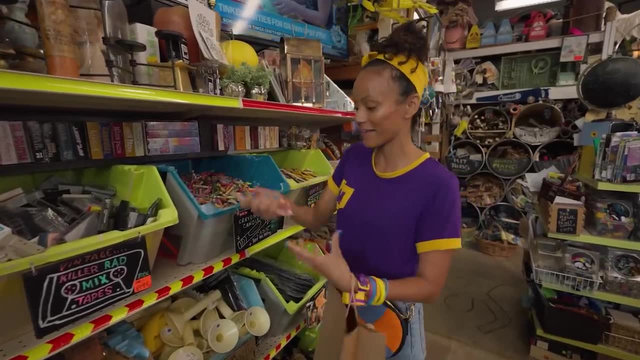 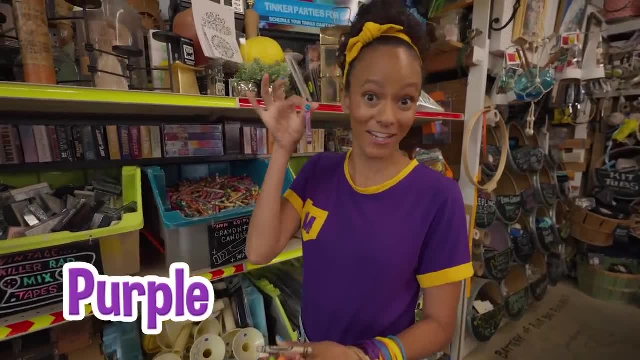 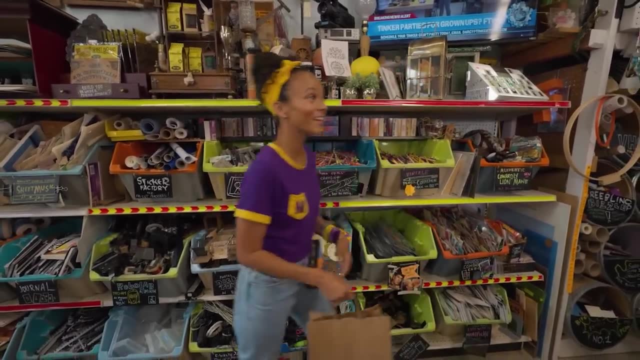 Oh, And look purple, one of my favorite colors. I'm going to put some in here, Some extra for Blippi. Oh, hey, Blippi, Hey, What are you finding? All sorts of things. I grabbed you some crayons so you can decorate your cat. 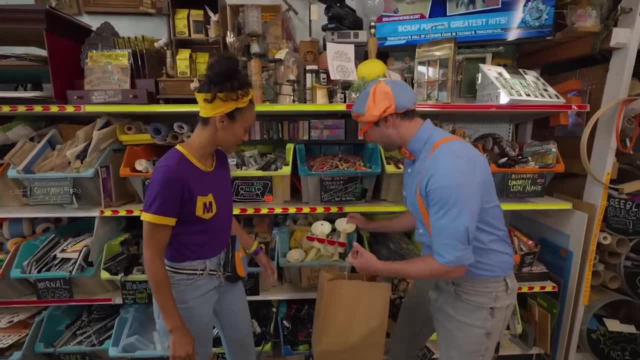 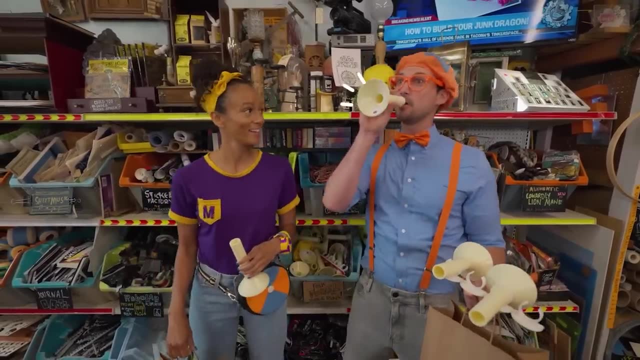 Oh, you got me some Yep, Ha-ha, That's so nice of you. Oh, What are these? Oh, It kind of looks like a trumpet, Ba, ba, ba ba, Or a megaphone. Hello, hello. 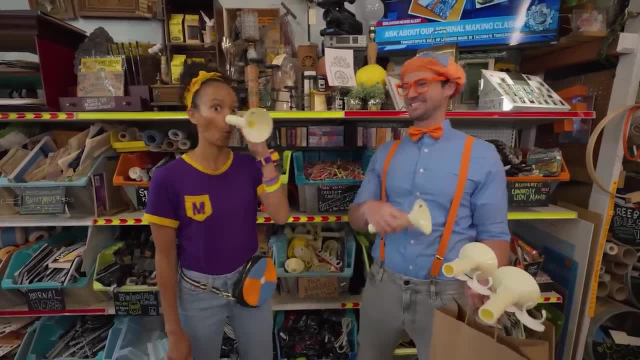 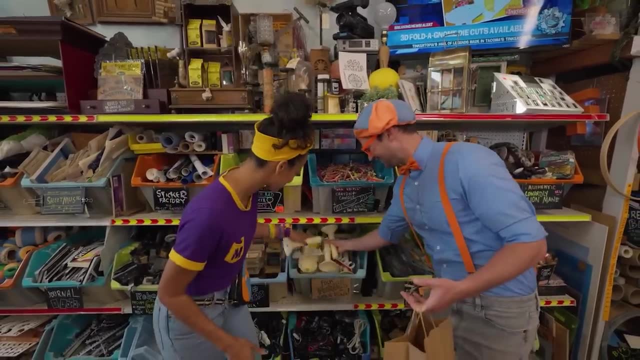 Or a really long nose- Oh, that's silly. Or an ice cream cone- Oh nice, You want a lick? Yum, Oh, it's really cold. All right, Wow, All right. What's over here? Oh, I want to go check this out. 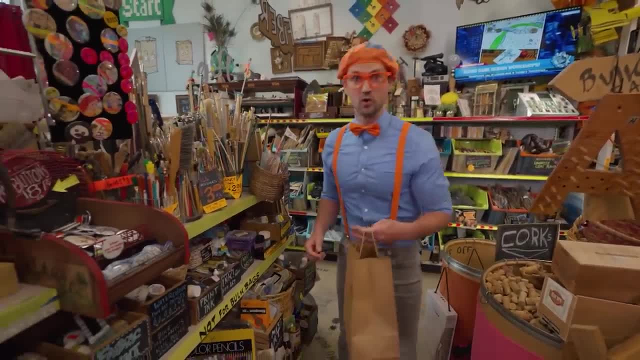 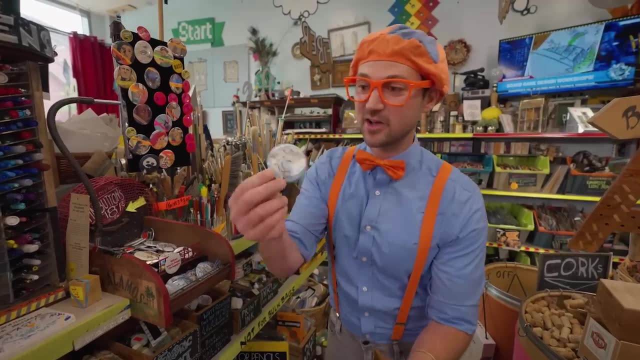 I'll be right back. Okay, see you soon. Wow, so many cool things. Whoa, look at this. Yeah, a pin. You can put that on your shirt And it says Tinkertopia. Okay, I'll put one in there for me. 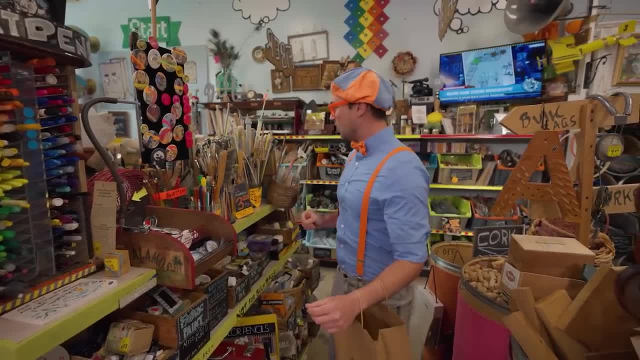 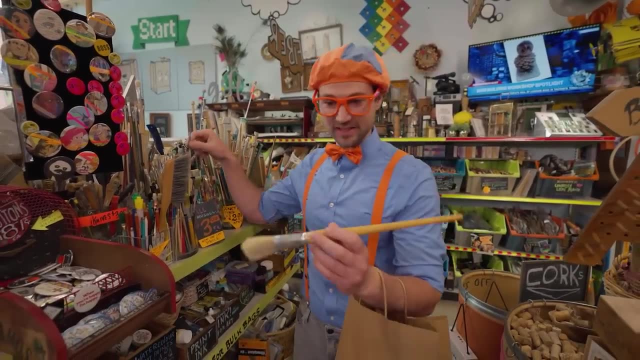 And I'll grab one for Mika Whoa, look at these, A giant paintbrush. Wow, you can make a big art piece with this one. Oh, or a really small painting with that one. Hey, this isn't a paintbrush. 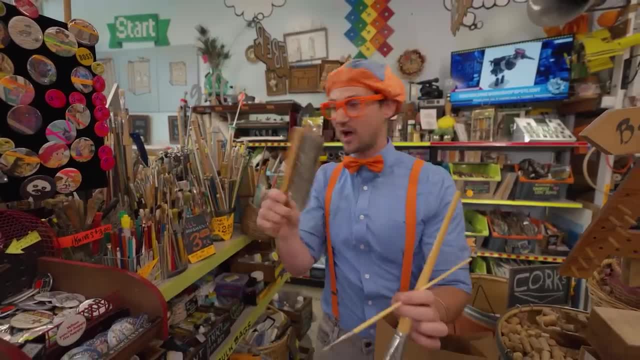 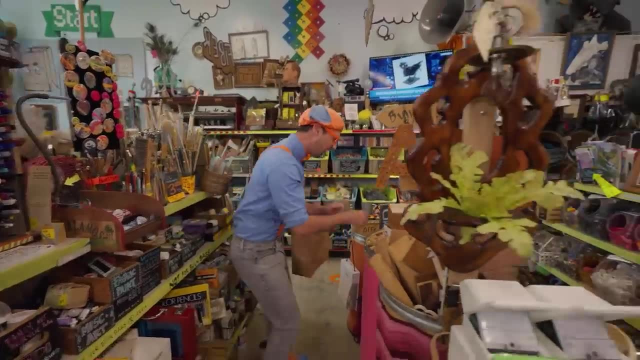 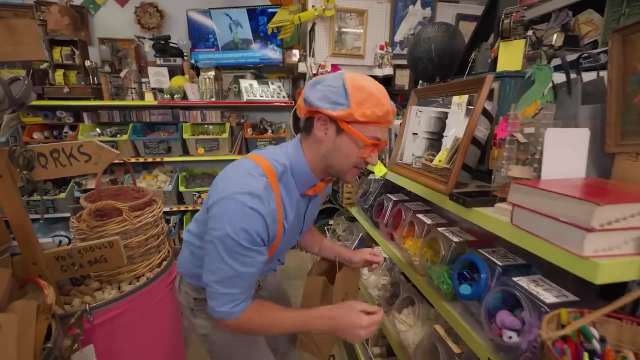 Wow, But I bet you can add some really cool texture to that art piece. Wow, All right, let me put the small one in there. Wow, And let's keep exploring. Whoa, some colorful things. Ooh, this is purple. 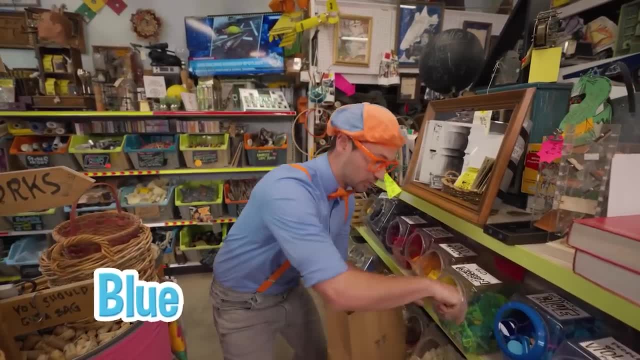 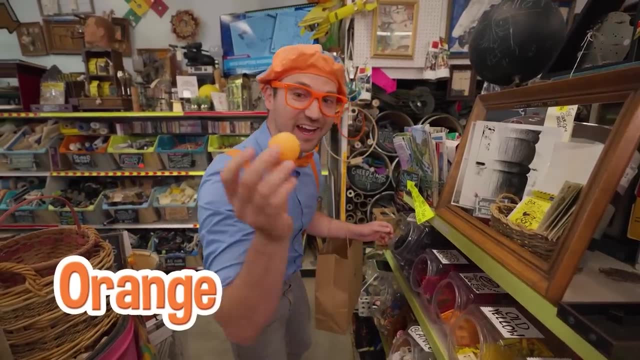 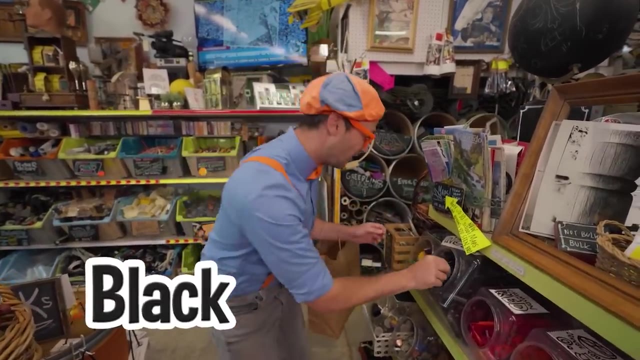 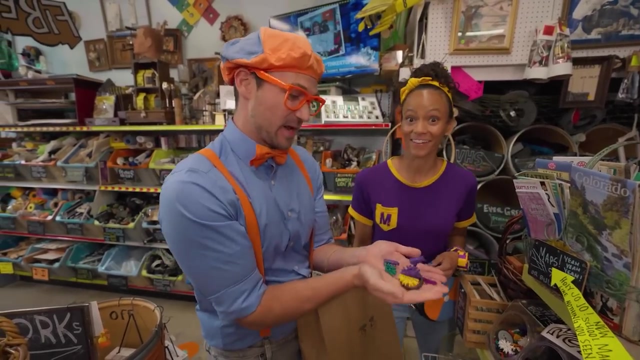 Wow, Blue, Green, Yellow, Orange, Red, Black, Whoa, And These are rainbow colors. Hey, Blippi, Oh, hey, Mika, What did you find? Well, these are rainbow colored objects. I don't know what they are, but maybe we could use them. 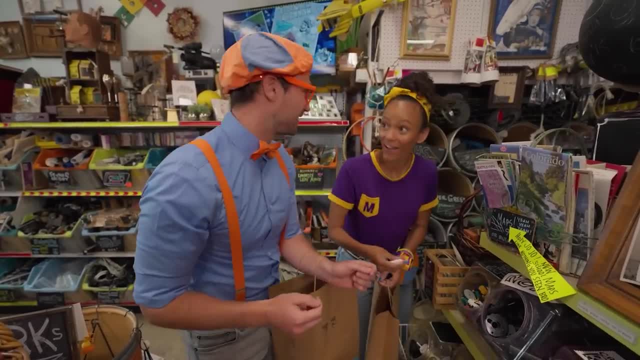 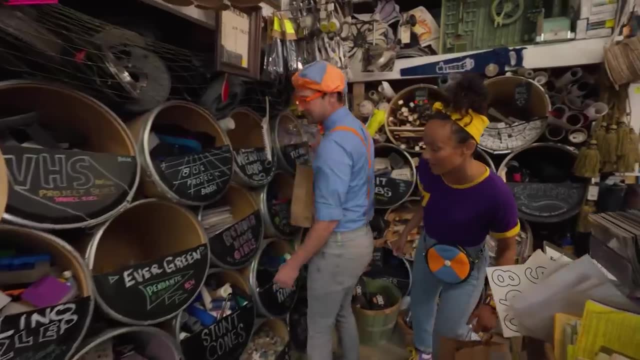 Oh yeah, These are cool. Yeah, and I got you a surprise for later. Oh, I can't wait to see. Wow, there's so many cool things here. Yeah, there's so much to look at and explore. Whoa, look at these. 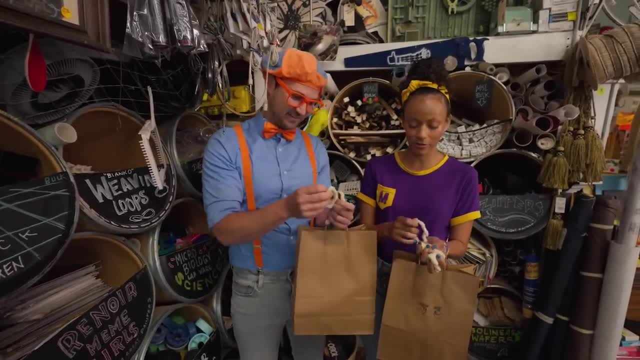 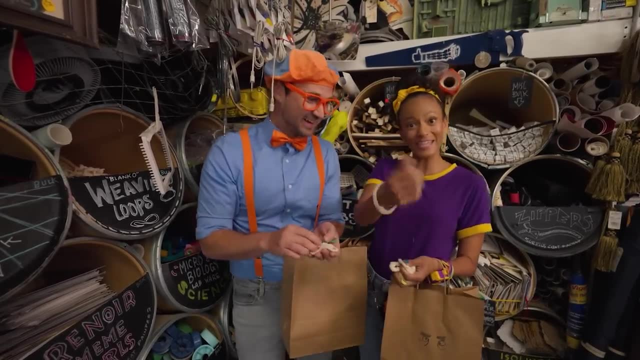 Oh, Oh, how I wonder what they are. Kind of looks like onion rings- Oh don't eat those. Or a rubber band- Whoa. or a bracelet- Oh cute. All right, I'm going to put some in here. 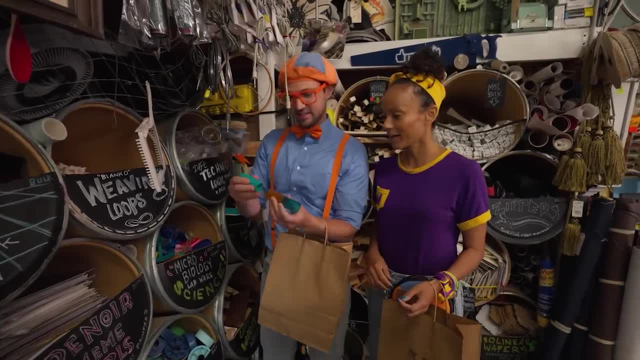 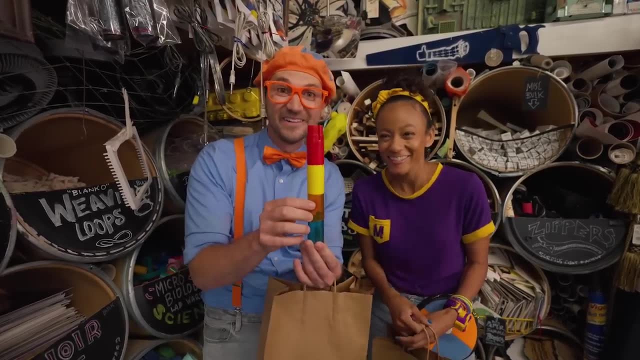 Yeah, Wow, Whoa. look at these. Oh, you could build a really tall tower with those. Oh, yeah, Will you say the colors with us from top to bottom: Ready, Red, yellow, orange blue, Whoa cool. 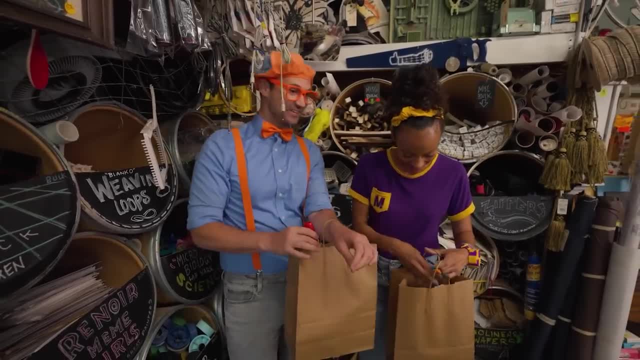 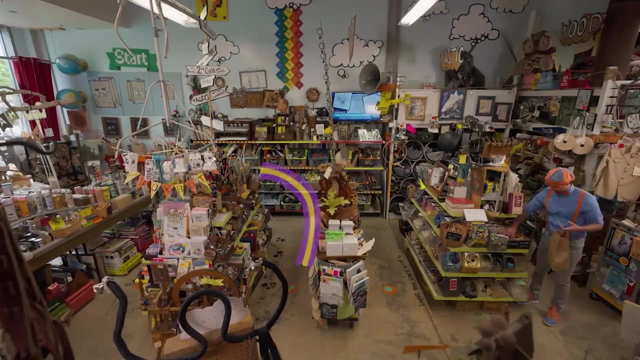 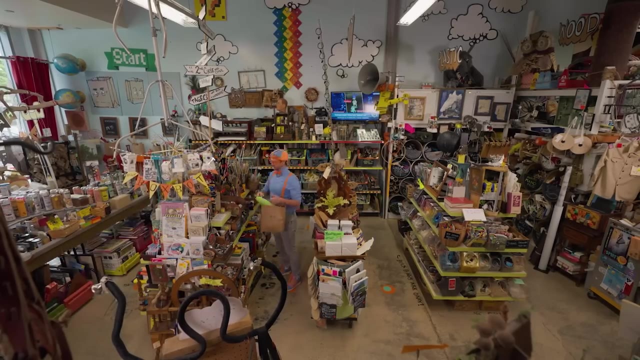 You want half? Yeah, All right, two for you, two for me. You're welcome, All right, shall we keep exploring? Yeah, Let's do it, Let's go. Looks like a great spot to put our craft together. 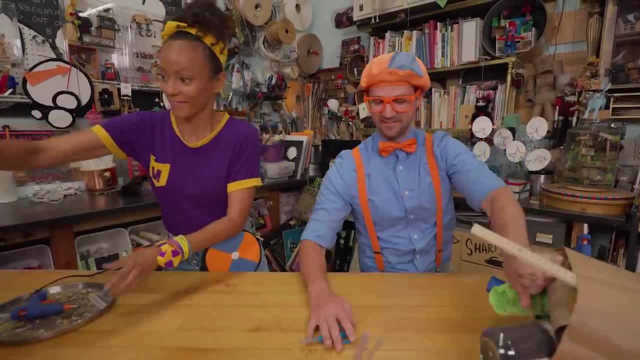 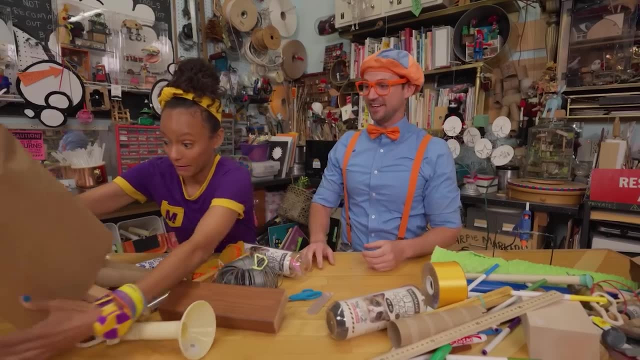 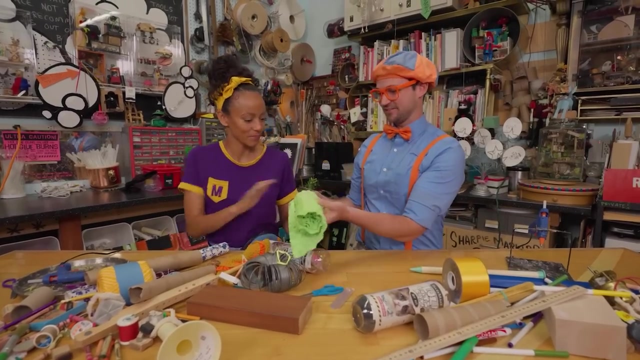 Oh yeah, Let's check out what we got. OK, Whoa, you did grab a lot of stuff. I got excited. Wow, Whoa, look at this. Oh, I like that color, Yeah, and feel how soft it is. 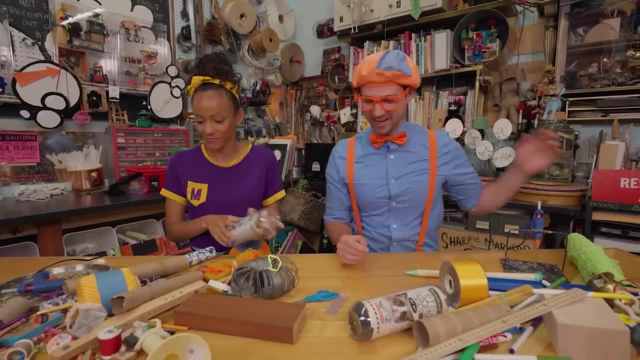 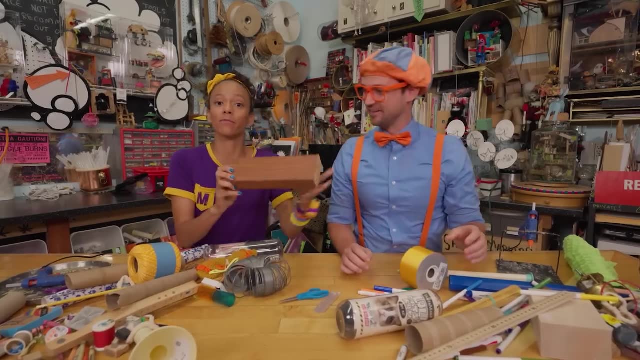 Oh, Oh, what did you get? I have some string. Wow, Oh, I have some ribbon. Oh, look at this nice wooden block. Oh yeah, Remember my wooden block. Yeah, Cool, Wow, Oh, hello. 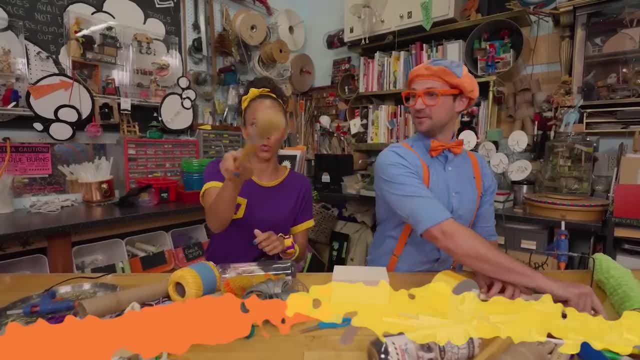 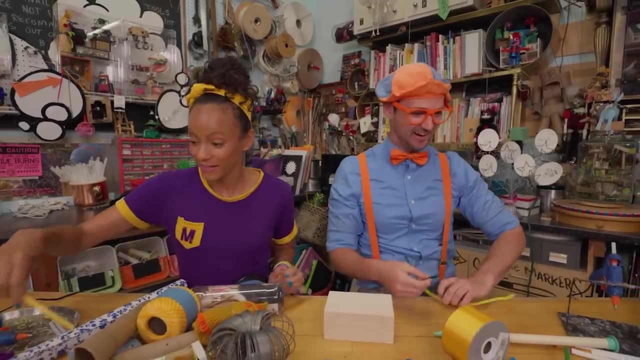 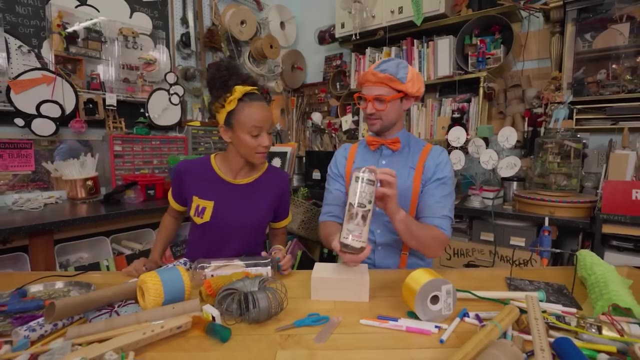 Oh, I got a really big paintbrush. Whoa, and look at these. Oh, cool antennas. Yeah, thanks, Wow. Check out this yellow glittery pencil. Wow, It looks sparkly. Yeah, Whoa. Hey, here's the cat. 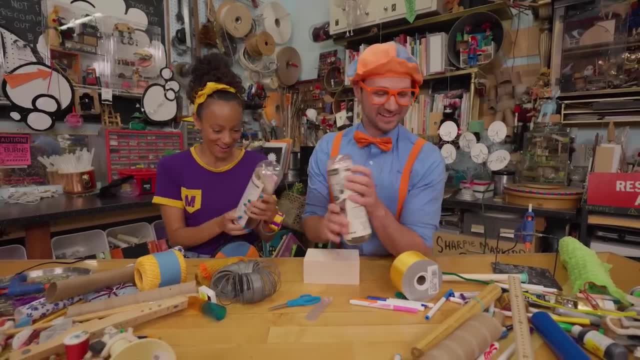 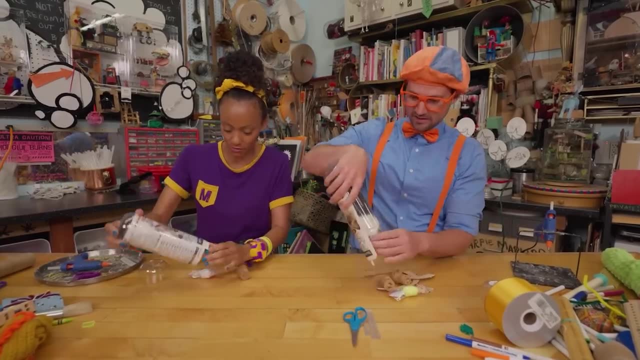 Oh yeah, Shall, we make these. I can't wait, Let's do it. All right, I'm going to clear some room. Yeah, Excuse me, Steph. Oh, that's probably the outside of the cat. Oh, so soft. 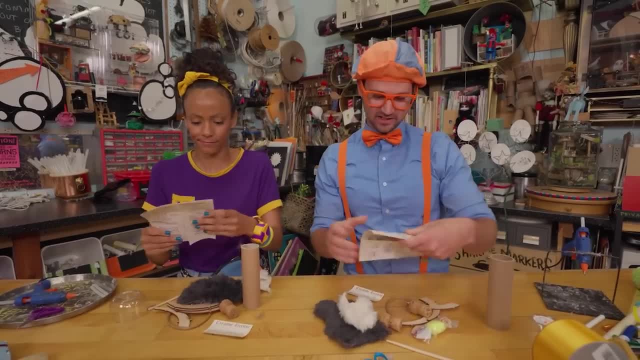 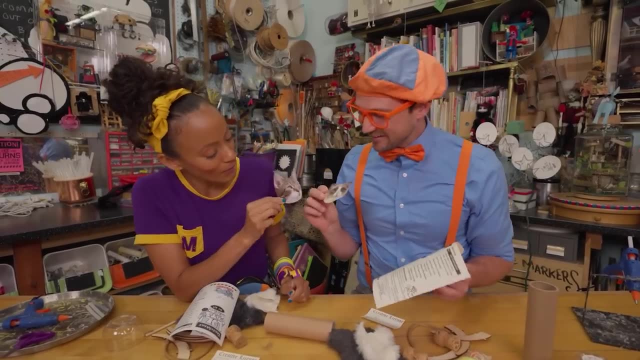 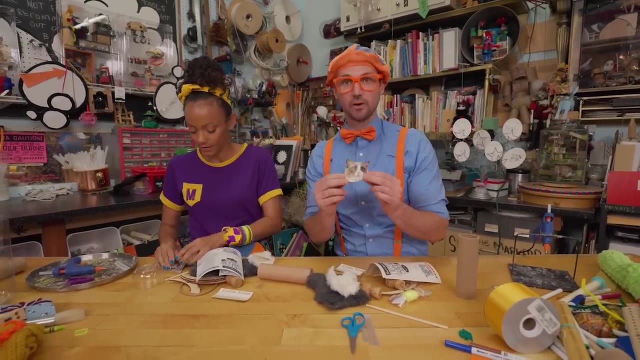 Yeah, Okay, Okay, Directions, Cat. Hey, Here's my cat head right there. Okay, That's so cute. What does yours look like? Meow, Oh, Meow, Yeah. Wow, It's so cool. These were probably cut out from a newspaper or a magazine or something. 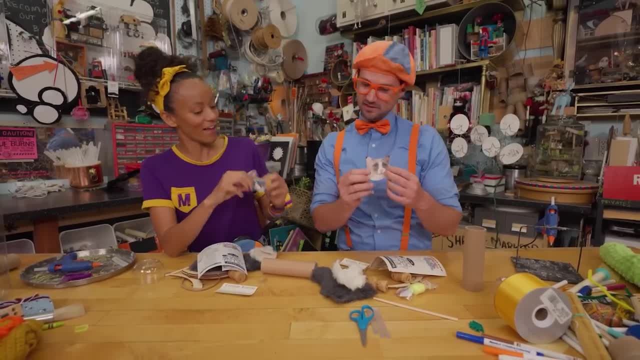 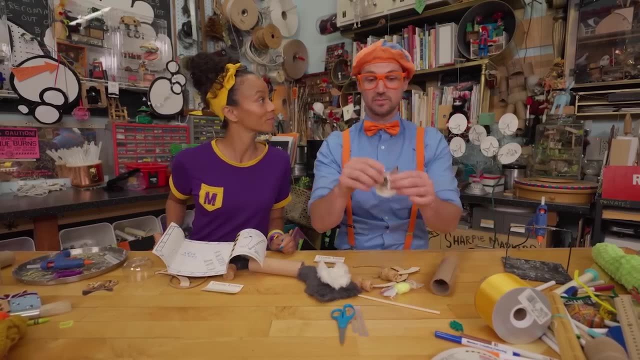 Yeah, You're right. Yeah, Yeah, They're repurposing it. Yeah, This place is so cool. Yeah, I love how you can repurpose things. You know, take something that used to be used for something, But then you use it for something new. 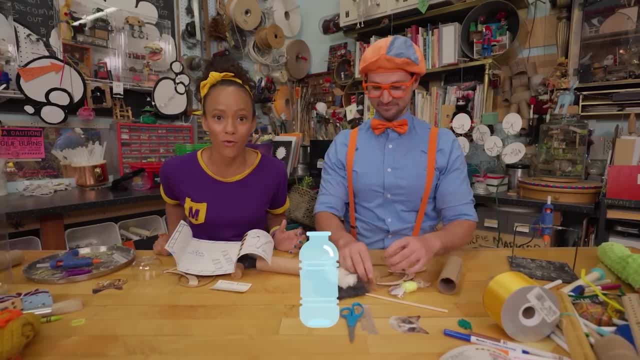 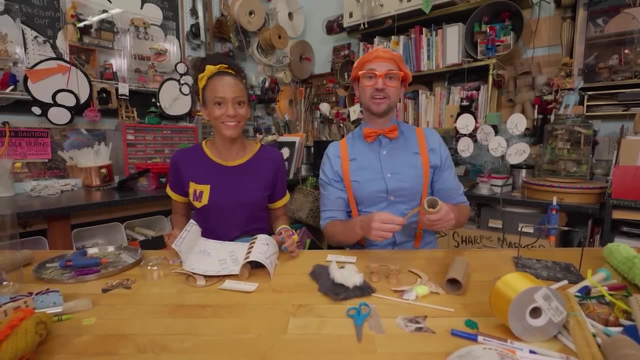 Yeah, For example, if you have a water bottle that you're drinking from, once it's empty, you can clean it out, dry it and use it as a pencil holder. Wow, It's so good and healthy for the environment to repurpose things. 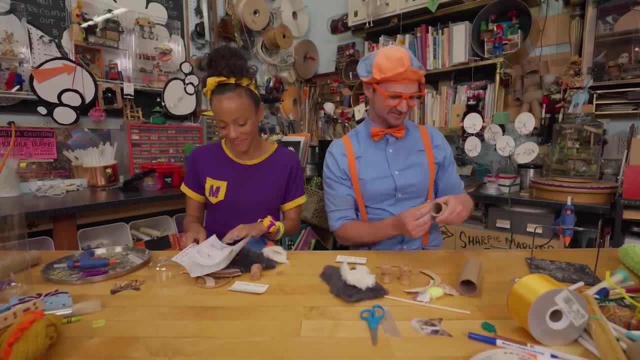 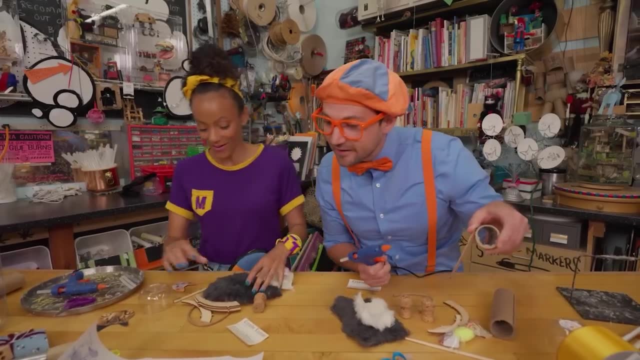 Yep, It's less waste around planet Earth. Mm-hmm, Here's some directions here. Ooh, I'm going to be very careful with this. I think these look like the legs, right? Oh yeah, You're right. 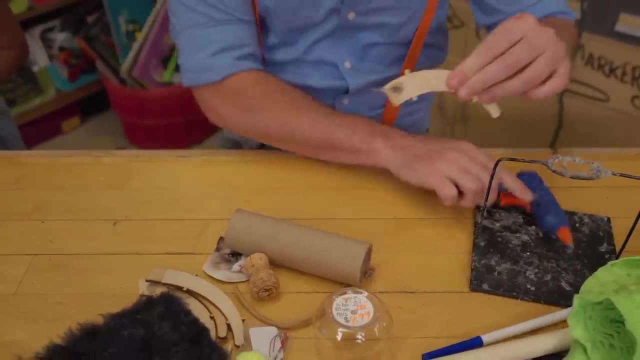 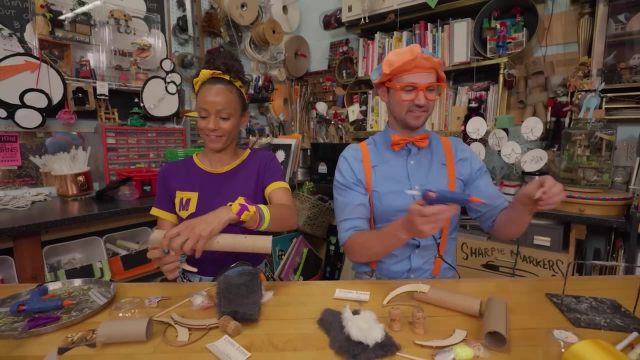 It does. This is some hot glue And you always want to have a grownup. help you. if you're using hot glue, Let's put on the legs. There's one leg right here. Okay, Here we go. Okay, Wow. 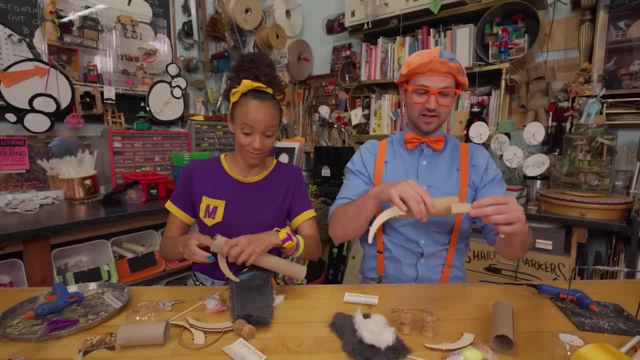 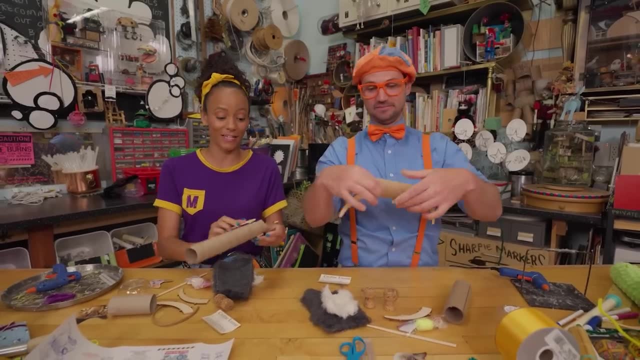 This hot glue is so cool. Yeah, It's very hot when it comes out of that hot glue device And then it cools down and then it's sticky and dries, Yeah, And it sticks really well. Aw, All right. 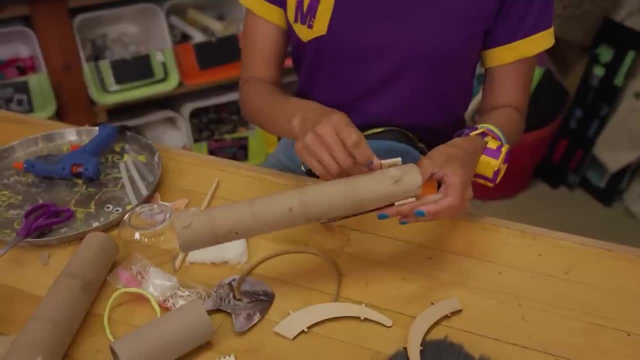 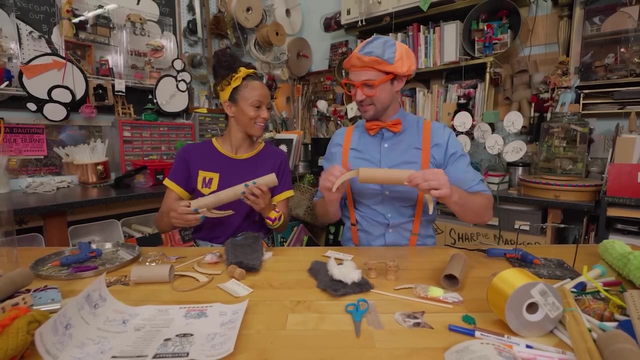 Here we go. How are your legs coming? Pretty good, I have two on so far. I'm going to make a really long cat. Whoa, Yours is really long. Wow, I'm going to make a medium-sized cat. It looks like this cat body would make it really small and short. 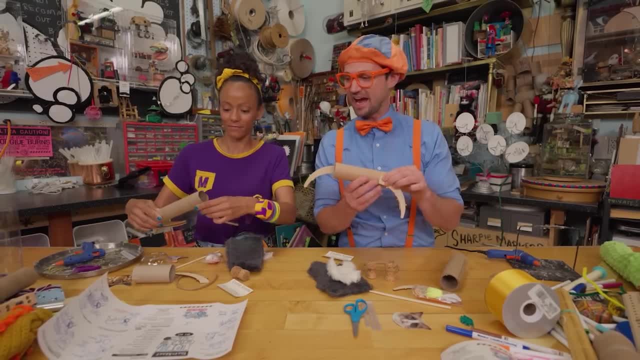 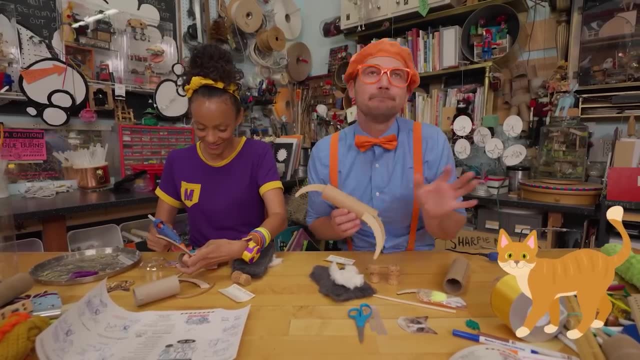 Like a little kitten: Meow, Meow. Look With my legs going this direction. it looks like my cat's running. Whoa Cool, You're so creative. Wow, Thanks, Whoa, But my cat can't see because it's too big. 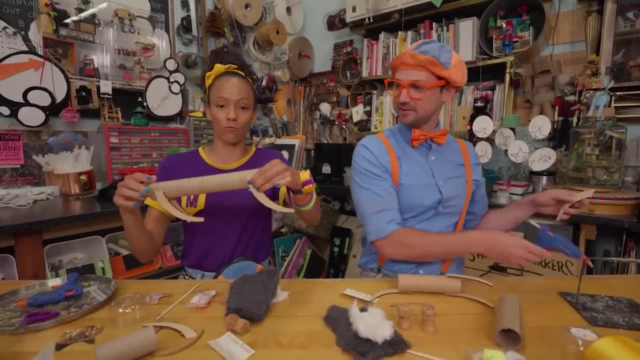 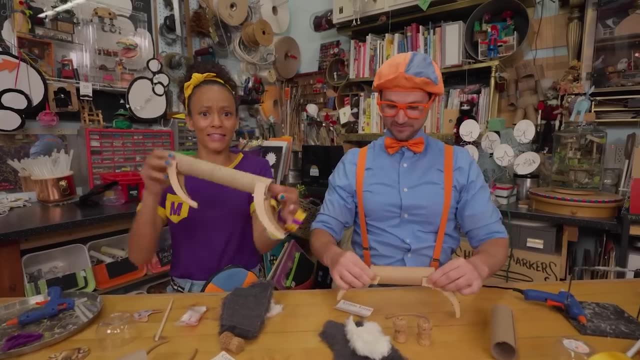 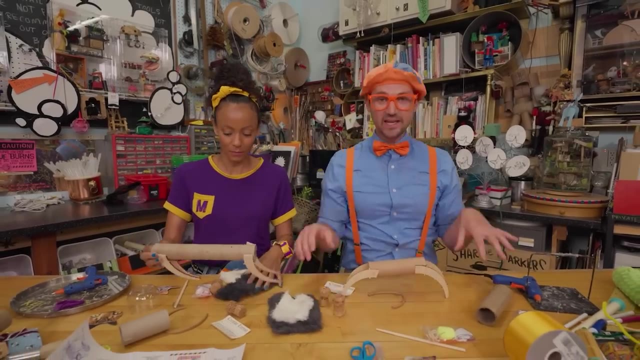 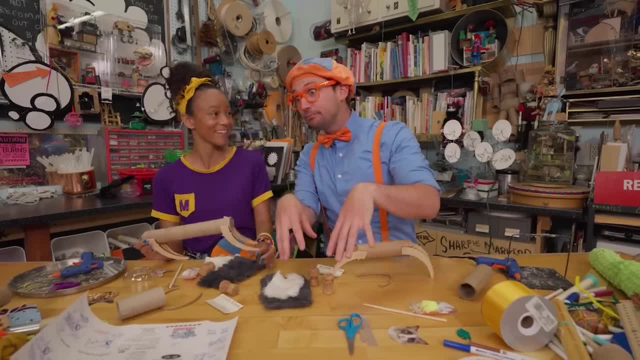 I'm hungry, Please feed me. I'll run and get you some food. Where'd I go? I can't see You're so funny. All right, Let's see I'm going to put my fur on next, I think. 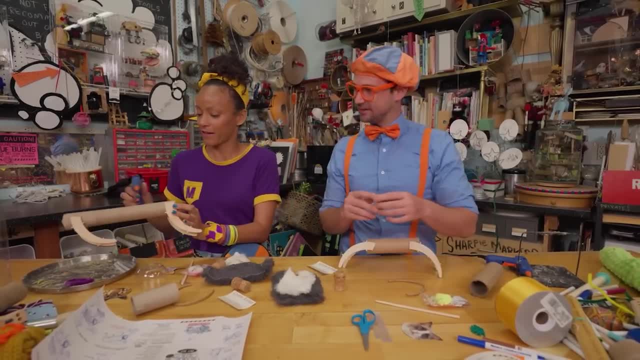 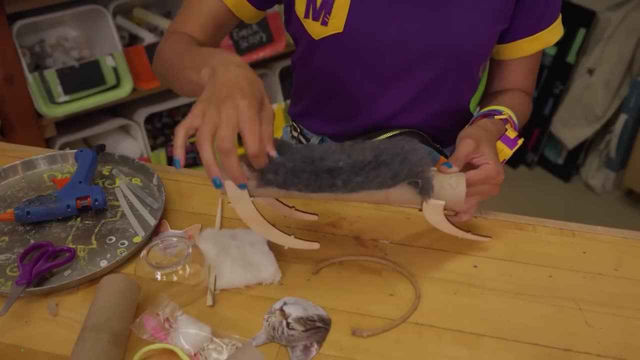 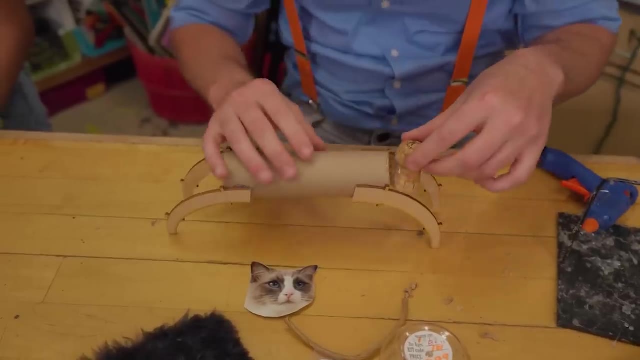 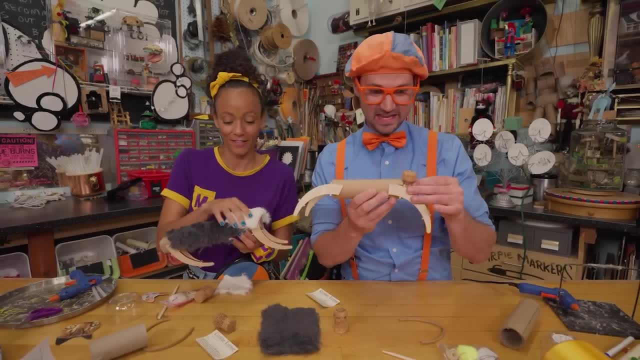 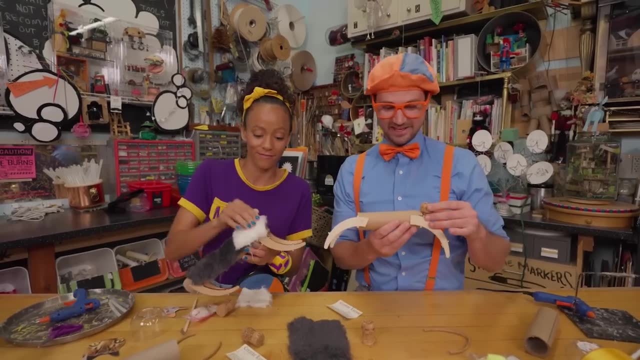 Do you like crafting things? Yeah, So fun. You can make anything and everything. Yeah, You just have to be creative. Yeah, And use your imagination. That's my favorite. Yeah, You are very good at being creative and using your imagination. 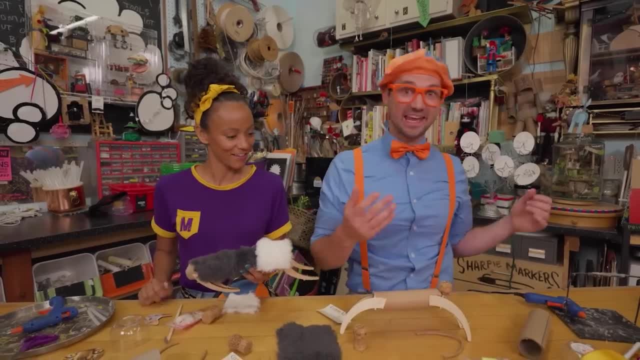 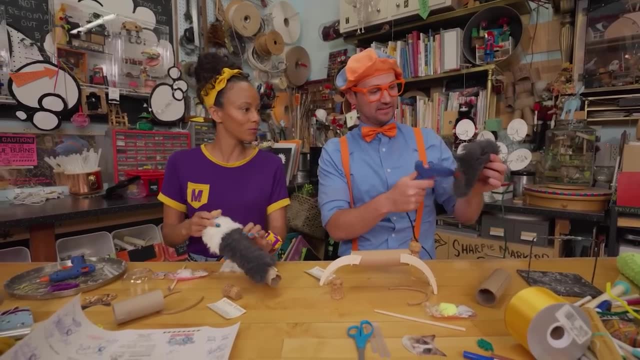 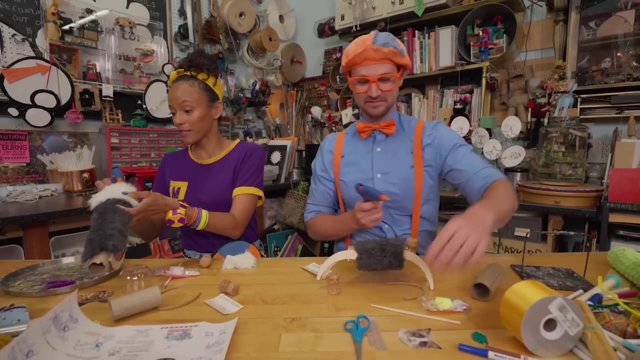 Sorry you Blippe. Yeah, I didn't even think about making the cat run super fast. Whoa, All right for my fur. yeah, oh go. hmm, our cats are the same color. yeah, i wonder if they're siblings or best. 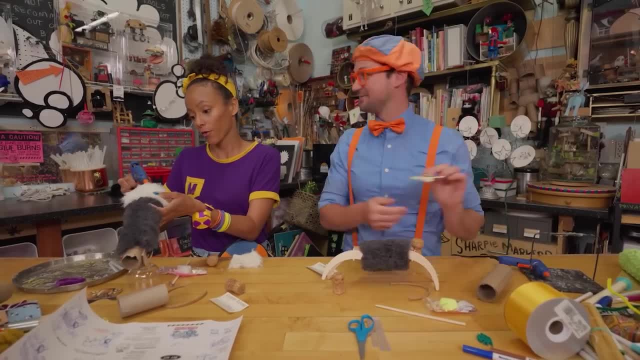 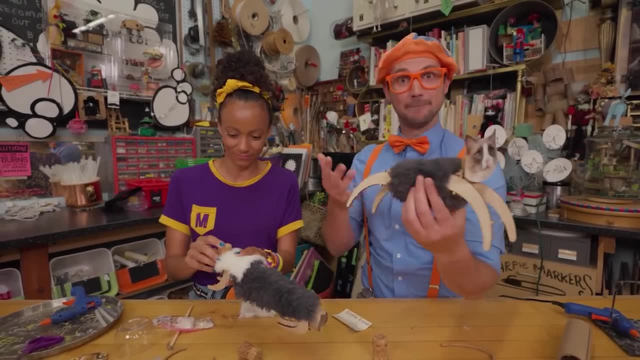 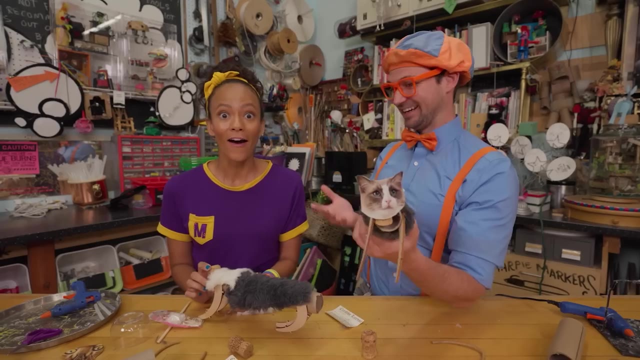 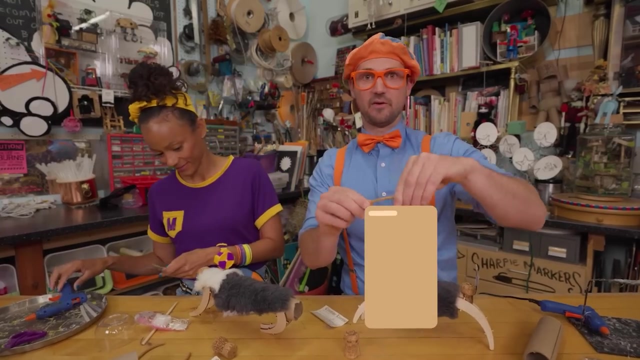 friends or cousins. maybe they live in the same neighborhood. oh yeah, how's my cat looking? whoa so cute. yeah, what's my cat missing? hmm, let me see legs, fur, cute little face. um, a tail. yeah, okay, looks like a tail, right? yeah, it used to be a top of a bag, i think. yeah, the. 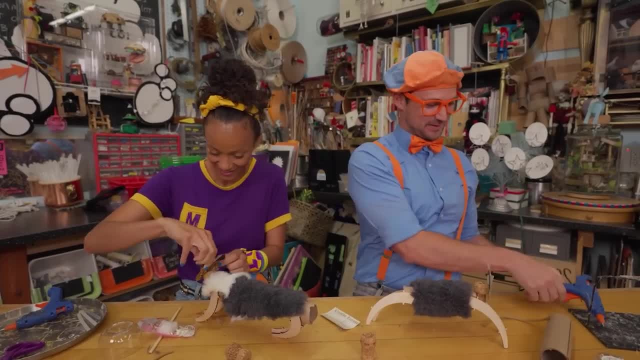 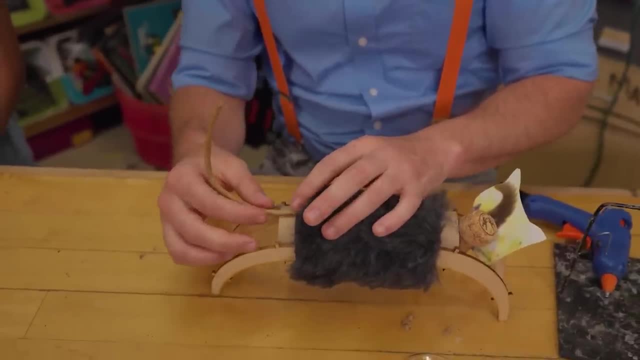 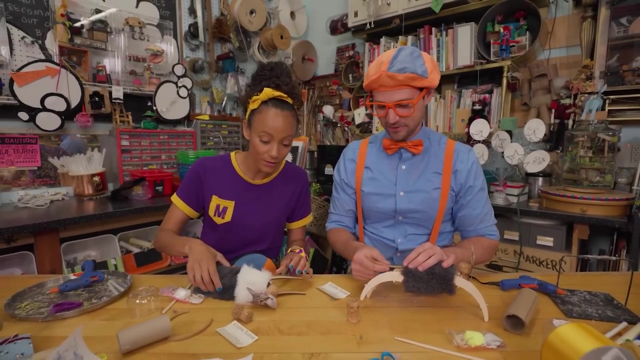 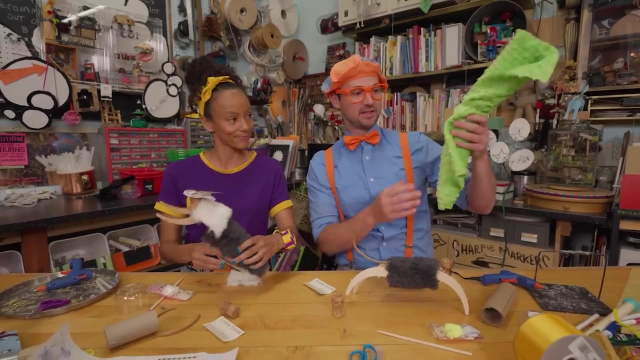 handle. all right, i'll put some hot glue on this. wow, there we go. oh, your cat is so cute, wow. and look at its eyes, they're very green, really green. wow, wow, hold it on, so it sticks. oh hey, i have an idea. why don't i cut some of this green felt? 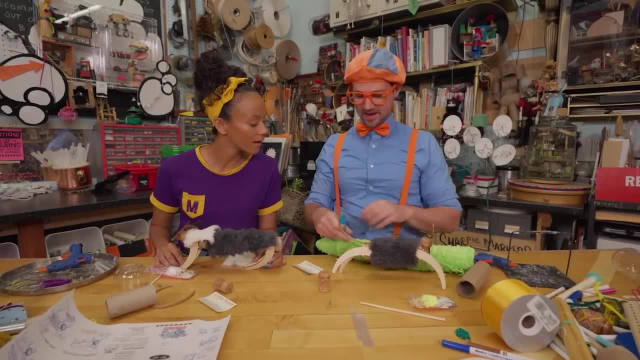 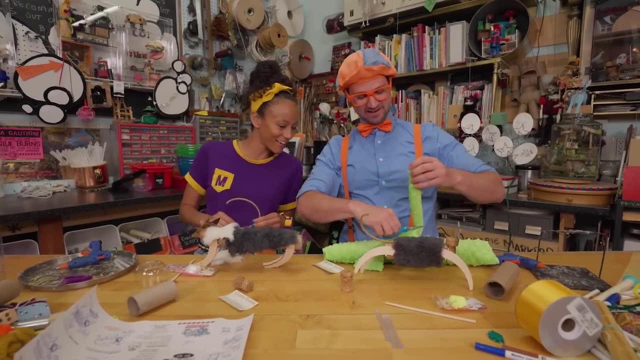 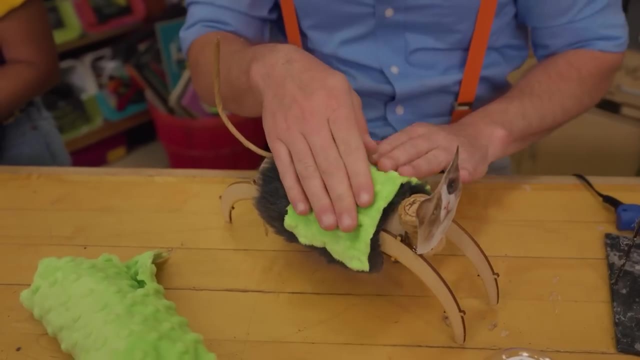 material, these scissors, and i'm gonna make a robe. oh, fancy cat. yeah, like it just got out of the bath. whoa, there we go. oh, this is so much fun. here you go, kitty, there you go. wow, meow, meow, flippy. what are you gonna name your cat? 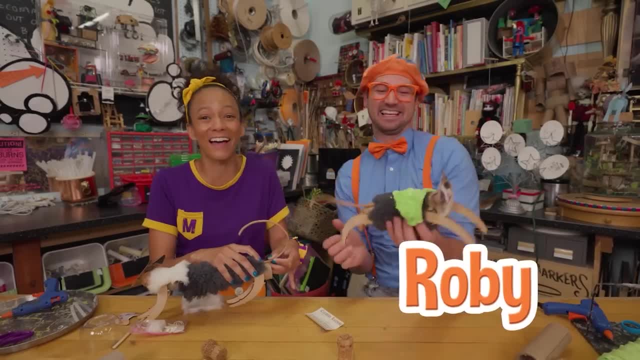 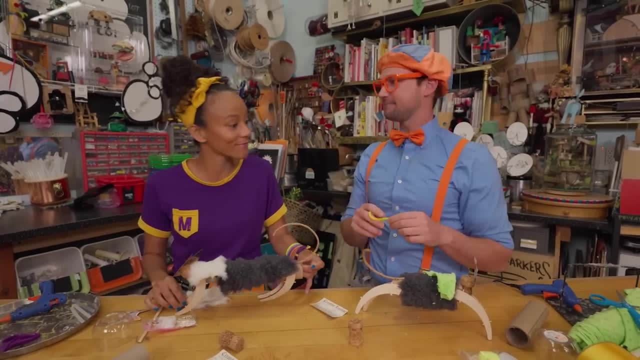 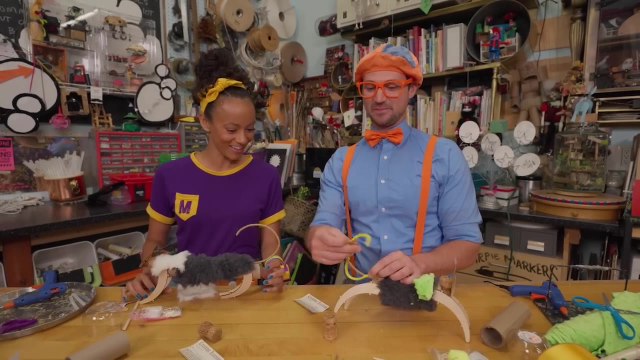 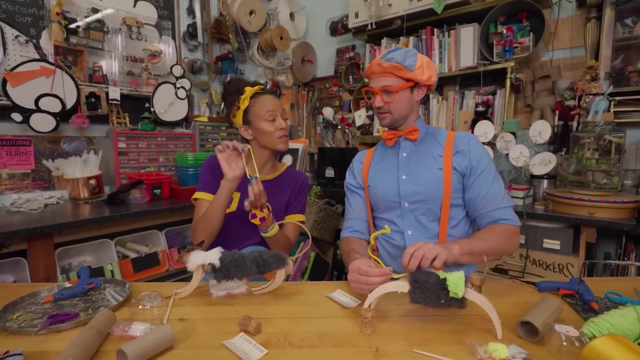 um, roby, roby, i love it. it loves robes, wow. and then look at this: my cat is so extravagant, wow. yeah, it loves to decorate its tail when it goes out in public. that's such a good idea. yeah, great way to express yourself. yeah, i think my cat's gonna wear a little scarf. oh cool, it's a little. 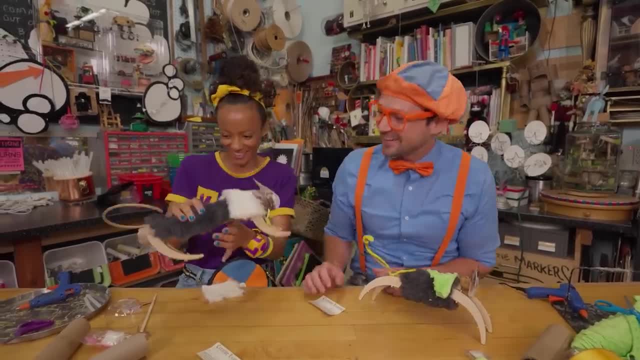 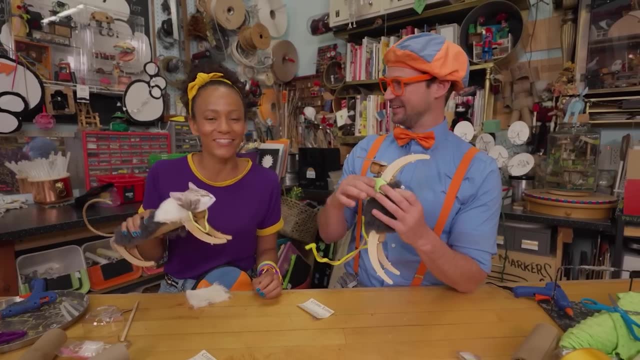 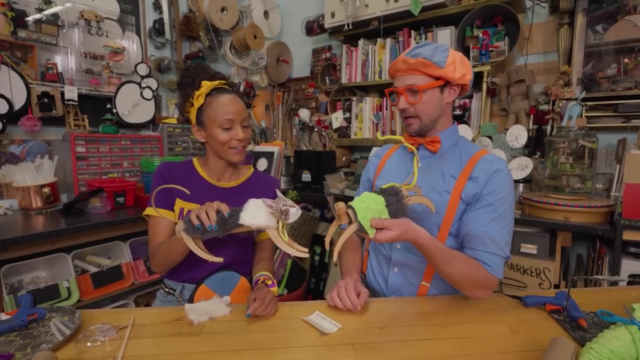 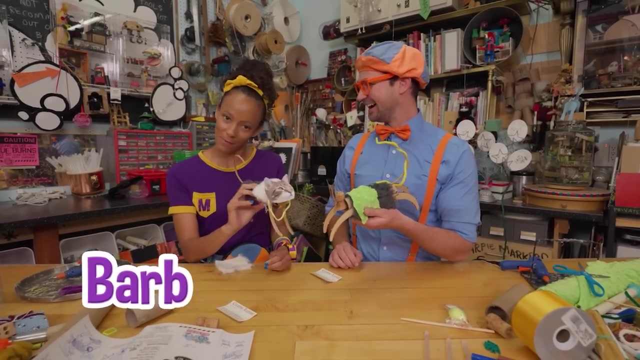 chilly. oh, there you go, kitty. oh, this has been so much fun. wow, i love repurposing things we do. robie, yes, would you like to go for a light jog with me? um, wait a second. i need to know your name first. i don't go on walks with strangers. i thought you'd never ask. my name is barb. oh, nice to meet. 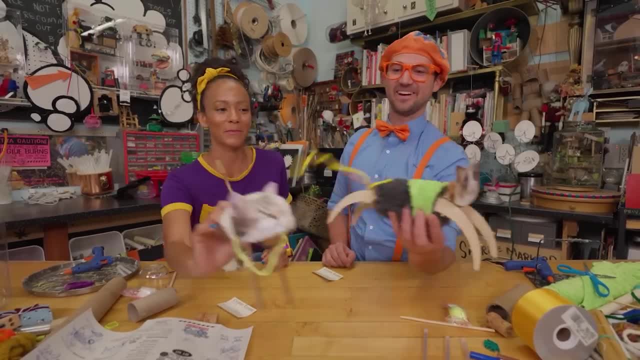 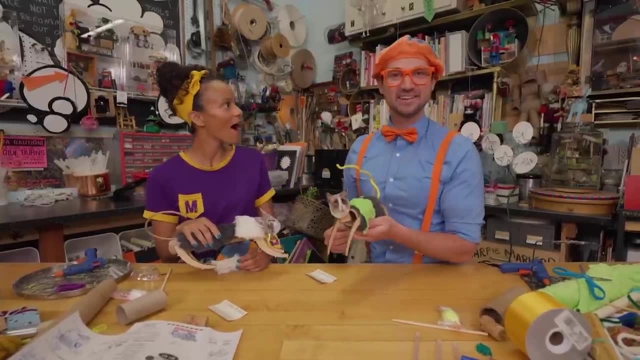 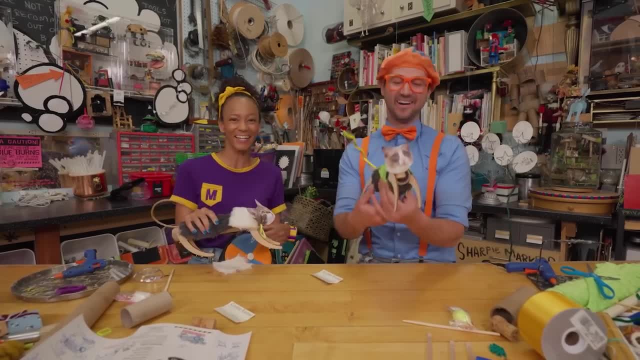 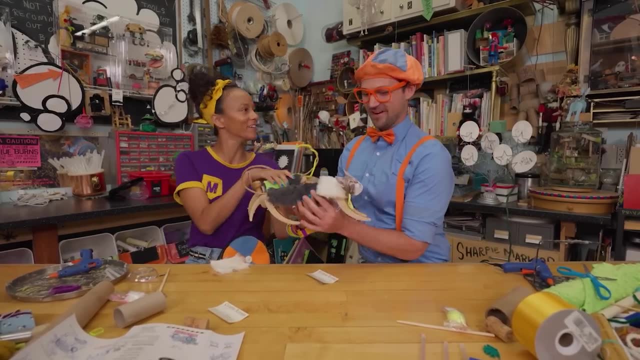 cat for you as a gift, because i know you like to run fast. oh, that's awesome. well, i know that you love rogues, yep, anything cozy. well, here's ruby for you and here's barb. oh hi, barb. oh ruby, i love you. you're so cute. 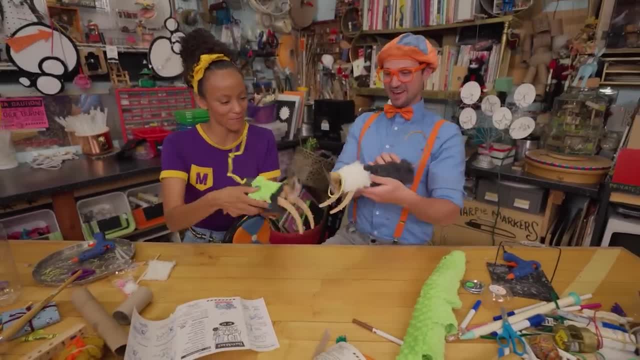 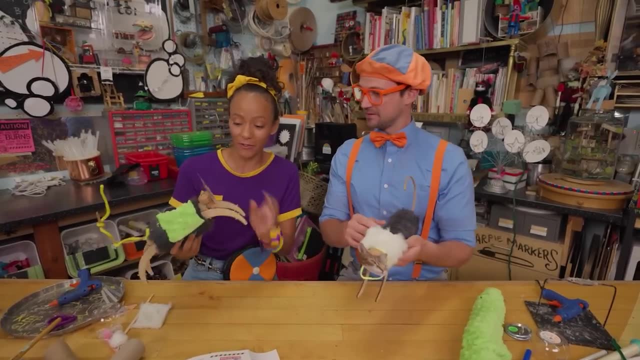 Meow-meow-meow-meow, Meow-meow-meow-meow, Meow-meow-meow-meow, Meow-meow-meow-meow. That was so much fun Making these cats together. Yeah, It's really cool how you can repurpose these materials. 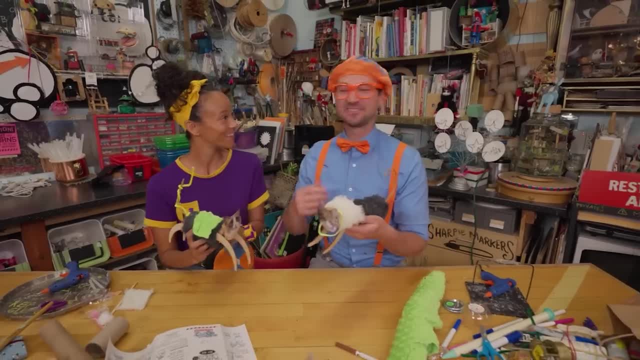 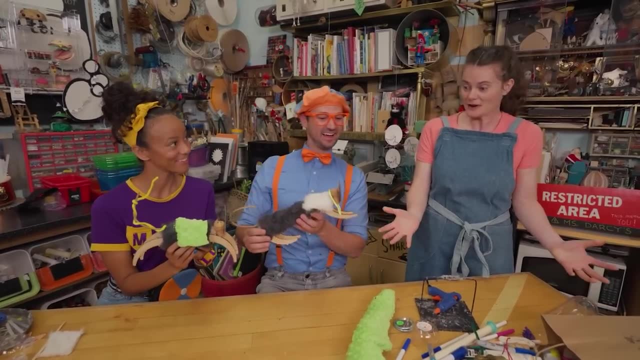 to create a little cat. Yeah, And I love being creative with you, Me too. Hi you two, How did you do? Oh, you tell us How did they look? They look like pretty great cats. Look at their little faces and their different tails. 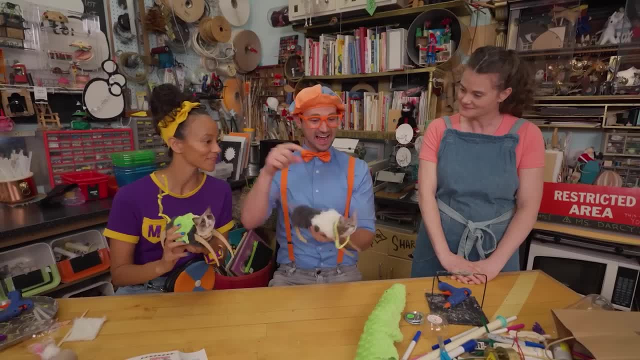 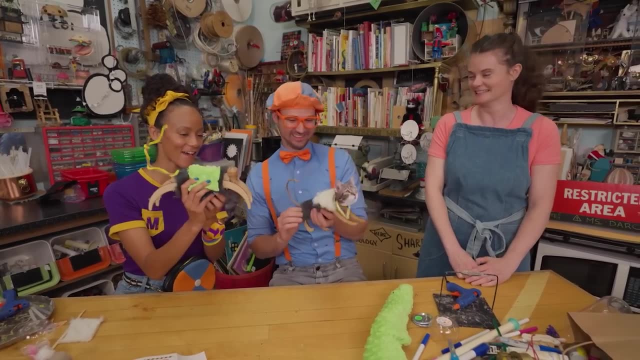 Yeah, Thank you. We had a lot of fun making them. Yeah, And we even named them. Yeah, Barb, hi, Barb, and this is Roby hi. thank you so much for having us. that was really fun. yeah, thank you, thanks for coming in. well, I'm gonna head back to 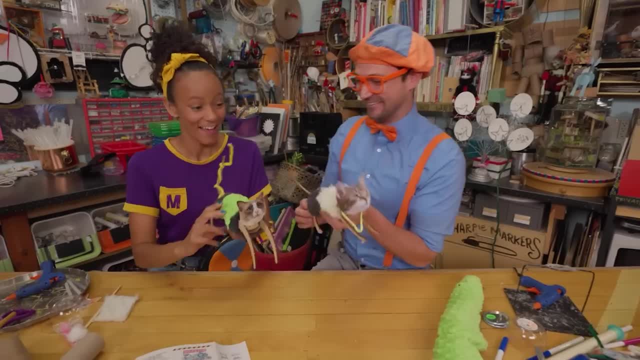 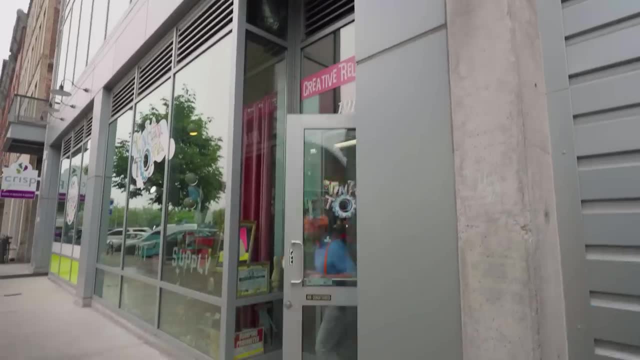 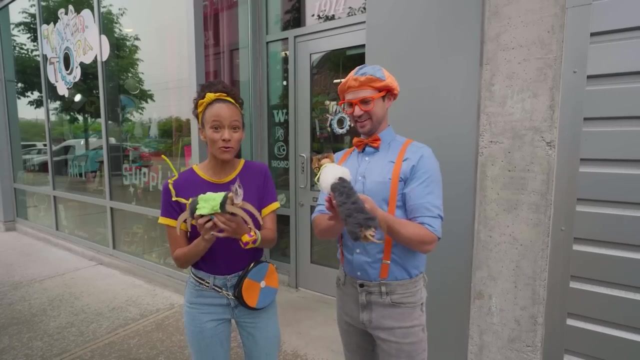 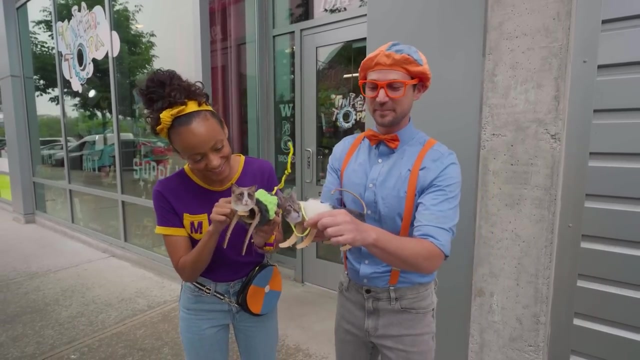 work. see you later. all right, so much fun making these crafty cats together. it was so cool how you can use donated items and repurpose them to make something new. yeah, it was, and it was so much fun being creative. oh yeah, you made a scarf for my. 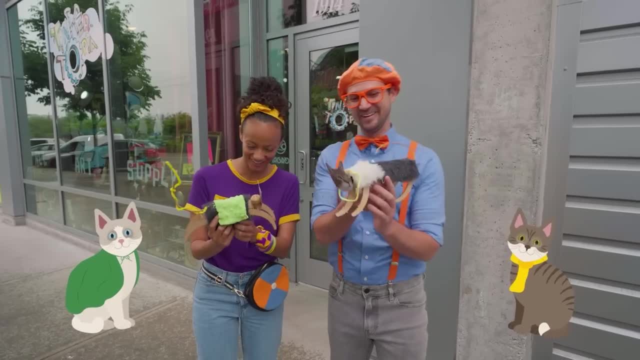 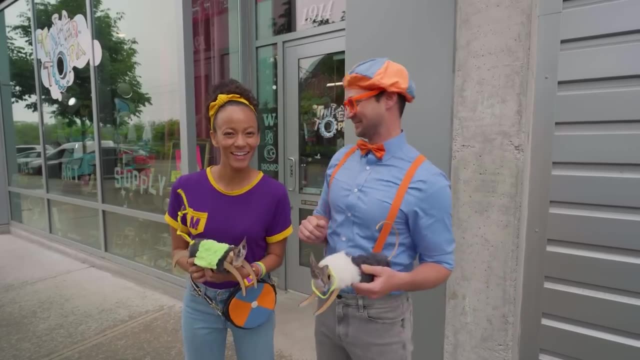 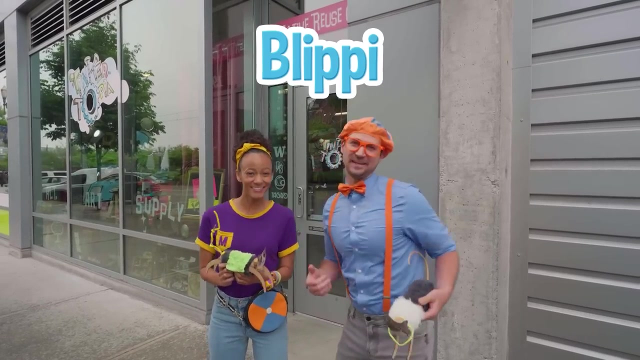 cat. yes, and a rope for Roby. oh wow, that was so much fun, hey. if you want to watch more of my videos, all you have to do is search for my name. will you spell my name with us ready? B L, I, P, P, I, Blippi, good job. 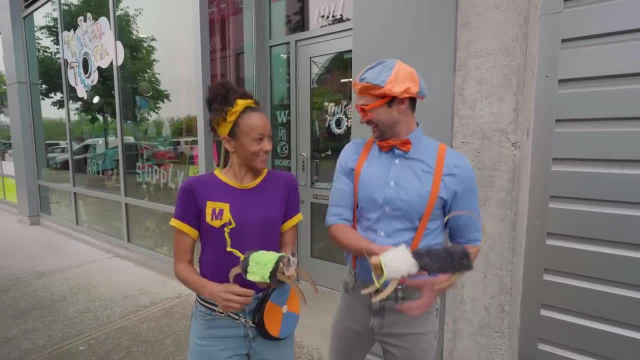 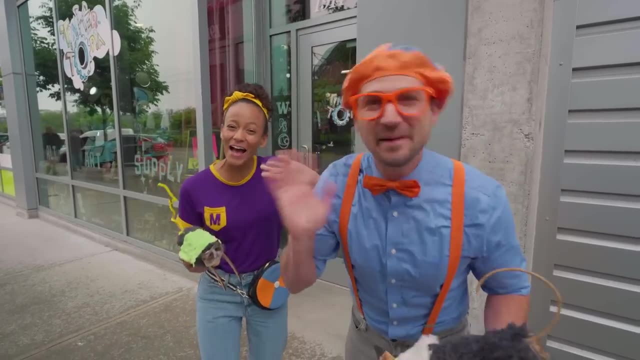 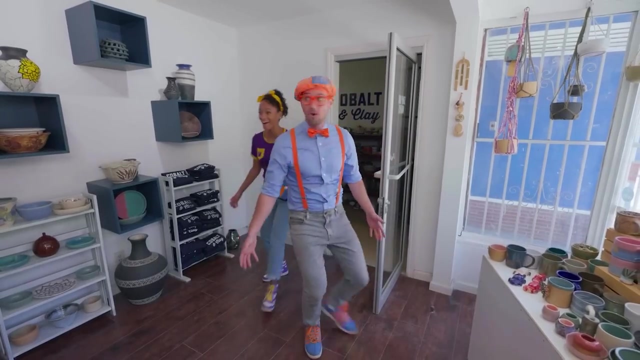 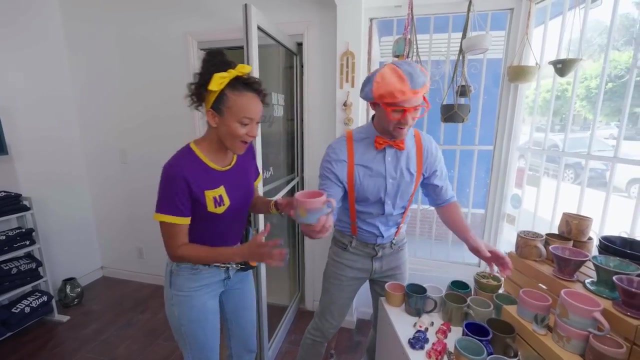 hey, will you spell my name with us? cool, N E E K A H, Mika. all right, see you again, bye-bye. wow, Mika, cool. yeah, this room is filled with different art pieces. yeah, check it out here. do you want one? oh, yeah, thank you. wow, unicorn mugs, these are so cool. cheers. 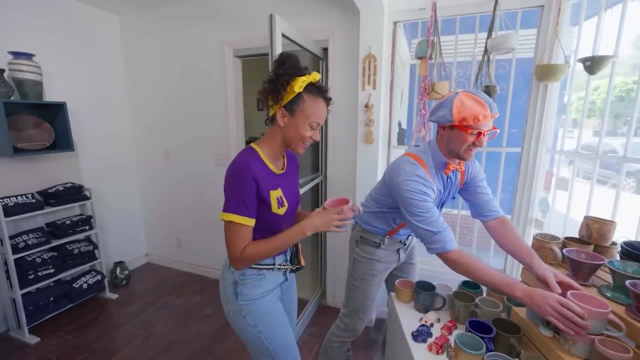 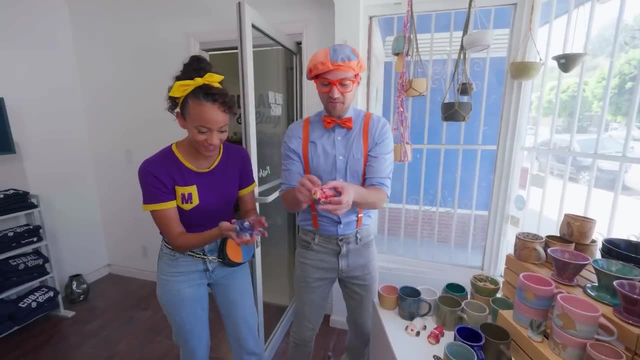 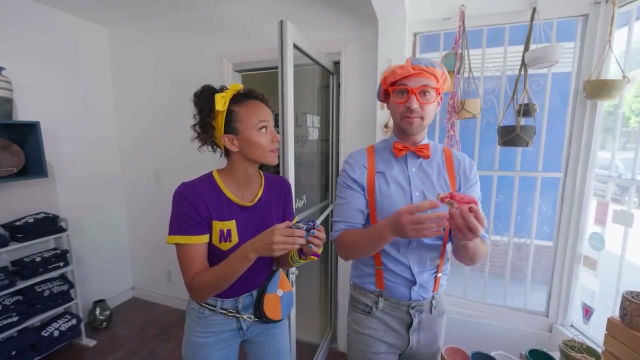 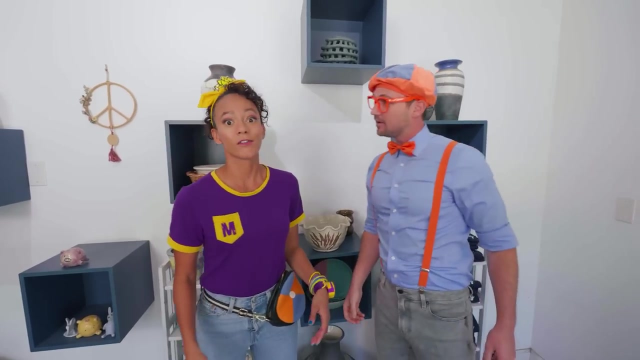 oh, there we go. nice and gentle, yeah, there we go. oh, check it out, cool cars- mine is blue and mine is red. so cool that you can even make cars out of clay. yeah, awesome. well, this pottery is so cool. new pottery is an art piece, that's. 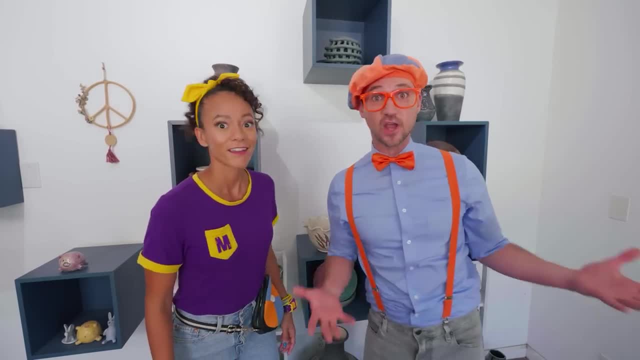 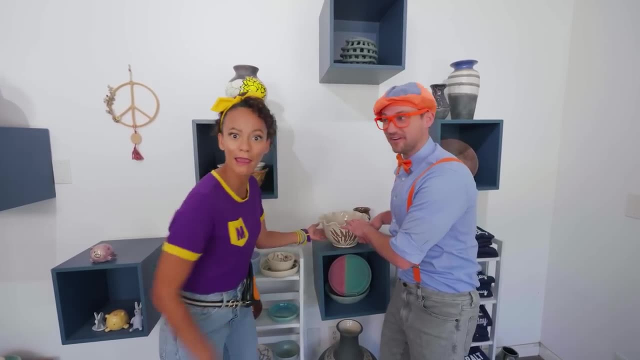 made out of baked clay, yeah, or other types of stuff, stoneware. yeah, it's really cool because it starts soft and squishy and then it ends up like this: it's nice and hard, yeah, oh cool. hey, look at this. oh, I'm being very careful when I hold these. 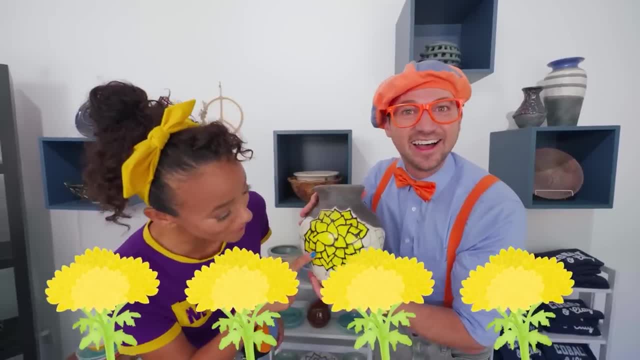 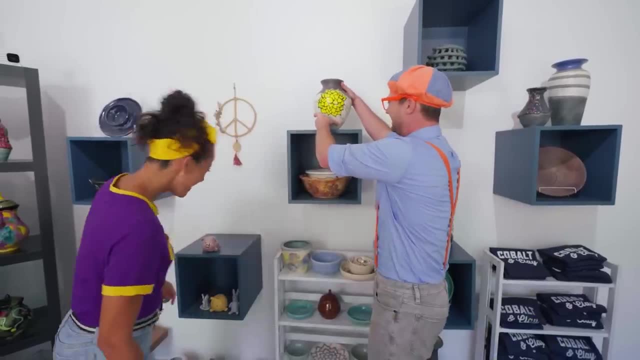 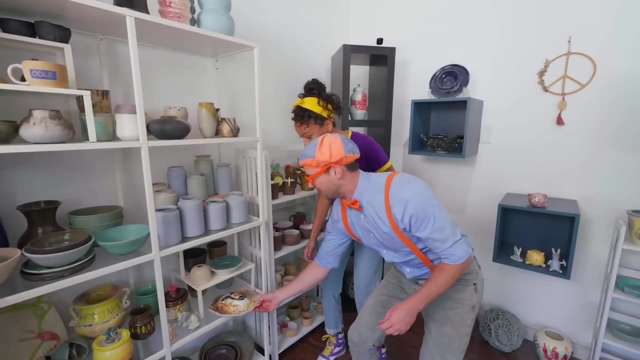 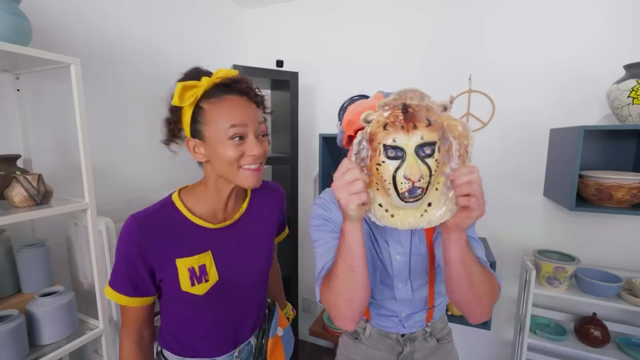 good job. yeah, a yellow flower. yeah, it's so pretty. yeah, smells just like clay. you're so silly. oh cool, whoa, do you see what I see? yeah, I do. whoa ready. do you know what animal that is? a lion. yeah, yeah, will you act like lions with us? 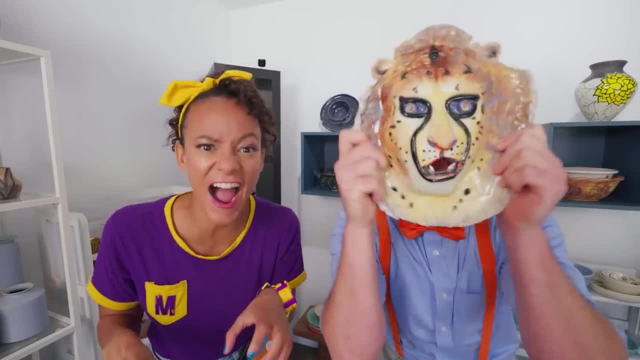 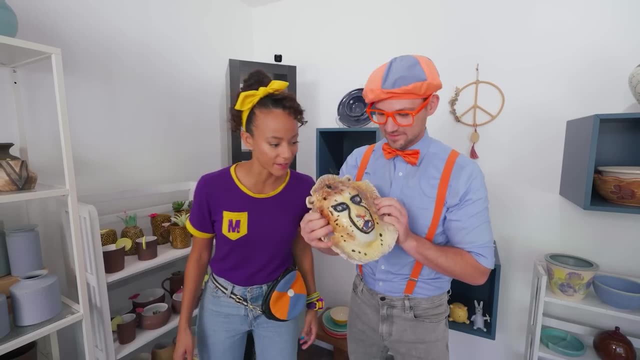 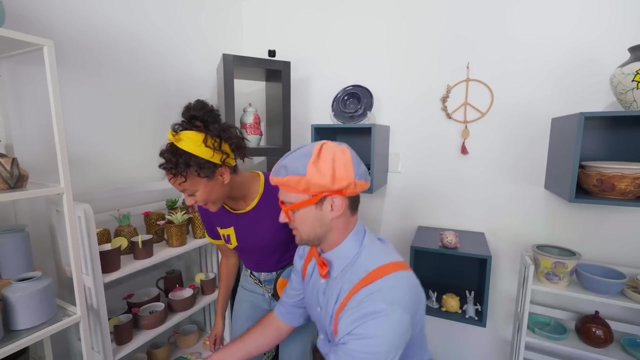 whoa, so cool that an artist made this lion out of clay. yeah, it's pretty awesome. yeah, and it's so colorful too. they must have painted it. yeah, look at the blue eyes. whoa kale, whoa very gentle when I set that down. nicely done, oh, thanks. 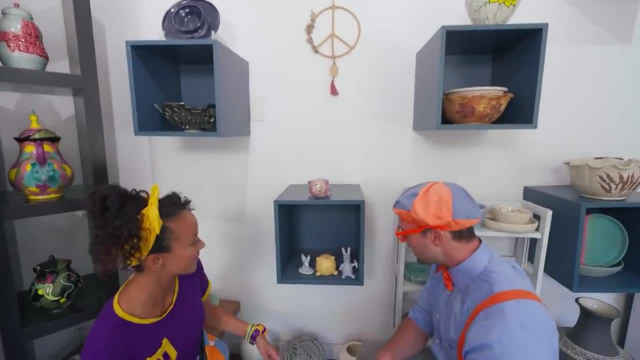 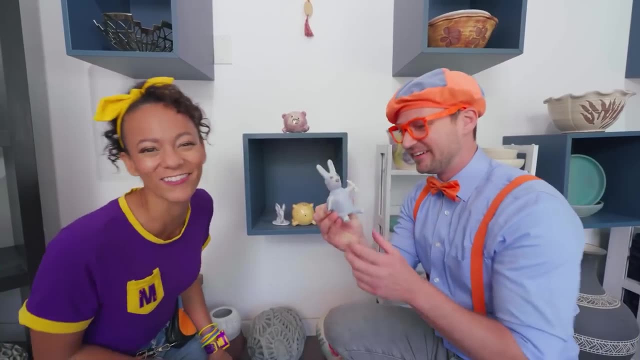 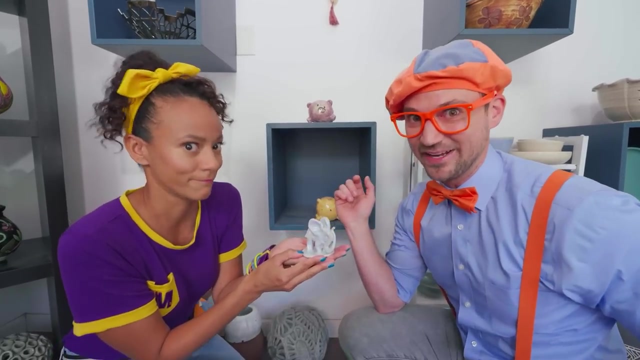 hey, Blippi, there's more animals down here. oh, yeah, you're right. look a bunny rabbit. aww, nice little carrot right there, it's so cute. oh, oh, what about this little elephant? aww little elephant but big ears. you got that right. oh, and look at this one. 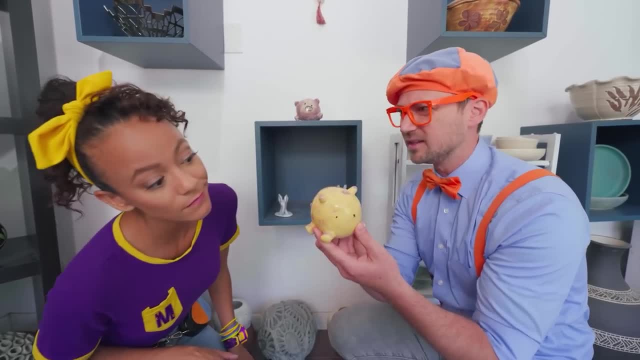 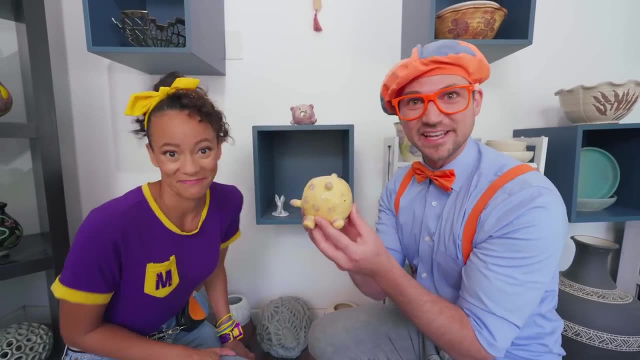 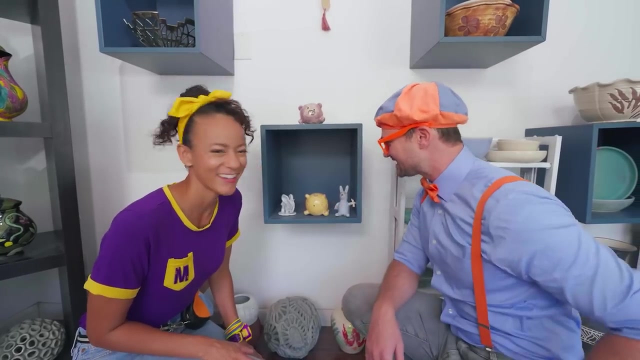 oh, what is that, do you think? huh, maybe a leopard? oh yeah, and it's really big, almost like a blowfish, but it's not a fish. yeah, so artistic, yeah, really cool. you can make anything you want. yeah, and it's so cool that these animals, yeah, are nice friends together. 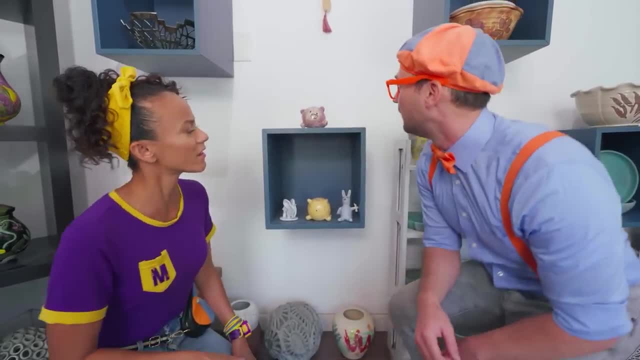 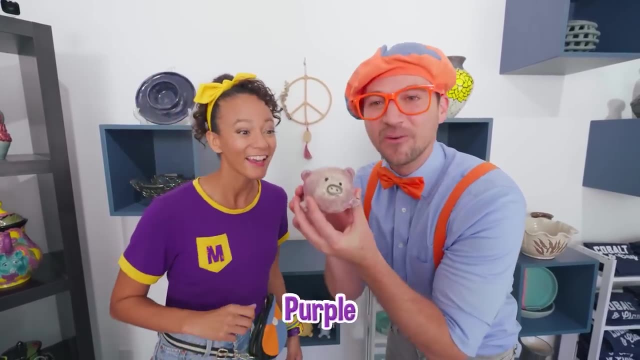 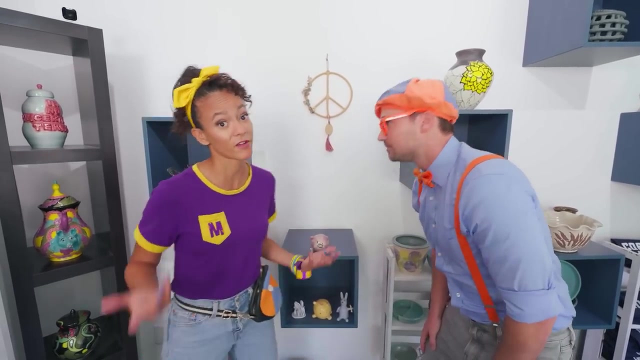 aww, so cute. yeah, oh look, there's another one up here. oh, interesting, looks like a pig right. yeah, and purple, one of my favorite colors, oh yeah. oh, wait a second, it's all alone. yeah, and it looks like there's some space for other animals. are you thinking what I'm thinking? 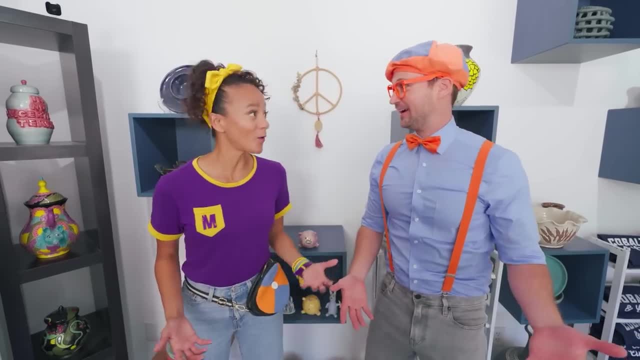 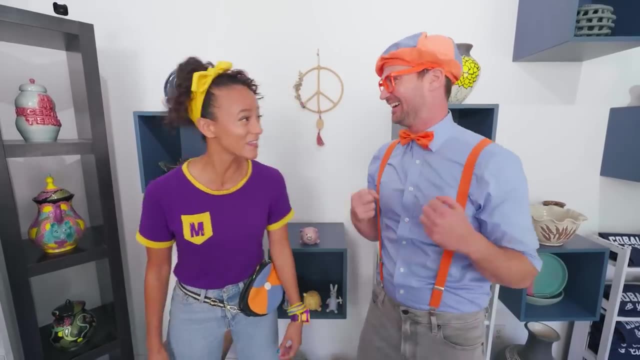 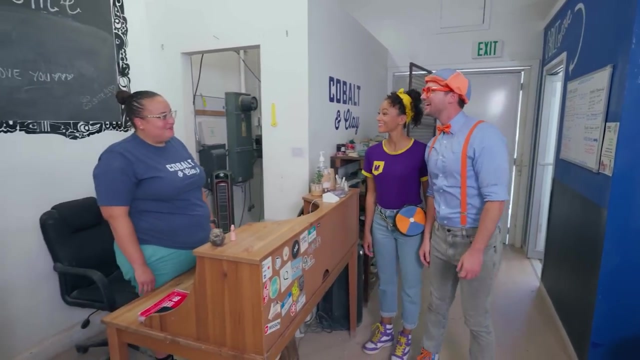 yeah, lunchtime. no, oh, we can make this pig some animal friends. oh, that's a great idea, Minka. yeah, let's do it. yeah, oh, oh. hey, who are you? hi guys, welcome to Koopa and Clay. my name's Nicole. oh, nice to meet you. I'm Blippi. 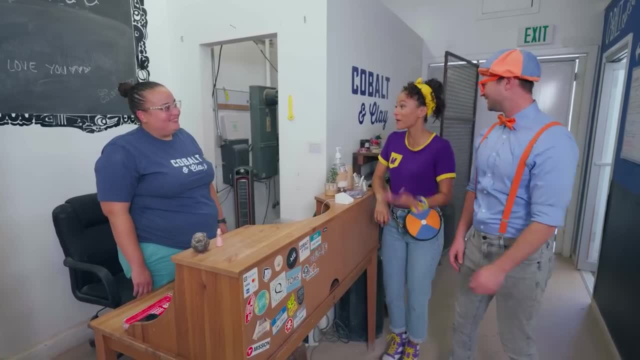 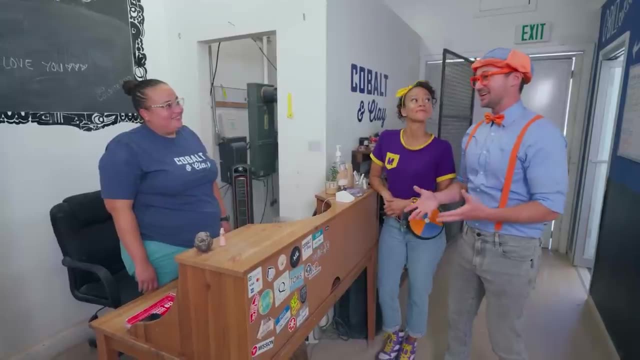 hi and I'm Mika. oh, so what do you do here? um, I'm the owner and instructor, oh cool. well, you might be the perfect person to ask: do you think we could make some pottery today? of course, oh yeah, we want to make some animal creatures. 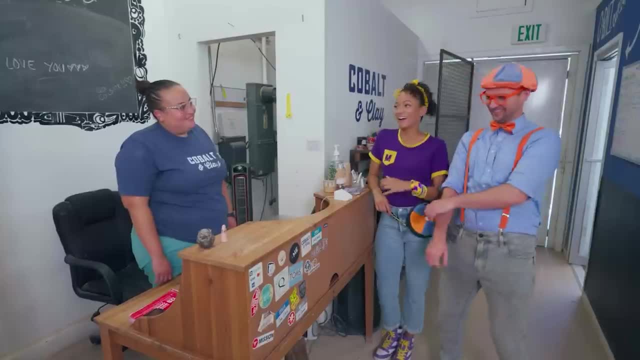 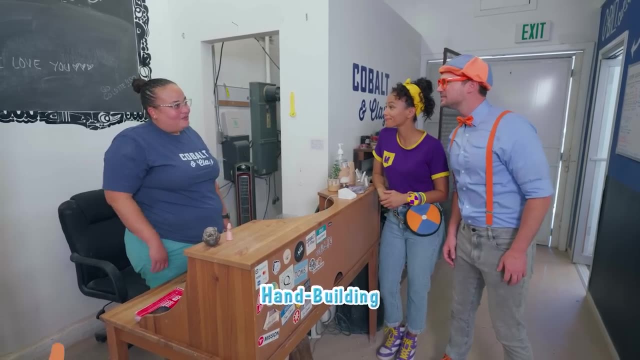 awesome. well, would you like to hand build or throw? what's the difference? well, hand building is where you use your hands to sculpt, and throwing is where we use the pottery wheel that spins. oh, could we do both, of course, yeah, oh, oh, oh, oh, oh, oh, oh. 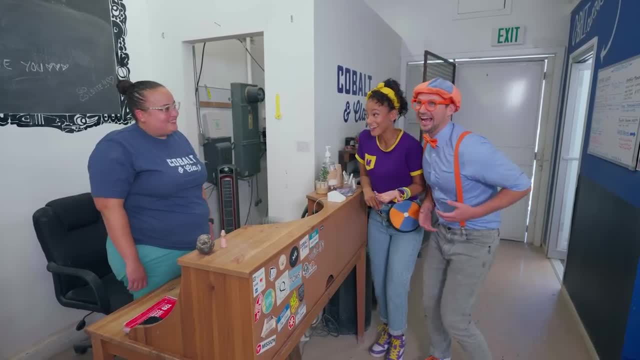 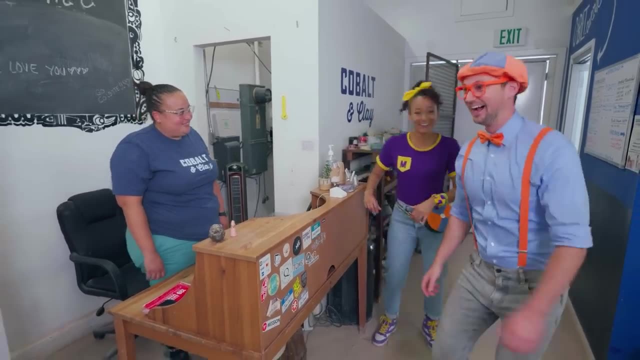 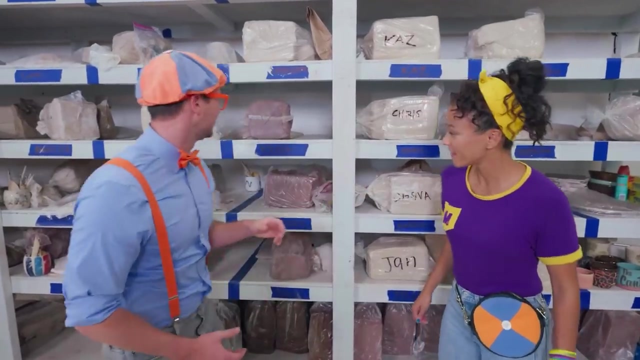 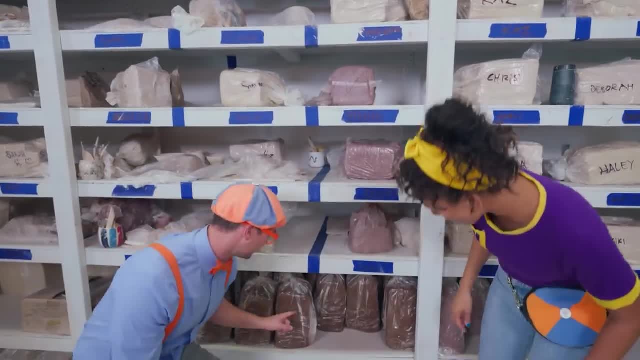 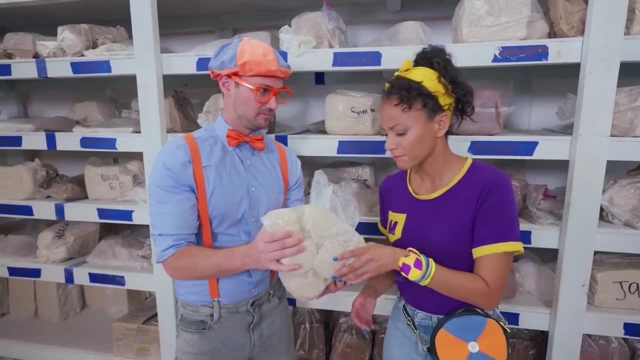 big blocks of clay. it looks like: yeah, oh, look at this one kinda looks red. yeah, you're right, almost like a brick, oh yeah, look down here. oh, this was like a dark brown, oh yeah, oh, and look at these, a nice tan colour. yeah, in the shape of balls, it looks like. 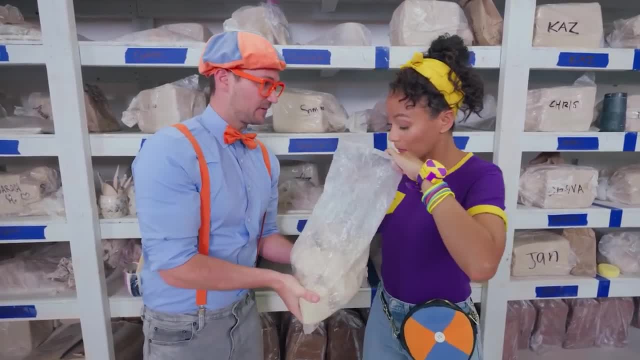 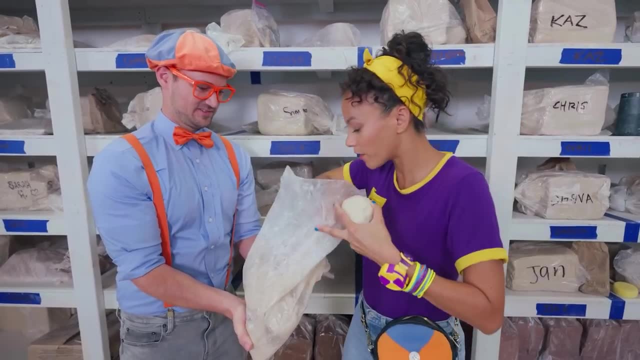 yeah, interesting, shall we? I wonder if they're the perfect size. Oh, check it out. Oh, cool, Yeah, There you go. One for you, Oh, thank you, And one for me, Oh, cool, Oh, and I have a great idea. 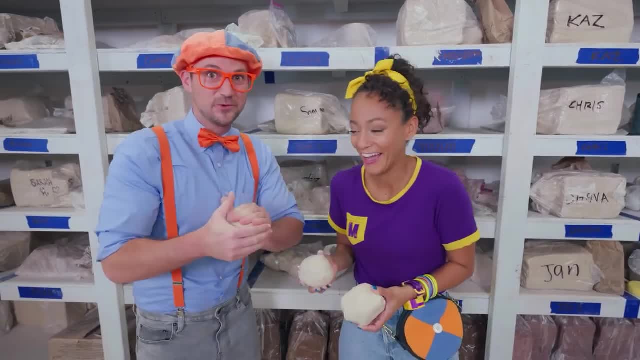 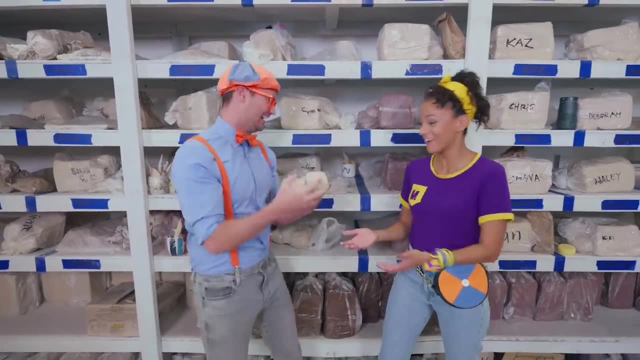 And since they're pieces of clay and they won't get ruined if they fall on the ground, I know what you're going to do. Yeah, here we go, Go flip it. Yeah, Nice job. Thank you very much. I should probably put this third one away, right. 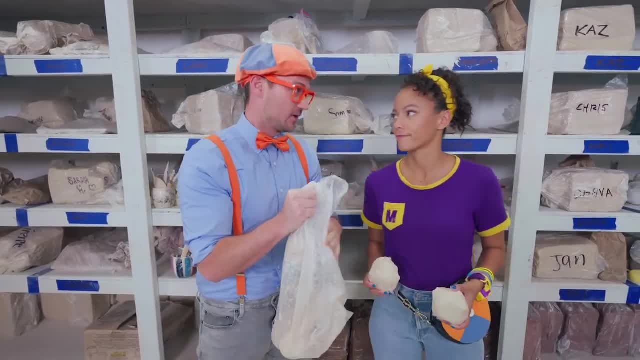 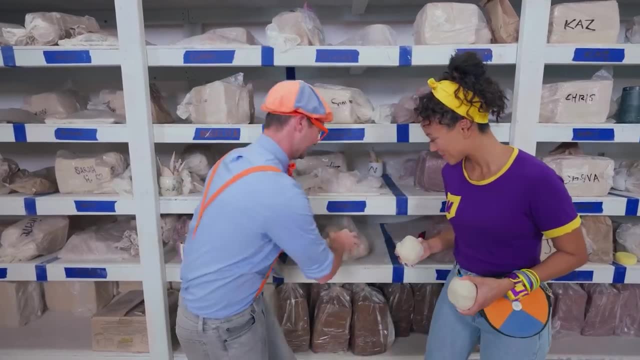 Yeah, Let's seal up the bag so then they don't dry out, right? Good idea, All right, Nice twist, All right, There you are, There we go. All right, Oh, check it out. Oh, scales. 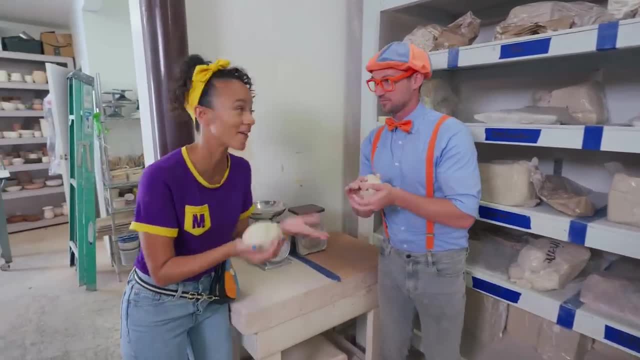 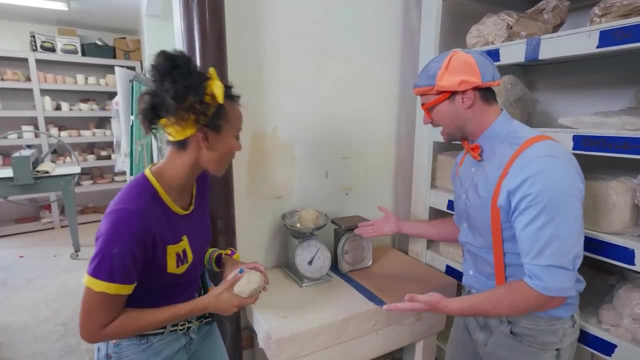 Yeah, Whoa, We can weigh our clay. Yeah, do you want to go first, or me? Oh, you go ahead. Oh, thanks, Mika. All right, Okay, there we go. Oh yeah, Looks like one pound. 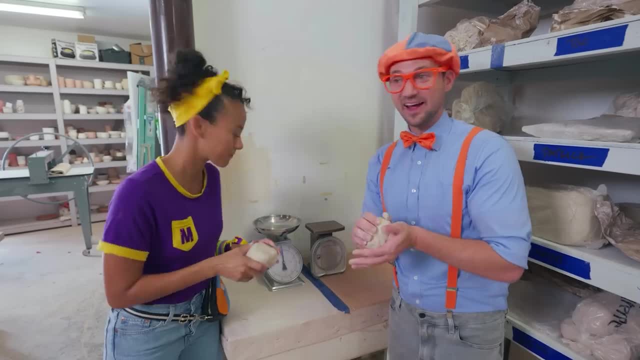 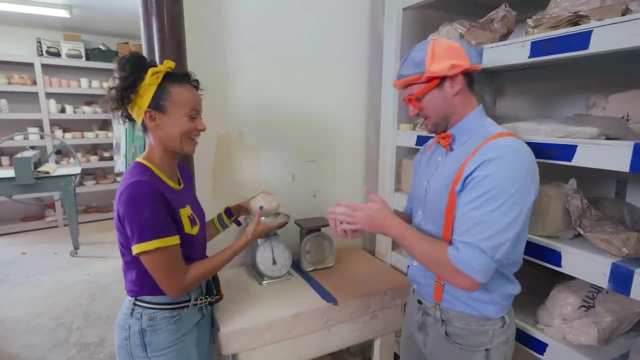 Oh nice, I wonder if mine's going to be the same or different. Yeah, Oh, also about one pound or half a kilogram, So silly. Well, I think they're good, shall we? Yeah, let's get started. 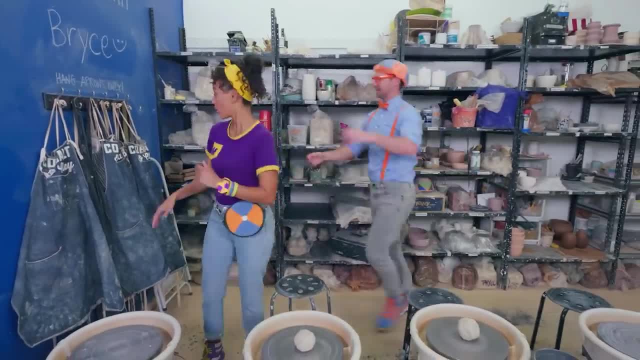 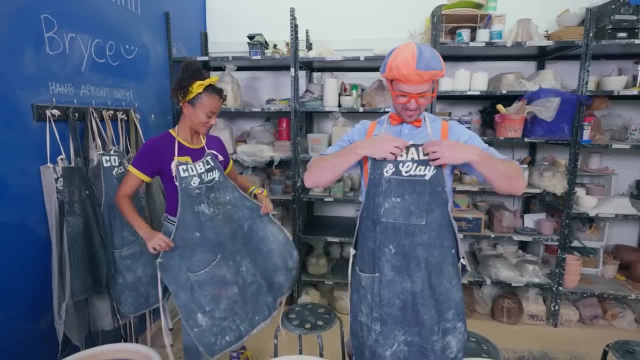 Okay, I'm so excited, Me too. Okay, we'll set that there. Aprons- Whoa smart. So then we don't get dirty. Yeah, this will protect our clothes. Yeah, And it even says cobalt and clay. 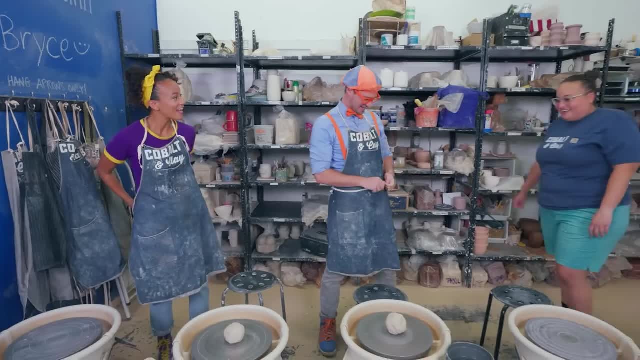 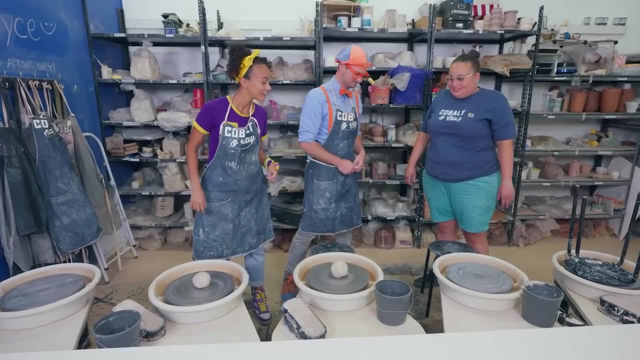 Oh, cool Matching aprons. Yeah, Oh, hey, Hi guys. Hey, Nicole, Are you ready to throw? Yeah, Throw, clay. So I'm going to go over a few things that we're going to be using. 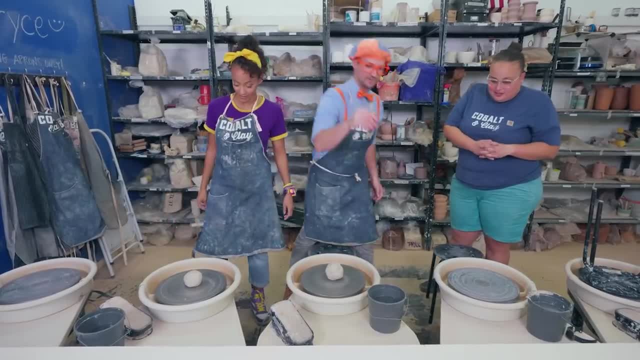 So we have a bucket of water here that's going to help the clay glide through our hands. And then the way the wheel works. there's a foot pedal on your table. You're going to set it on the floor and that's going to control the wheel speed. 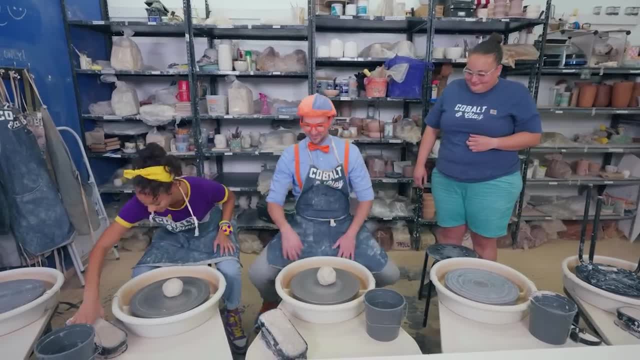 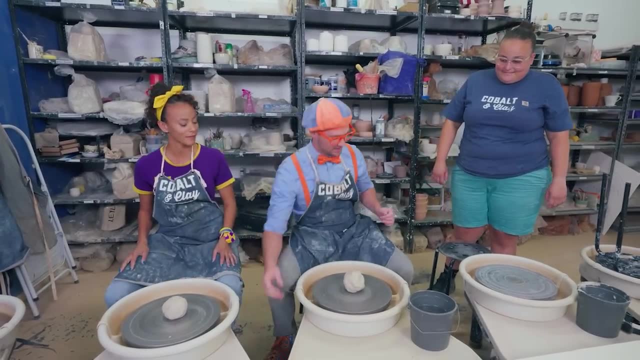 Okay, and do we sit down? Yeah, you're going to sit on your stool. Cool, Nice and relaxing. Whoa Okay, Pedals on the floor And that's what you use to control the spin. And then what about the cobalt? 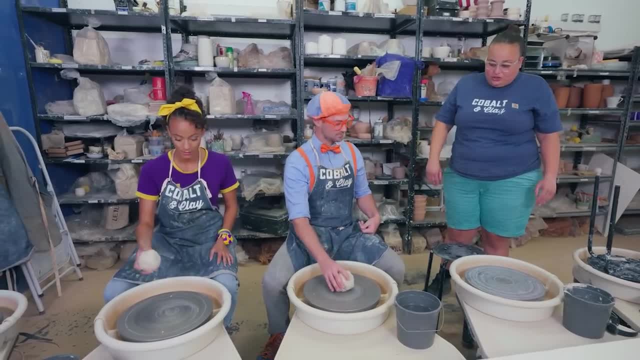 Clay. So you're going to take it, You're going to smack it in that center circle, You'll tap the sides really well, seal the base and then you'll just start to mold your piece. Sounds like fun. Thank you so much. 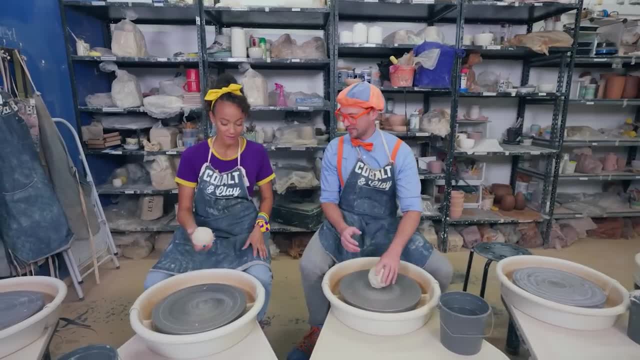 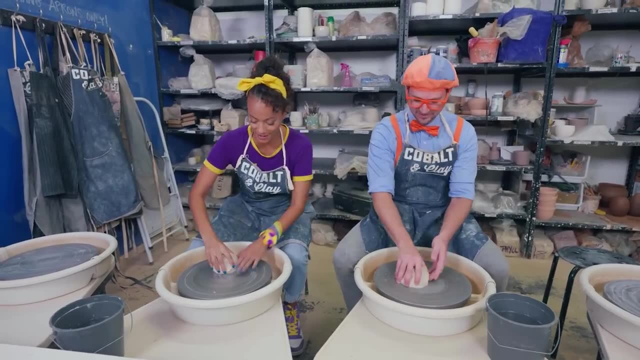 Okay, I'm going to set up our next station. All right, Thank you, See you. Okay, Ready to throw it, Ready to throw. I missed the center, Me too. We should probably do that again. Three, two, one. 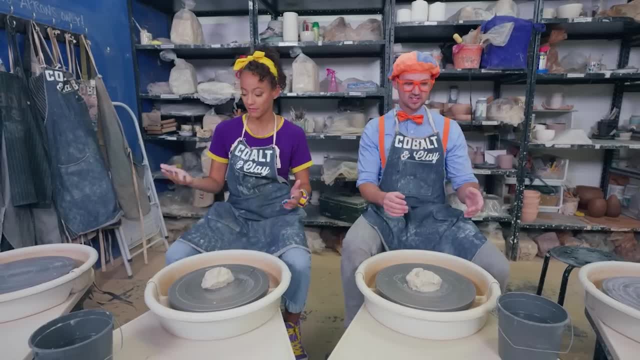 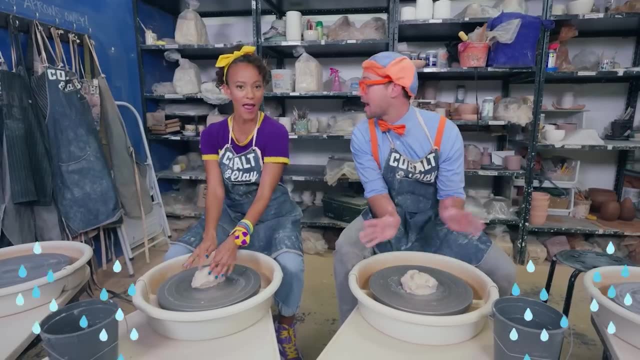 Yeah, Nice, Okay. and then I think she said to use some water: Oh yeah, On our hands, right, Let's water our hands. Okay, water our hands, Water our hands, Water, water, water, water our hands. 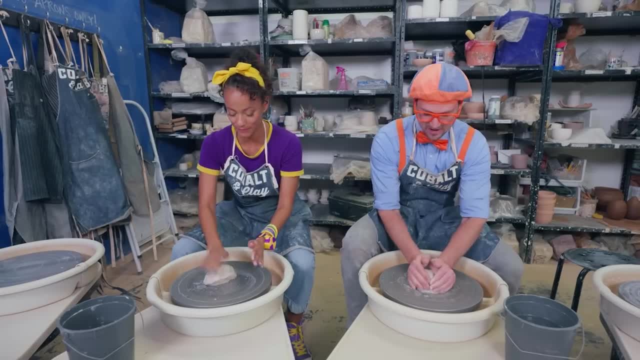 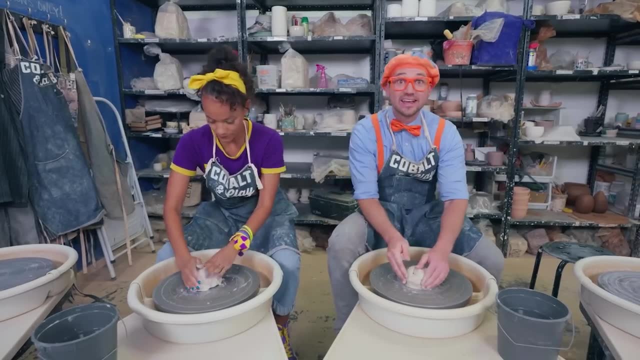 Okay. Okay, There we go. All right, Smack it, Oh. and then she said: seal it right. Oh, so maybe push it down. I think we go around the edges like this. so then it seals from this plate. 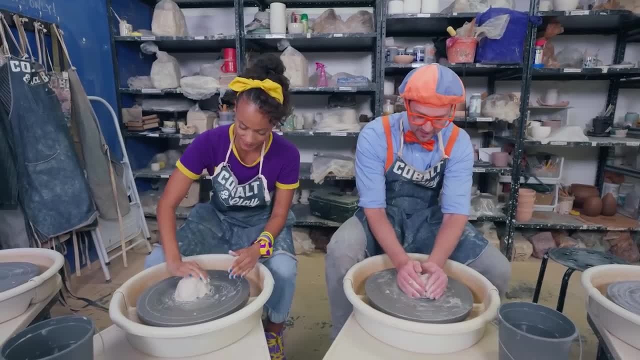 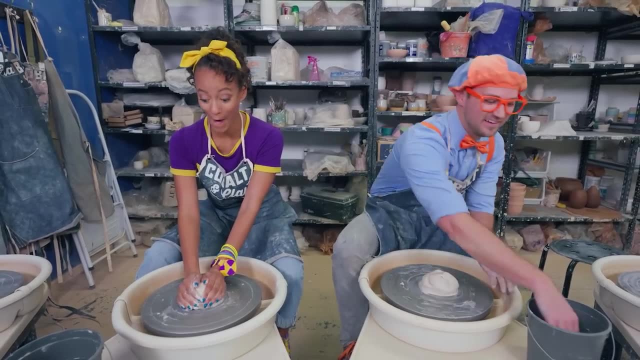 That sounds right to me. Yeah, Yeah, Okay, Okay, Whoa Whoa, That's fun Really. Yeah, Can't wait to try Whoa Whoa, Okay, Oh, it actually goes pretty fast, huh. 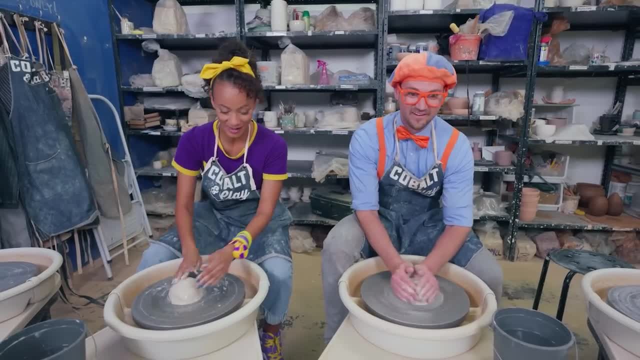 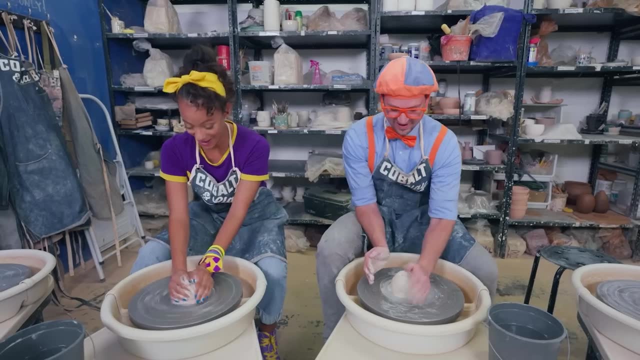 Does it? Whoa, Yeah, Whoa. My clay's going for a ride. Yeah, Mine's a little off center, so I'm going to push it in the center. Yeah, like that. Oh, that's a good idea. 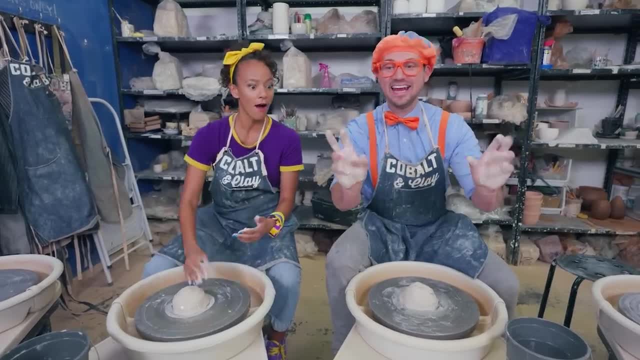 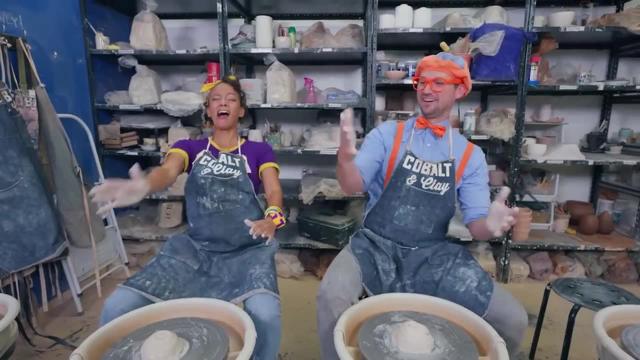 Yeah, maybe it'll work. I don't know Whoa. Look at my hands. Oh, mine too. Whoa, Sticky and slimy. How about a clay? high five, High five. Oh, it's on my face. 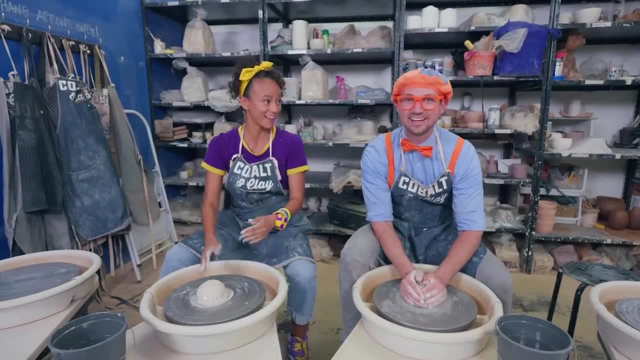 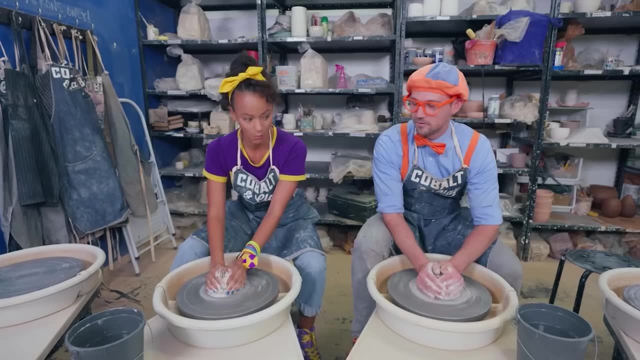 Isn't that silly Trying doing clay can be pretty dirty, I know, but it's really fun. Jeez, Okay, here we go. Whoa, Whoa, Whoa, Whoa. Okay, Don't let go of your clay. 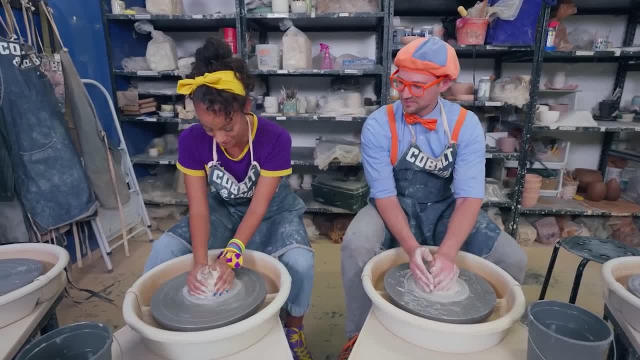 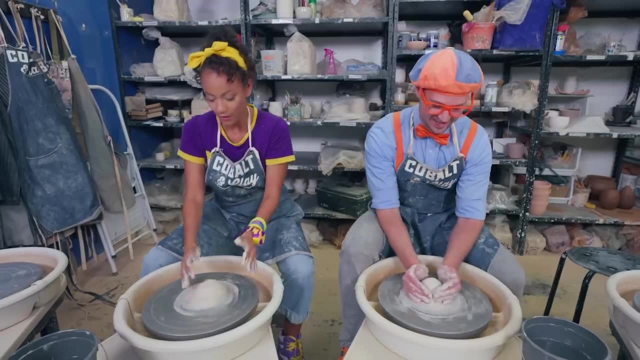 Okay, You're so silly, Mika. Oh, How are you doing? I don't know. Whoa, I don't know, I can't stop. It's pretty wobbly, Whoa. Okay, Here we go. 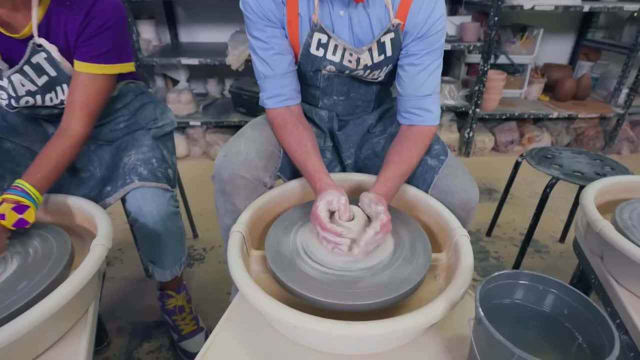 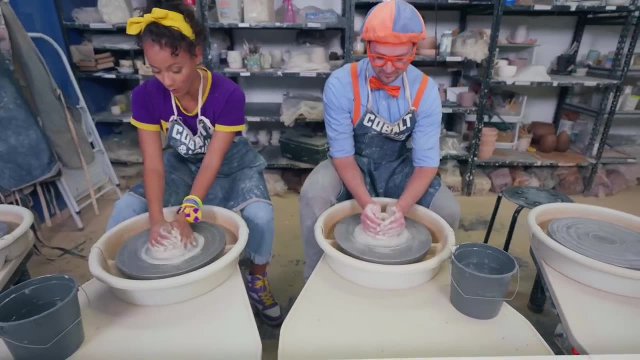 Here we go. Whoa, Look at that blibbly Yeah Making a cereal bowl. Oh, cool, Whoa. All right, Here we go. Whoa, Whoa, Whoa, Whoa. I think mine's going to be a little wobbly. 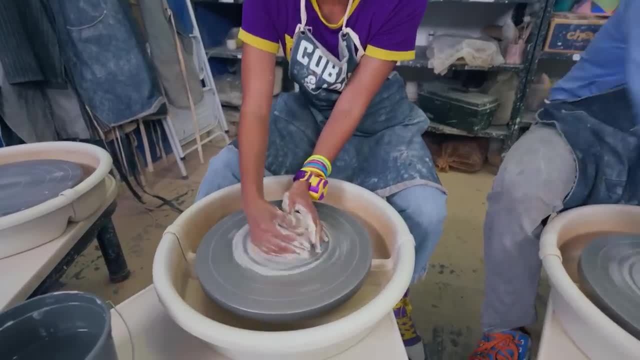 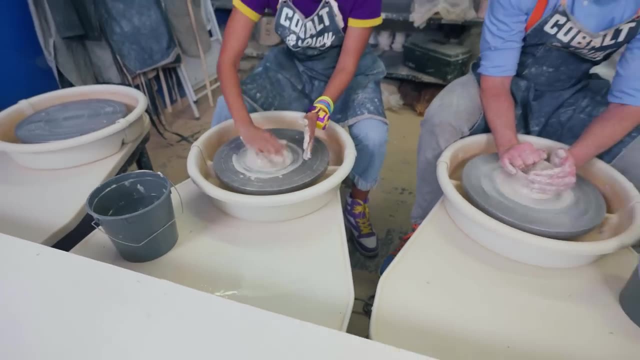 Whoa, Oh, Should we take a look? Yeah, Let's check it out. Oh, Okay, I'm going to keep going with that shape. Let's see, Whoa, Look at what I made. Whoa, Oh, that looks amazing. 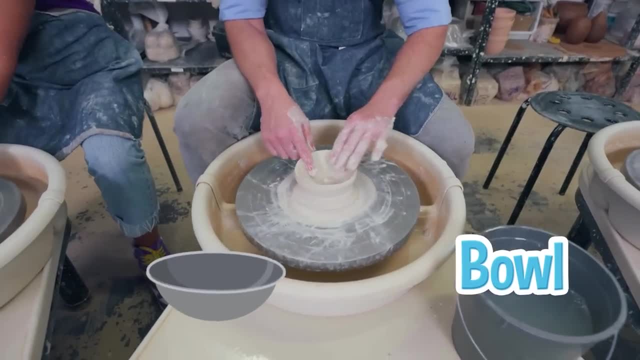 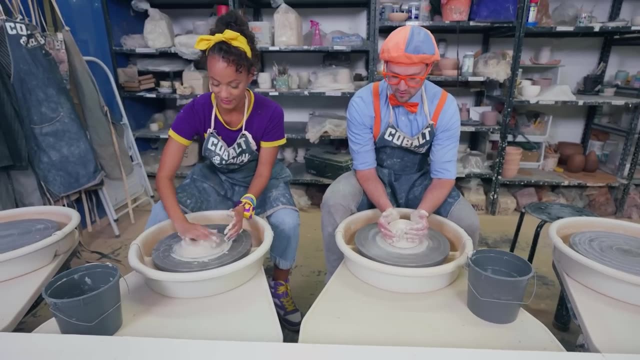 Yeah, Like a bowl. You can put all sorts of knickknacks in here, Yeah, Or you can put little snacks in there, Oh yeah, Smart Ooh, And it's so cool Because when you want to go higher, you just pull it up. 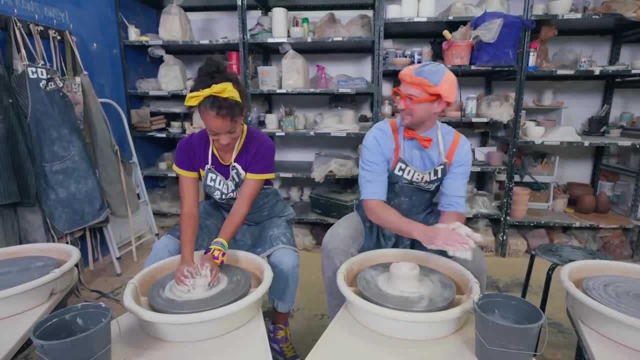 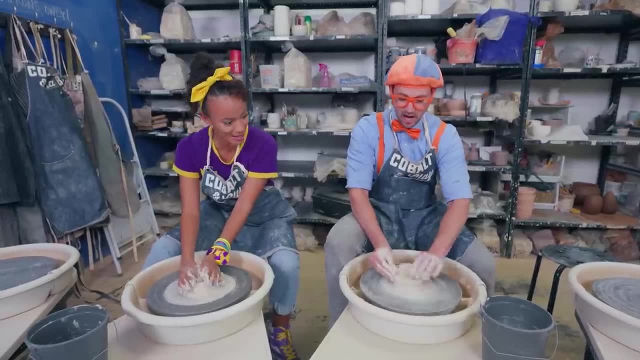 You don't even have to spin your hand around, Blippi, you're such a natural. Thanks, Mika Ready. Here we go. Whoa Oh, my goodness, Blippi too fast. Whoa Oh, Oh. 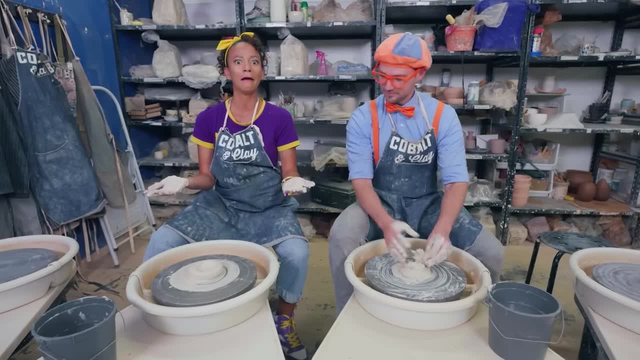 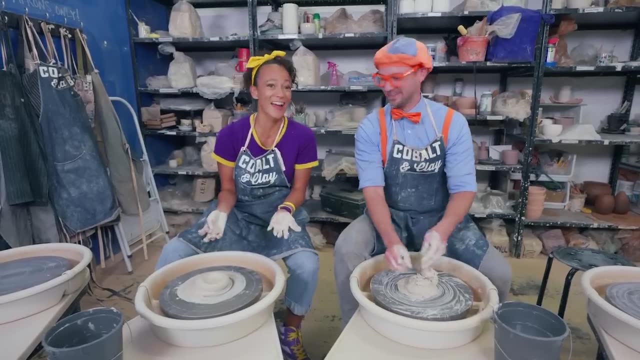 Oh, It's actually harder than it looks. huh, Yeah, I ain't broke. Oh, yours looks pretty cute though. Oh well, thank you. Oh Well, shall we go to the next station? Yeah, let's try it out. 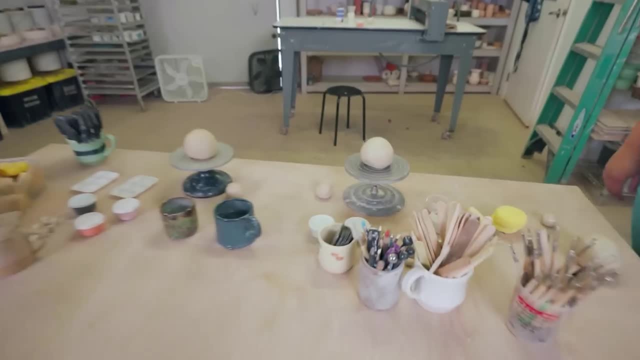 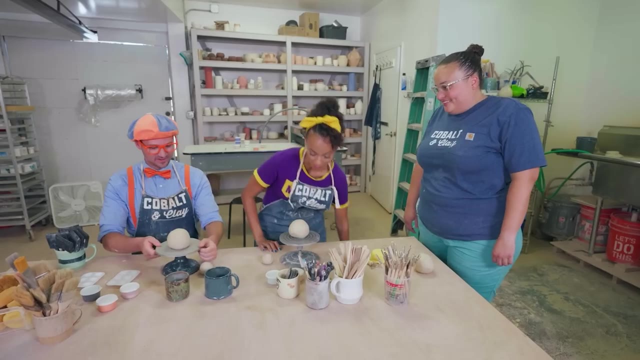 Oh, this is fun. All right, come on. Okay, Yep, Washed hands. I think we're ready. Yeah, I'm so excited. Yeah, All right. And what's this station called Hand building? Hand building. 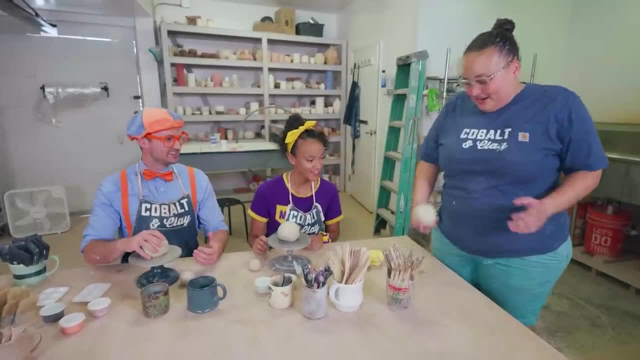 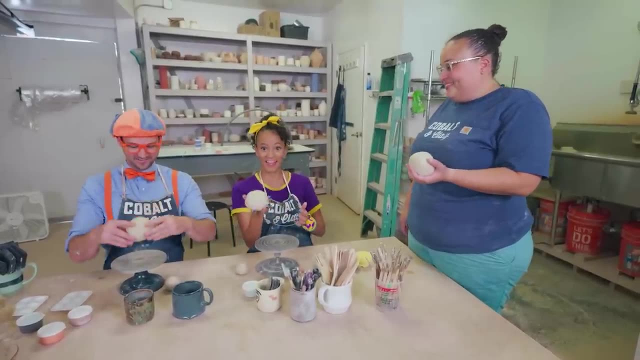 Whoa, So do we build with our hands? Yeah, we're going to sculpt our animals right now. Oh, Okay, Is this the body or the head? This is going to be our animal body. Oh, Okay, Fun. Oh, and look at this. 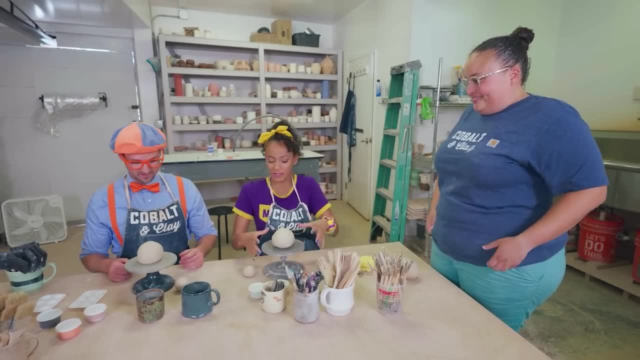 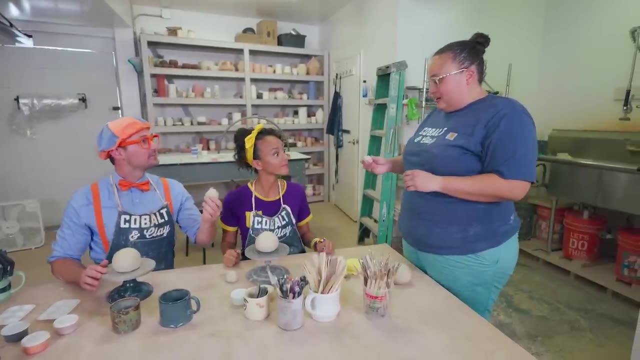 Wee, Wow, It's kind of like the wheel we were at before, but smaller. Yeah, Whoa, Wow, Sorry, It's okay. And what's this one for? We're going to use these to make our attachments to like. 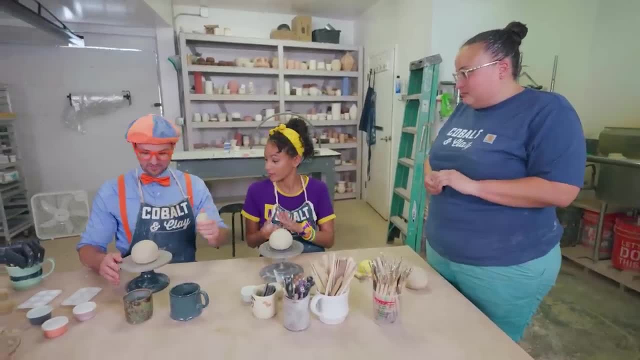 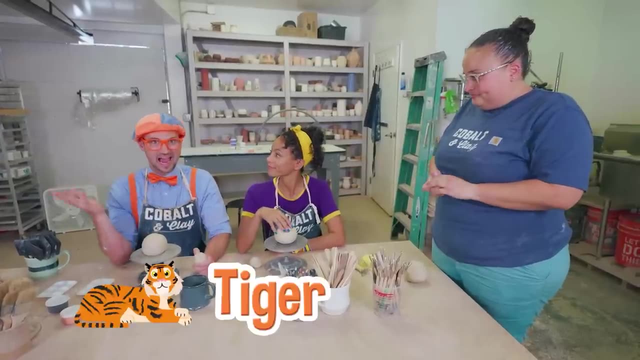 the animal's limbs and maybe like some fins or some. whatever you're trying to create. Oh cool, Well, huh, what kind of animal do I want to make? Um, maybe a tiger? Ooh, that's a good one. 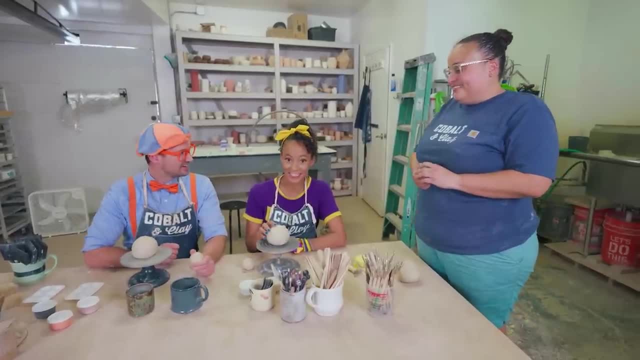 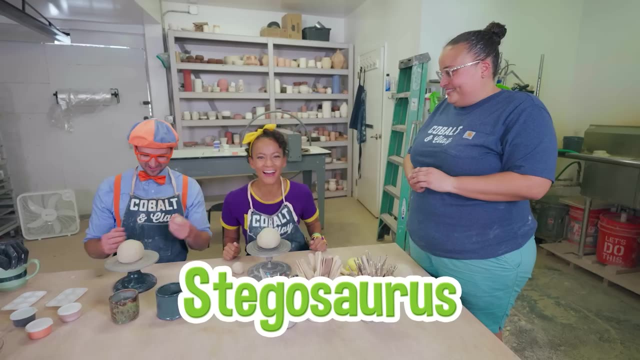 Yeah, What about you? I think I might do a dinosaur- Oh fun, You know, with plates down the back. Ooh, like a stegosaurus. Yeah, Cool, All right. So how do we get started? 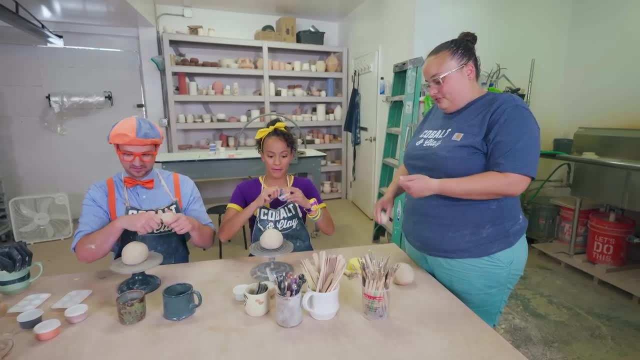 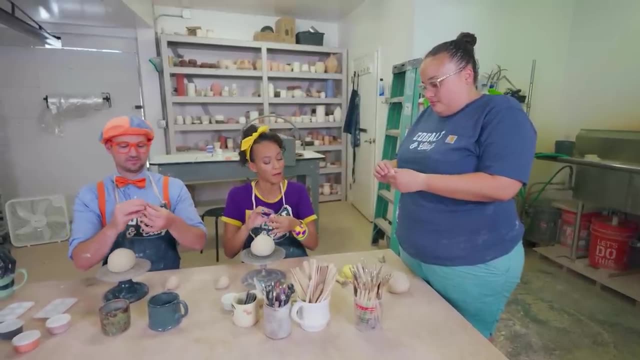 Just pull it off. Yeah, so you're going to just pinch a little piece of clay off, OK, And then you're going to roll it. Use your fingertips to mold the shape that you'd like. So, if you're trying to make um, if you're trying to make a limb, 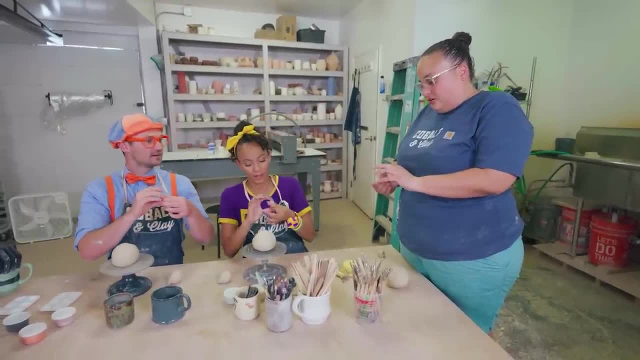 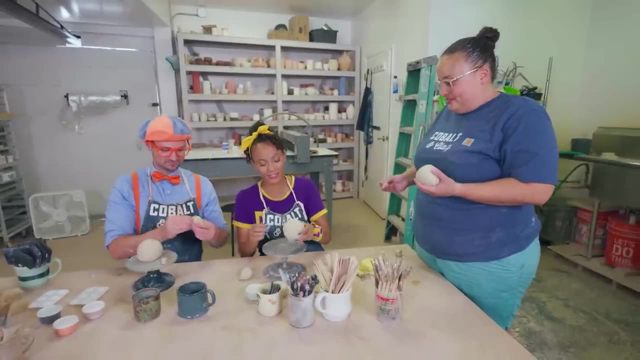 then you know you just want a little foot or a paw of some sort, right? Oh yeah, look at this. A really short leg like this, Yeah, Boop, Nice. And how do you get it to stick? 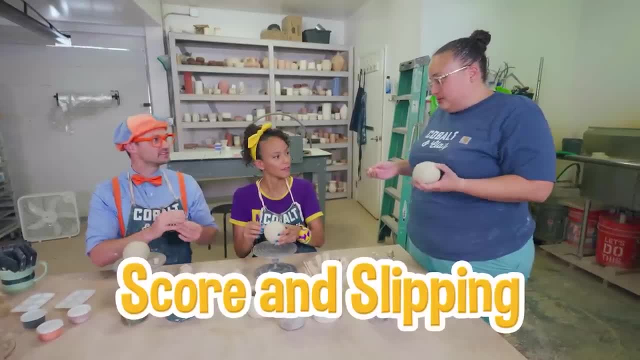 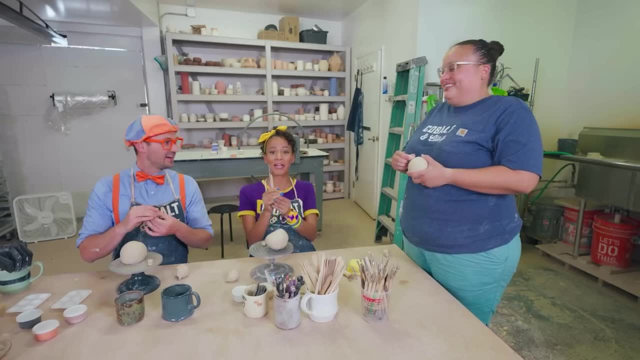 So when you make clay attachments, it's called score and slipping. So what we need first is needle tools. Needle tools- Oh, Nicole, I have them right there. Oh, Here you go. You can just have these needle tools in your jam pack. 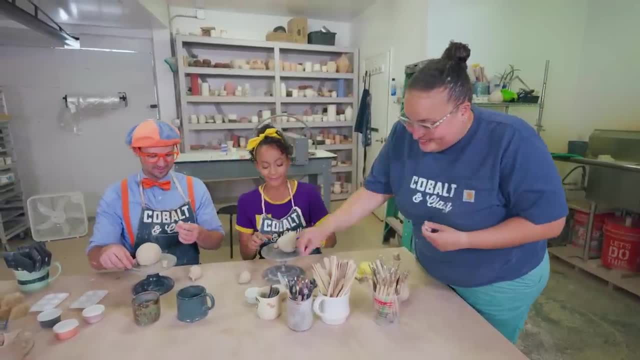 I have everything in my jam pack. Oh cool, Mm-hmm. OK. So how do you do it? So you're going to take the needle and then we're going to make a little tic-tac-toe mark on one of the bottoms of our piece. 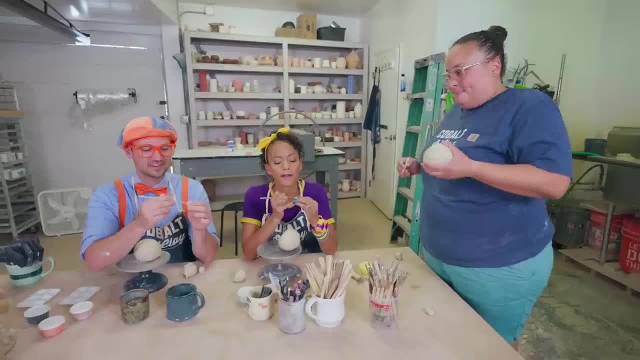 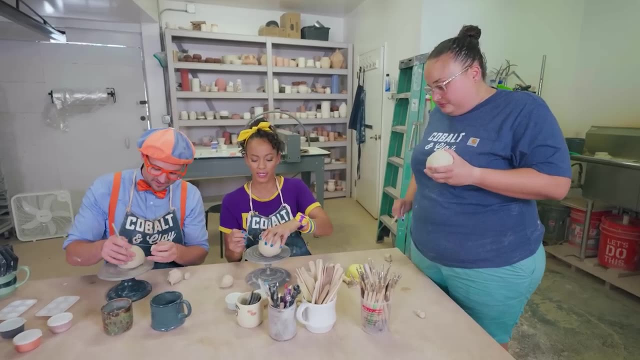 OK, Tic-tac-toe, Tic-tac-toe. What a fun game. Yeah, there we go. And then you're going to do it to the body as well, where you're going to connect it. OK, Oh, where should I connect it? 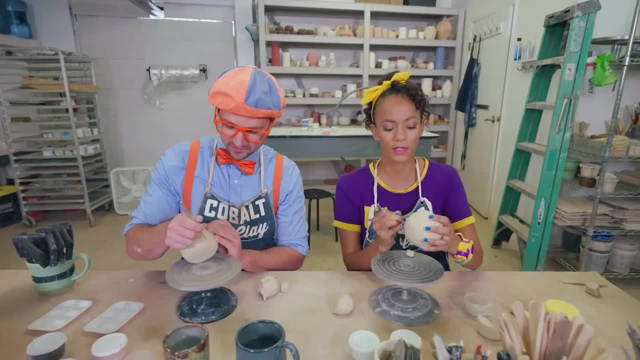 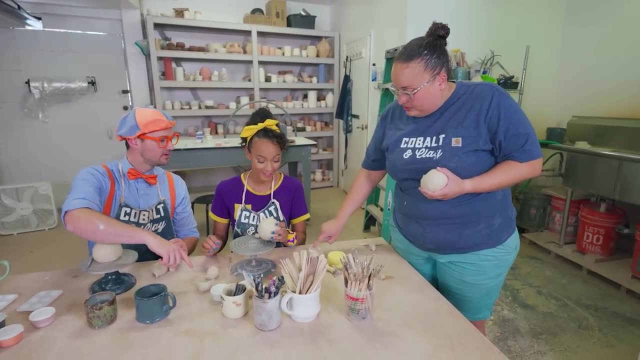 OK, how about, right here, One, two, three, four. OK, There we go, All right, And then in these cups, these are called slips. So what you're going to do is you'll dip your finger in the slip. 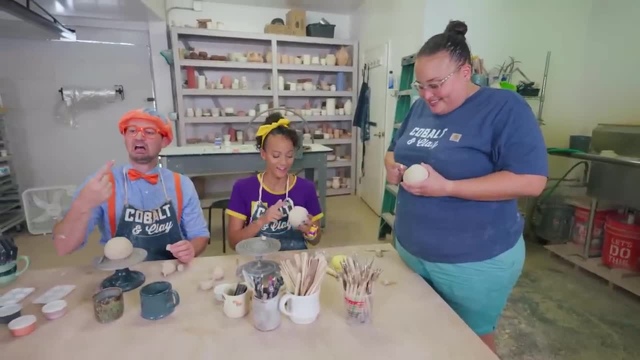 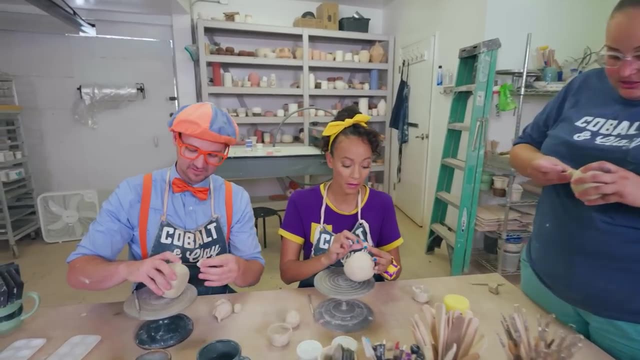 Oh, like glue, It's glue, It's clay glue. basically, You're going to dot the tic-tac-toe, You'll put them together and then you'll firmly push it so it could stick to one another. OK, 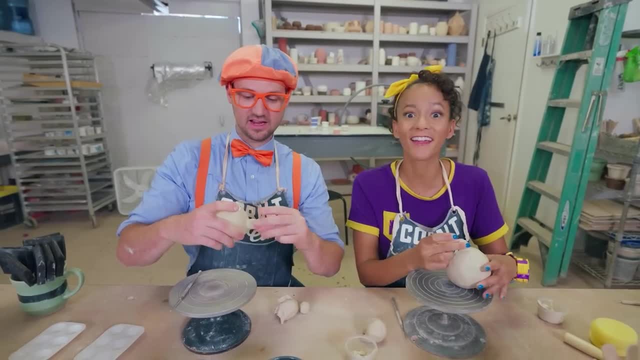 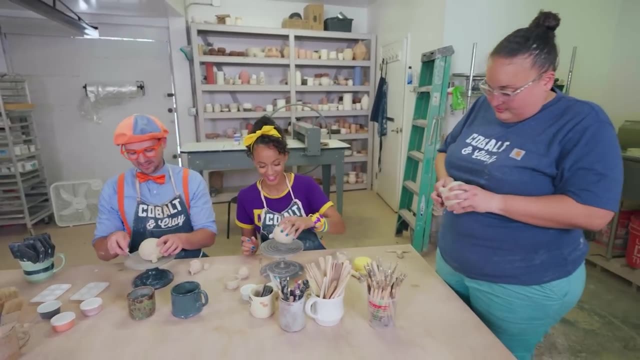 There we go, Push it together. Oh yeah, it's sticking. Oh yeah, it did Check it out. Oh cool, Look at mine. Good job, One leg done. There we go. That looks so good, Blippi. 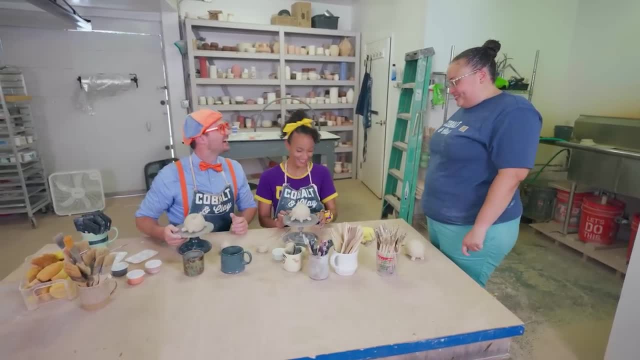 Oh, yours too. Oh, thank you. Wow, guys, your animals look great. Thank you, Thank you, Thank you. What do we do next? So now we're going to paint them, bring them to life. Oh cool. 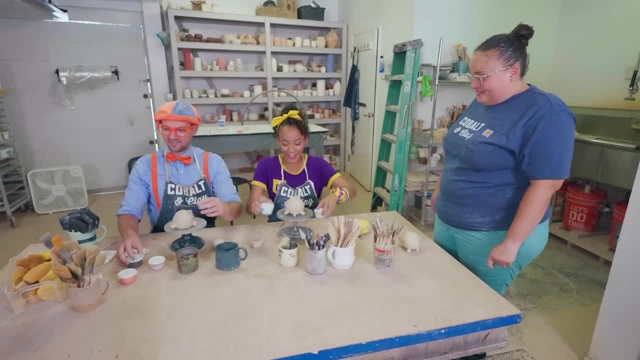 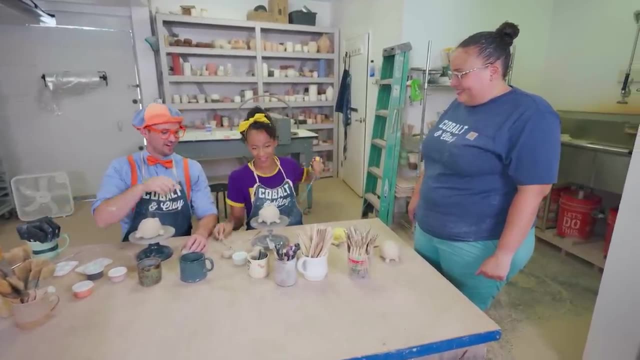 Paint them Cool. It looks like we have some paint right here. Oh yeah, Oh, but these brushes look way too big, Mm-hmm. Oh, don't worry, I have paint brushes right here in my jam pack. 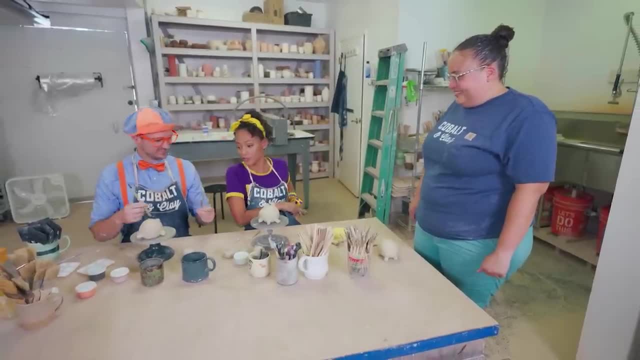 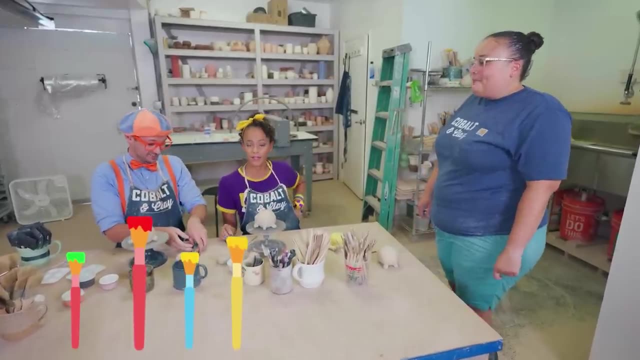 Oh, you have everything in there. I really do. I have some more too. if you want other options, I have a little one, I have a bigger one, I have another little one. I also have a medium-sized one. 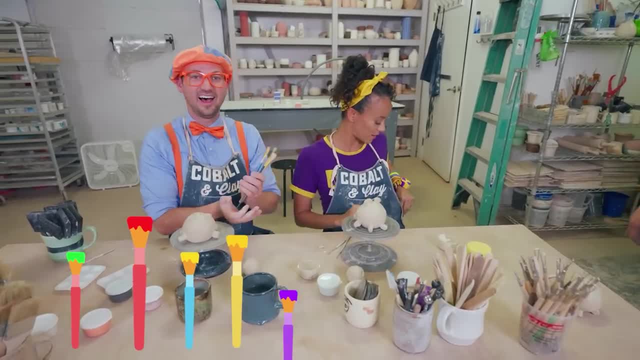 And I also have another one that's oops, sorry, that's not it. And I have a tiny one and I have another tiny one. Whoa, OK, I'll use this one and this one. OK, sounds good. 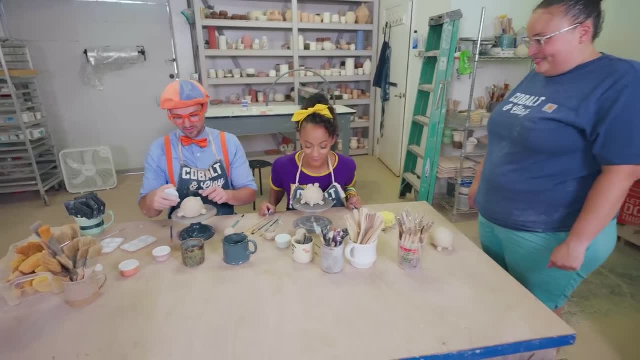 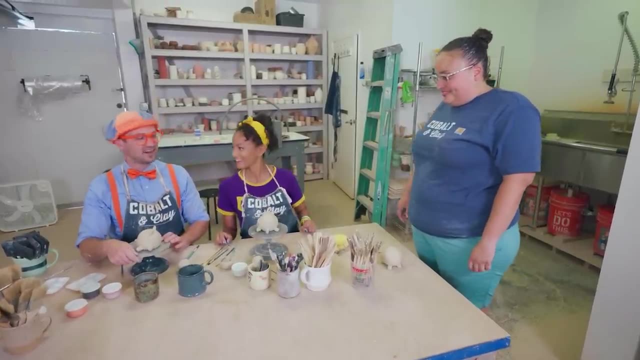 Oh, and then we just use these paints and put them on the animals. Yes, whatever color you want it, whatever designs you want, you're going to dip it in and then you'll just paint it onto your animal. Awesome, Thank you. 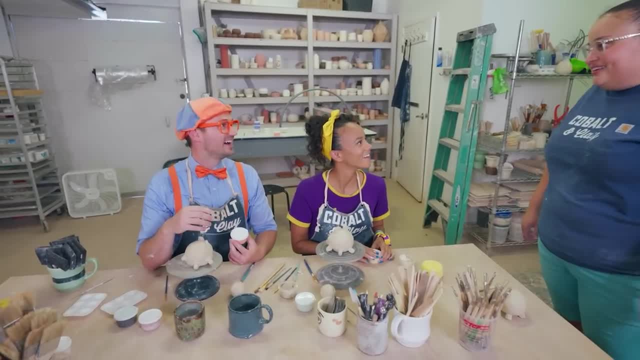 Let's do it. Yeah, since you guys have what you need, I'm going to go check on the kiln and I'll come back and I'll have a check on you. OK, thank you, All right, thanks, See you. 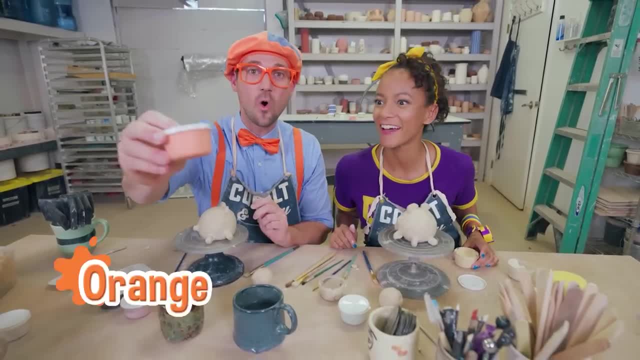 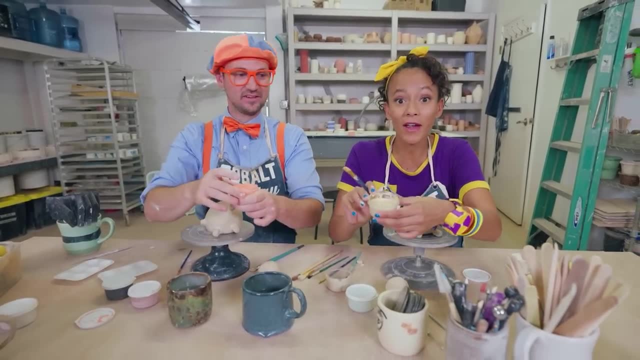 Whoa, cool. OK, since I'm doing a tiger, I'm going to use orange- Oh, cool, Good idea. Whoa, And I'm going to use yellow for my dinosaur. It doesn't look like yellow right now. 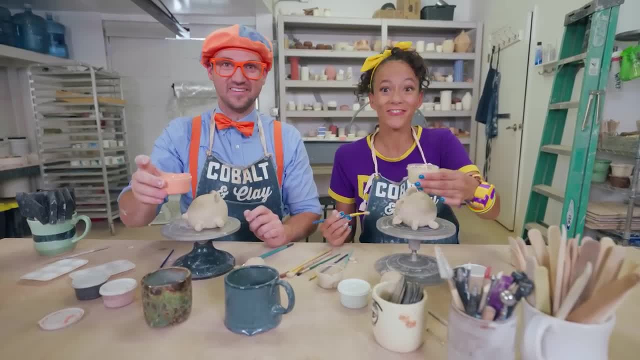 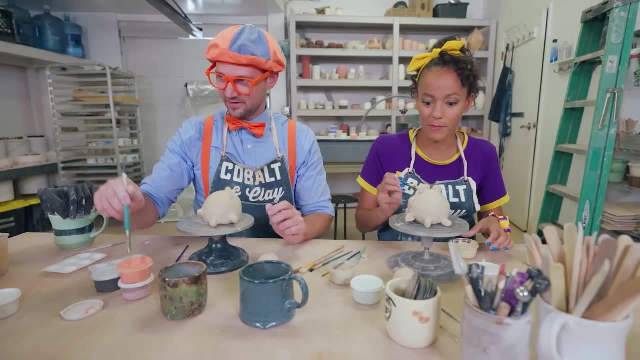 but once it's baked it's going to turn to a nice bright yellow. Oh cool, Check this out. Ooh, Ooh, There we go. OK, Hey, I've never painted clay before Me, neither. Whoa, it's really fun. 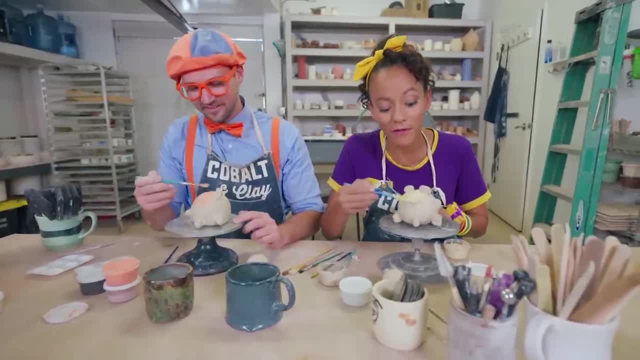 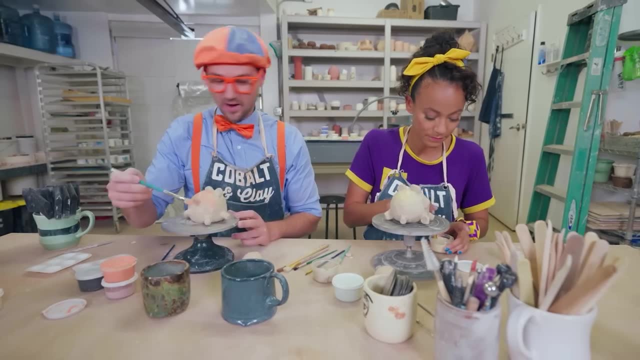 Oh see, Whoa, Right now it looks like the same color as the clay. I can't wait to see it when it's yellow. Yeah, my orange isn't that bright, Right, but I bet after it gets fired in the kiln. 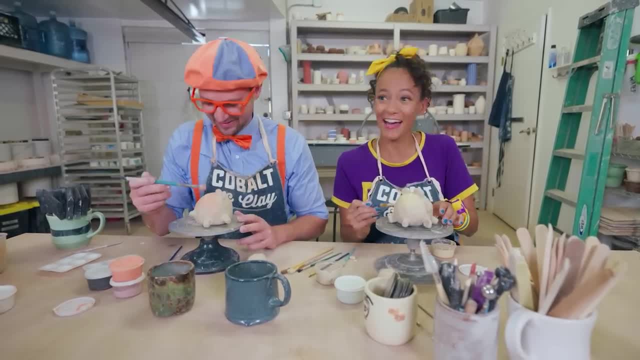 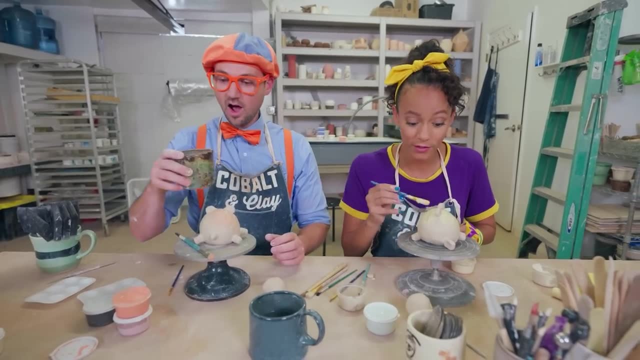 then from there I bet it'll turn really bright orange. Oh yeah, Oh look water, Pretty thirsty. No, no, Blippi, What That's for your paintbrush. Oh smart Yeah, you dip your paintbrush in this water. 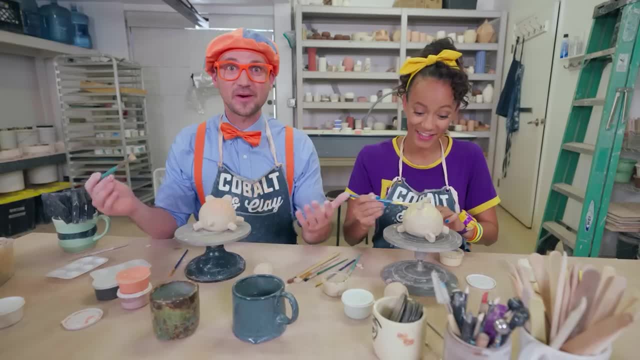 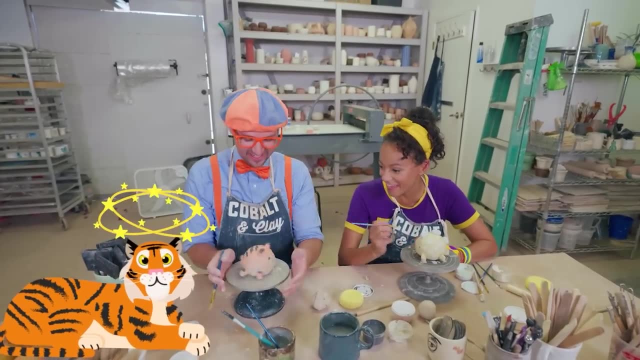 You don't drink it, And so then you can use a different color without mixing them. There you go. Thank you, I got you. I'll get some water later. Whoa, dizzy tiger. Yeah, Whoa, this thing's so cool. 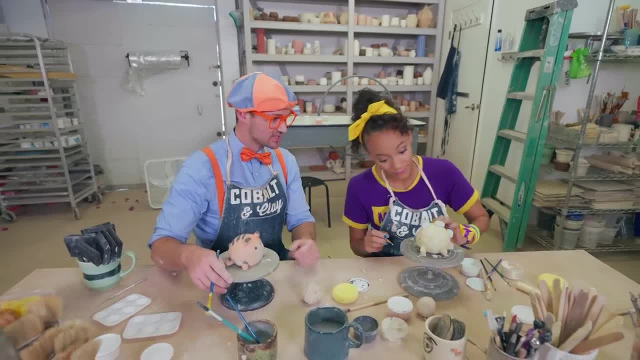 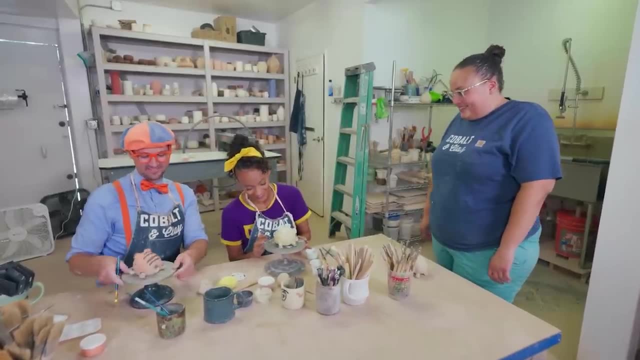 Yeah, hey, your tiger looks really good. Wow, yours too. It's so colorful, Thank you, Oh, hey, Hey, wow guys, Your pieces look great. Yeah, you like them, They're amazing. Oh, why aren't they so bright and colorful? 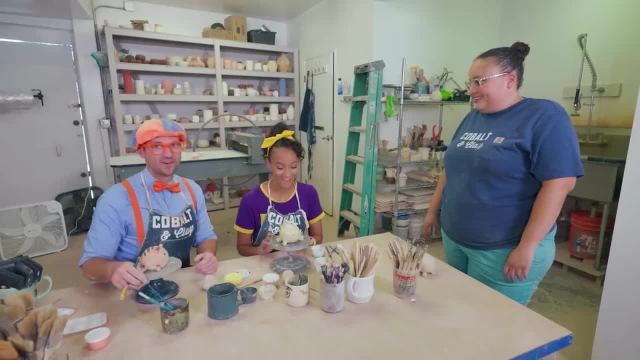 So once we take them and put them in the kiln, the colors are going to get a lot brighter. Oh cool, Can't wait to see them. Yeah, so is my orange going to get, like my suspenders and bow tie. 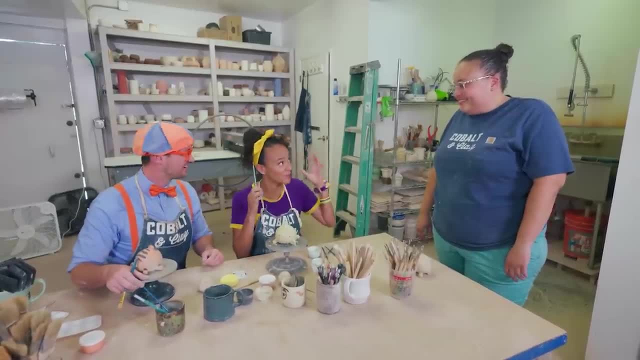 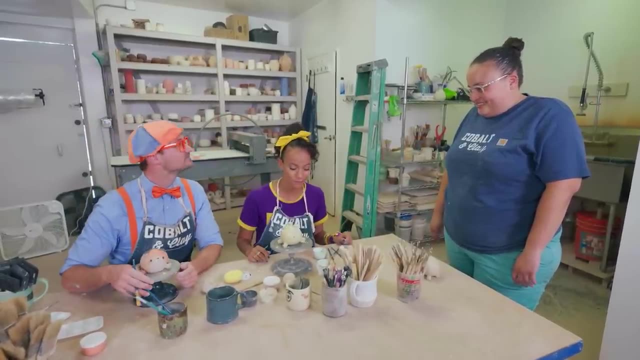 Exactly Whoa, and will mine get as bright of the yellow as my headband? Yes, Oh, that's fun. Whoa, Oh cool. Well, what do we do next? Well, what I'm going to do is I'm going to take your guys' animals. 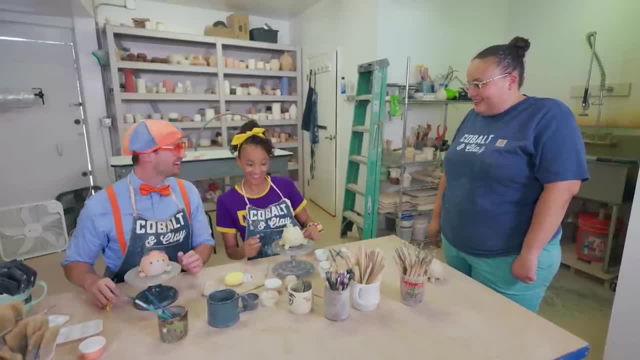 and then I'll put them in the kiln And then you can come get them when they're ready. Oh fun, Sounds like a good plan. OK, here you go. See you later, tiger. OK, be gentle with it. 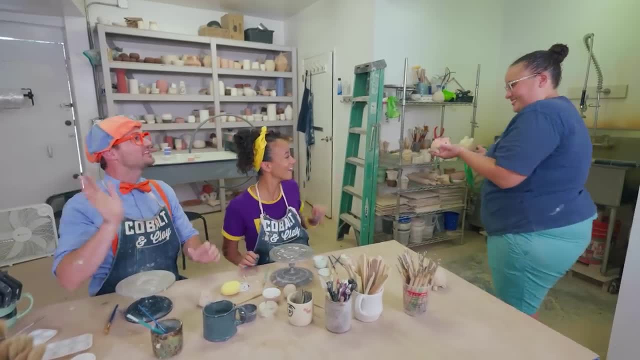 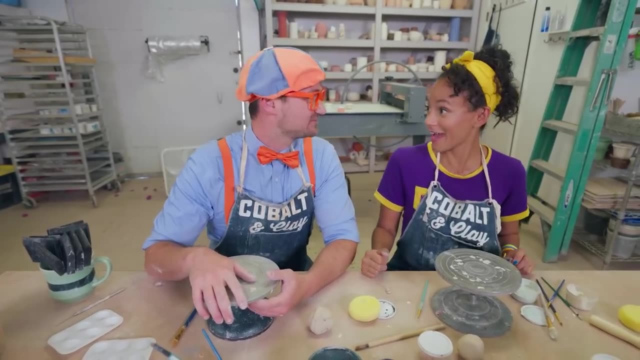 Here you go, Thank you, Bye. Well, thank you so much, See you. Wow, that was so nice for teaching us about pottery. Yeah, that was really nice. We learned a lot. Yeah, I can't wait to see what they look like. 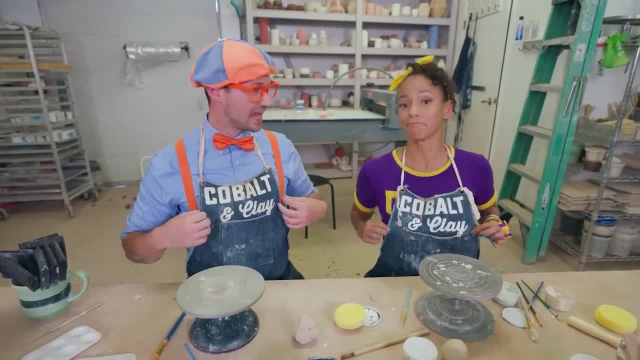 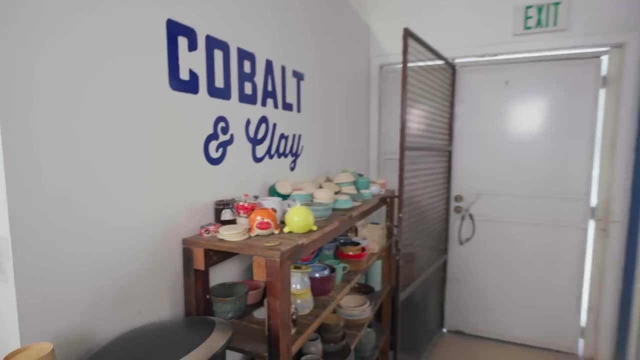 I know That was really fun. Yeah Well, shall we return the aprons? Yeah, let's do it, And then we can come back to pick up our things. Great idea, All right, Woo-hoo, Whoa, lookie, look. 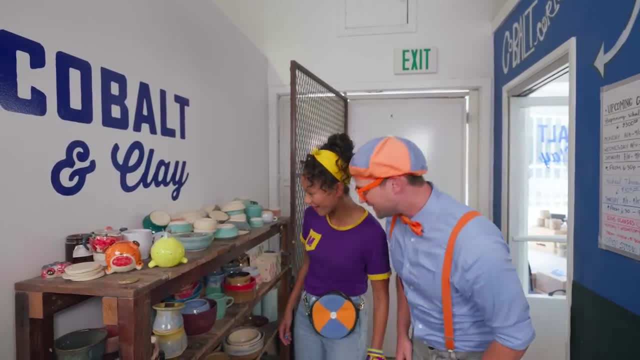 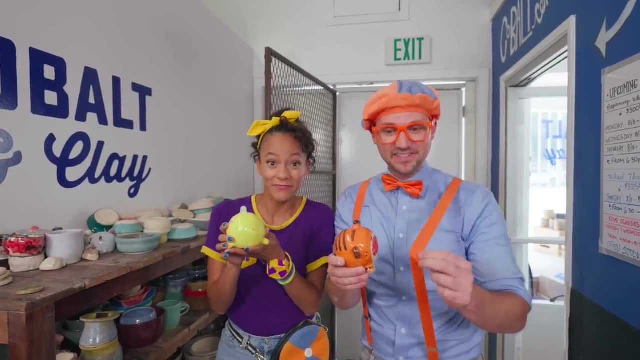 Cool. This must be where everyone picks up their pottery. Yeah, Oh ours, Yeah, Cool. What do you think? Oh, she's right, It did turn bright orange. Yeah, it really did, And mine turned bright yellow. 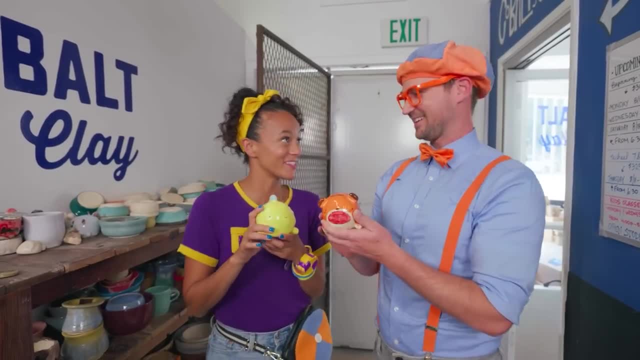 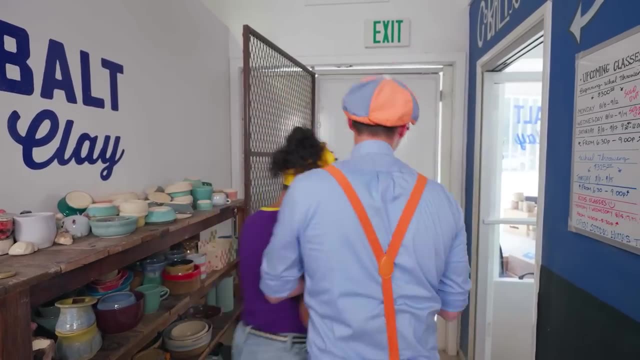 Oh, yours looks so great. Thank you, I really like yours too. Oh, thanks, Hey, shouldn't we go? Yeah, put it by the pig. Yeah, let's go. Come on, Oh, Uh-oh. 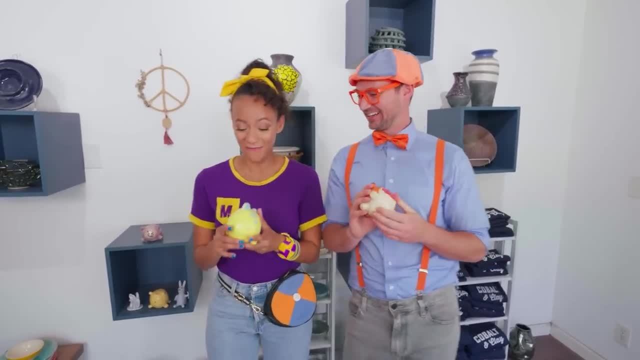 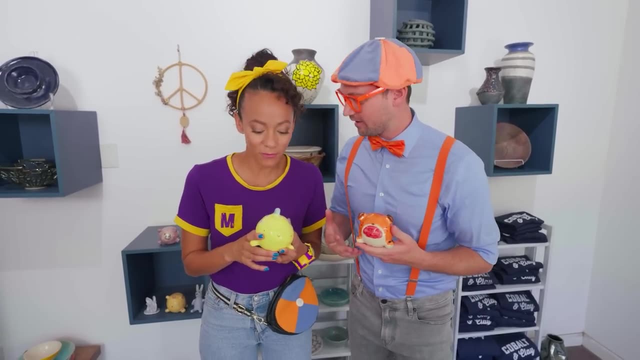 That was so much fun today. Yeah, that was a great time making these new friends. Yeah, Whoa, Hey, did you notice they both roar. That's right, because mine's a dinosaur And mine is a tiger. That's cool. 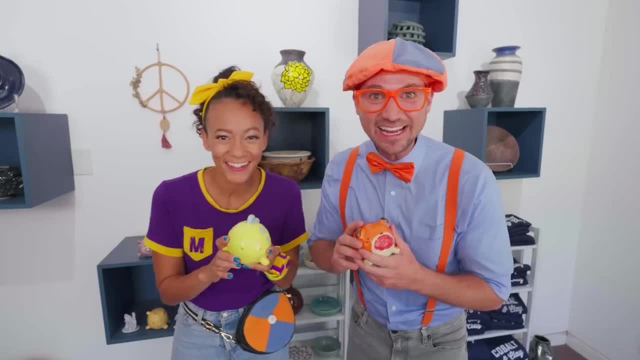 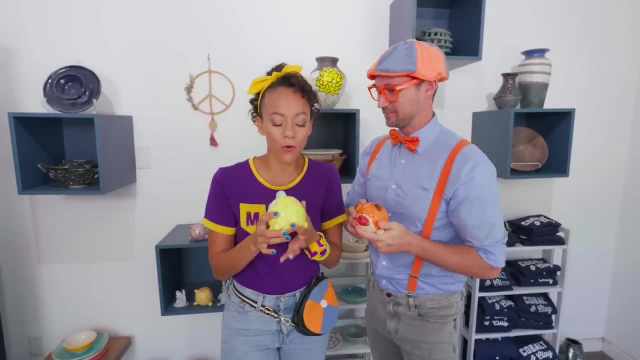 Should we roar together? Yeah, will you roar with us? Ready, Roar, Roar. Oh, that was awesome. Yeah, it was so cool molding that clay and creating these- Yeah, And then using the paintbrushes and coloring them. 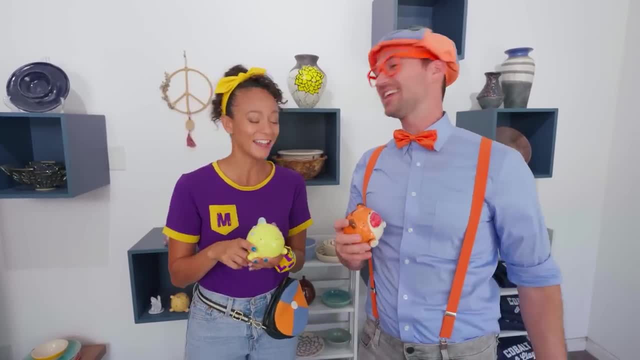 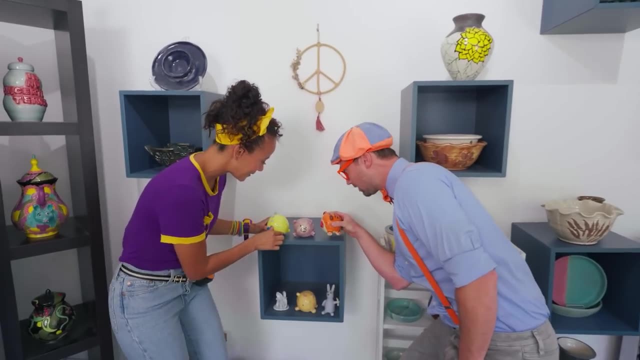 Yeah, Oh, Making art is so fun, Yeah, especially with friends. Yeah, Oh, speaking of friends, Oh yeah, Hello, Will you be our friend? Please say yes. Please say yes. Yes, Yeah, we did it. 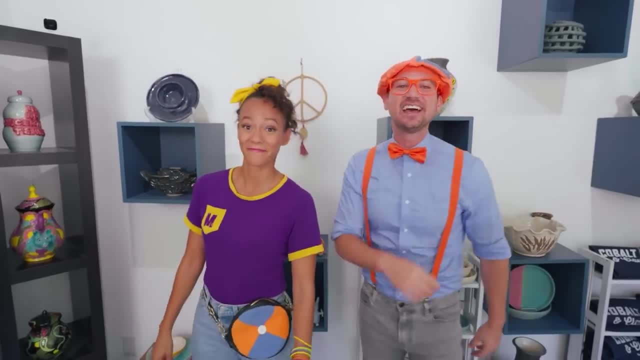 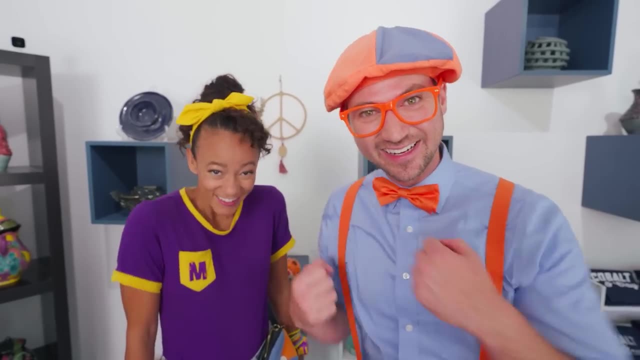 Nice job, Nice job. Well, this is the end of this video, But if you want to watch more of my videos, all you have to do is search for my name. Will you spell my name with us? Cool B-L-I-P-P-I. 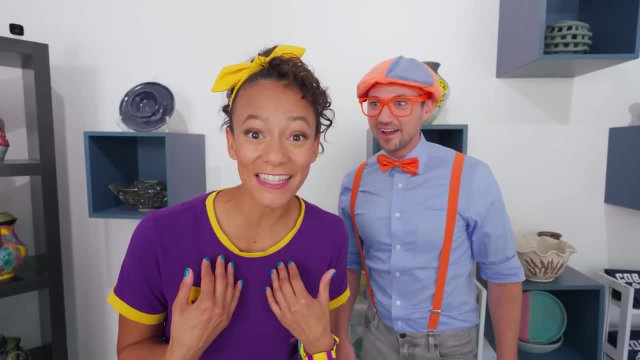 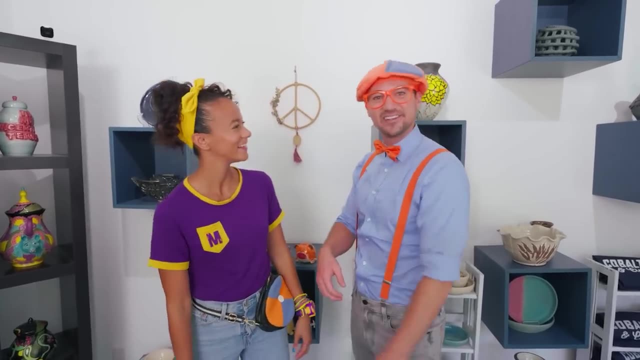 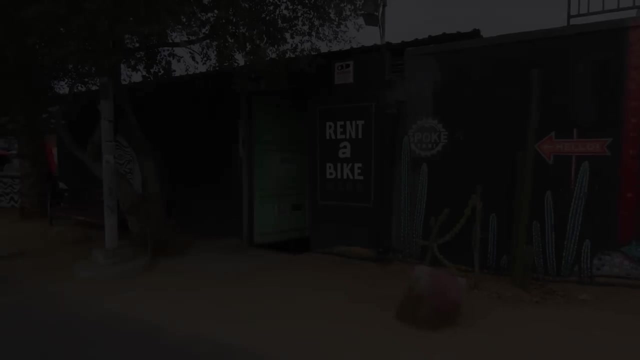 Blippi, Good job. Will you spell my name with us? Awesome, M-E-E-K-A-H. Mika. All right, see you again, Bye-bye, Bye, Bye, Wow, Whoa, Hey, it's me Blippi. 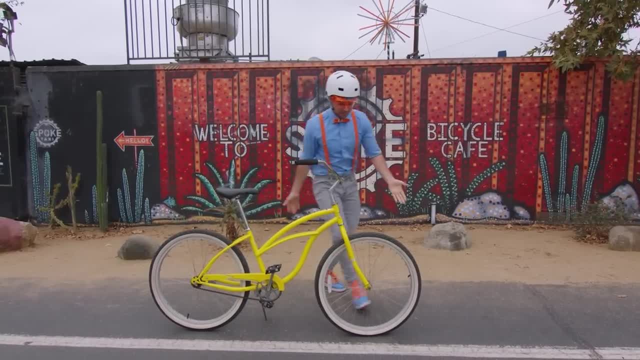 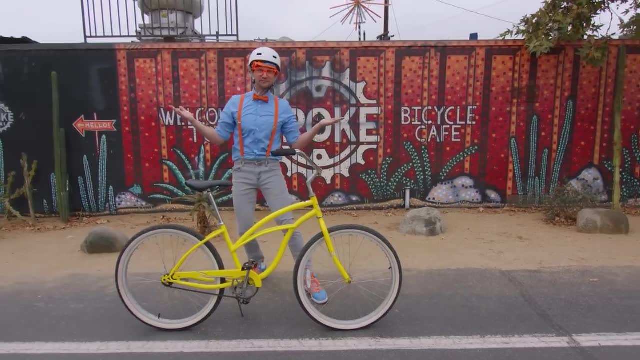 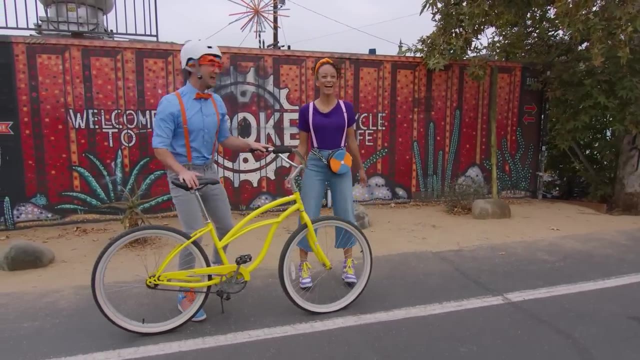 And look, I'm riding a bike, But my bike has a flat tire. Oh no, I love riding bikes, They're so much fun, But you can't ride a bike with a flat tire. Ah, Hey, Blippi. 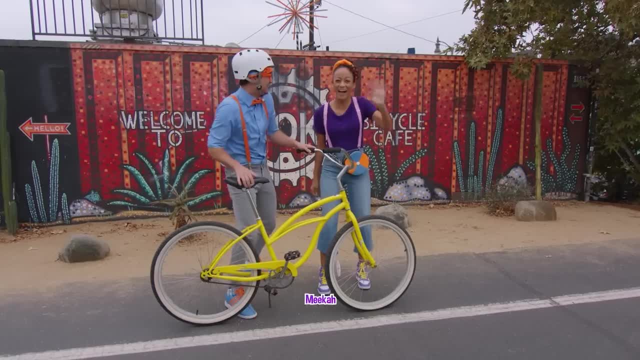 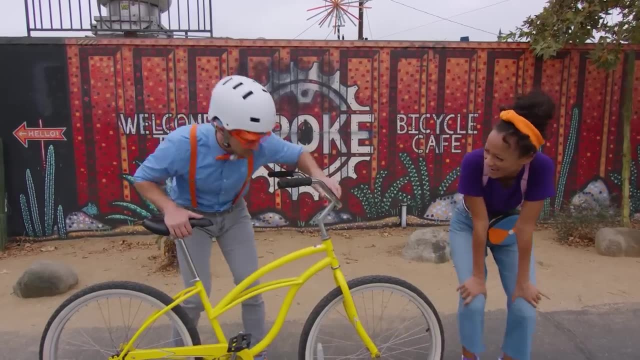 Oh hey, Mika, This is my best friend, Mika. Hi everyone, Ooh bike Blippi. Oh, thanks, Mika. Uh-oh, Looks like you have a flat tire. Yeah, I was just telling our friends. 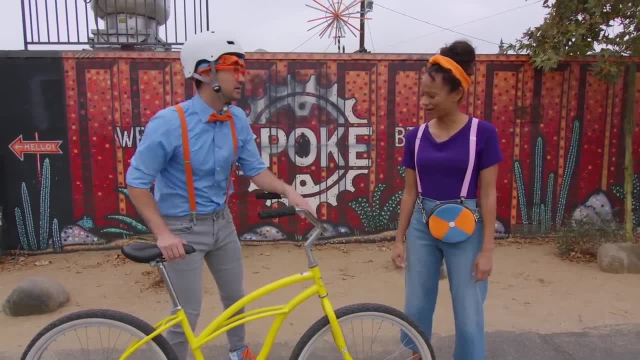 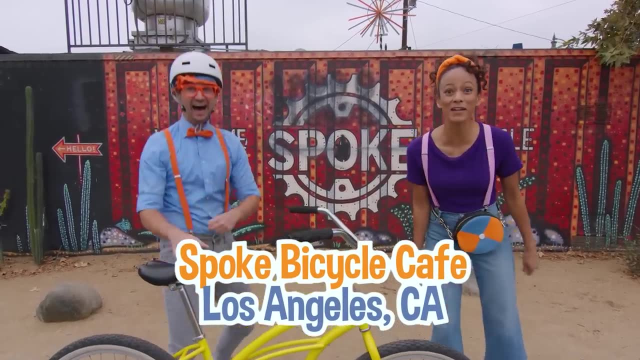 that I have a flat tire and now I can't ride anymore. Aw Well, good thing we're at Spoke Bicycle Cafe in Los Angeles, California. It's a cafe and a bike shop. I bet someone inside could help you. Whoa really. 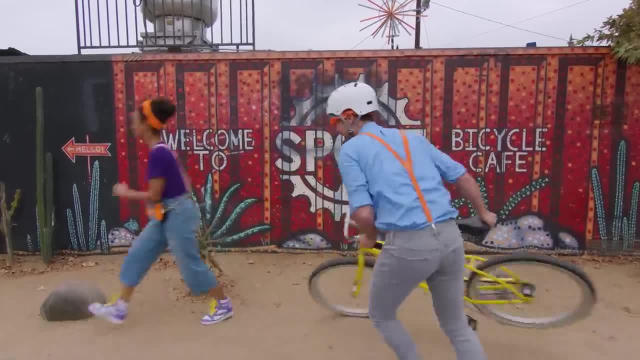 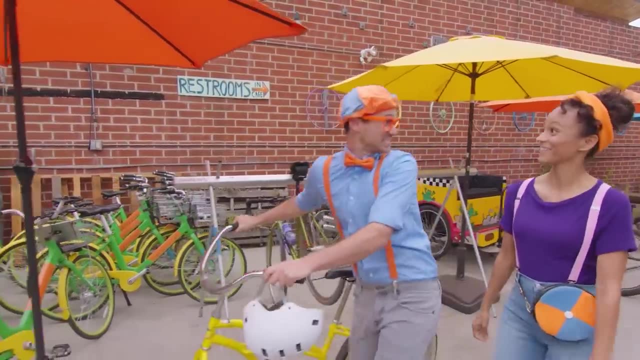 Yeah, Whoa, let's go. Yeah, let's ride out. Come on, Whoa, Whoa. So you said, this place has snacks and bikes. Yeah, it's a cafe and a bike shop. Whoa, Whoa. 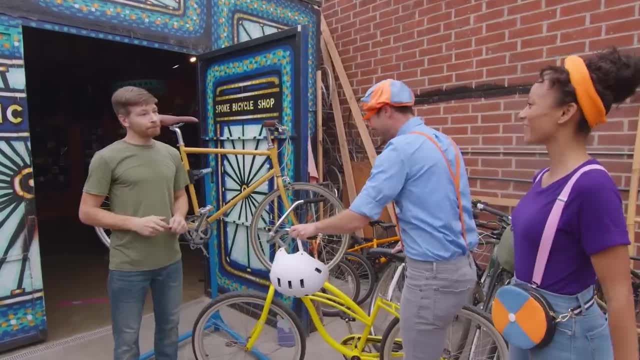 Hey, who are you? Well, hi there, My name is Dane. Oh, hi, I'm Mika, Yeah, and I'm Blippi Nice to meet you. So what do you do here? I'm the head bicycle mechanic. 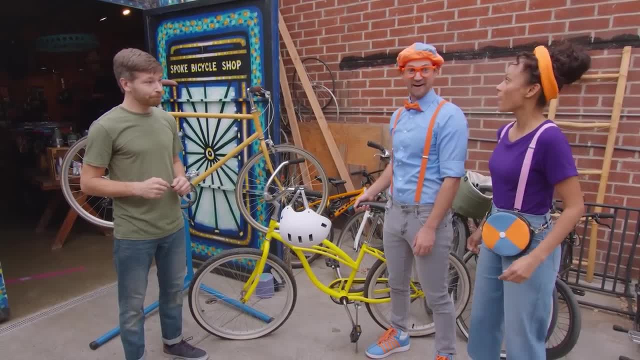 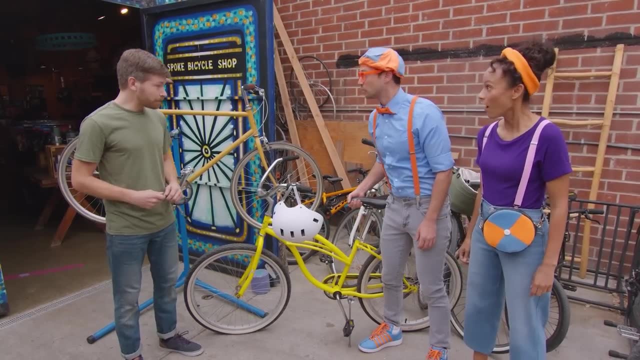 So you fix bikes? I do. Wow, You're the person we need. Blippi has a flat tire, I don't know. Well, if you follow me, we'll get you ready to roll Really. You can fix it, I can. All right, let's. 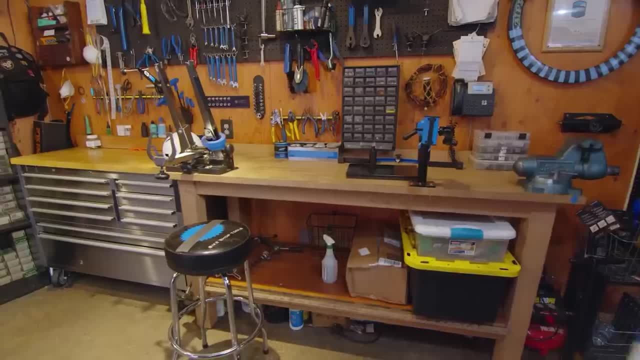 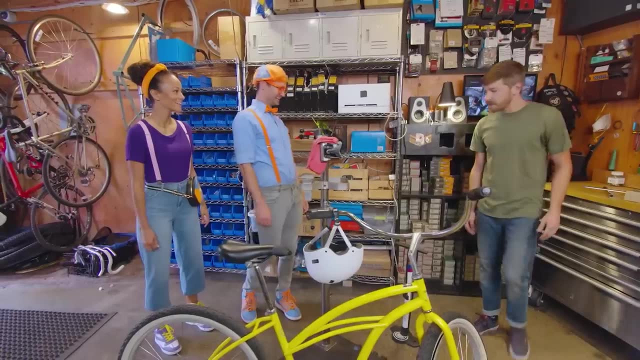 go: Come on, Whoa, This is going to be great, Whoa, cool. All right, I now have everything we will need to fix your flat tire. Yay, I'm so excited. Whoa. So the first thing. 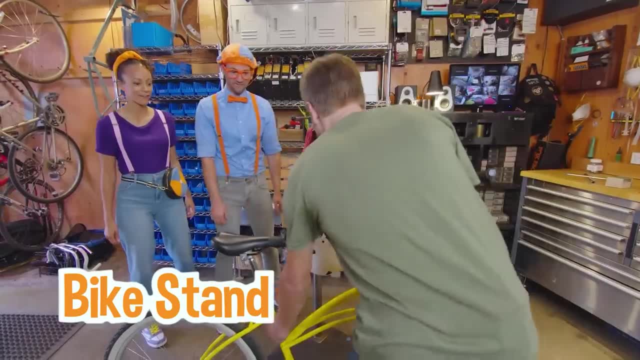 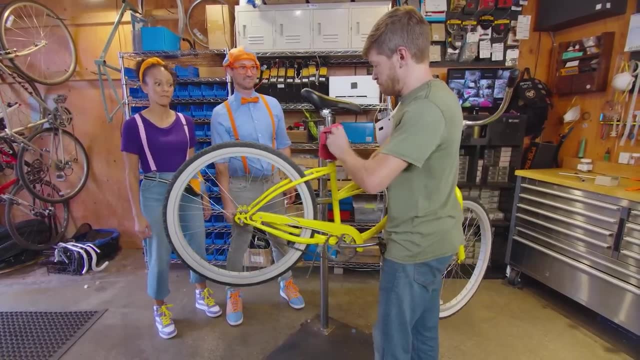 we will do is put your bike into the bike stand. Wow, cool, Oh, a bike stand. Whoa, this is what you had out there. I saw it. Oh, that's right. It must make it much easier when the bike 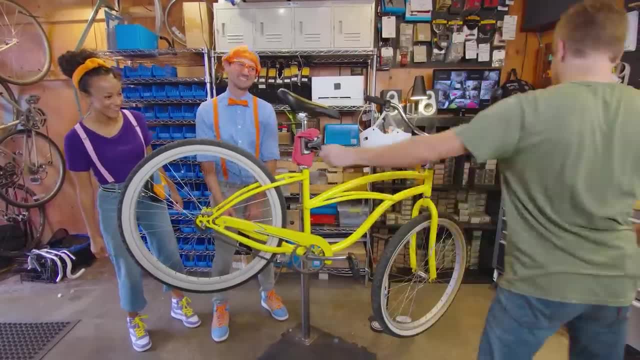 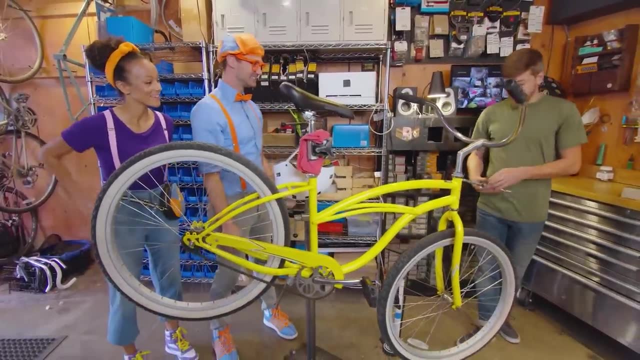 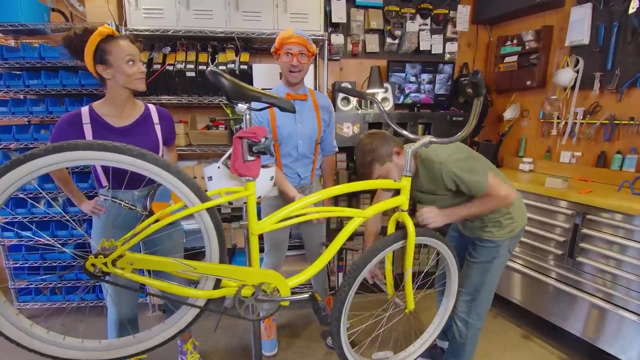 is up high like that, Much, much easier Smart. Can I put the helmet right here? You certainly can. So the first thing we're going to do is remove your front wheel. Whoa, So you're going to remove the front wheel and tire. 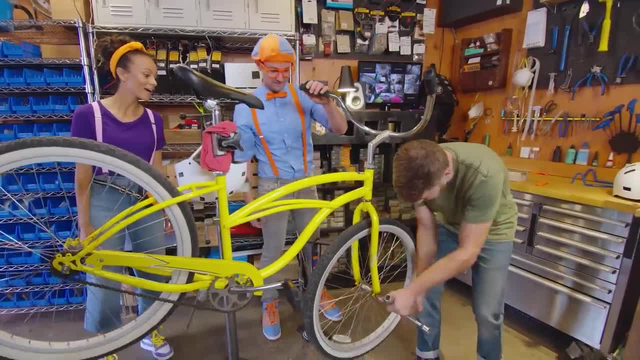 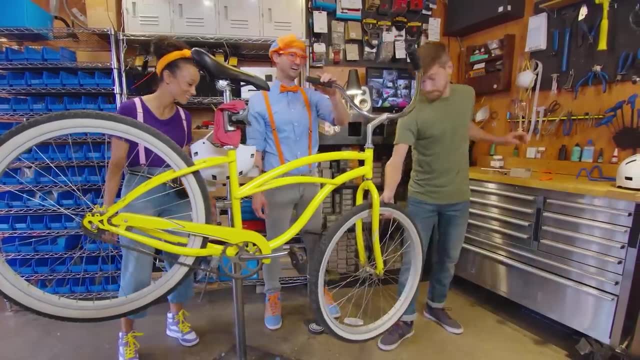 Correct. So we will take this 15 millimeter box wrench and loosen the axle nuts on the wheel. Whoa, You know a lot about bikes. Whoa, look at this. Whee, It's a bicycle. I did not want to ride a bike like that. 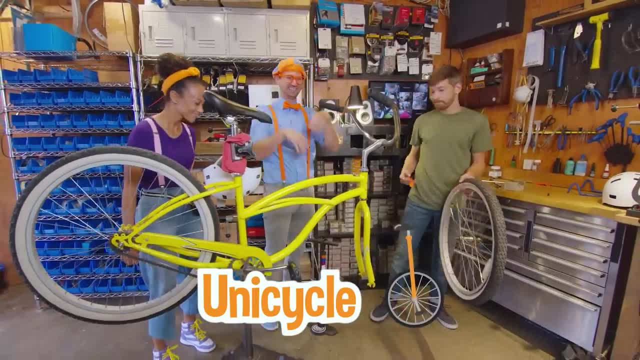 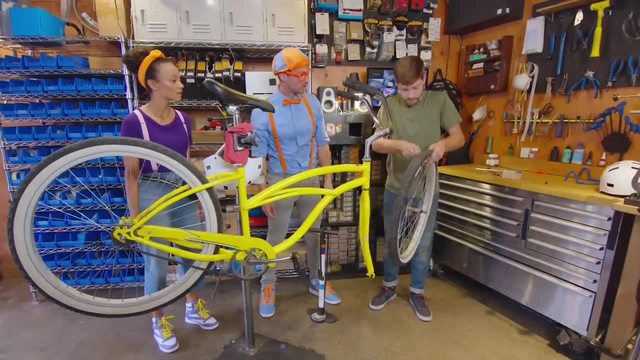 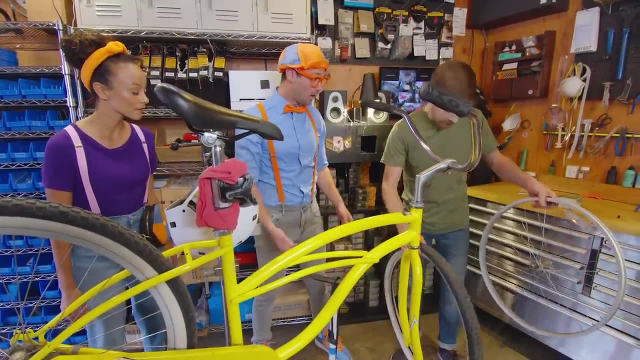 I know Now it's a unicycle. Next, we're going to take a tire lever to remove the tire from the wheel. So you're removing the tire from the wheel right now. You got it And just like that it releases the wheel. 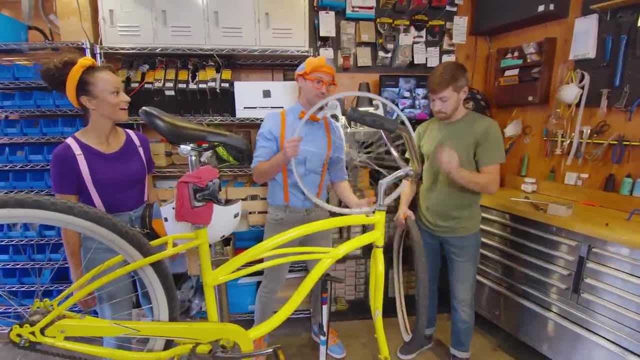 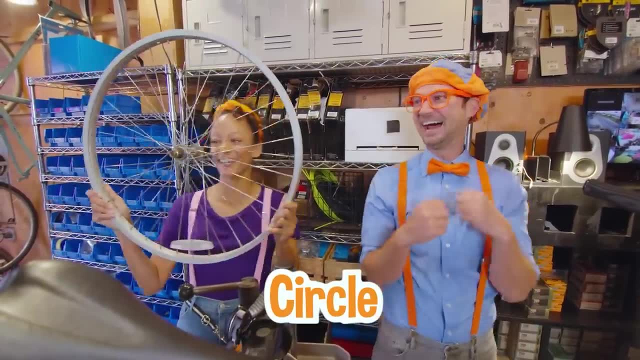 Whoa cool. Can I see the wheel? Whoa, check it out, Mika. Wow, A bike wheel with no tire. Yeah, look a big circle. Yeah Cool, Really cool, And it's actually kind of light. 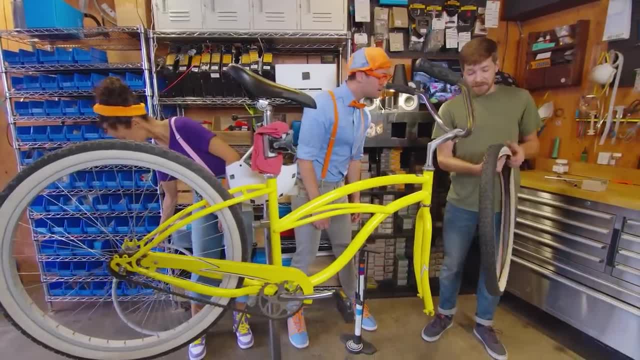 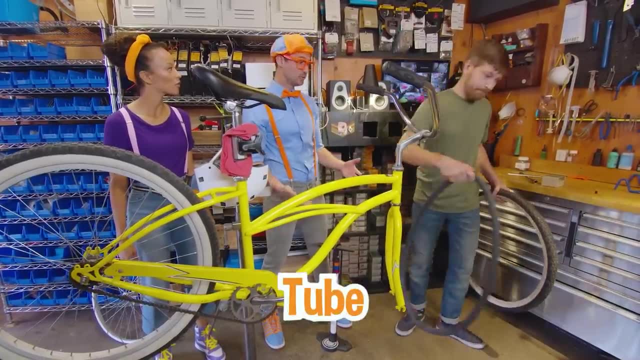 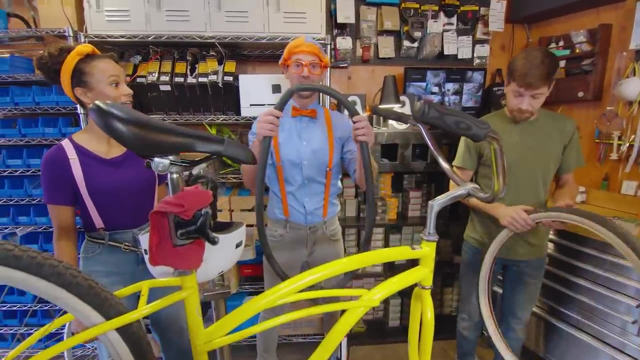 Yeah, Okay. And the next thing we're going to do is remove that tube, which is what created the flat tire. Whoa, So there's a tube inside the tire. Oh, can I check it out? Whoa, So this has a hole in it. 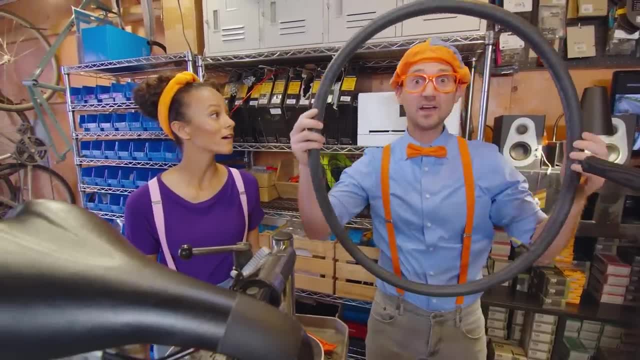 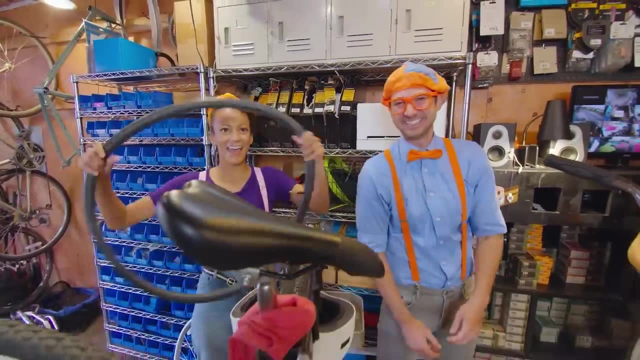 And this is what was inside the tire. That makes sense. Whoa, Oh, it's squishy, Yeah it is. It's like a balloon, Yeah, cool. There you go. Oh, So, as we're now done inspecting the tire, 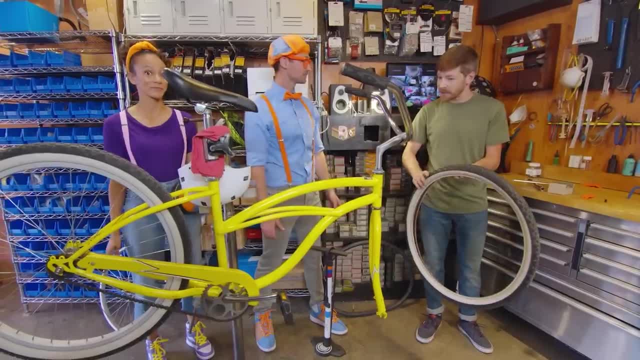 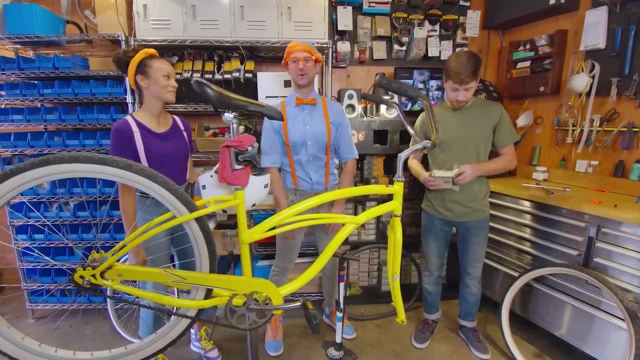 to see if there's anything stuck inside of this that created the flat. we're now safe to put a new tube back inside. Okay, so it's just the tube that had the hole. Yeah, so you're going to get a brand new tube. Yay. 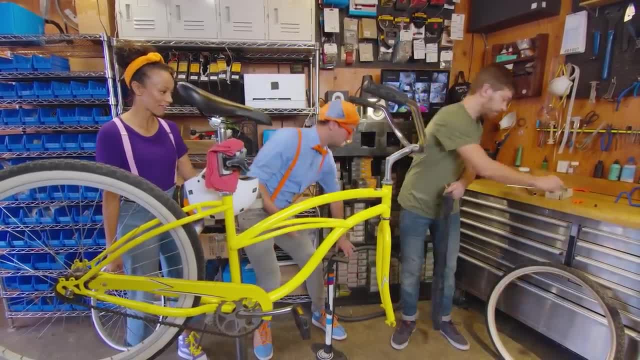 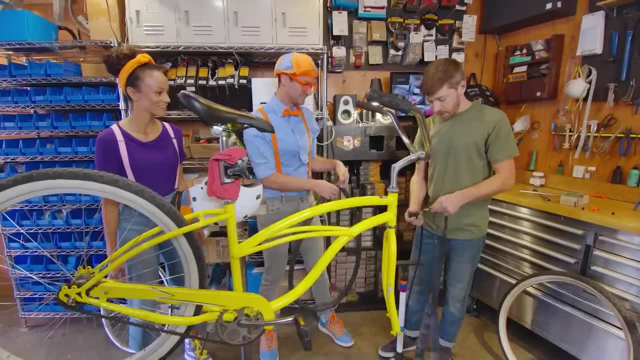 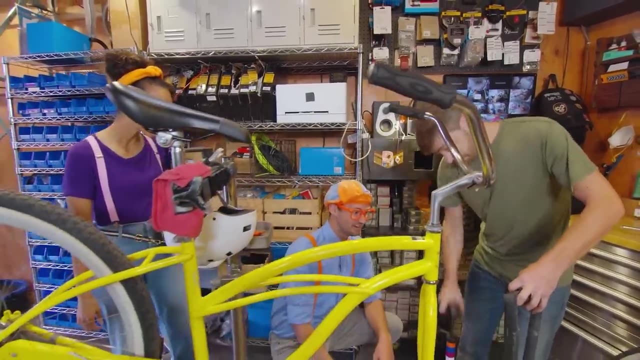 Whoa Yeah, it looks flat. Yeah, So that is this, but brand new, Exactly. So what we're going to do is fill it up with a little bit of air to make it easier to install. Whoa Cool. 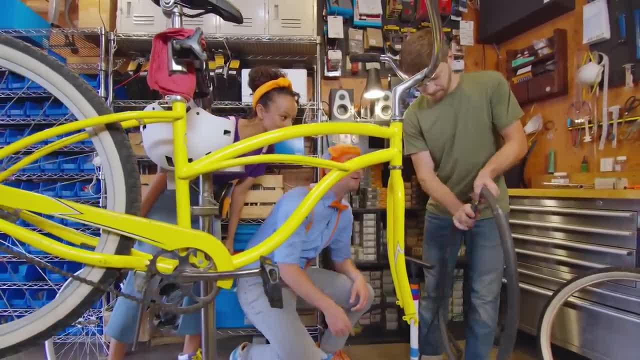 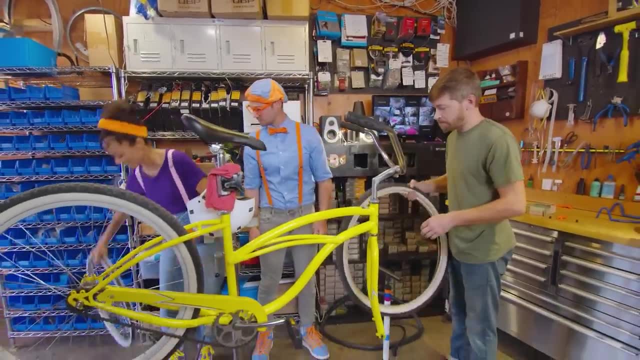 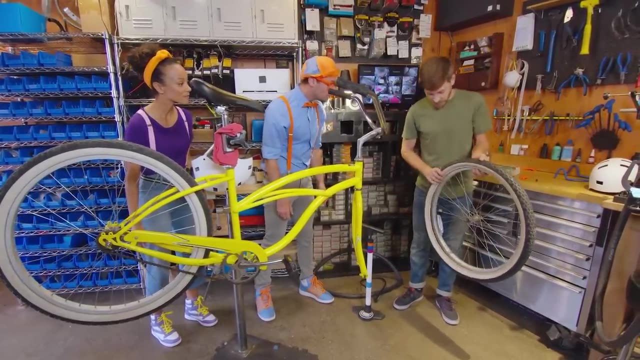 Look at it, It's getting blown up. Yeah Whoa, Next we will need that there. wheel back: Oh, here you go. One wheel, One wheel, Thank you. And so we're going to set just one side of this wheel inside. 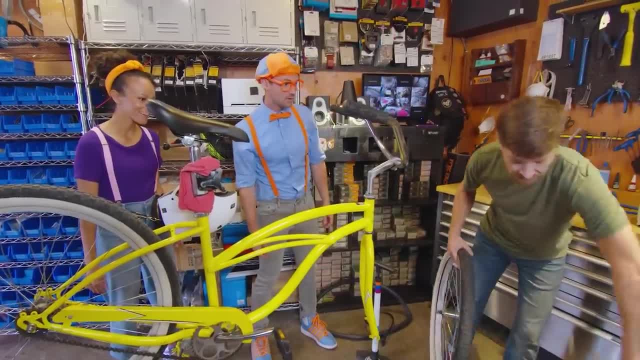 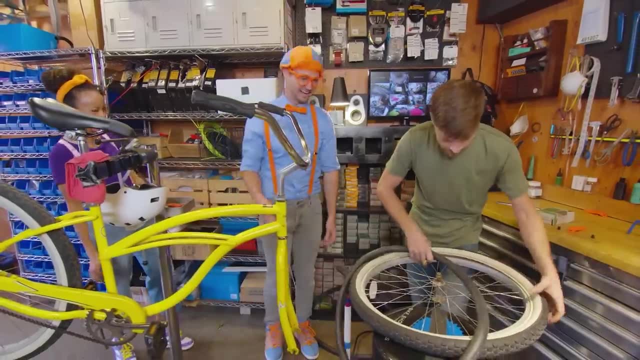 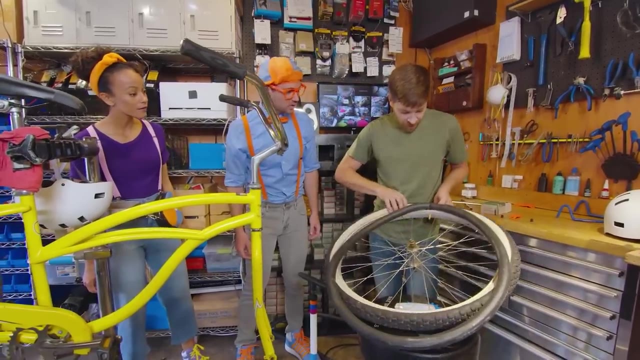 of the rim itself. Okay, And this is where I like to create a dinner plate, Dinner plate. I love dinner. I do. Whoa, Wow. So what are you doing now? I'm going to insert and reinstall a new inner tube to replace. 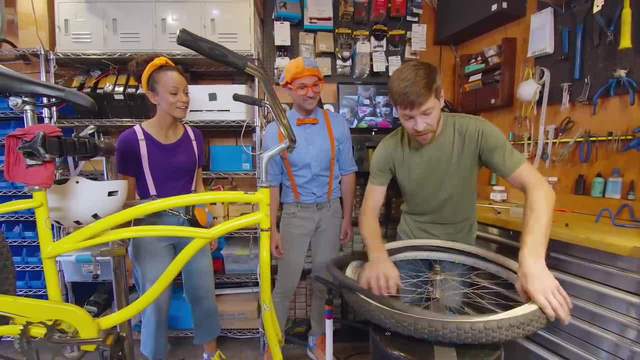 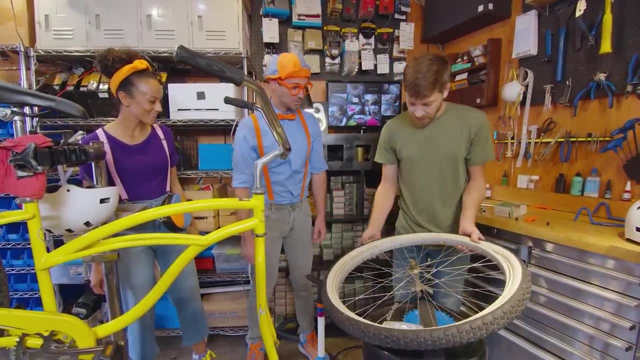 the compromised one. Wow, And you can see, once you have it set up like a dinner plate, it's easy enough to just add it back inside of the tire. Yeah, fits in nice, isn't it? And now we're going to. 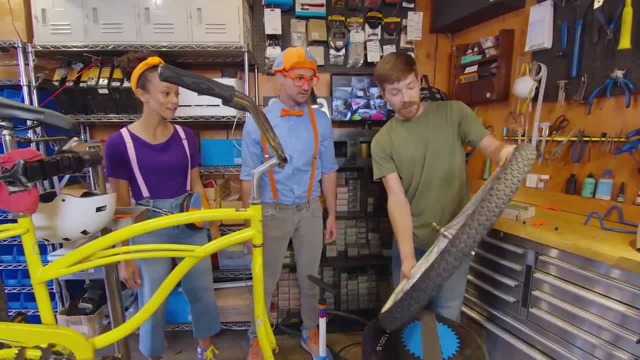 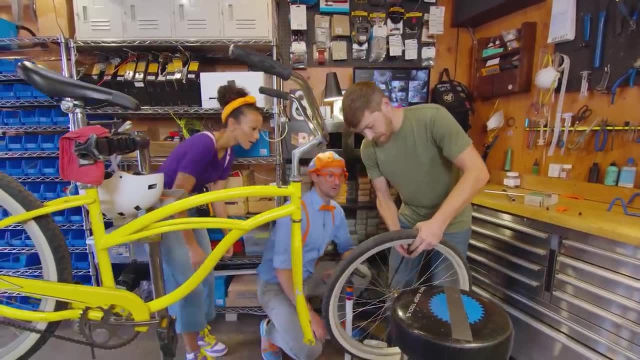 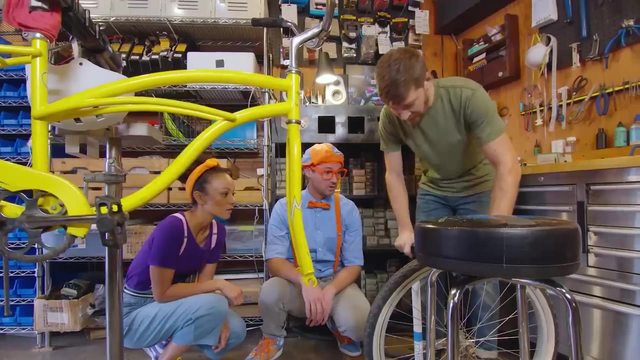 reseat the other side, just like that, and now we have a fully reinstalled tire. Yeah, Woo. So, last but not least, we're going to put air pressure back into the tire. Wow, This specific tire goes up to 40 psi. 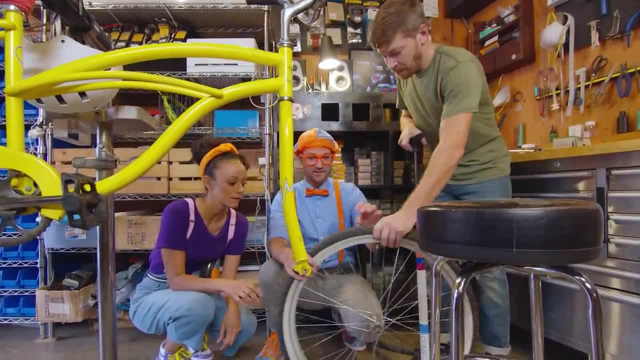 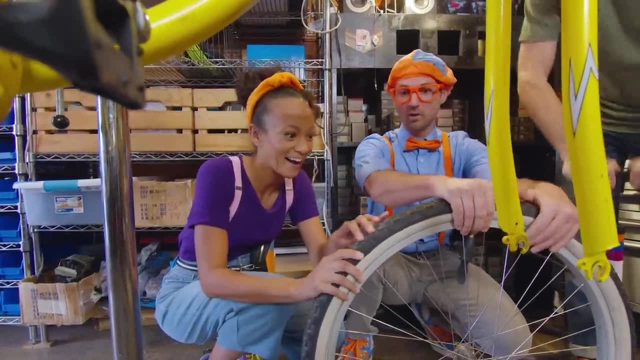 or pounds per square inch. Can I hold the tire and wheel? Certainly Okay. See if we can feel the air being pumped in there. Yeah, Oh, yeah. Whoa, It is feeling like a normal bike tire now. Yeah, it's. 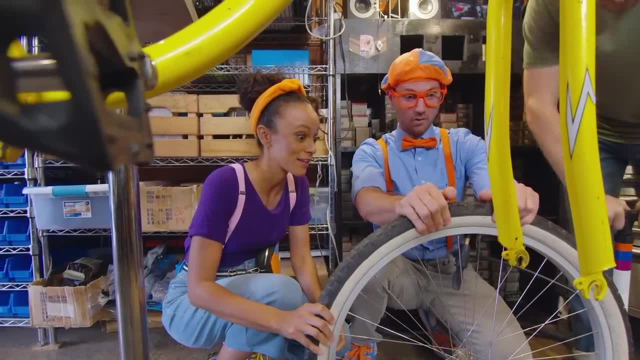 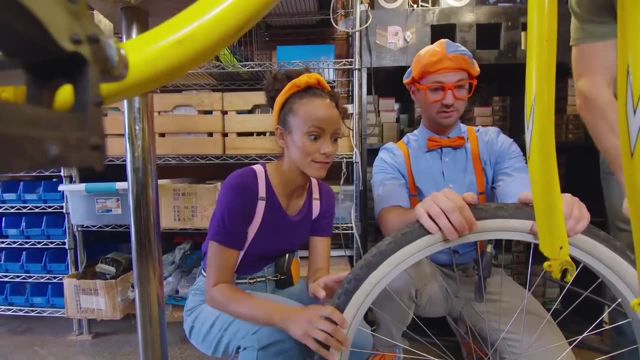 really filling up, Yeah Whoa. So when doing this, you always want to read the side of your tire first before you start to apply air pressure. Okay, And that way you won't over inflate the tire. Oh, so it doesn't explode. 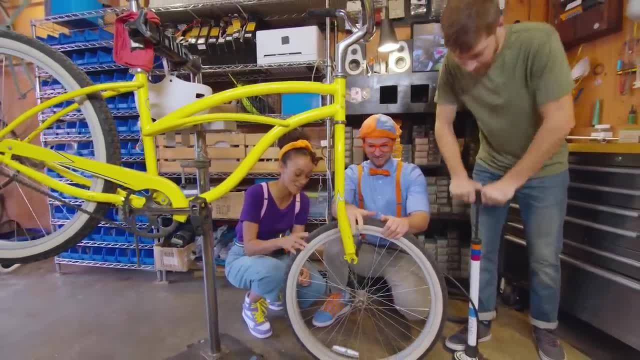 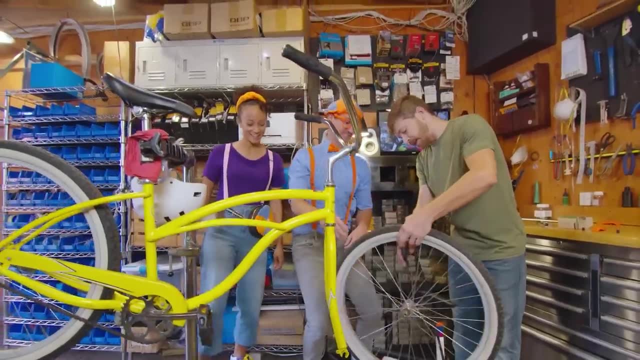 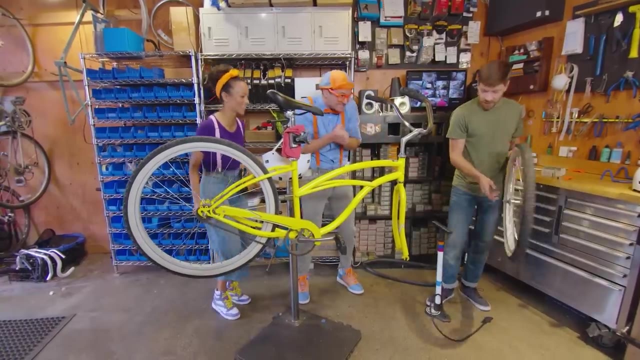 Makes sense. That's right. Wow, Now this feels like a bike wheel that you can ride on. Yeah, Yeah, And now it is. So, last but not least, we're going to reinstall this back onto the bicycle So that you. 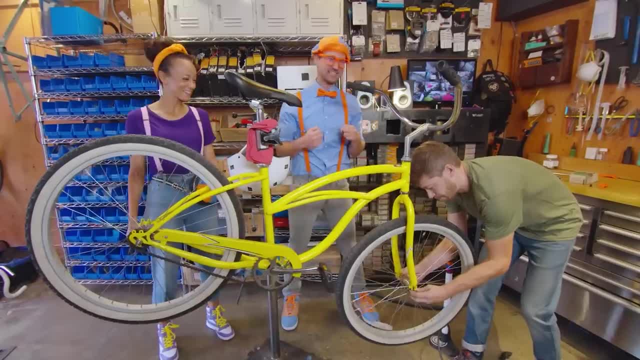 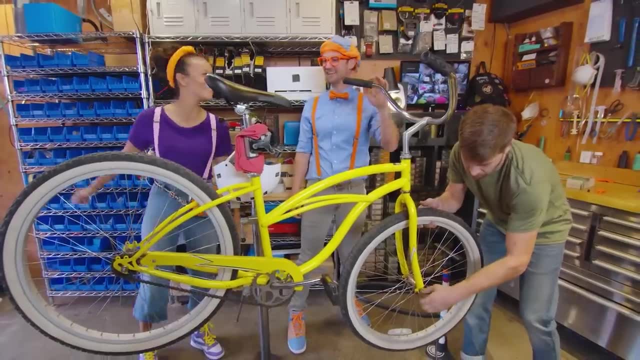 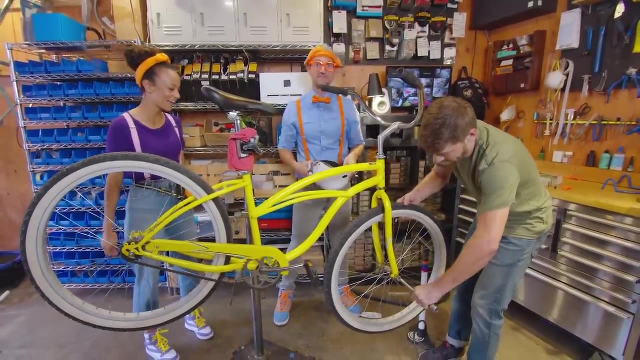 may continue your ride. Yay, Yeah, I'm so excited to ride my bicycle again. Whoa, There it goes. Whoa, It is new. Yay, Whoa, You are such a good mechanic, Dane. You did that so fast. 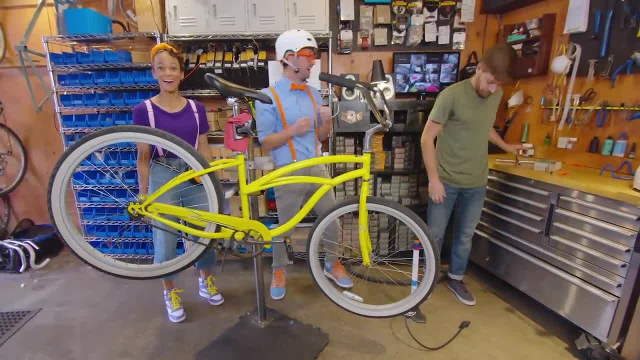 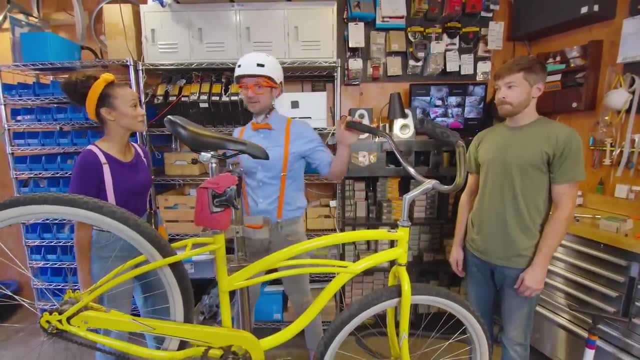 Wow And voila, Whoa Awesome. Thank you so much. Wow, Now I can ride my bike again. Oh, Blippi, can I ride bikes with you? Oh, that's a great idea, but I don't have a helmet or a bike. 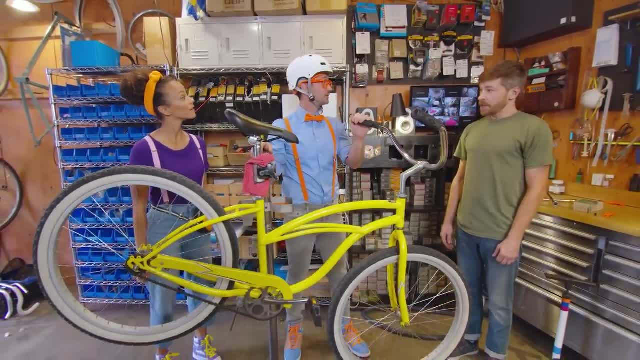 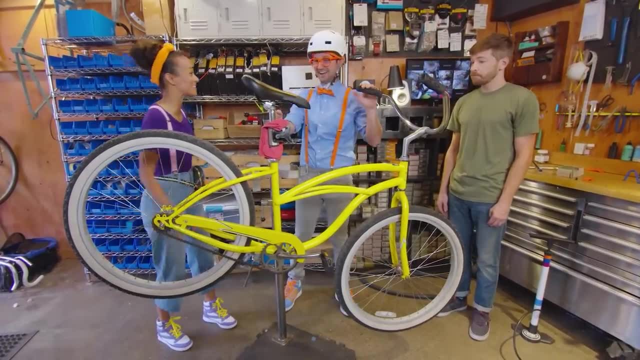 I don't have anything. Well, the good news here at Spoke Bicycle Cafe is we both rent bicycles and helmets. Yeah, Mika, you can come, I can't wait. Oh, can I maybe use that helmet right there, Indeed you. 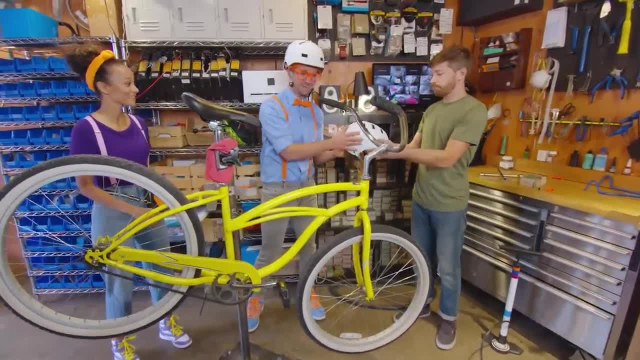 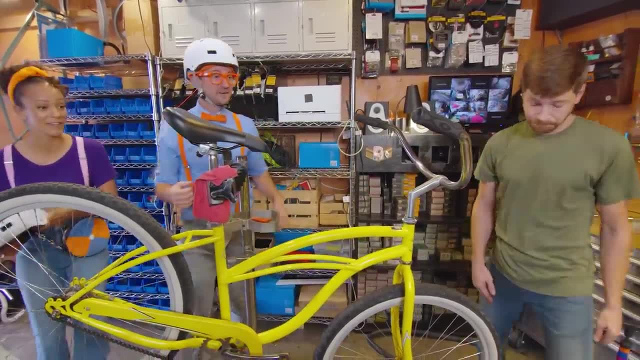 can. Oh great, Wow, Here you go, Mika. Thank you, All right, We just pick out a bike out there Indeed. All right, Let's go. Well. thank you so much, Dane, You're welcome Wow. 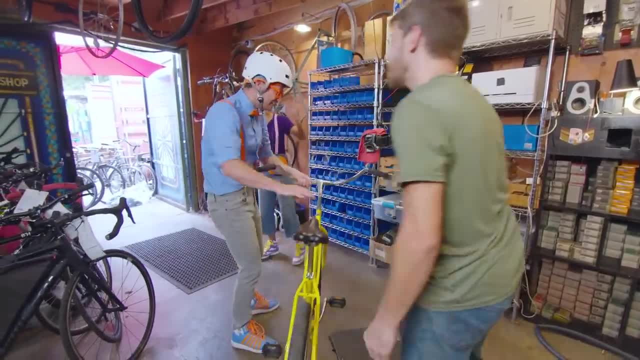 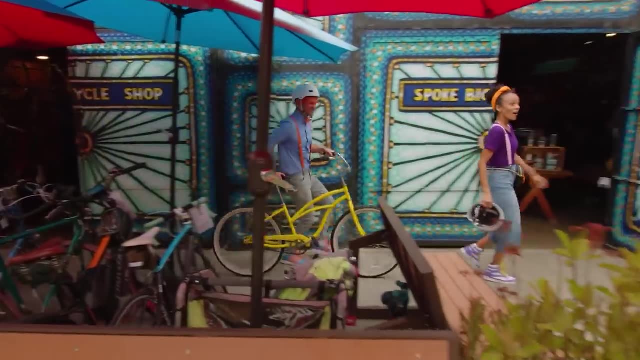 Cool, All right, See you later. Thanks, Dane, Enjoy your ride. See you later. Thank you, Come on, Blippi, All right. Yeah, So excited to see what bike you choose. Wow, Look at all of these bikes. 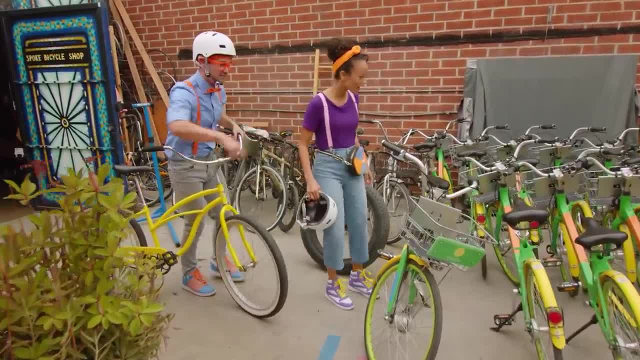 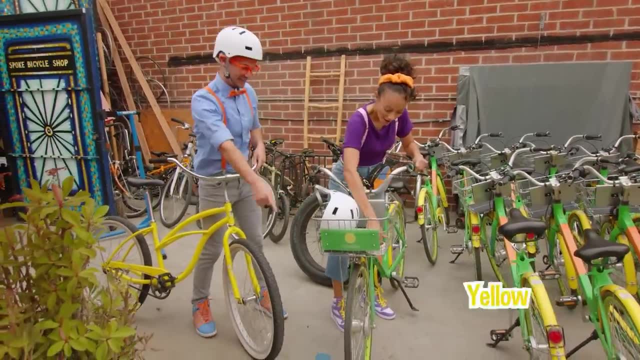 Whoa, That wheel's really big. Whoa, These bikes are so colorful. Yeah, I like these. I think I'll just take this one. Wow, Look at the colors. Yeah, Green, yellow and orange. Wow, So colorful. 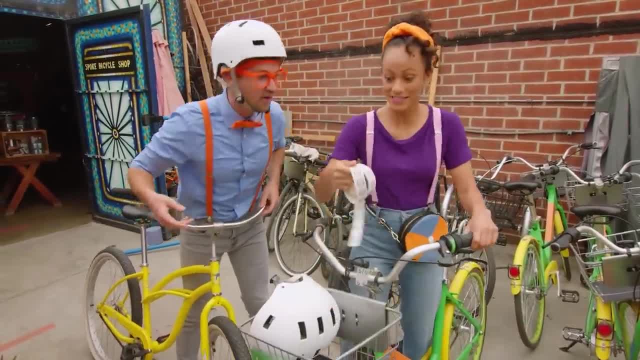 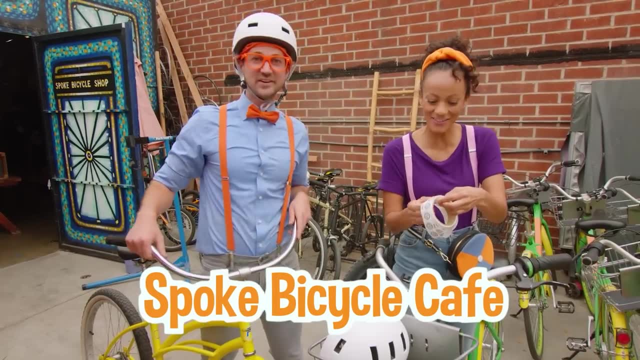 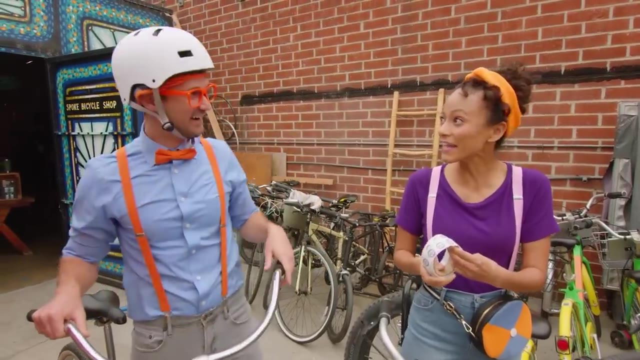 Whoa, What did you find? I found some stickers. Look, Wow Cool. It says Spoke Bicycle Cafe. That's where we're at. Do you want one? Sure, Here you go, Check it out. That gives me a great idea, Blippi. 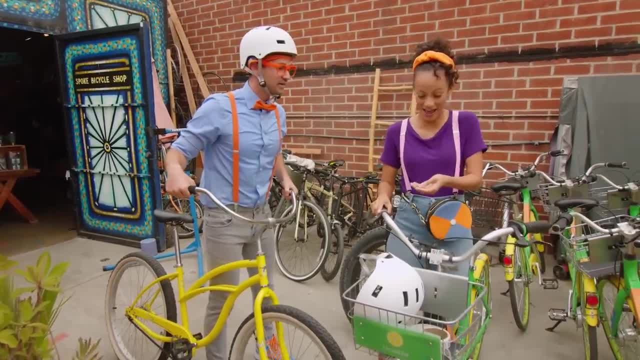 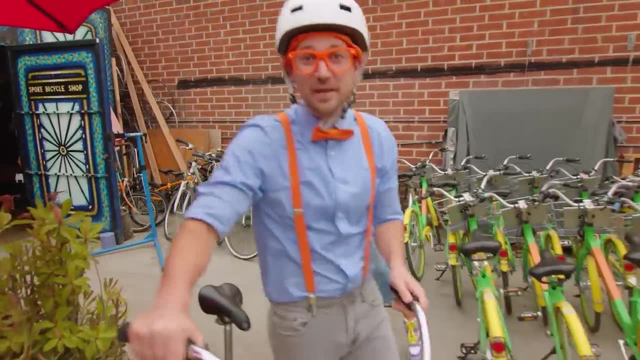 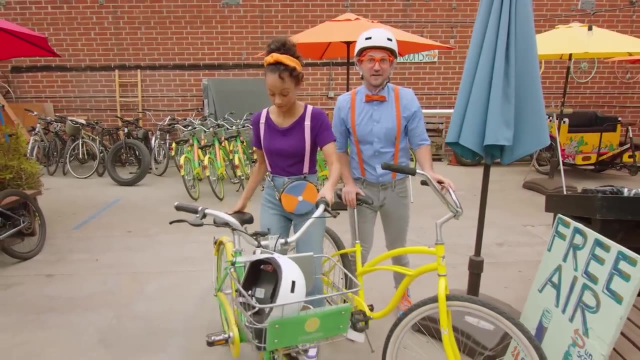 What I have- some other stickers right here in my bag. Do you want to decorate your helmet? That's a great idea. Let's decorate my helmet before we go on our ride. Okay, Whoa, Whoa, Okay. But you also said that they have. 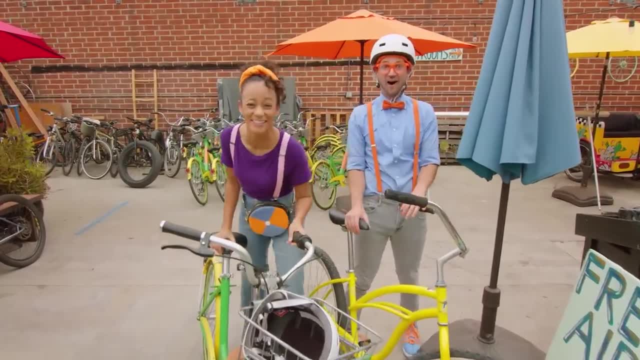 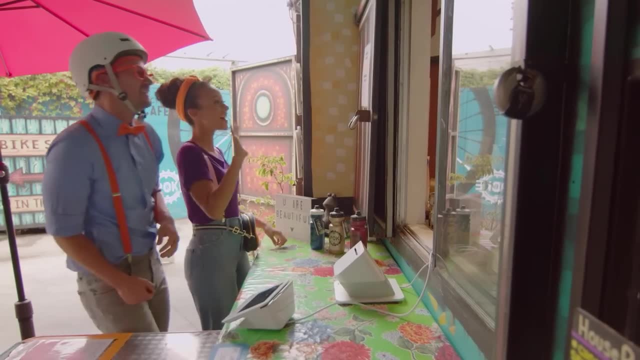 food and drinks- right, It's also a cafe. We should probably get hydrated before we go on our ride. That's a great idea. Yeah, Let's go. Come on. Hey, Hey, Hello. We're about to go on a bike. 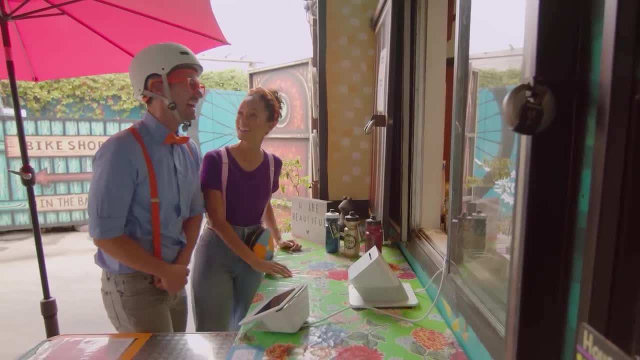 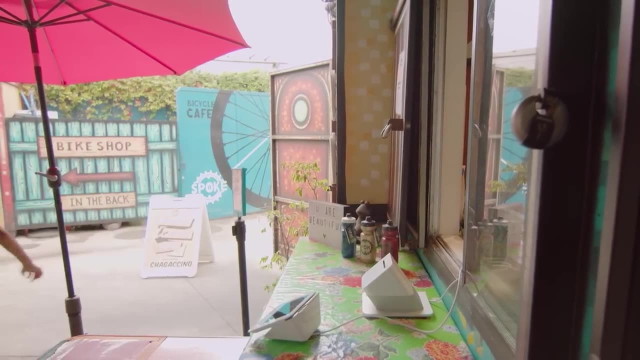 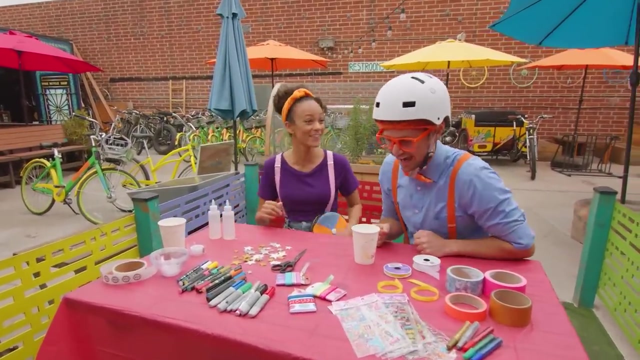 ride. Yeah, We're looking for some refreshing drinks before we go. Yeah, Do you have any water? Whoa, Thank you. Yum, Thank you, Whoa. Yeah, Look at all this stuff. Wow, Such great craft supplies. Yeah, Let's decorate. 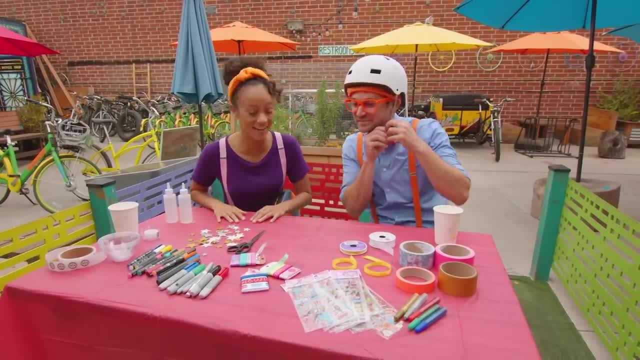 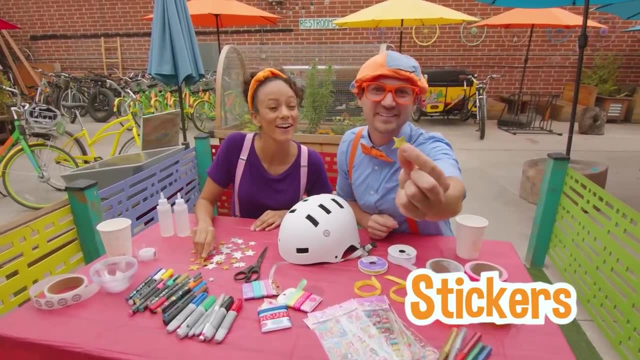 your helmet. All right, I love decorating. Yeah, This is going to be so much fun. Yeah, Looks like we have some stickers. Mm-hmm, Look A little star. Yeah, Which one is that? Gold, Gold, Ooh. 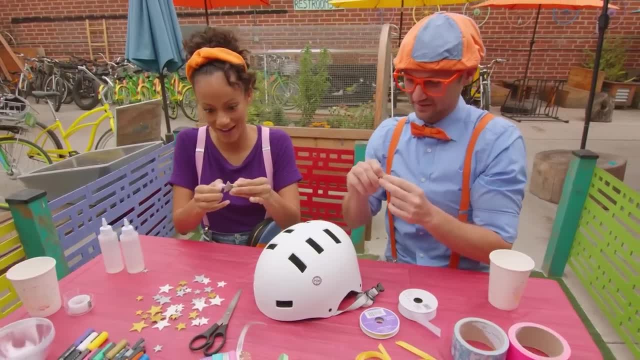 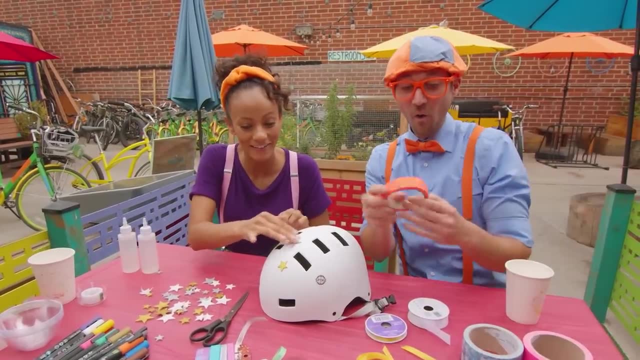 We have silver too. Okay, Ooh, Peel off your bag. It's a little tricky to peel it off. How about one right there? Nice, I'm going to put one here. Ooh, Orange tape, One of my two favorite. 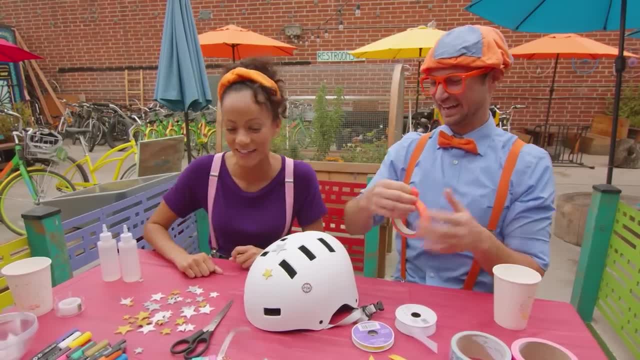 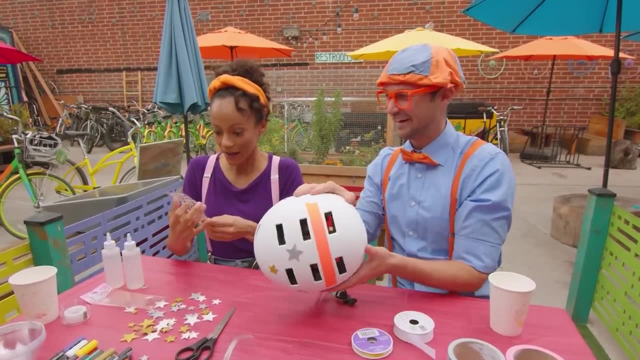 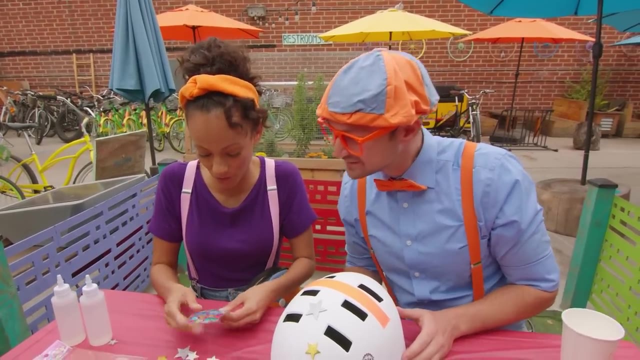 colors. I knew you were going to pick the orange tape. Yeah Ooh. And these are really cool stickers- Whoa All right. Wow, Look Underwater sea creatures- Whoa Cool. What animal are you going to pick? Hmm? 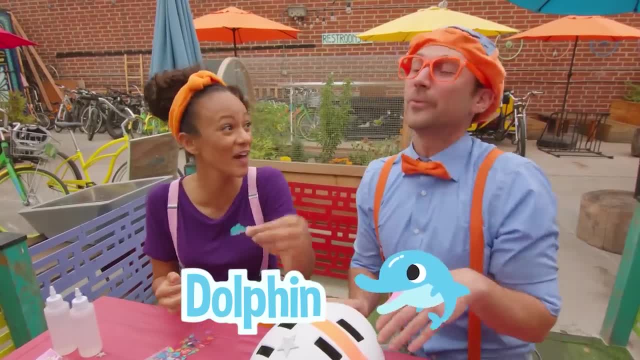 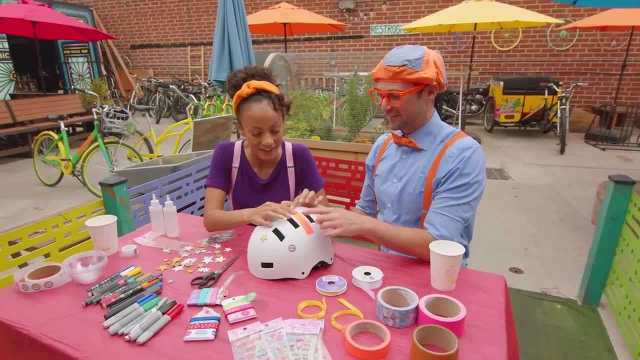 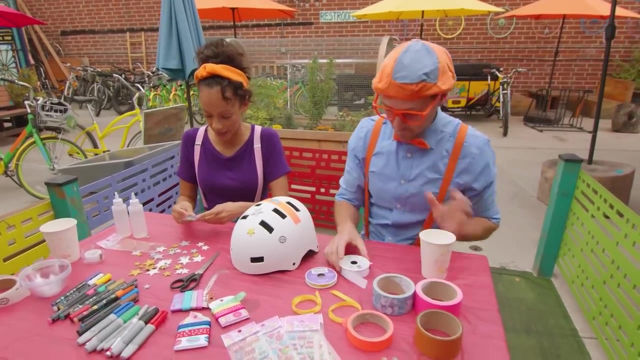 Ooh, What about this really fun dolphin. Can I put it right here on the orange tape? Sure, Wow, Cool. Orange and blue together- My two favorite colors, Yeah, Whoa, Ooh, I really like this walrus. 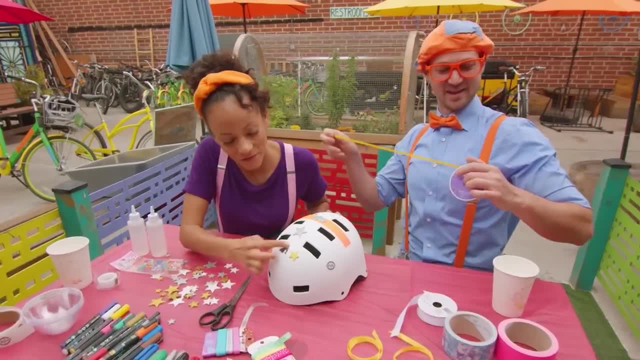 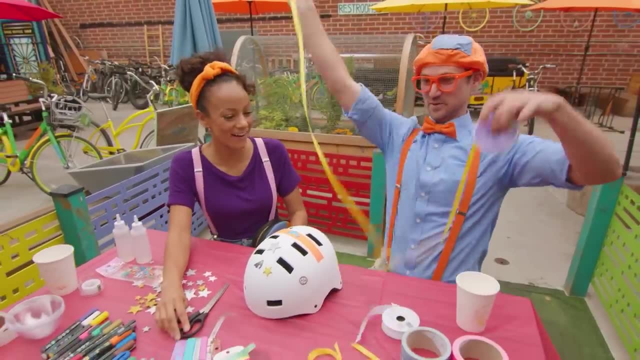 Whoa, Yeah, Another animal that lives in the water. Yeah, Ooh, Check this out. Whoa, Do you know what I'm going to do with this? No, It's a surprise. Do you need help cutting Exactly? 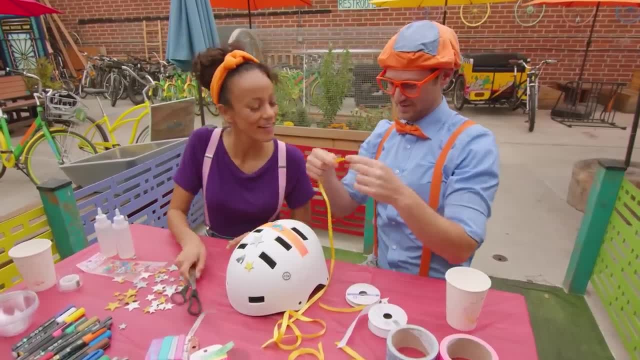 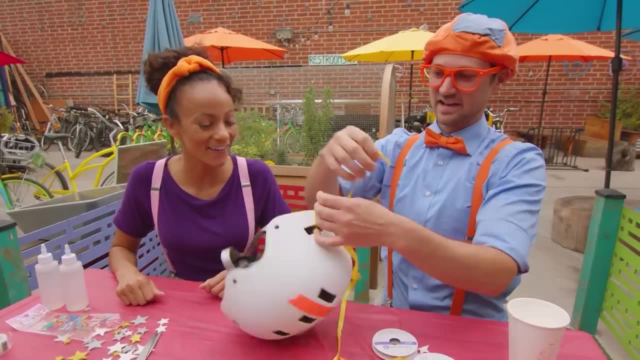 Yeah, Thank you very much. All right, Watch this. Okay, I'm going to put it in this hole and then I'm going to put it out of this, Wow, And then I'm going to tie a little knot And I'm 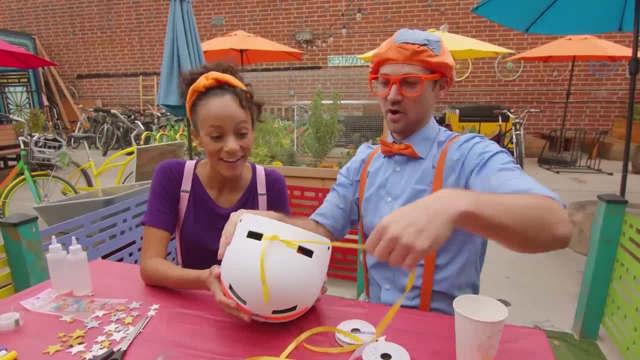 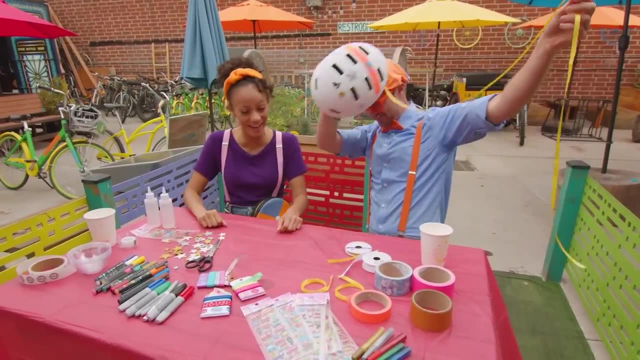 going to make really cool ribbon tail, So then when I go super fast, it'll fly in the air. That's such a great idea. Maybe we should cut it just a little shorter though. Yeah, How about right there, Like that. 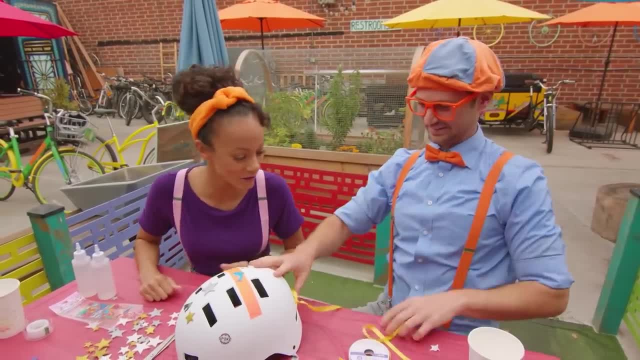 Yeah, Perfect, There you go. All right, That's going to look really, really cool. Oh, thank you, And you might be able to Do. we need to try to make it a little curved. Ooh, cool, I don't know if it'll. 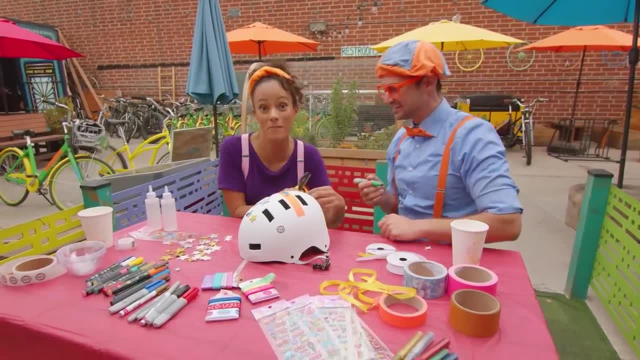 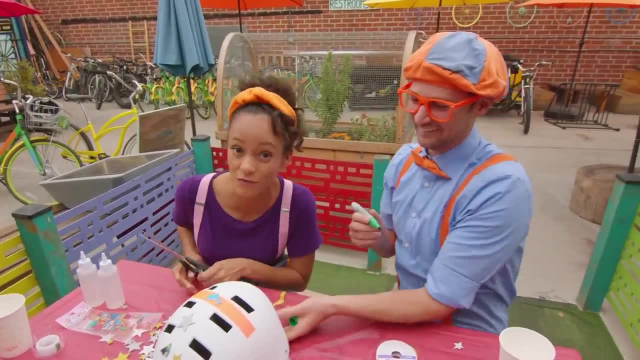 work with this ribbon, but it's a trick, All right, This is something a grown-up can help you do to make your ribbon. It's not working, That's okay. Yeah, Let's use a different ribbon for that trick. Yeah, And here's a green marker. 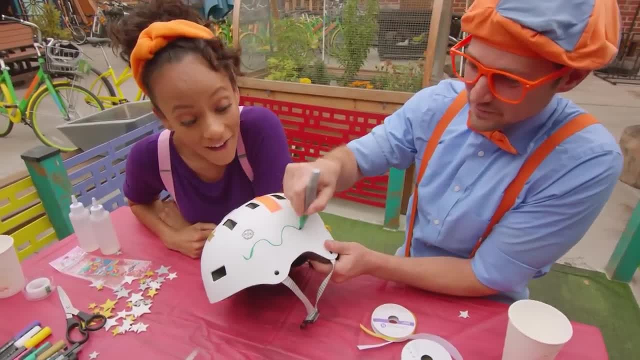 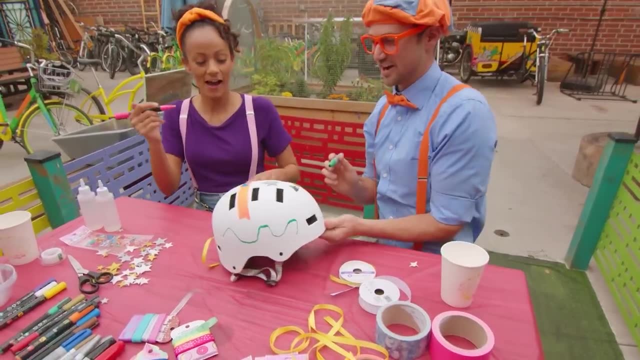 Ooh, All right, Let's make some squigglies on that side. That's a good idea. Yeah, You're really good at drawing. You should try and draw. I'm going to do a big pink heart on the back. 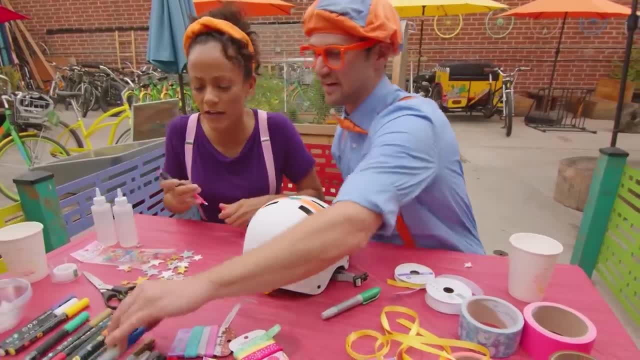 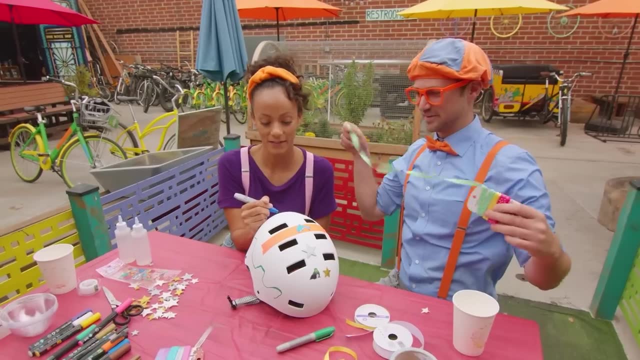 This is pink. Wow, Let me try a different. Yeah, That would be good. All right, One of your favorite colors? Yeah, Okay, And I'll work on another ribbon. Whoa, It's going to be a surprise what she's drawing. 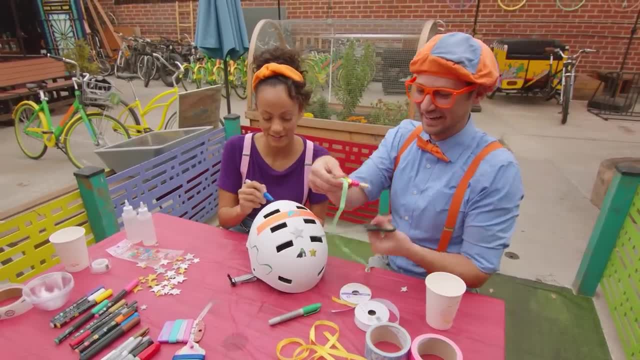 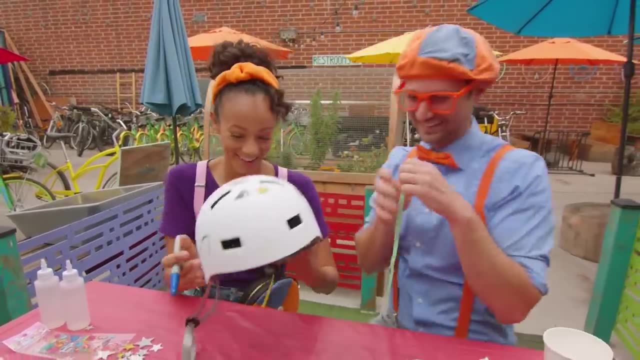 Whoa, That is so cute of you to do that. Yeah, Are you excited to see what she's drawing? A blue heart for my best friend, Oh, Miko. Yeah, Okay, I cut another ribbon. Ooh, Look at the stars on it. 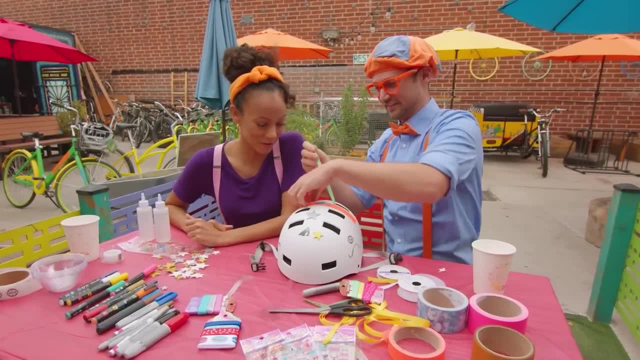 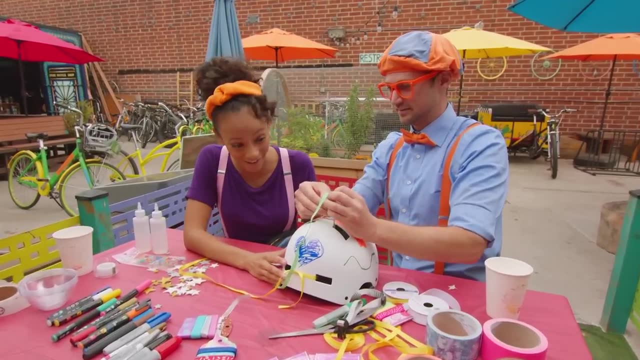 Yeah, I just think it'll look so cool when I'm writing really fast. It will. It'll be blowing in the wind. Yeah, All right, Check it out. All right, How does this look? It looks very good. Okay, Do you think it looks good enough? 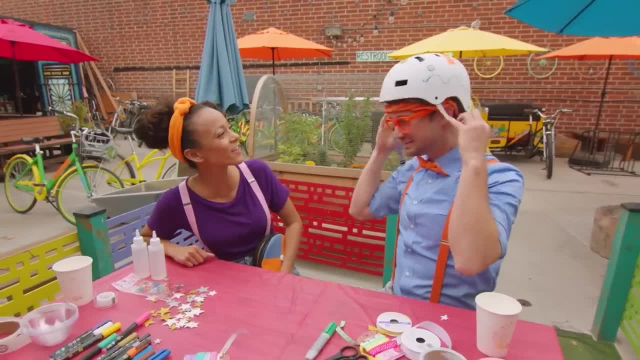 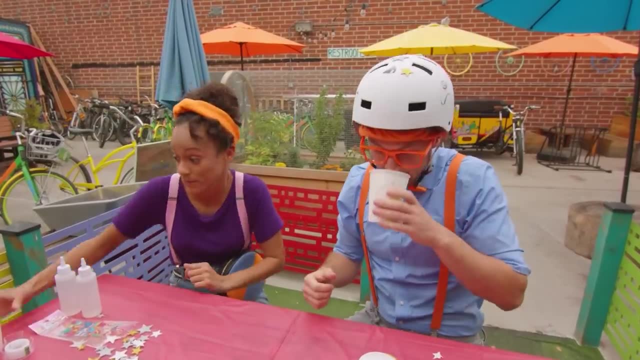 Yeah, All right, Let's try it on. Okay, Let's see how you look. Blippi, This helmet is fabulous. Yeah Well, shall we go on a ride? Oh yeah, Let's go. Okay, We'll come back here later to clean up. 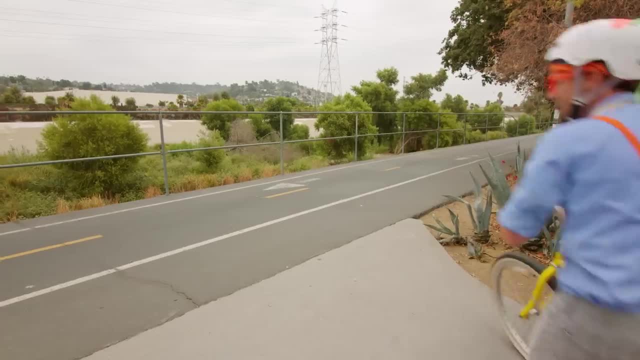 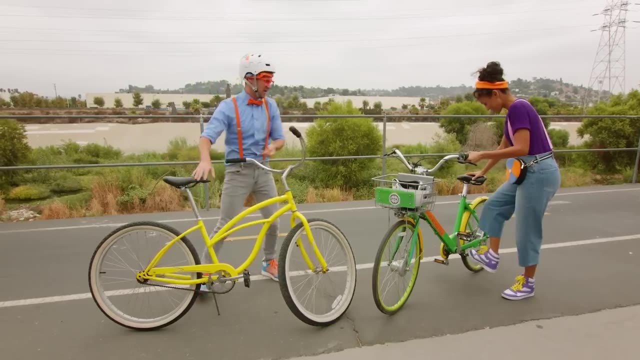 But now let's go on a ride. Yeah, Woohoo, This is going to be so much fun. Yes, This is such a great day to ride bikes together. Yeah, We have cool looking bikes. Yeah, We drank a bunch of water. 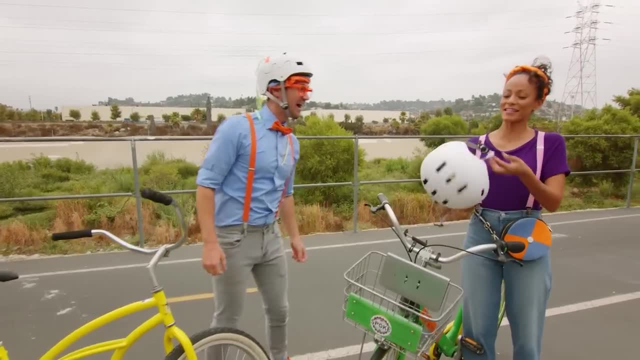 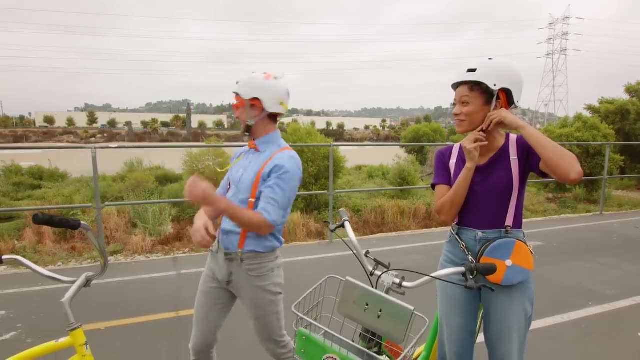 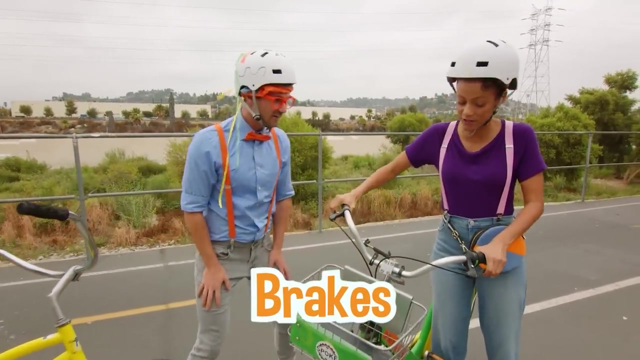 So I think we're ready. I need to put my helmet on so I'm nice and safe. Oh yeah, And we decorated my helmet. I look real cool. You look so cool. Yeah, Hey, check this out. I have brakes on my bike in case I need to stop. 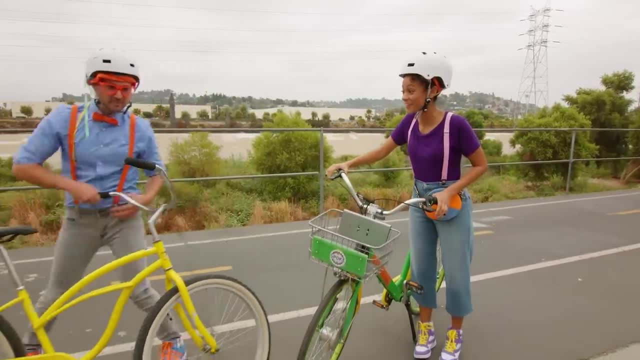 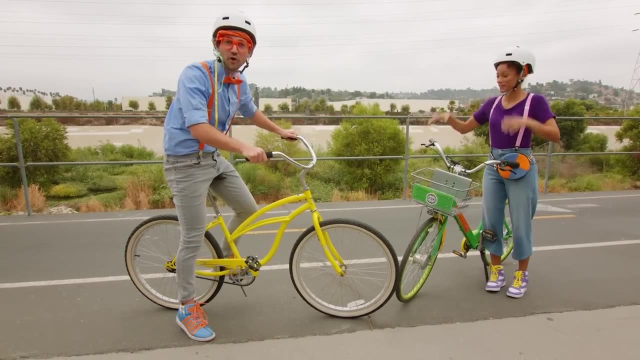 See, I just pull back like this. Oh, yeah, With your hands. Yeah, Oh. and look at my bike. Yeah, I don't have hand brakes. Yeah, I have brakes when I pedal backwards. That's right. Yeah, Are you ready? 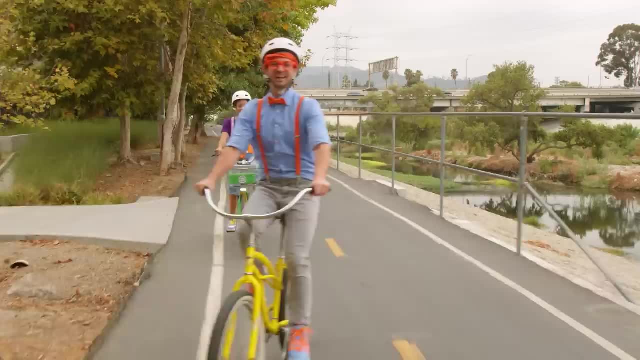 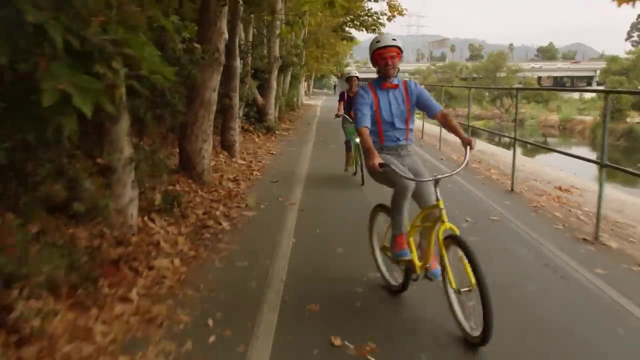 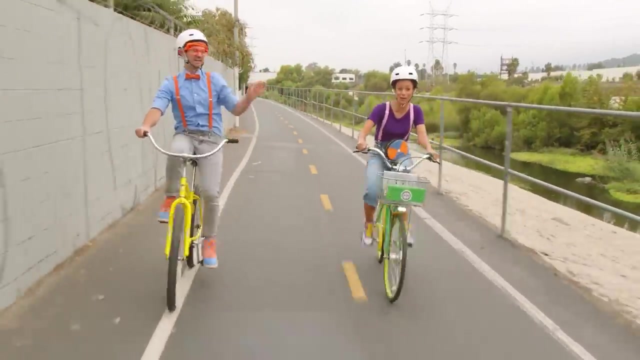 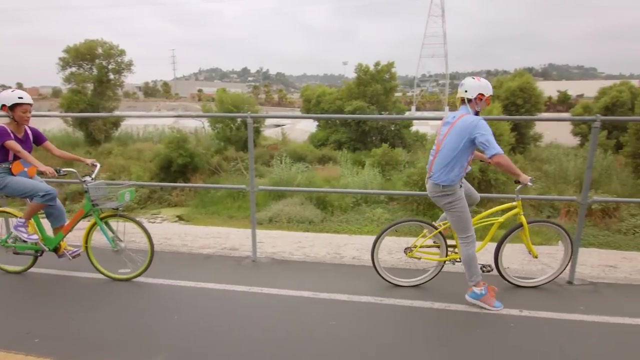 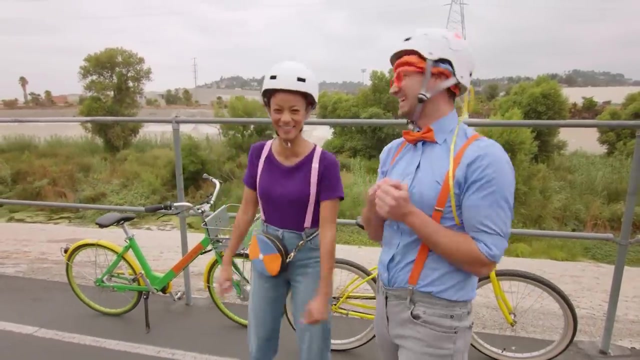 Oh yeah, I can't wait, Let's go. Whoa, Yeah, Yeah, That was awesome, That was super fun. Wow, I love riding bikes- Me too. Blippi, Oh, Mika, Yeah, Two people for two bikes. 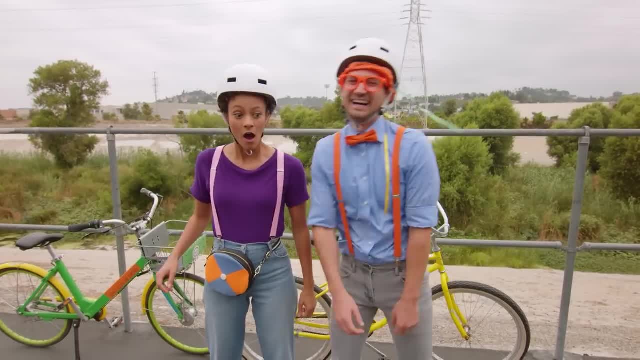 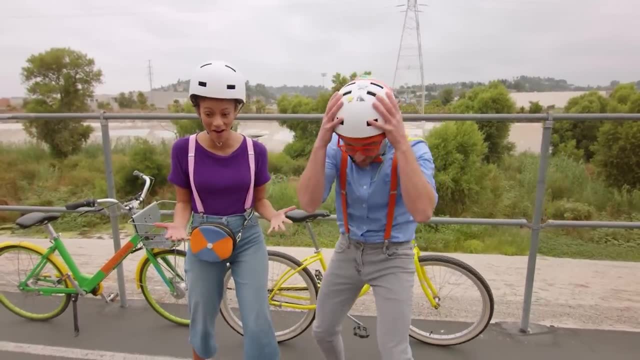 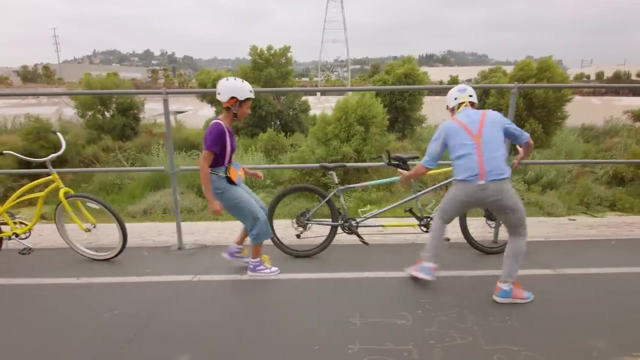 Yeah, It's so fun riding bikes together. Yeah, What if there were a bike where two people could ride the same bike? What, That would be so cool. Yeah, What, What? Look at this, This is a tandem bike. 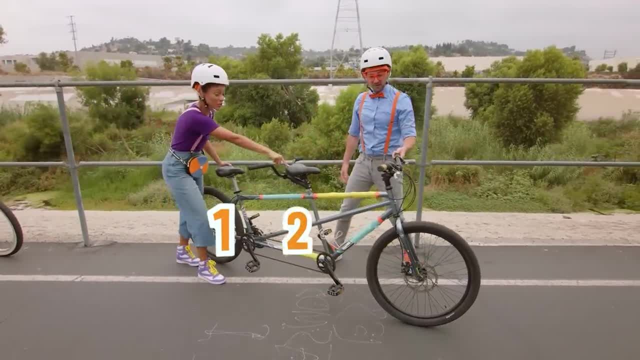 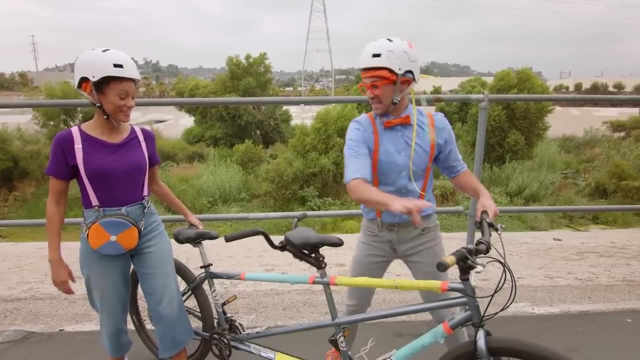 Wow, There's two seats on this bike: One, two and two sets of handlebars. Yeah, These handlebars up front are for the person that steers Yep, And these are for the person in back, So then they don't fall off. 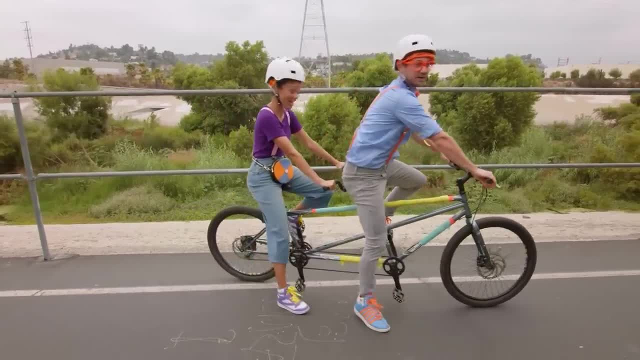 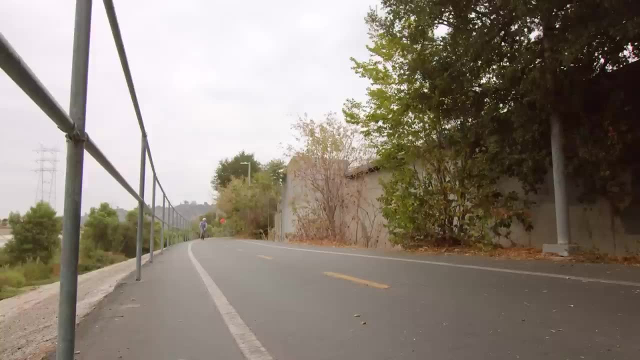 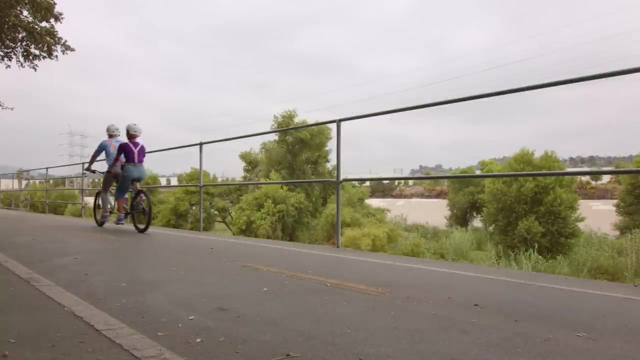 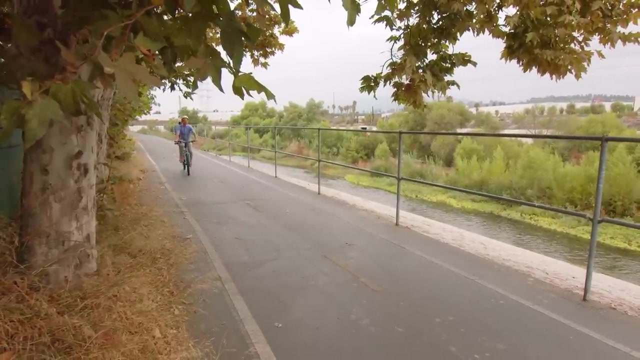 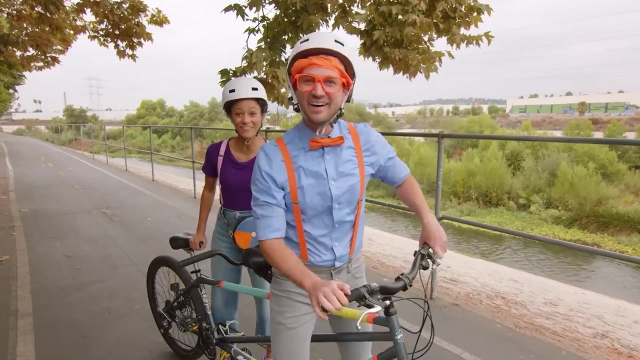 Yeah, Shall we try it. Yeah, I can't wait. All right, Two people, one bike, Here we go. Okay, Music, Wow, That was so much fun riding bikes with you, Mika. Yeah, it really was. 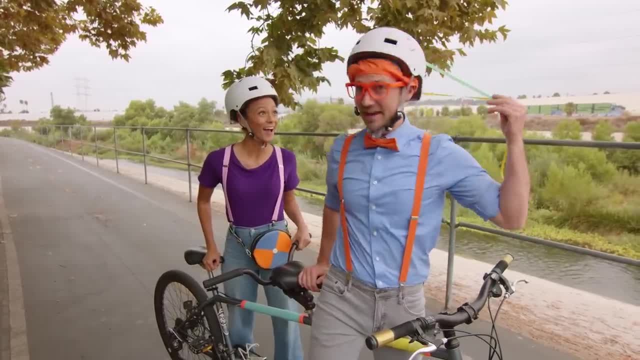 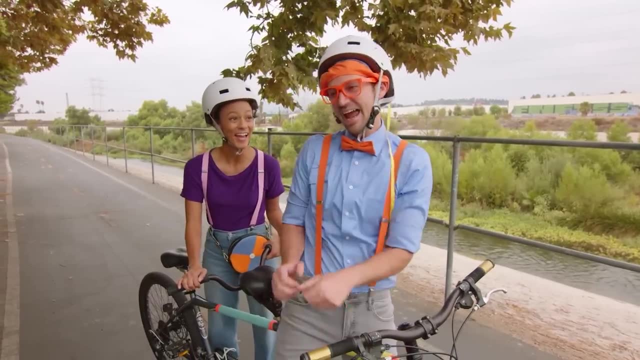 We had a great day riding bikes. Yeah, It was so much fun decorating my helmet with you. Yeah, it looks so good And I'm really happy that you got your tire fixed. Oh thanks, Mika. Yeah, and it's really cool how we learned that you need to stay. 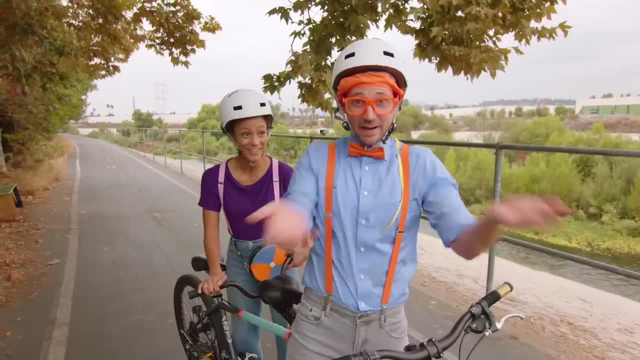 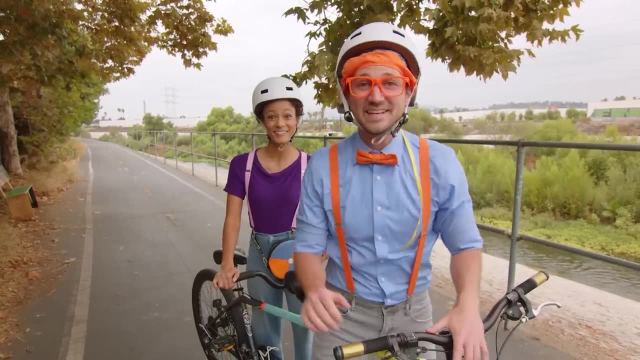 hydrated before you do really active things like riding bikes? Yeah, and riding bikes are great. It's good for the planet and good for your body. Yeah, well, this is the end of this video, but if you want to watch more of my videos, all you have to do is search for my name. Yeah, Will you spell? 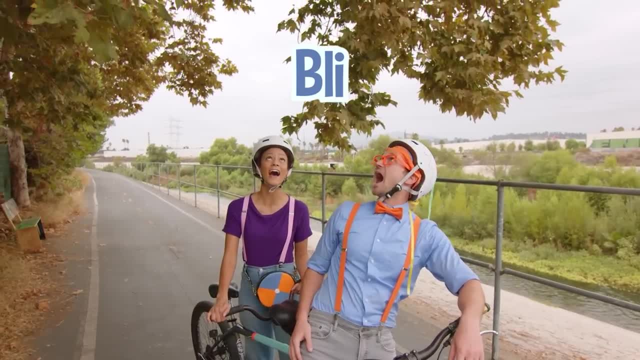 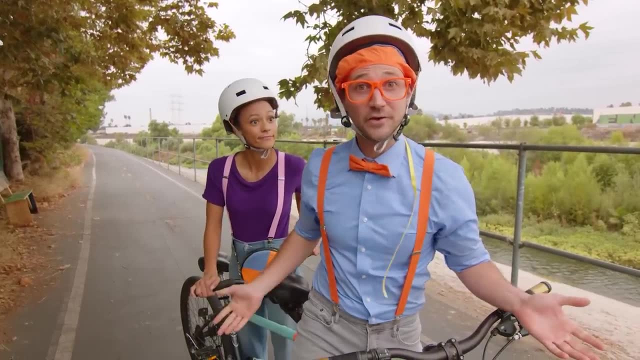 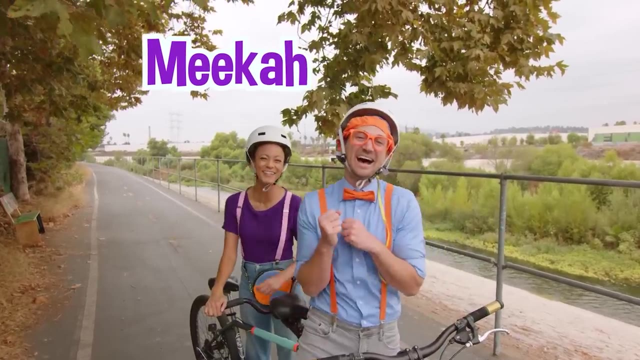 my name with me. Uh-huh, B-L-I-P-P-I- Blippi, Good job. Hey, Mika, how do you spell your name? Oh, I'll show you. It's M-E-E-K-A-H. Mika. Wow, that is so cool. All right, see you again. Bye-bye, Here we go. 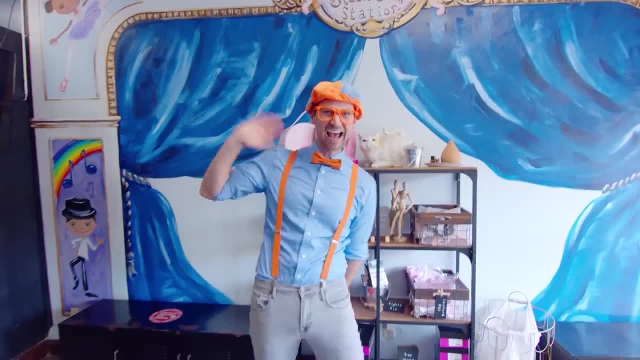 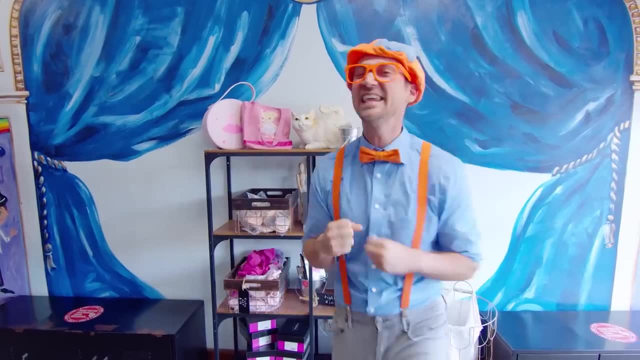 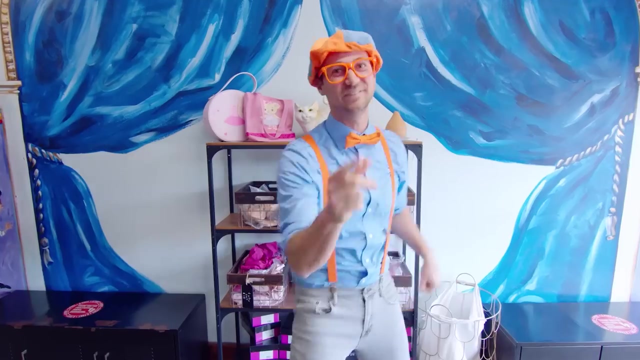 Woo-hoo, Whoa, Hey, it's me Blippi, And today we're at Creation Station in Studio City, California. Yeah, I love this place. This is a place where you can dance. Yeah, they have dance lessons here, and you know I love dancing. 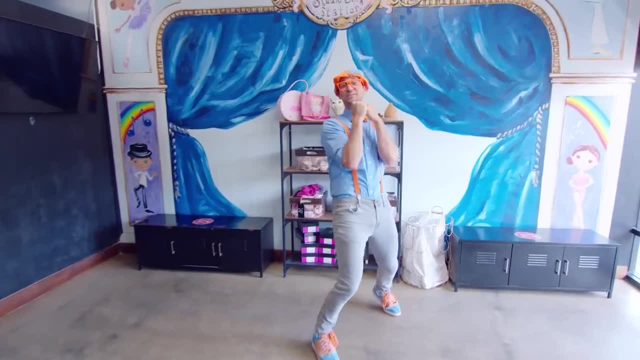 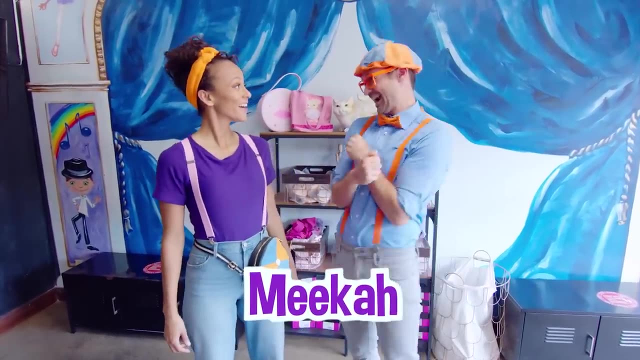 But first I have someone really special to introduce to you. Hey Blippi, Hey Mika, Hi everyone, This is Mika, She's my best friend. Oh, Blippi, you're my best friend. Oh, so silly, I'm so excited. 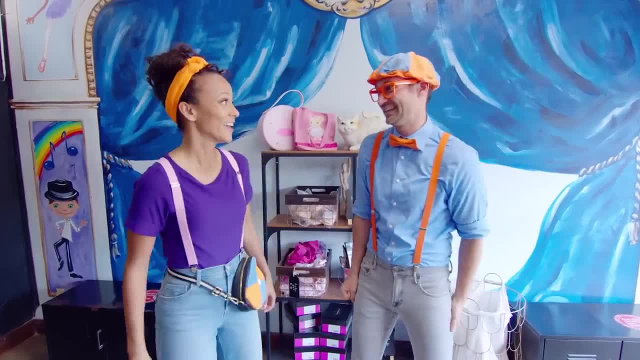 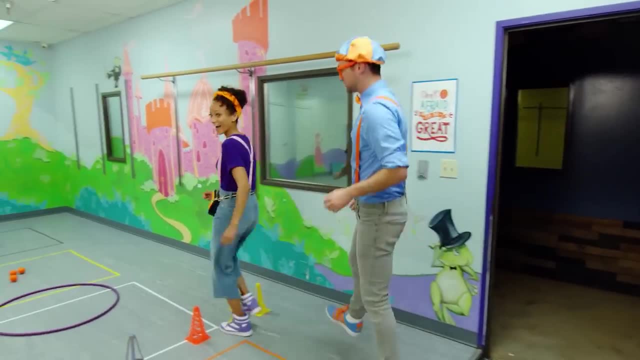 because, Because we're at a dance studio. Yeah, Are you ready to dance? I'm so excited. Yeah, let's go, Come on. Whoa, Well, we should probably warm up before we do some dancing today. Yeah, same idea. Look at all. 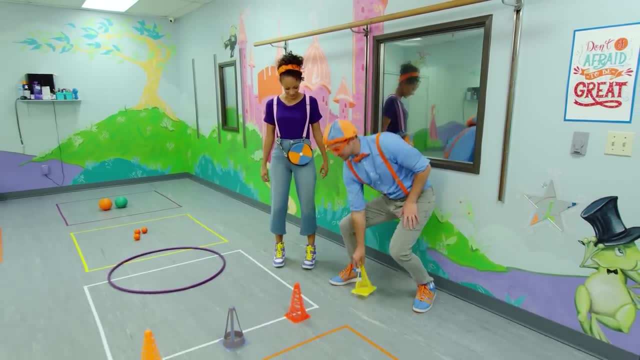 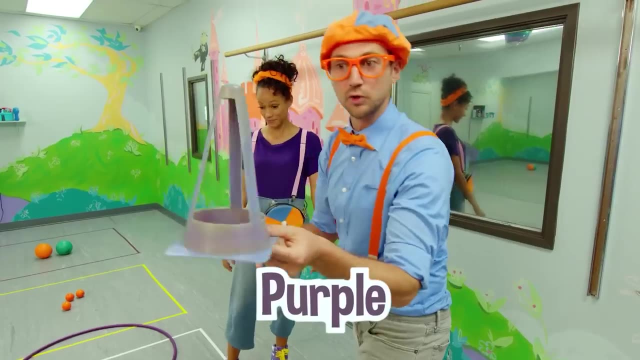 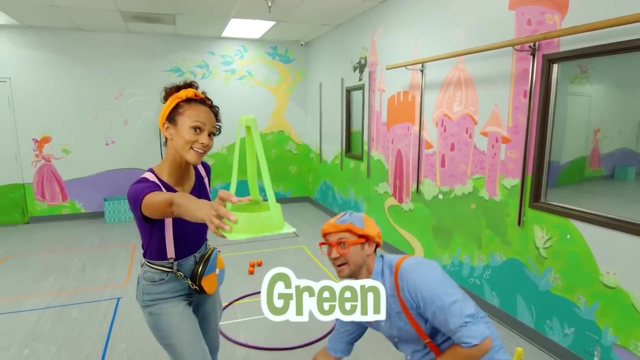 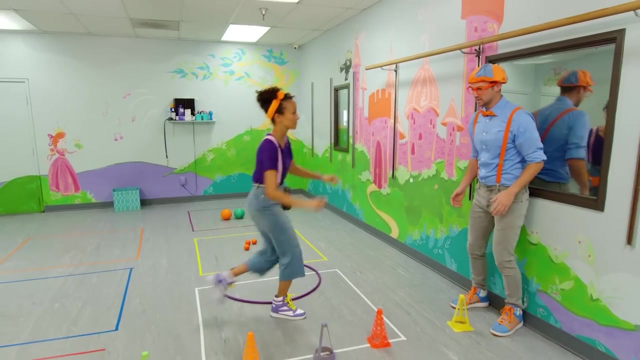 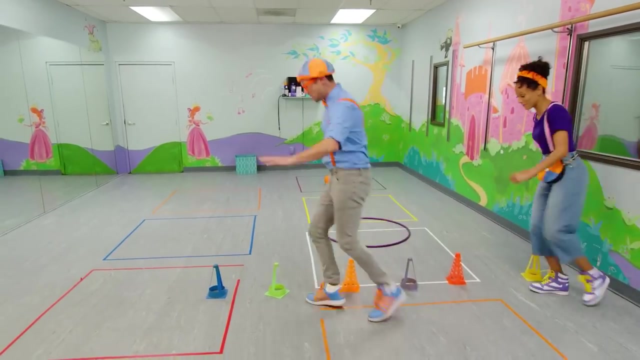 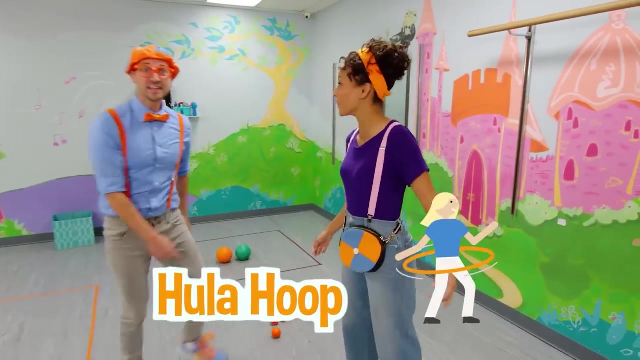 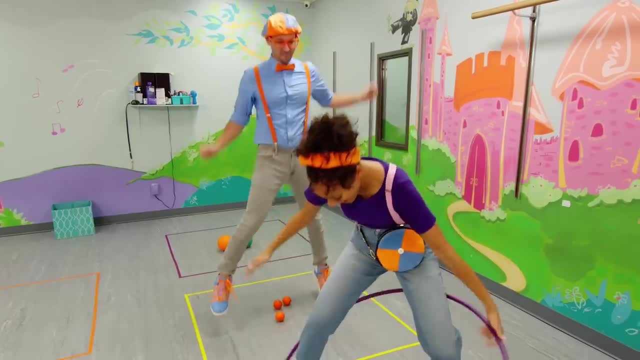 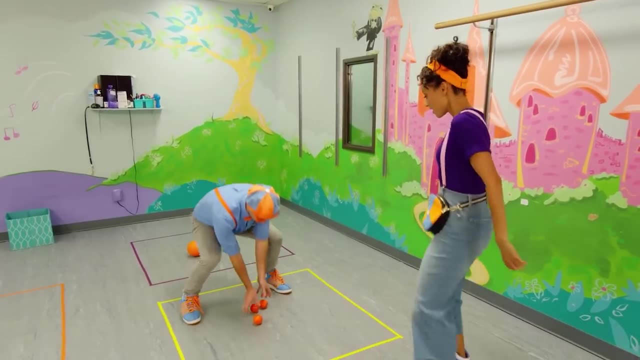 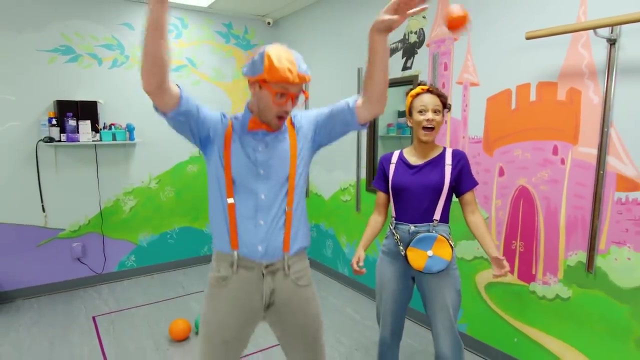 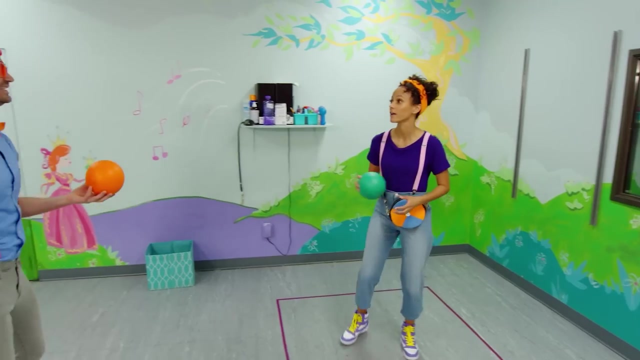 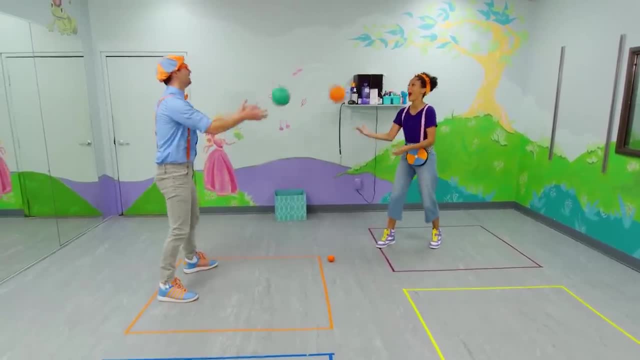 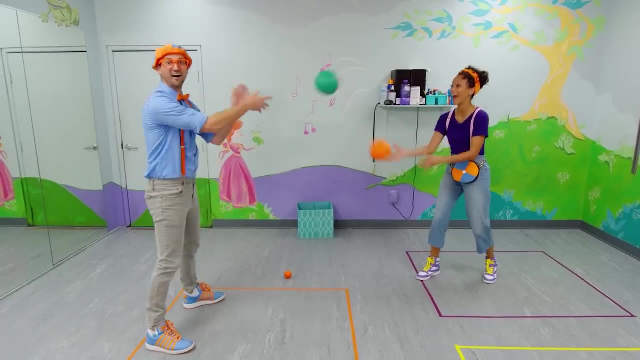 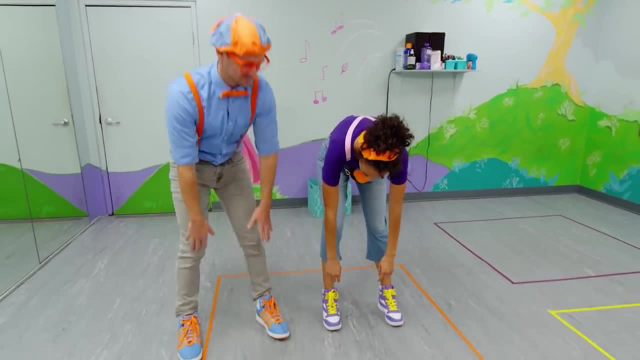 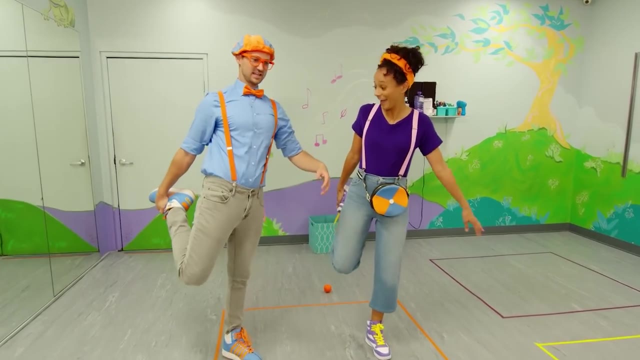 Yeah, let's do some stretches. All right, Yes, Stretch your toes. Oh Oh yeah, Feels good to stretch. Yeah, it does. Ooh, Nice leg stretching. Now we're gonna be able to dance really good. 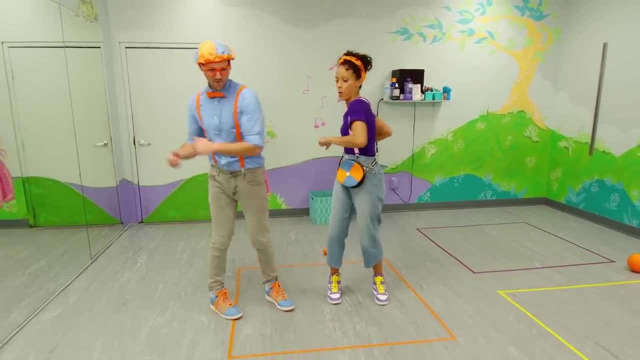 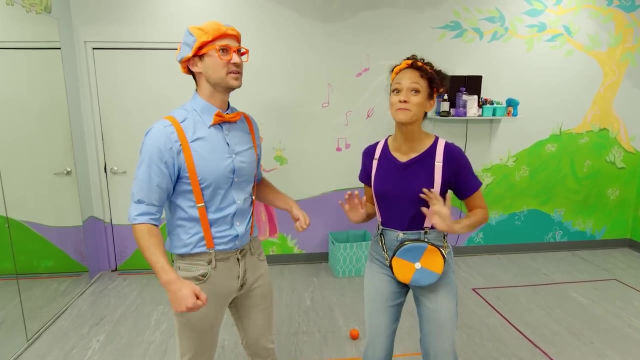 Yeah, I cannot wait to dance. Oh, Hoo, Hoo, Hoo Hoo. Do you hear that? Yeah, It sounds like beautiful music. Yeah, I wonder if someone's dancing to the music. Let's go see. 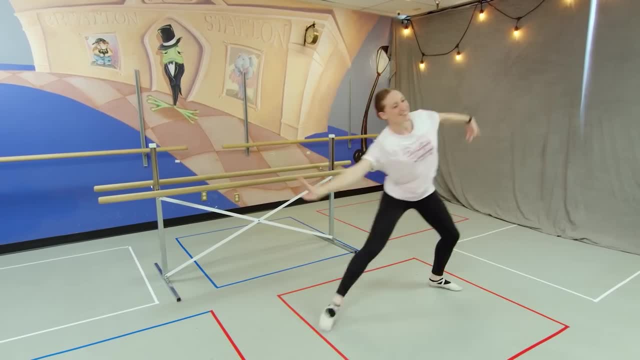 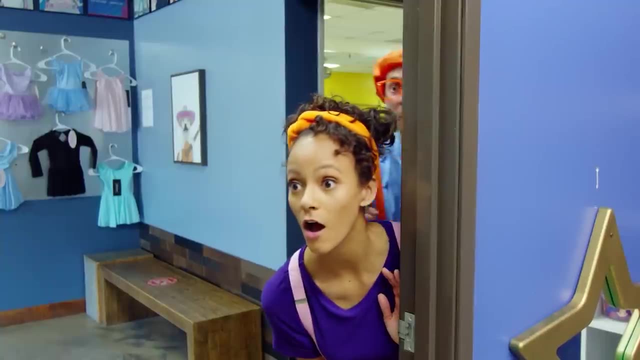 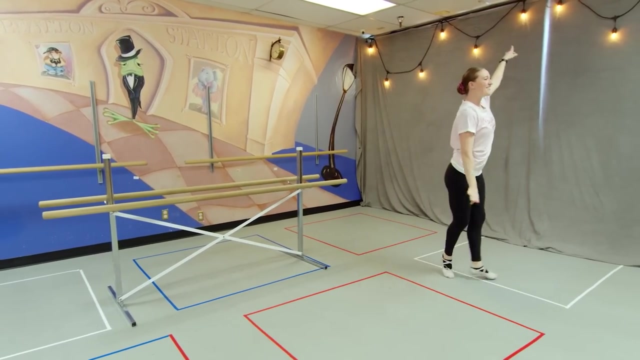 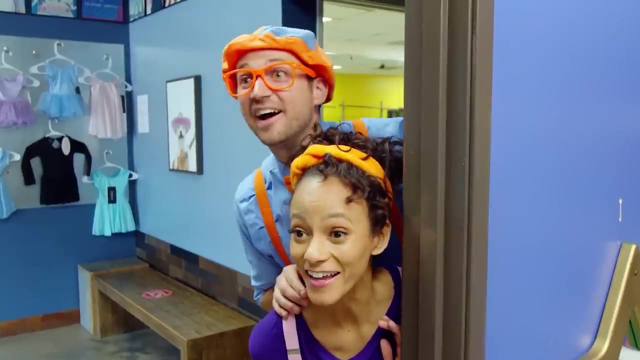 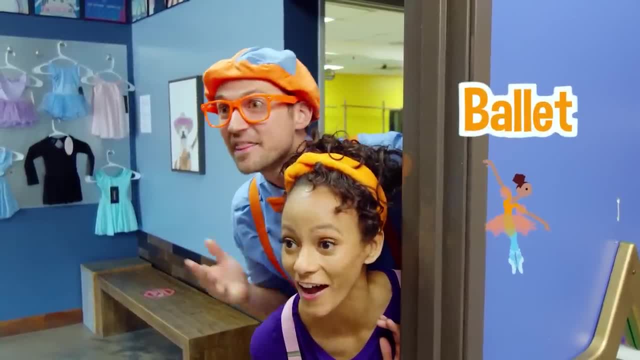 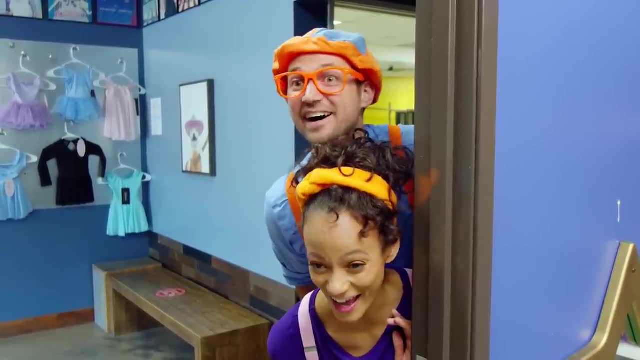 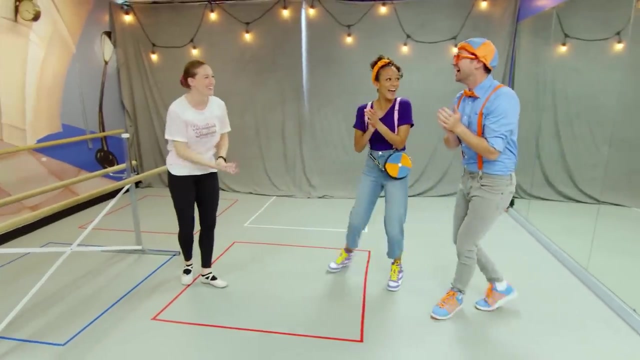 It's someone doing ballet. Yeah, That's what the music was: So pretty, She's really good. Yeah, very graceful. Yeah, Wow, Wow, Whoa, so good. Yeah, Wow, Thank you. Wow, Who are you? 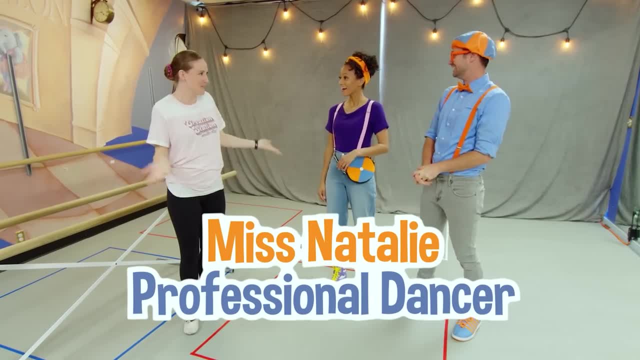 Hi, I'm Miss Natalie. It's nice to meet you guys. Who are you? Hi, I'm Mika And I'm Blippi, Hi, Blippi, Hi, Mika. It's nice to meet you guys, Yeah. 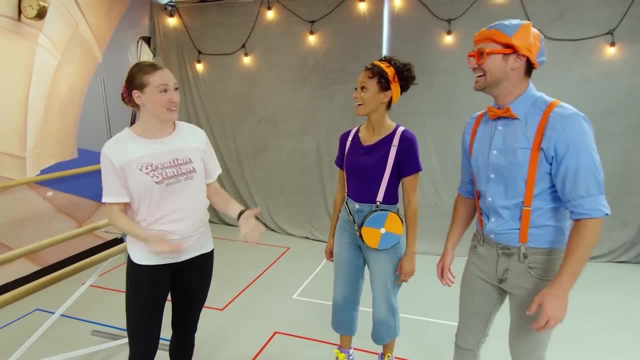 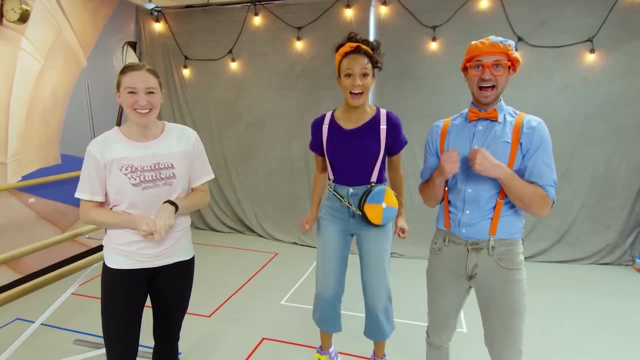 Nice to meet you. So are you a dancer? I am. I'm a real-life professional dancer and I was just doing some ballet. Wow, Would you guys like to learn some ballet with me? Yeah, Excellent, Come on over to the bar. 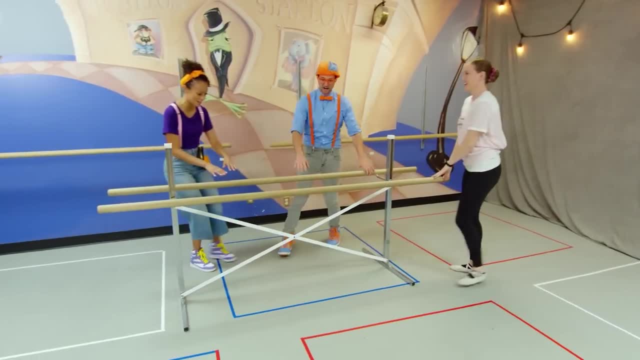 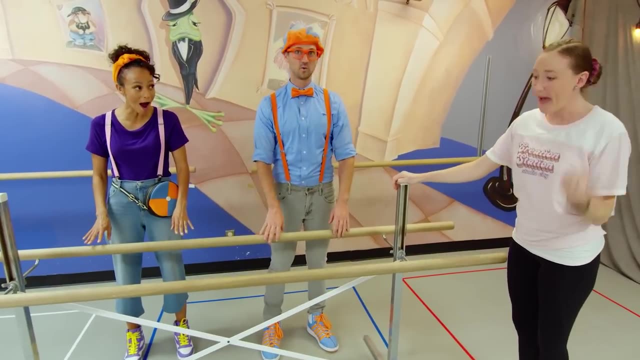 OK, We'll get you guys all set up. Whoa cool ballet. What is this? Thank you. This is our ballet bar. Our professional ballerinas learn balances and how to be more flexible, all with this bar. So the first thing a ballerina needs to know is first position. 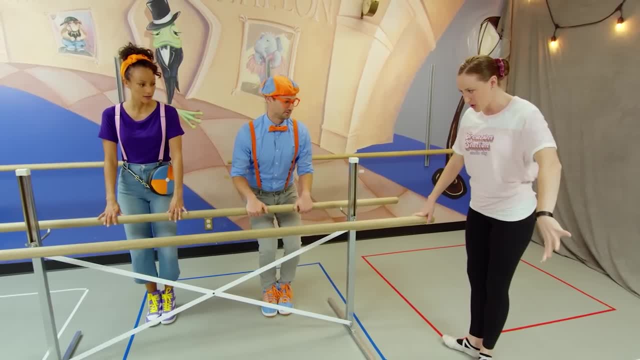 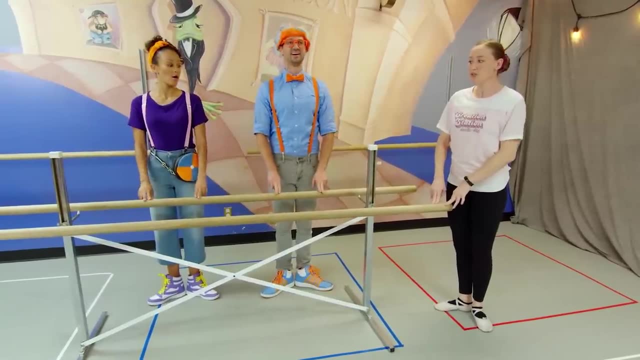 You're going to get those feet together nice and tight And just open up your toes like a piece of pizza Pizza, And then stand up super tall. yep, And I like to only put two fingers on the bar so we're not putting too much weight on it. 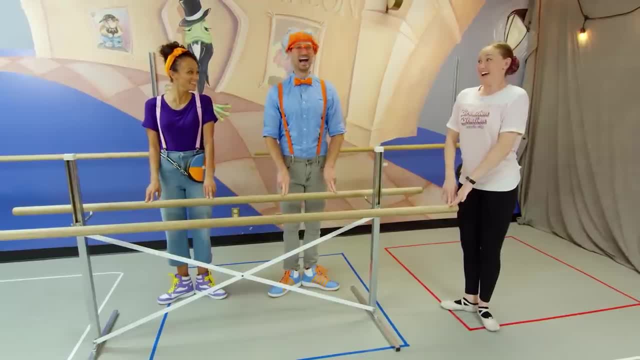 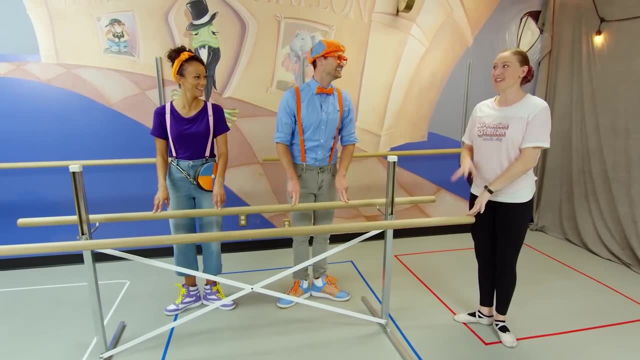 but just enough to stand super tall. OK, Yeah. So there's some ballet moves that we need to know because they're important, and then there are some that are just super fun. So we're going to start with one that's important. 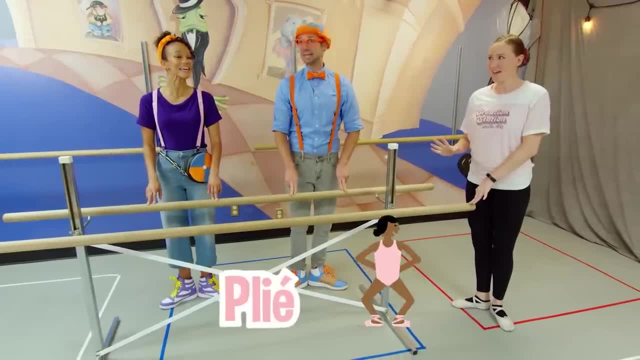 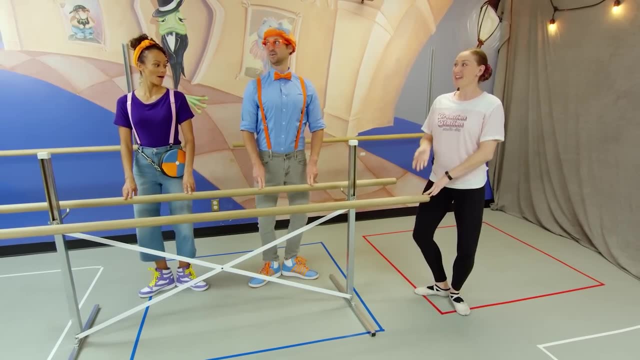 OK, Always use plie. Can you guys say plie, Plie, Excellent, We're just going to bend down, but keep tall, Yep, and then set it back up and then down, And I'll flip you like a real ballet dancer. 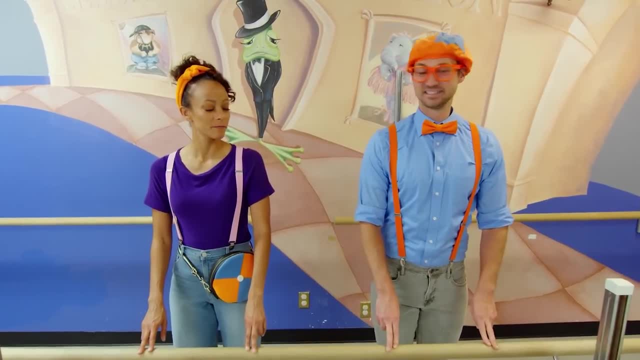 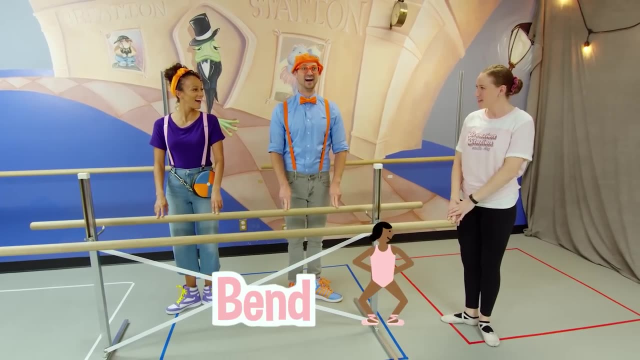 Yeah, Do you guys think you know what plie might mean? Our knees do it. when we do the plie, You're bending, Bending. Yes, that's so good. Plie means to bend. Oh, that makes sense. 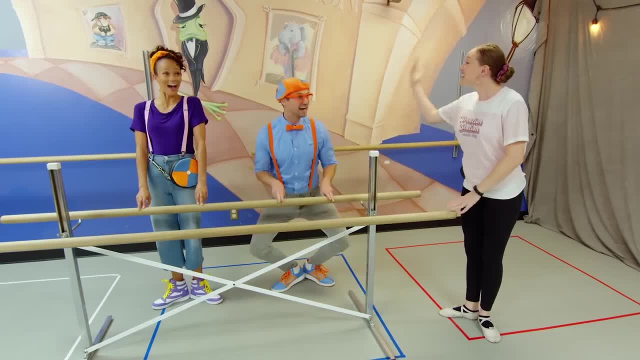 We kind of look like frogs, though. Yeah, Like we're about to jump in the air. Exactly, That's a plie move. Whoa, really. Yep, we're going to take that plie and we're going to jump straight up into the sky. 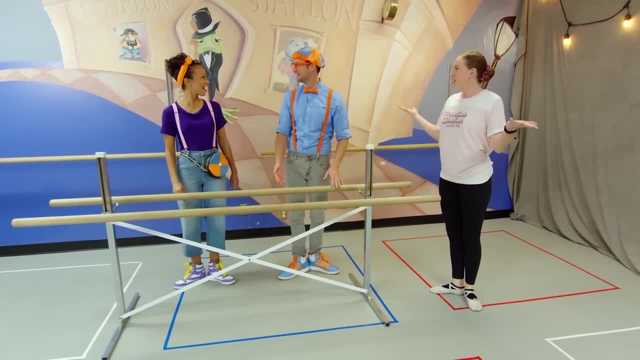 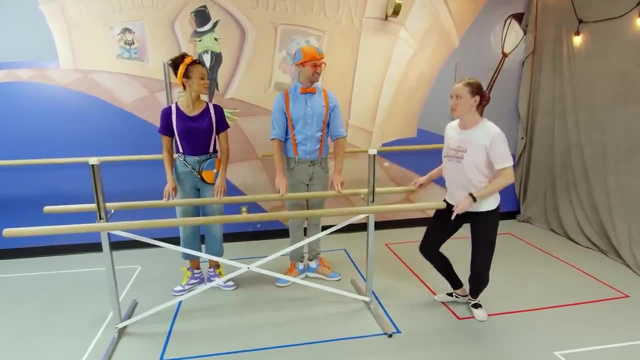 Wow, And land back in that first position. Whoa, Yep, and that move is called sauté. Can you guys say sauté, Sauté, Perfect, Sauté means to jump. You got it. You guys are so smart. 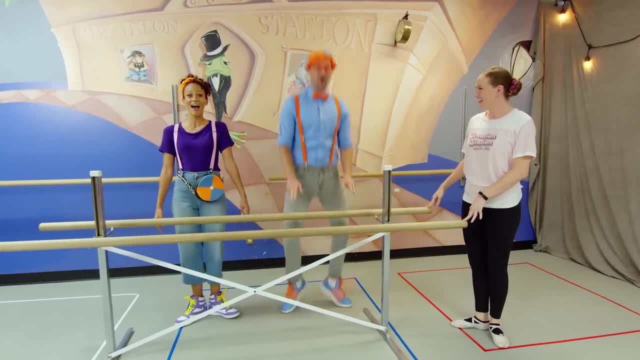 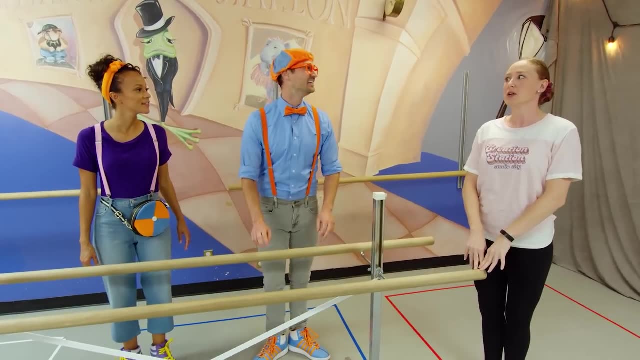 Whoa, That's so cool. Whoa, Whoa, Whoa, Woo-hoo, So good. OK, another important one now, So that one was super fun. Yeah, Another important one is passé, Passé, Passé. 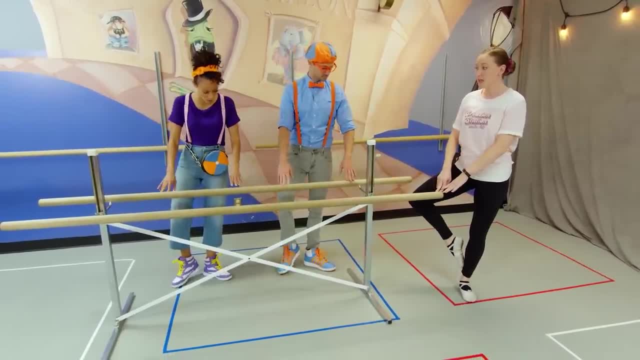 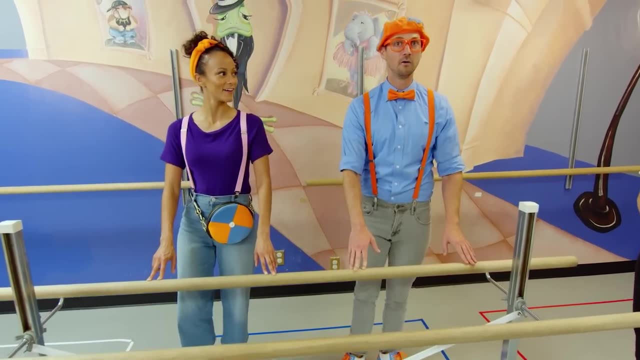 Passé. You're going to slide that toe up to your knee, finding your balance, keep that knee pushed back, stand super tall, and you're going to stand a little right back down. So it's kind of like an elevator ride. 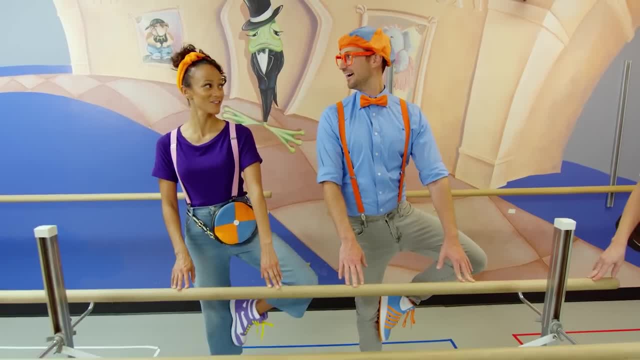 Your toe takes up the leg, Doo-doo-doo-doo-doo-doo-doo-doo-doo Going for a ride, And then back down to first position. Whoa, OK, Whoop, Whoop, Whoop. 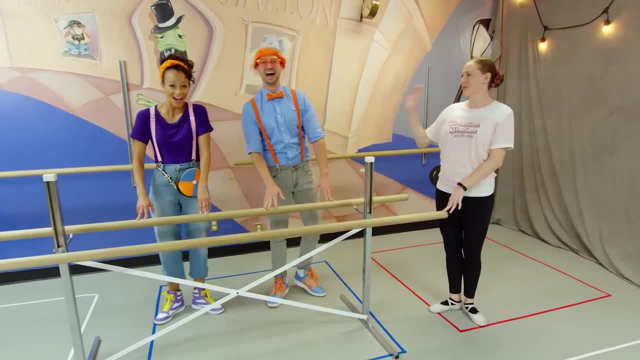 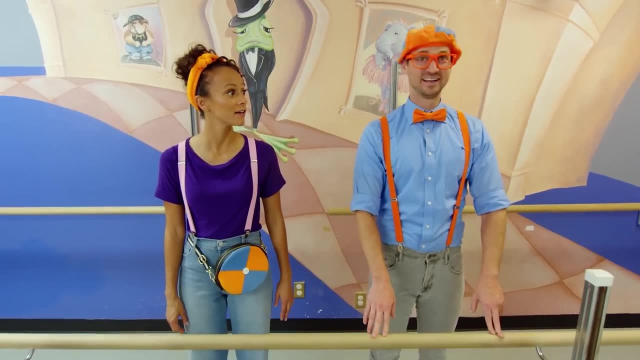 Whoop, Whoop, Excellent. Whoop, Whoop, Whoop, Whoop, Whoop. You guys are pro So good. Wow, That is really fun. One more at the bar, OK. Also super important, OK. 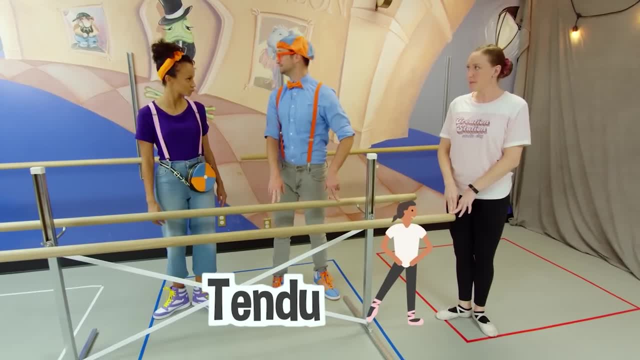 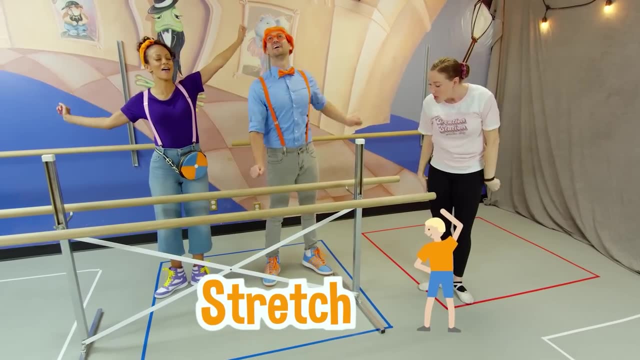 Tendu, Tendu, Yep. It's kind of like what you did next door. It's the first thing I do in the morning. It means to stretch. I love stretching And it's for our leg and our ankle. 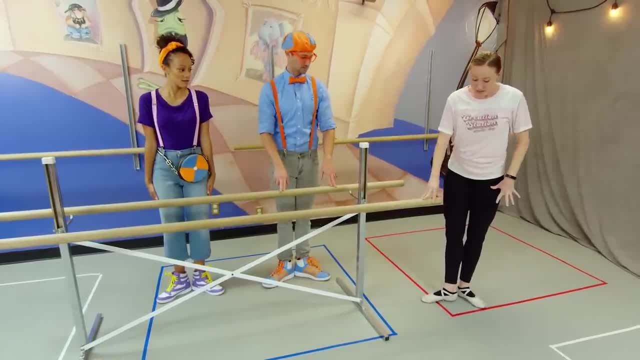 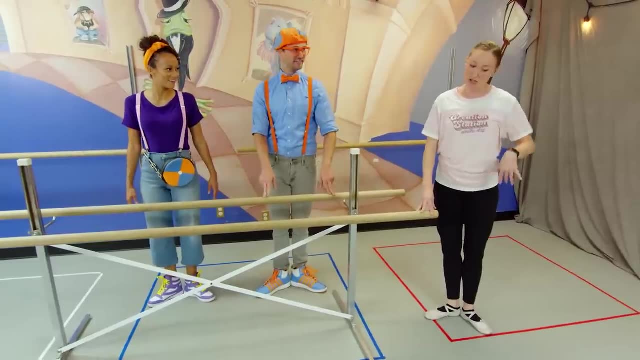 So you're going to stay in that first position And you're going to do your best to slide that toe forward. keep your toe on the floor and then slide it back- Perfect, Wow. And then use the other leg, Slide it forward as far as you can and stretch. 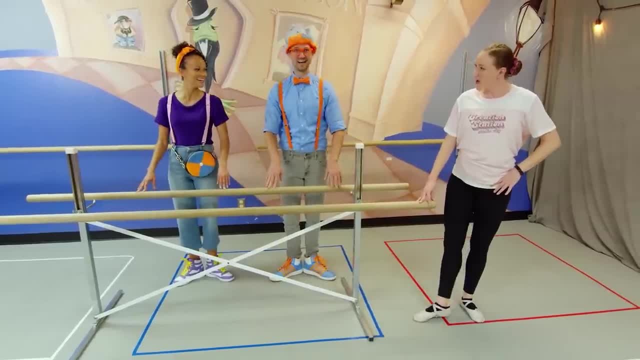 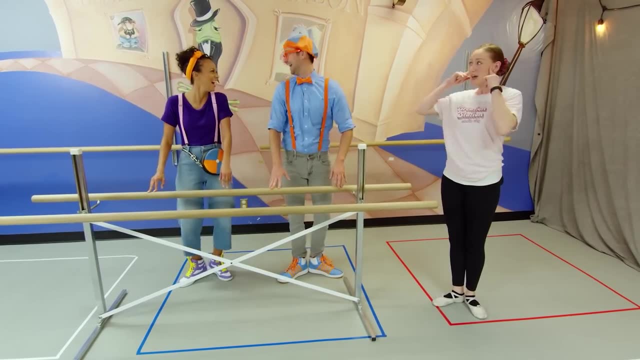 And then bring it back to first. Oh, that feels good. Yeah, it does. Tendu Doo Doo, Tendu Doo Doo. Excellent, Whoa. So that's to the front. 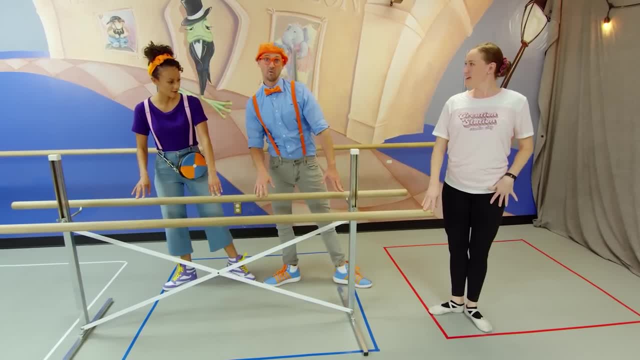 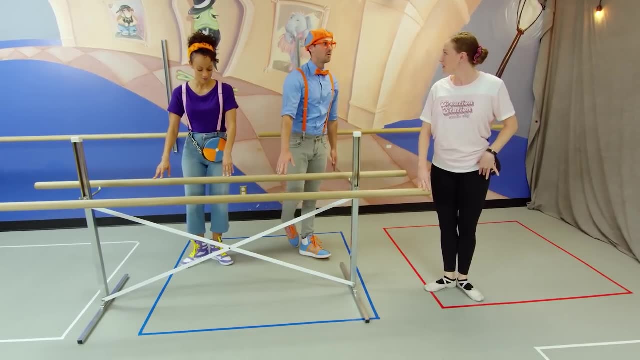 But you can also go side OK, Whoa, And to the other side, Whoa, And you can also go back, Ooh, Whoa, And then you can connect, And then you can connect all those tendus and make kind of like a circle around yourself. 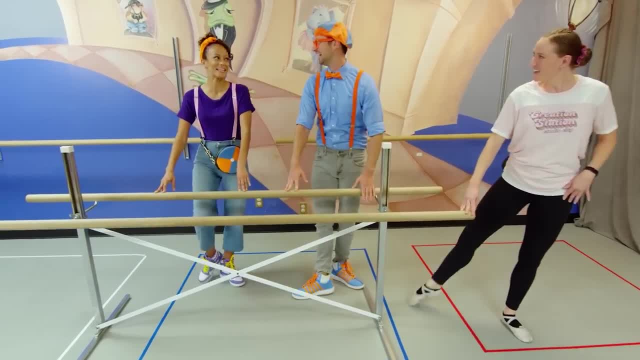 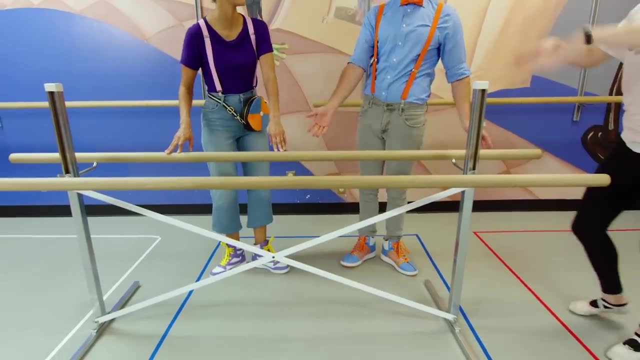 Wow, Oh, this is fun. Yeah, it kind of feels like skating. Yeah, Woo, We learned a lot of ballet already. Yeah, This is cool. So many words, huh. Now we're going to. if you can help me move this bar. 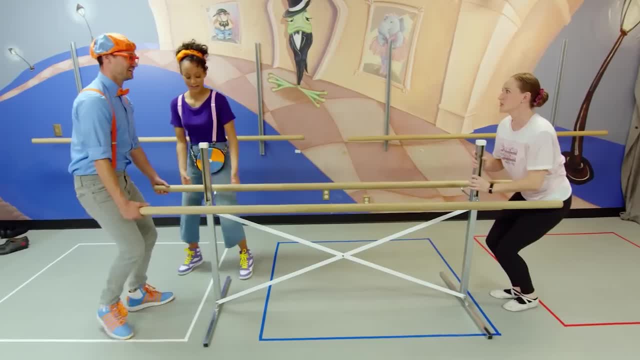 I'm going to teach you just like two or three more fun words, Oh, And then we can play some music. OK, Woo Woo, Woo, Woo Woo. Thank you. There we go. You got enough space there, Yep. 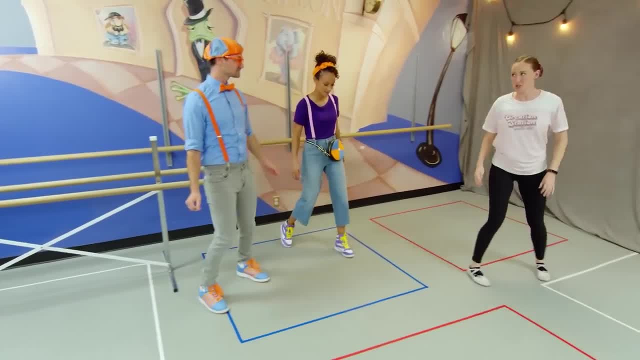 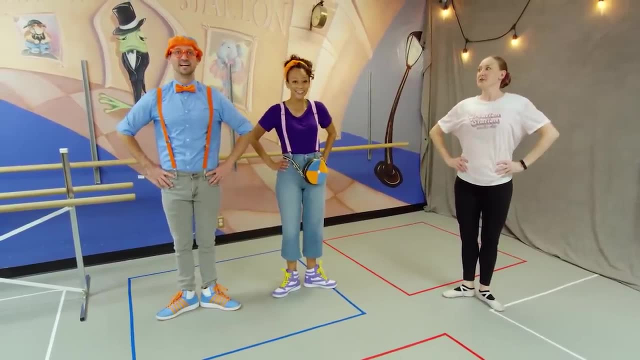 Perfect. OK, We're going to stay in that first position. OK, Feet are together, Toes are open. Let's push our hands on our hips. Yes, We remember: saute, Saute, Saute, Saute, Saute. 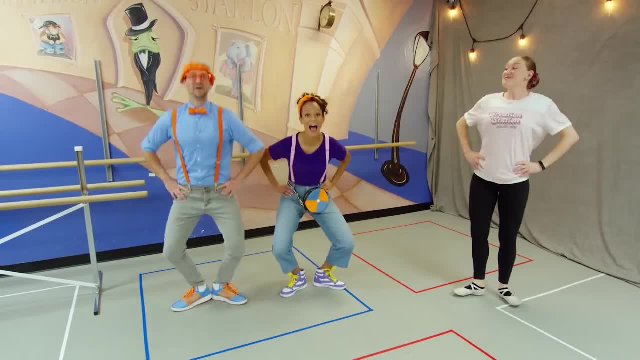 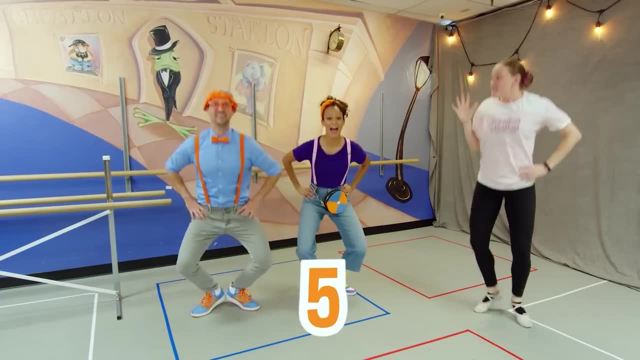 Saute Means to Jump, Jump, Jump, Excellent, Whoa. So we're going to do eight super quiet sautes Shh, Oh Ready. One, two, three, four, five, six, seven, eight. 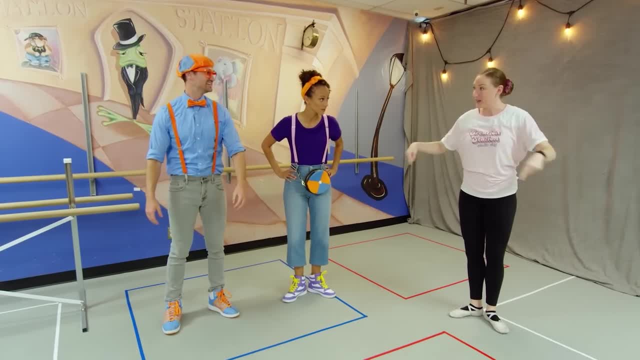 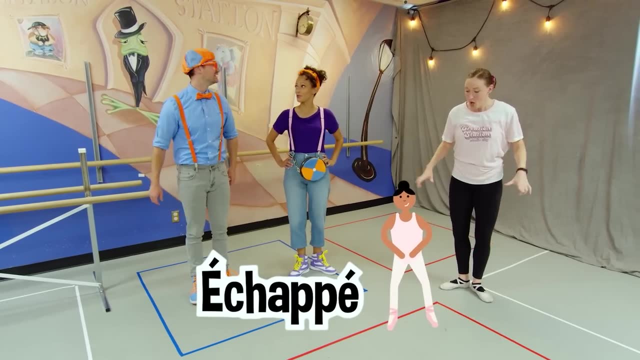 That was perfect. Now we're going to jump open and close. Whoa, Whoa. All right, This is called eight. All right, A chape, A chape. Lots of new words. Yeah, it is. It's kind of like a jumping jack, so it's super easy. 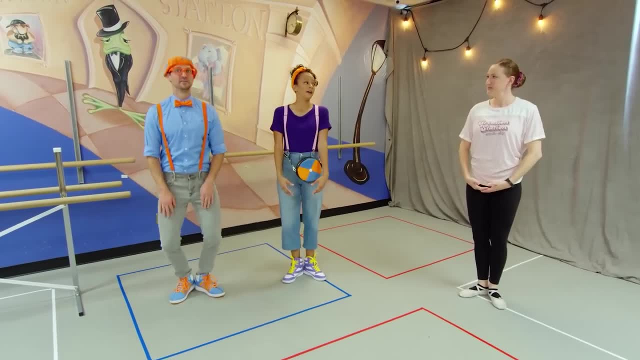 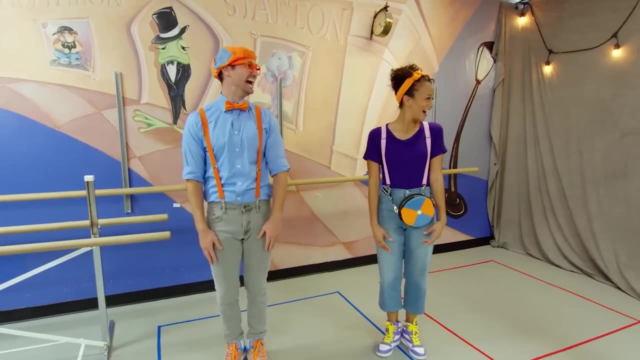 Just jump open, use that plie and then jump close. You got it. A chape, A chape, One more. A chape, A chape, Perfect. Yeah, Nice Whoa, We did it really good. 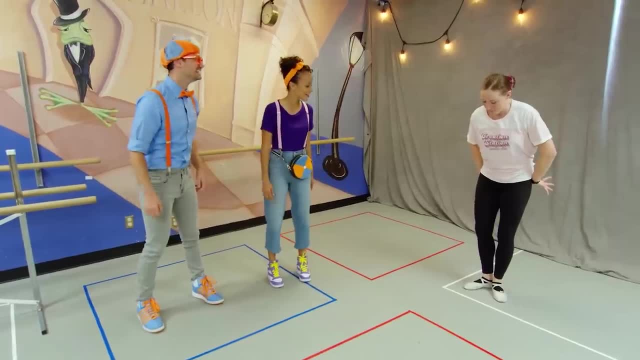 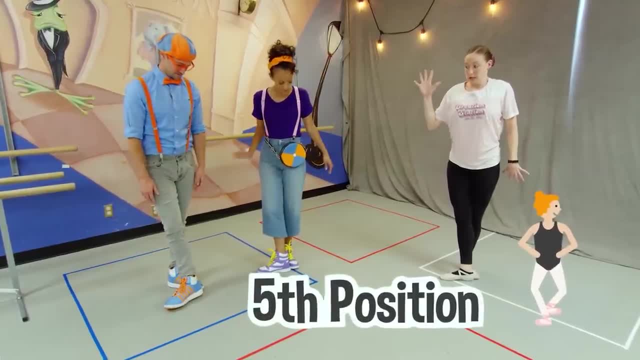 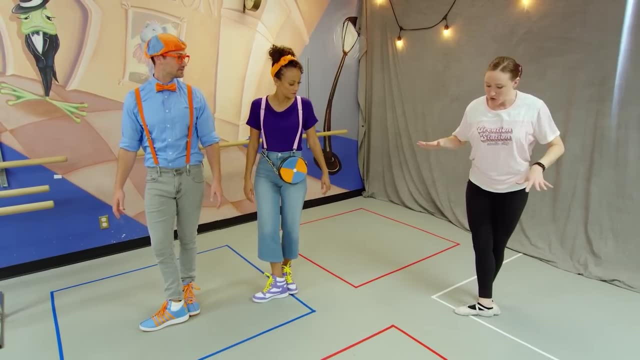 This is called fist position, Fit, Fit, OK, Yeah. So this jump, we call it shanjma And it means to change. So all you have to do is jump up in the air and land with your other foot in front. 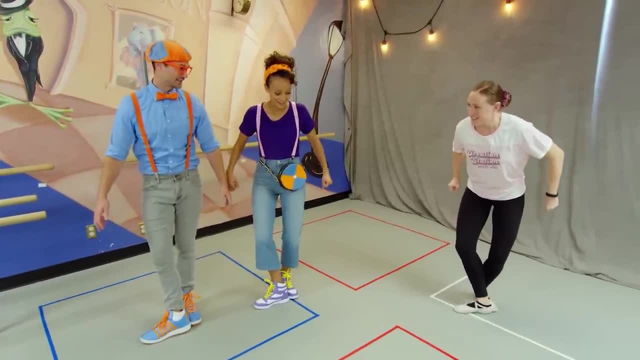 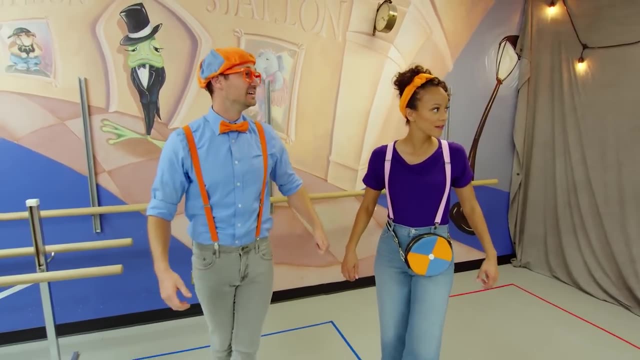 OK, Can you try? Yeah, Sounds tricky. One, two, three shanjma. You did it, Whoa. Yeah, That was perfect. Let's try to do three shanjmas in a row. All right, Ready. 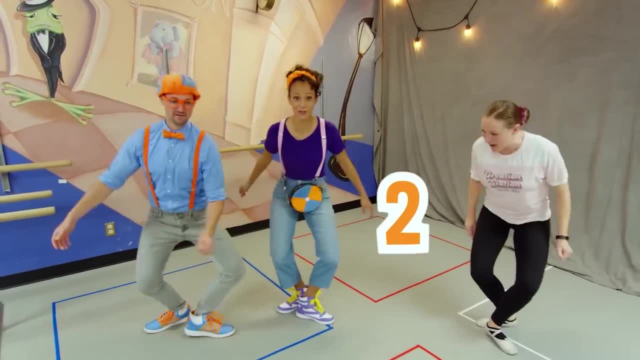 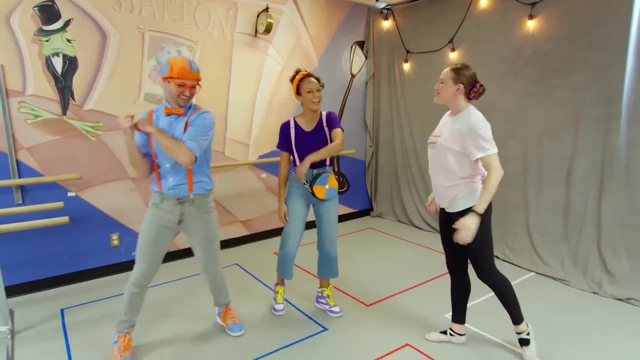 OK, Yep, Shanjma One, two, shanjma Three, Whoa Perfect, You did it. Yeah, Yeah, Good job, Good job, Good job. That was awesome. I'm so proud of you guys. 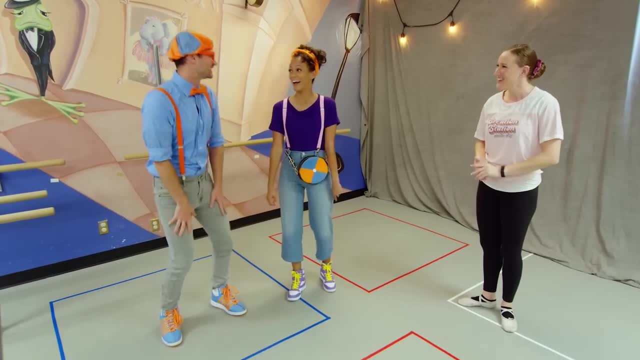 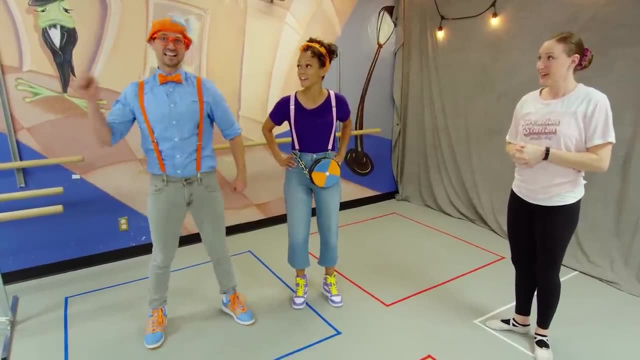 You learned so much. Yeah, Thank you so much for teaching us. You're welcome. I don't know, Do we want to put it to music? Yeah, That sounds fun. Yeah, All right, Let's hit that music, All right. 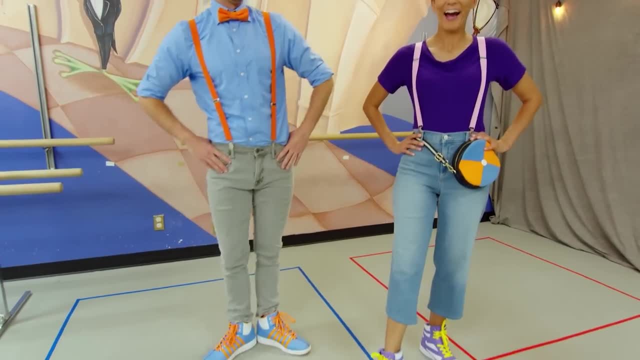 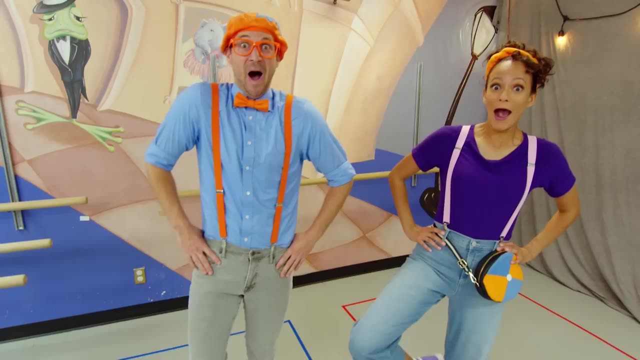 Let's do this. No, All right, I'm going to do it, All right. Ok, Now who's doing the best shanjma so far? Let's do the best shanjma I could. I wish you high scores or low scores. 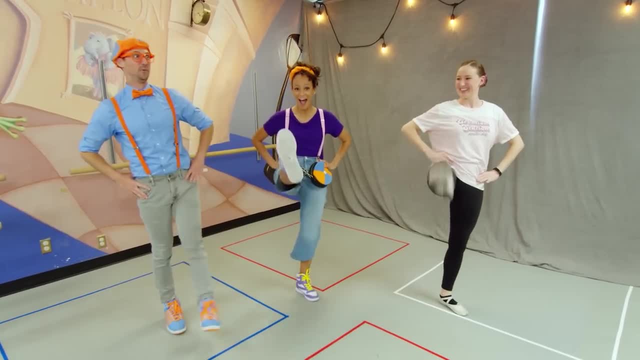 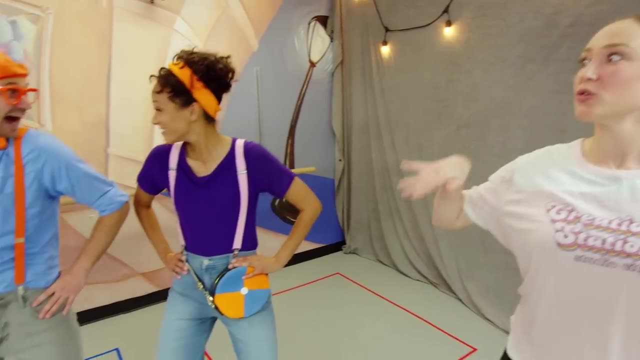 By the way, the ones who did best. shanjmas, Who strong you were. Some of us are comme these right here And I'm really proud to be. Good luck this year. It was a great show. Draw some text. I strands. 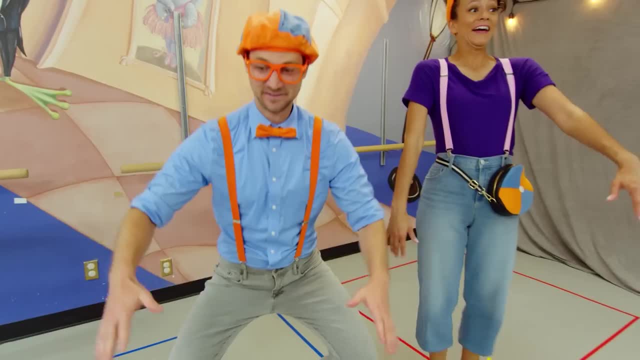 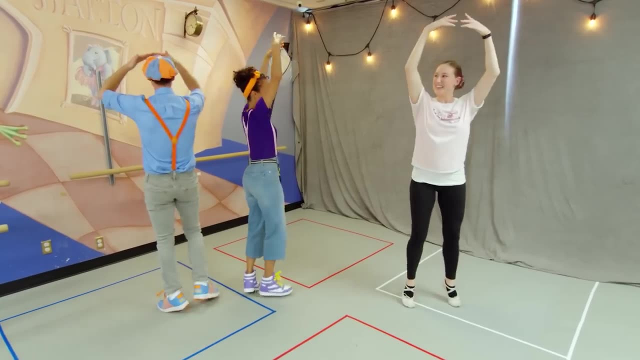 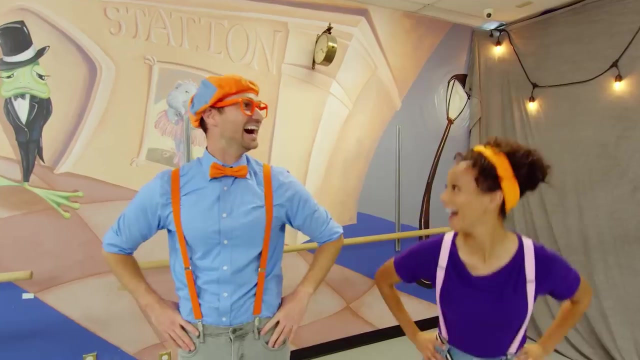 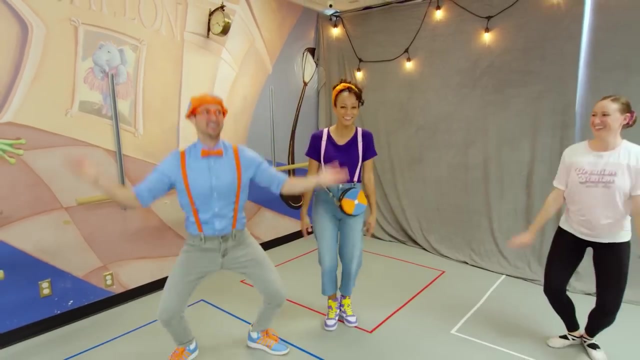 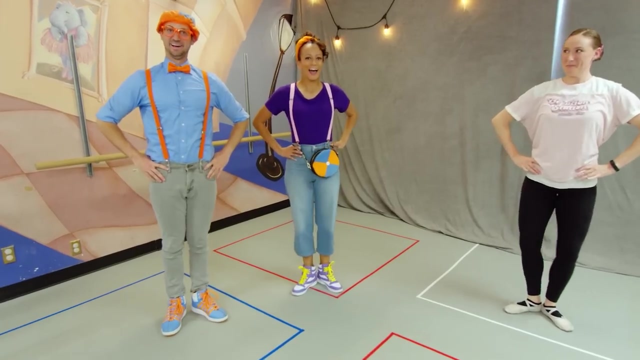 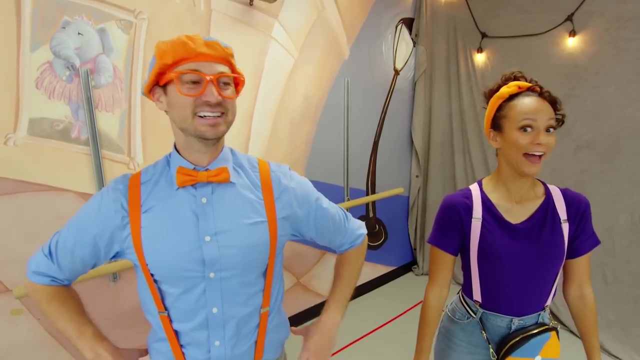 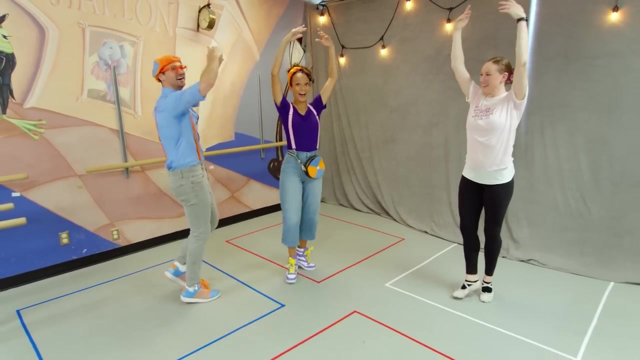 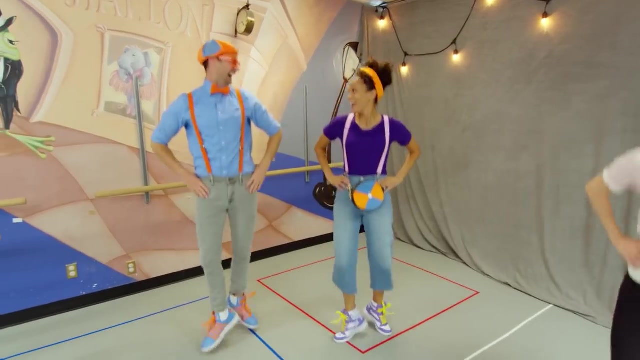 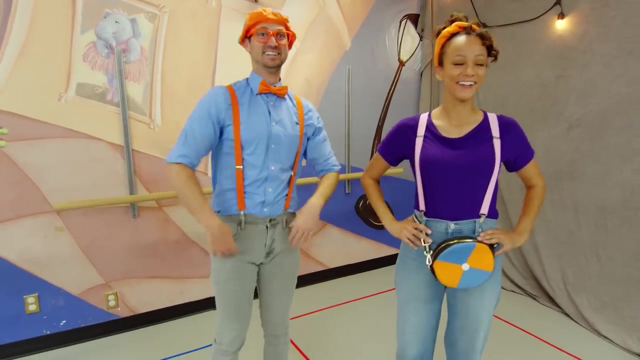 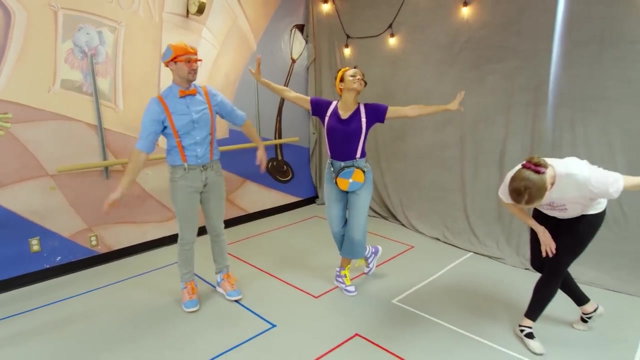 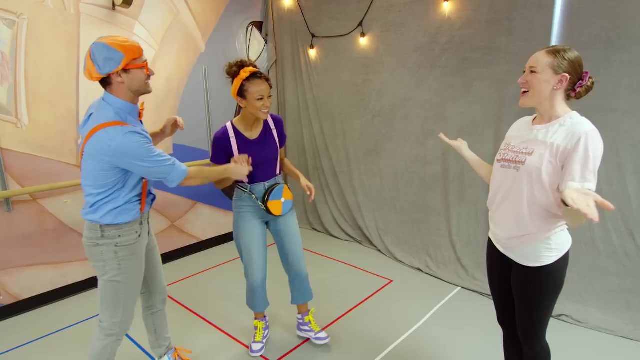 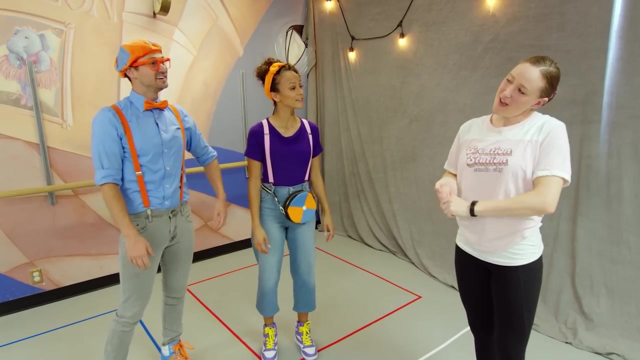 You Draw some text. Thank you, Thank you. Thank you so much for teaching us. You're so welcome. You know, I teach another style of dance too, if you guys want to learn it. Yeah, what kind of style is it? 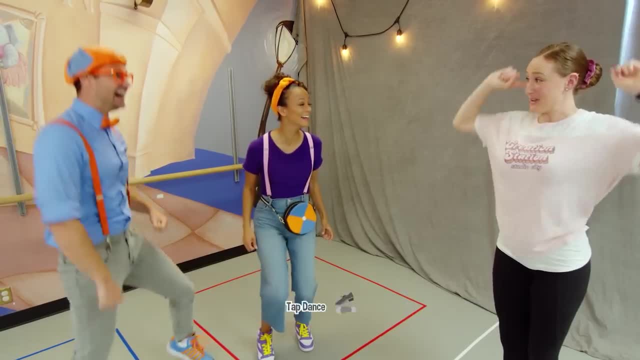 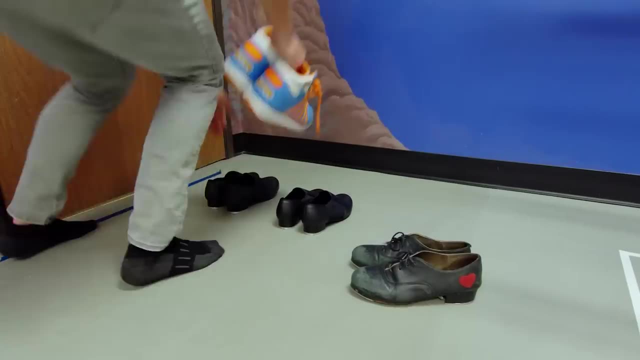 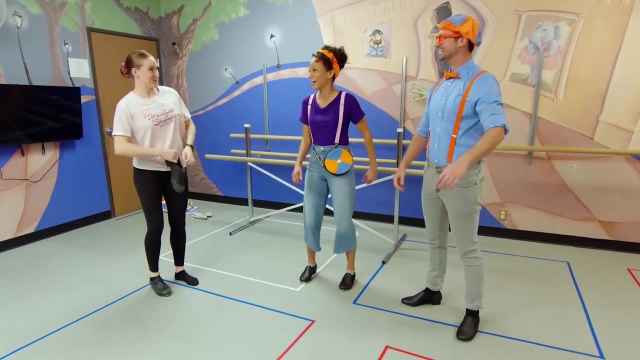 Task dance. Yeah, That means we have to try it again. We're going to change our shoes and then we'll come right back. All right, let's go. Wow, Wow. You guys put your shoes on super fast. You're so excited. 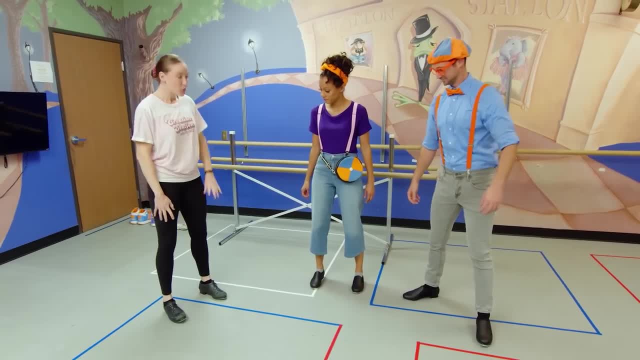 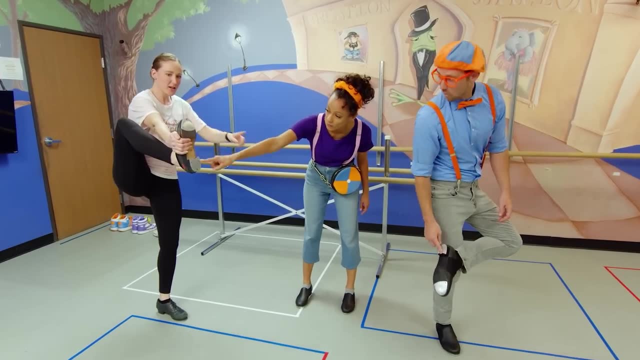 You did too. Thank you, Okay. two important things to know about our tap shoes before we start. The tap shoe has two metal shiny parts, right? Wow, they do. Okay, we have to learn what they're called Okay. 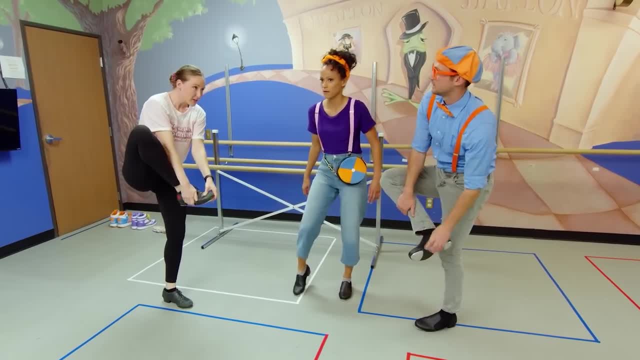 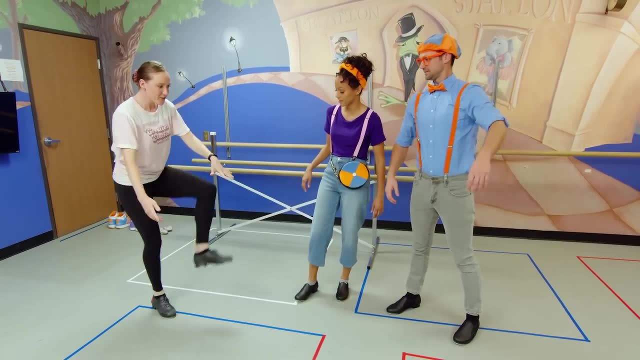 So up here, I mean, what's in that part of your tap shoe? Are your fingers in there? No, No, it's your toes. So we're going to call this the toe. Okay, Okay, Okay. The other part is called the. 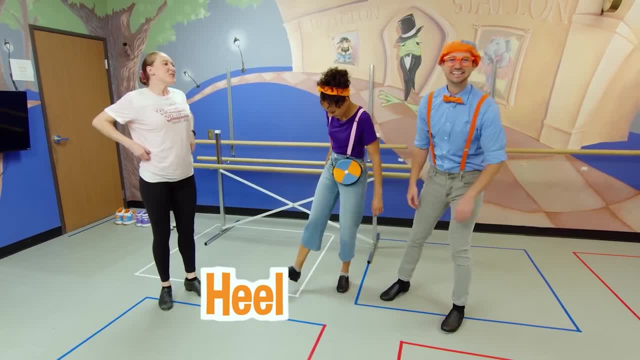 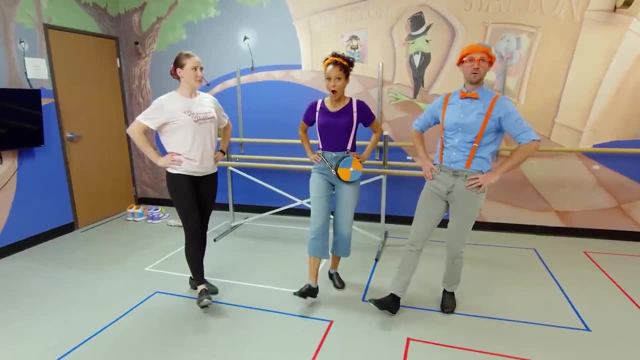 Heel, The heel, Exactly right. So the first few things we learn are going to be super easy-peasy: Put that leg out, Don't let it move. But you got to tap your toe. Ooh, I love that sound. 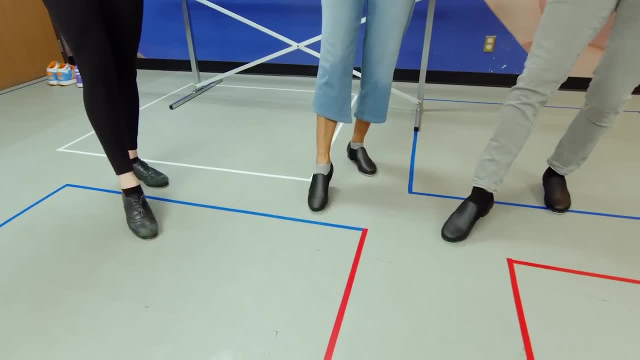 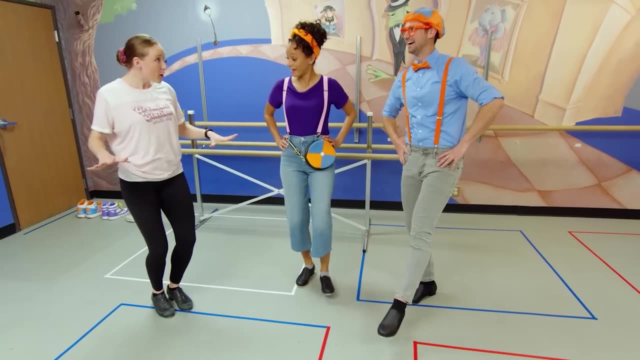 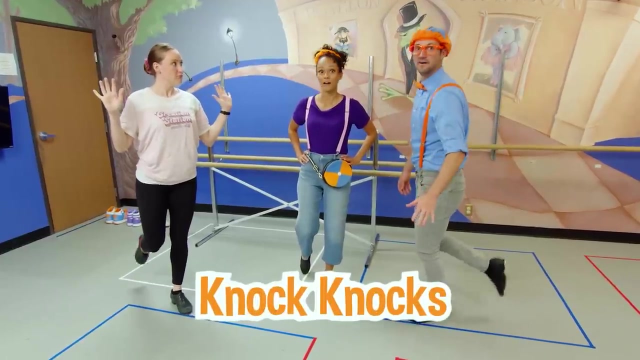 Excellent, Good, Can we try the other foot? Perfect, Now we're going to use the same part of your shoe, but you're going to put it behind you. Oh, Uh-huh, It's called knock-knocks. Yeah, like knocking on a door. 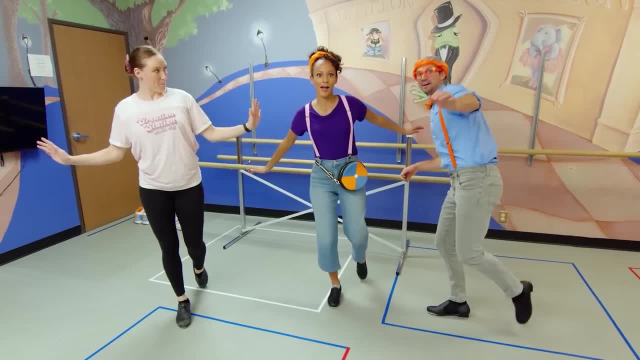 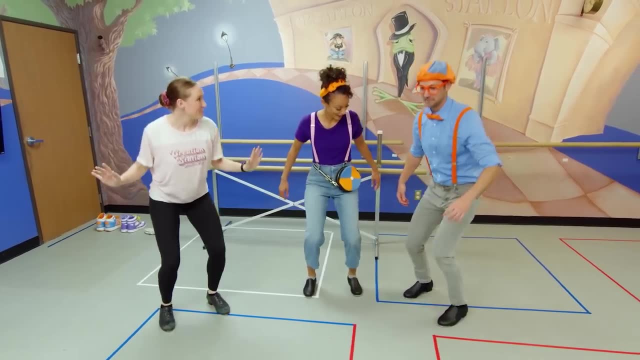 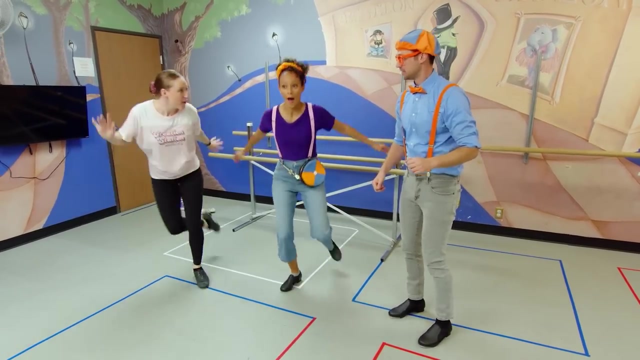 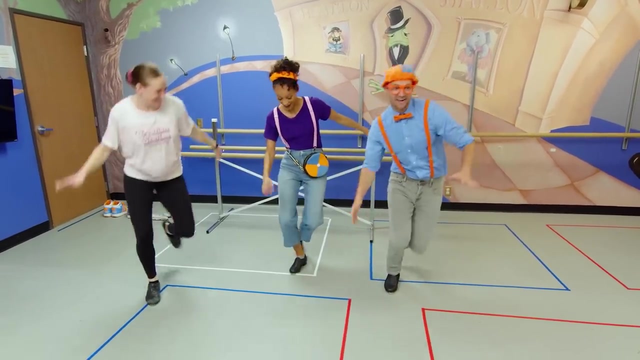 Let's try the other foot: Knock, knock, knock, Knock, knock, knock. Excellent. Now with the knock-knocks you can switch. Hey, Nice, Then you can jump. Excellent, Very good, Nice, Blippi. 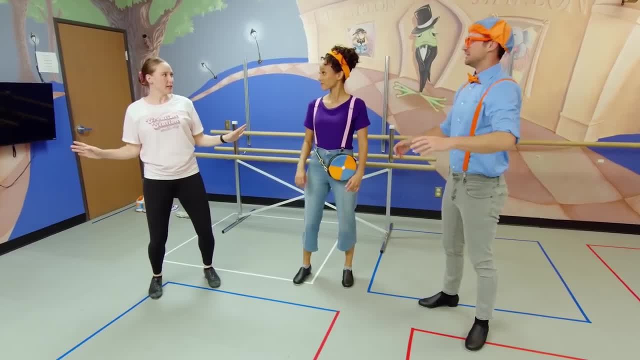 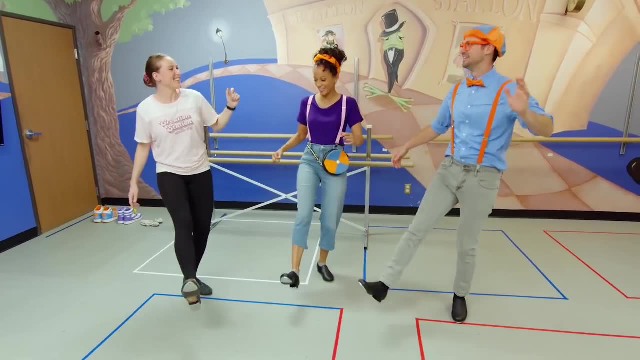 You too, Mika. Good, Now let's switch and use our heels. Okay, Put it out in the front seat And dig, dig, dig, Dig, dig, dig. Excellent, Very good, Let's try the other foot. 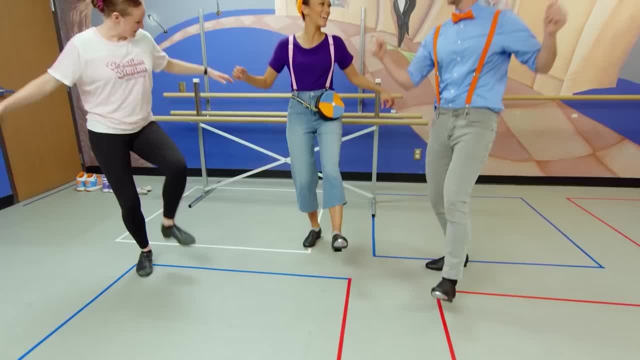 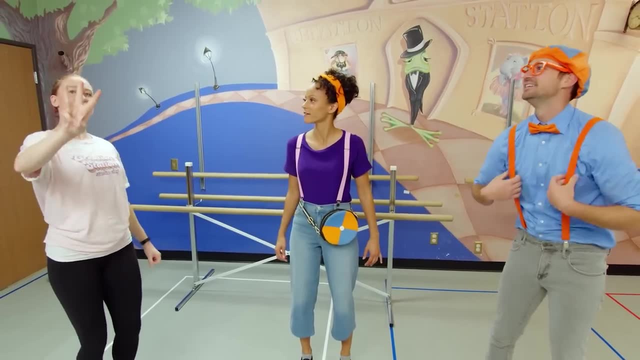 Dig, dig, dig, Dig, dig, dig. You got it, you guys, So easy. The next one is going to be a shuffle. Ooh, Can we say shuffle step, Shuffle step? How many sounds do you think a shuffle step is? 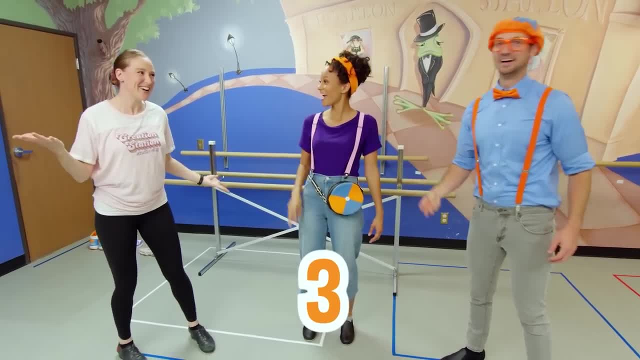 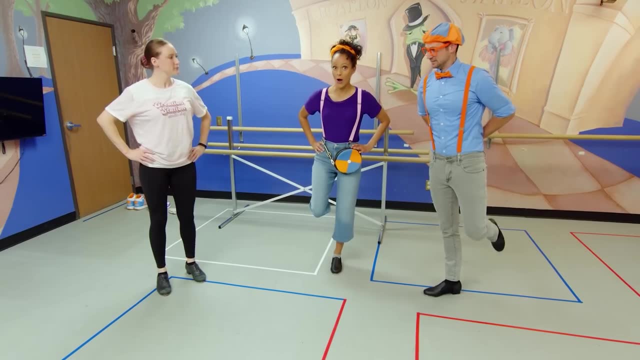 Shuffle, step Three, Three sounds. You got it. So we're going to start kind of like a flamingo bird. Ooh, find the balance And we sweep the floor, Sweep the floor, Sweep the floor, Perfect. Now, what's important with the shuffles is that our heels don't touch. 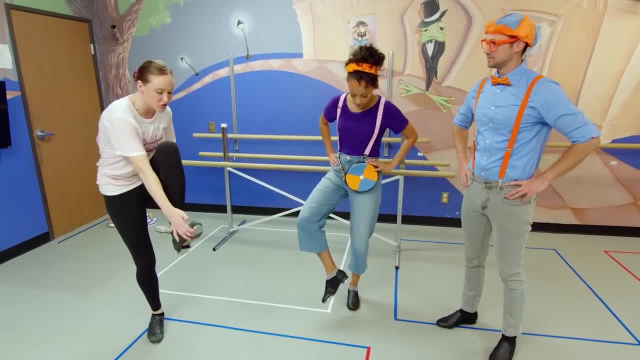 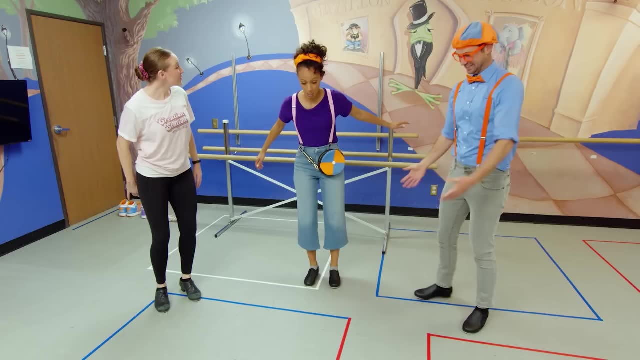 It's just for the toes, So keep your heel off, just your toe Shuffle. Yeah, Mika, That was very good. Okay, I'll try. Shuffle floor. Holy cow, That was perfect. Good job, You're a top dancer. 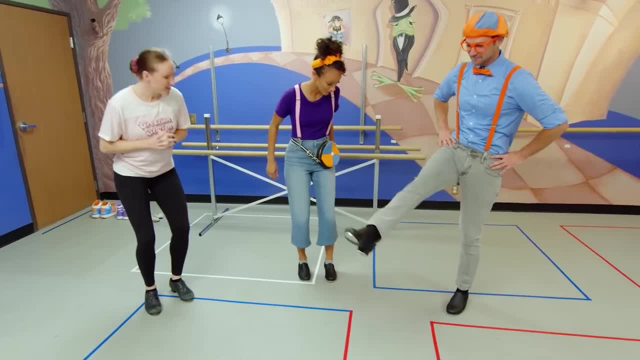 Yeah, I am. Okay, we're going to learn an even harder one. Okay, This one is a paradiddle. Whoa, This one is a paradiddle. Whoa, This one is a paradiddle. This one is a paradiddle. 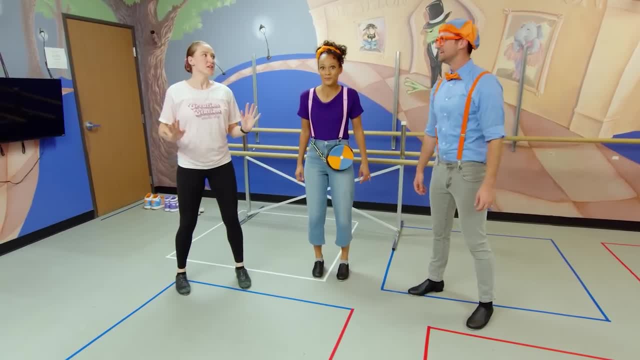 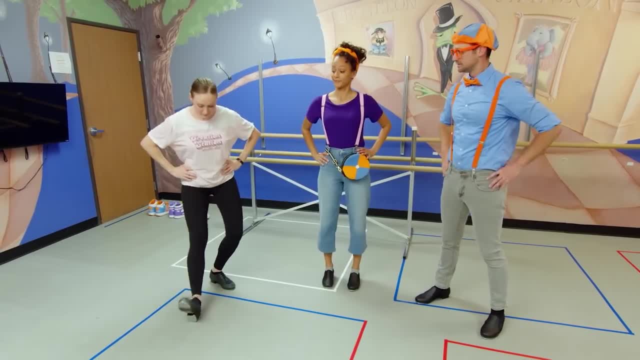 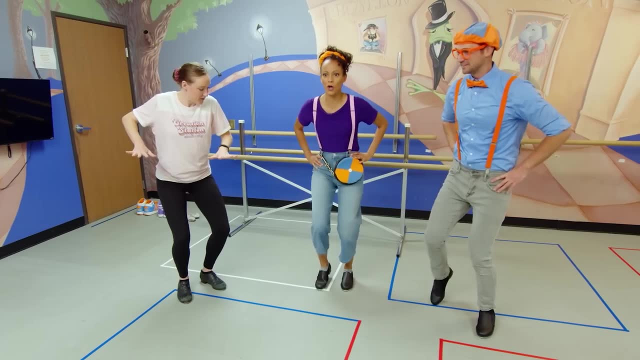 You got it And then set it down: Toe heel, Toe heel. Yeah, you got it. Let's try the other leg, Dig Spank Toe Heel. All right, Can we do it all together? Yeah? 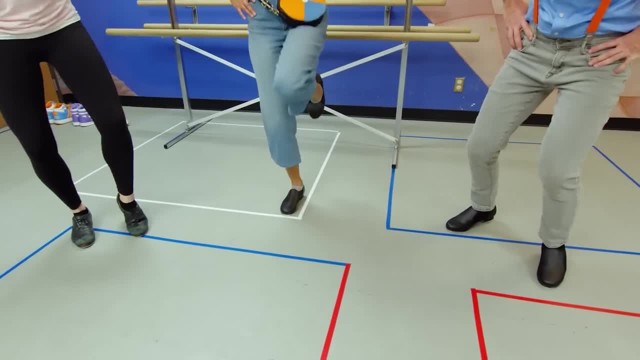 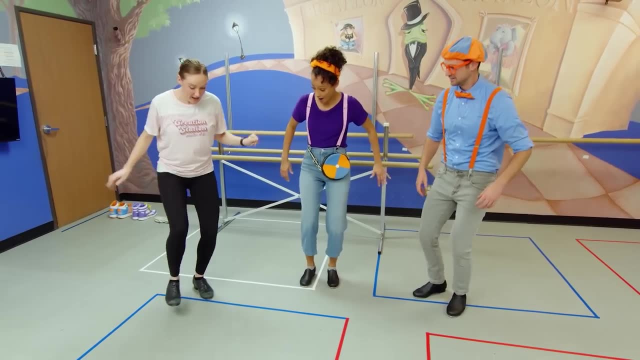 Okay, Five, six, seven, eight, One, two, three, four, Perfect, Perfect, Perfect, Perfect, Perfect, Perfect, Perfect. Now do a half spin and big spank Toe heel Dig, Spank Yeah. 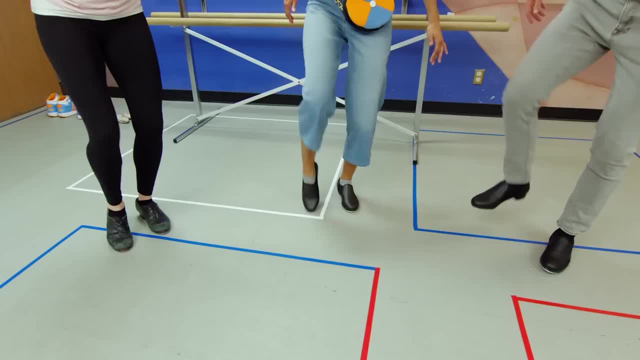 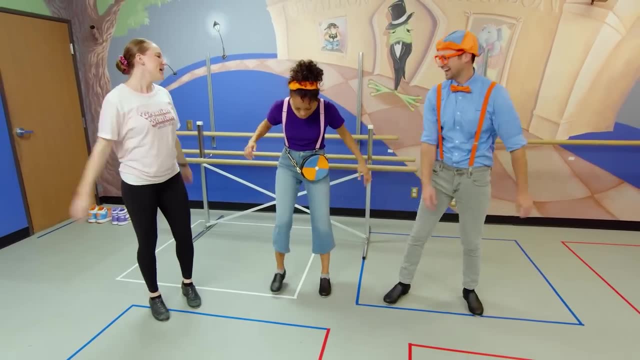 One more. You got it. Other foot Dig Spank Toe heel. I messed up. That's okay. Messing up is totally fine as long as you're having fun. Yeah, and I sure am having fun. Yeah, me too. 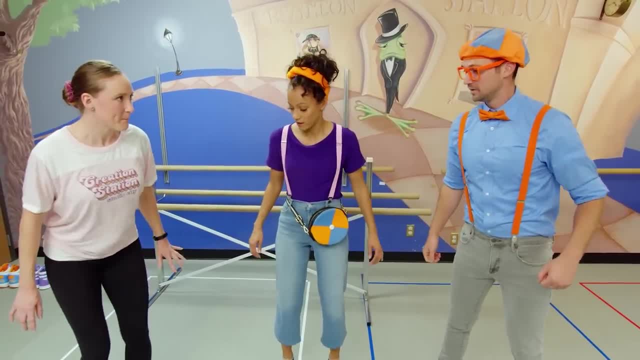 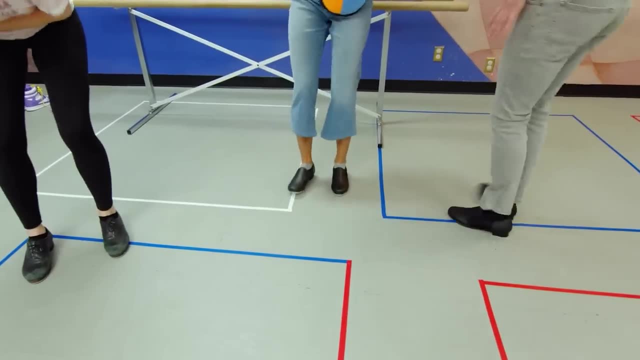 Yeah, Perfect, Let's learn a fun one. All right, Get those feet moving as fast as you can, And then it goes in a circle. Whoa, Okay, Excellent, fast feet. And then one more favorite move of mine is called: 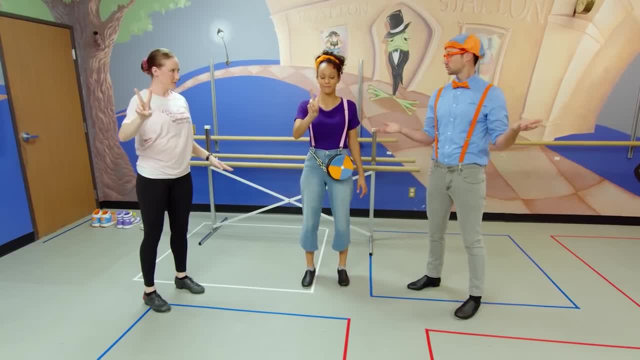 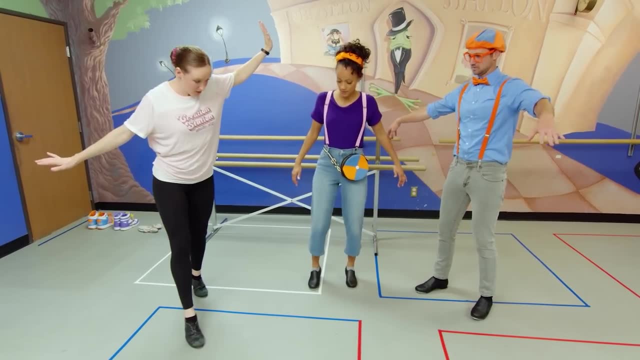 fa-lap, fa-lap, fa-lap. Two, two steps And, like I said, with the shuffles, you gotta try to stay on your toes and you're gonna kick a ball forward and then step on it. Yeah, that was pretty darn good. 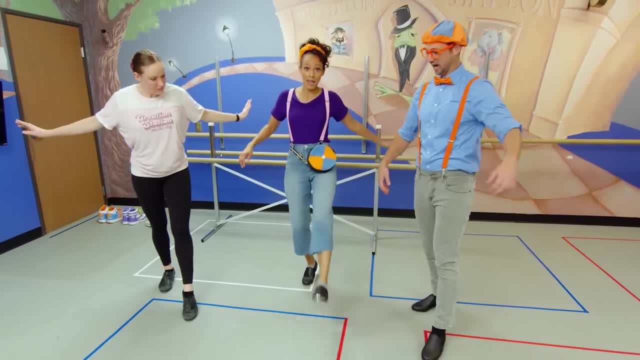 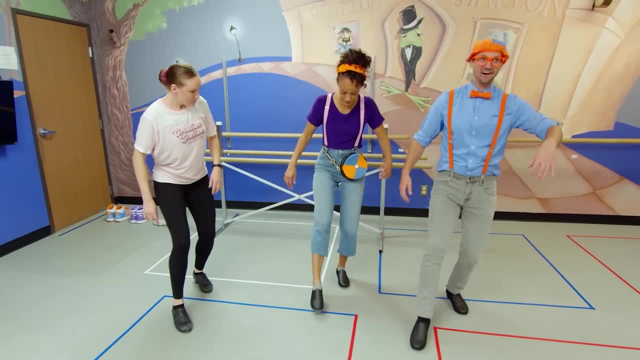 Can you try the other foot: Fa-lap, fa-lap. I know this word's a little sticky, Yeah, Fa-lap. So think about down: Fa-lap, fa-lap, fa-lap. There you go. 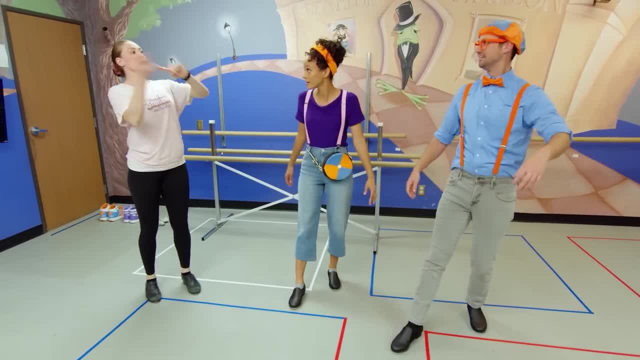 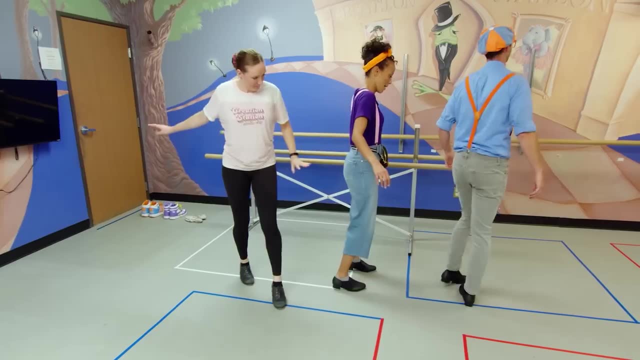 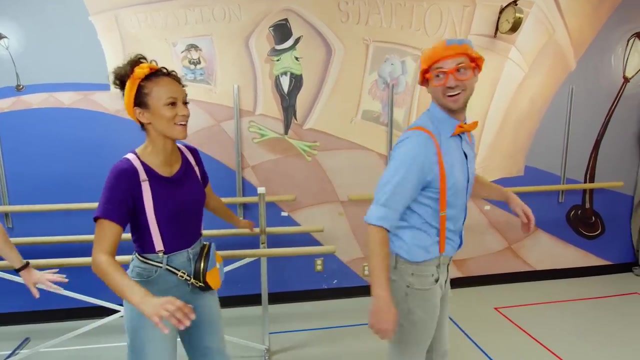 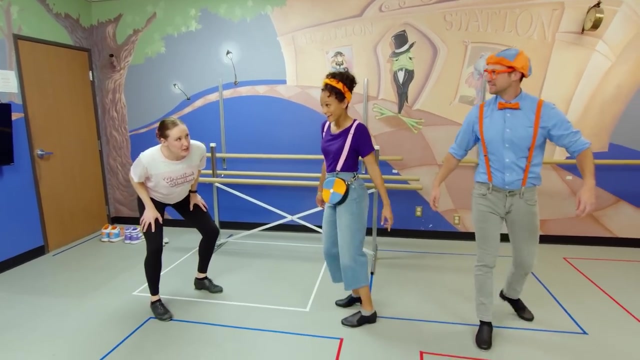 You got it, And this is a moving step, so you can walk around a circle doing fa-laps. Whoa, There you go. It's hard. I like how it sounds. Yeah, Whoa, Very good, Excellent. and then another easy peasy, moving one. 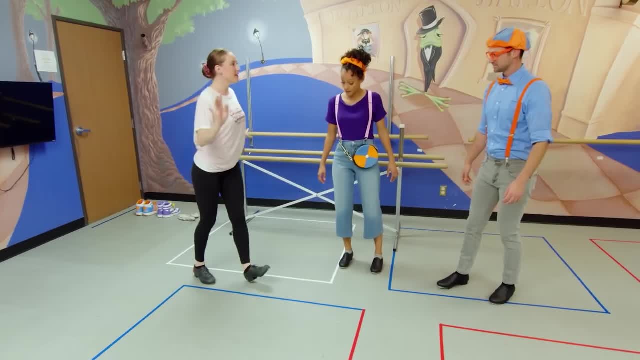 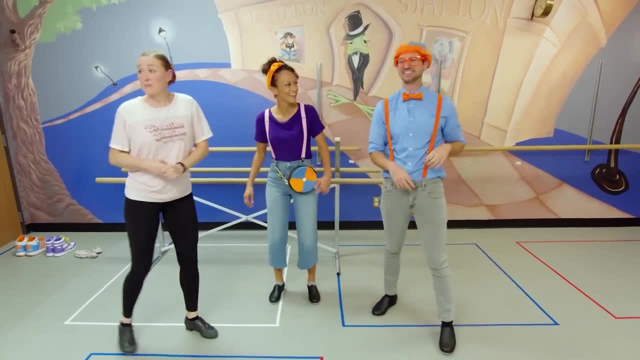 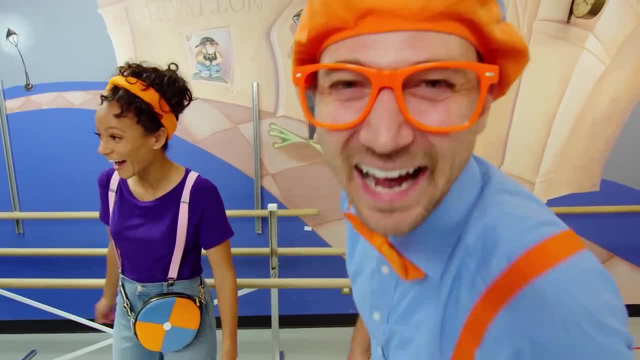 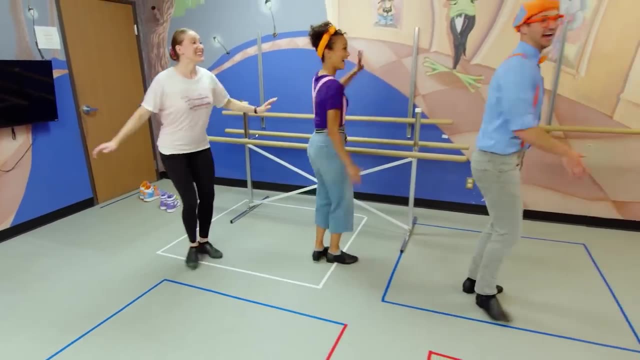 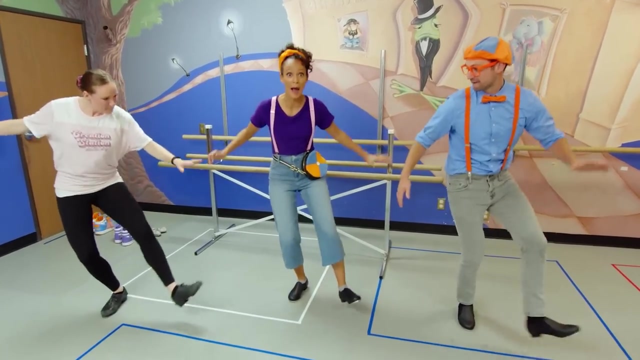 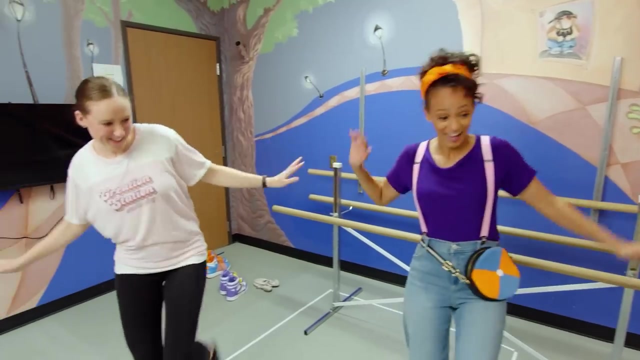 All right, let's get some music going. Okay, All right. So thank you for joining us for this session and I look forward to seeing what you all will be doing for your coming up next week. Sound good, Sound good. See you guys. 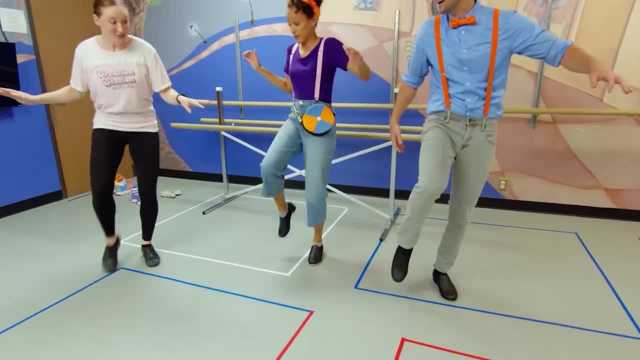 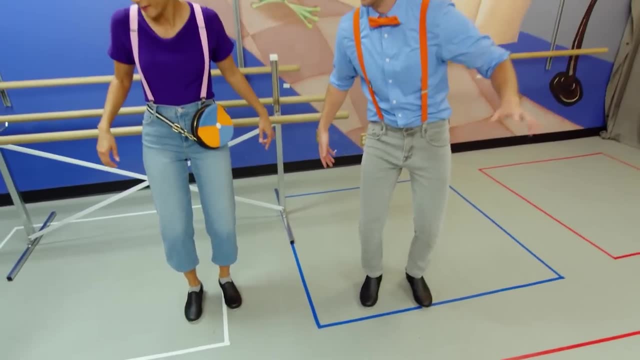 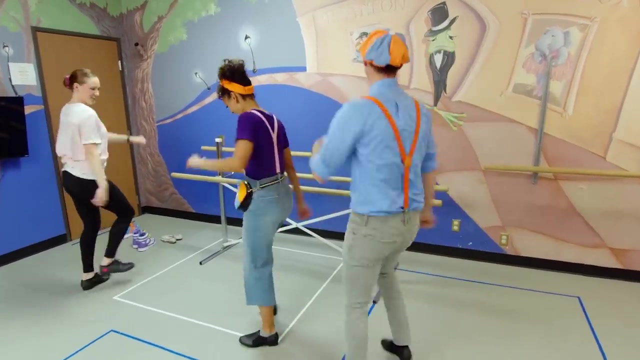 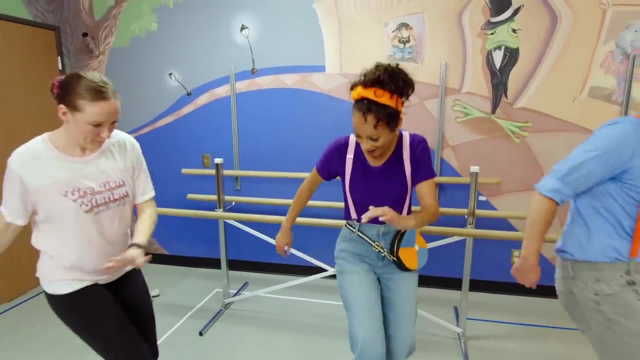 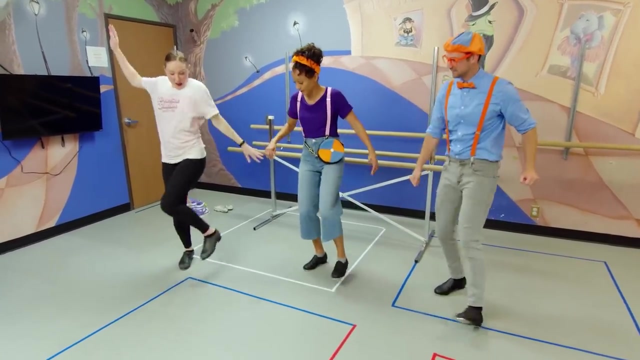 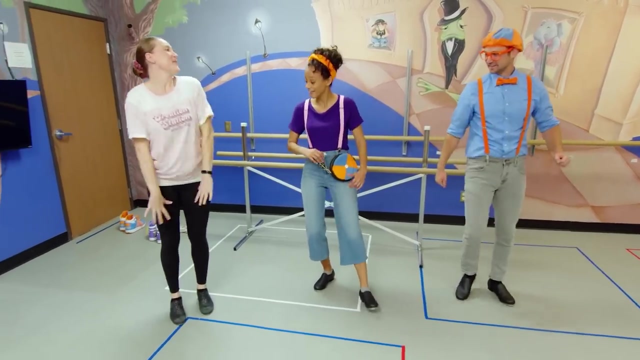 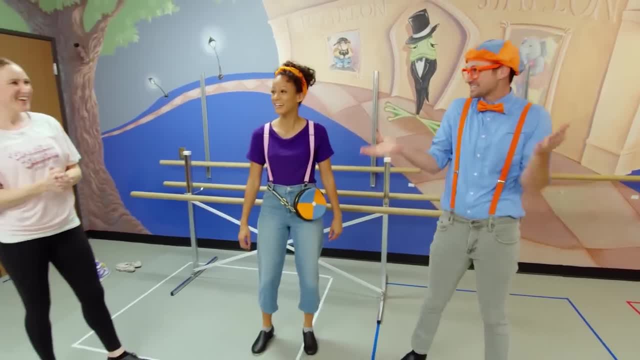 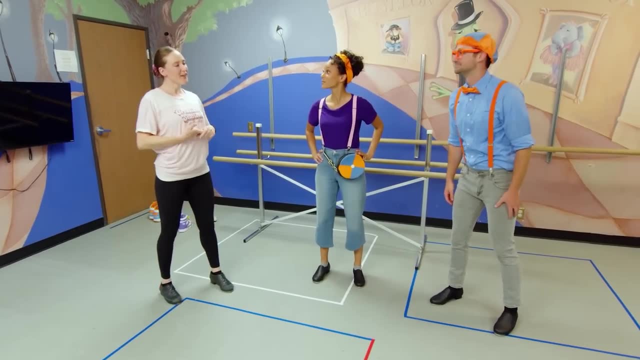 That was excellent, you guys. Thanks for teaching us how to tap dance. You're welcome. Excellent memories too, Thank you. you're a great teacher, Thank you. You know, I have another teacher here who teaches another style of dance. 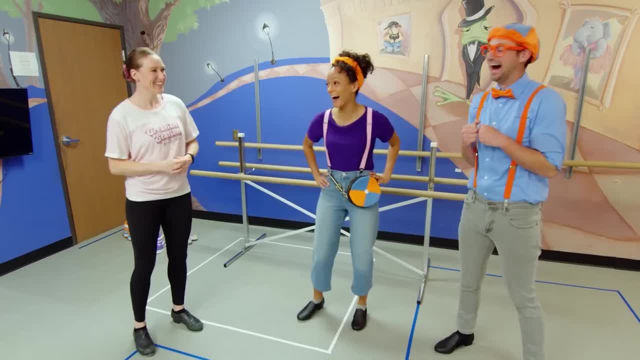 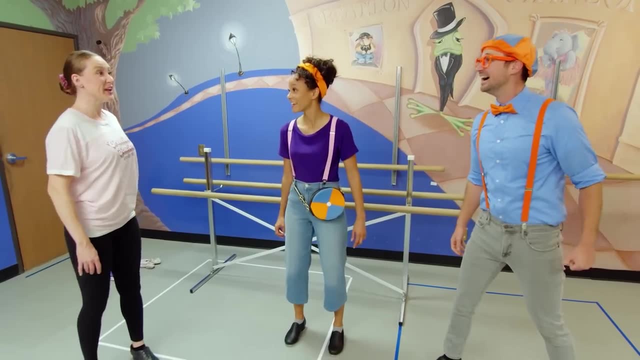 if you are up to learning one more style. Yeah, He teaches hip-hop. Hip-hop sounds really cool. Yeah, it does. His name is Mr Kaden and he's just down the hall Here. follow me. Okay, we're gonna get our shoes first, though. 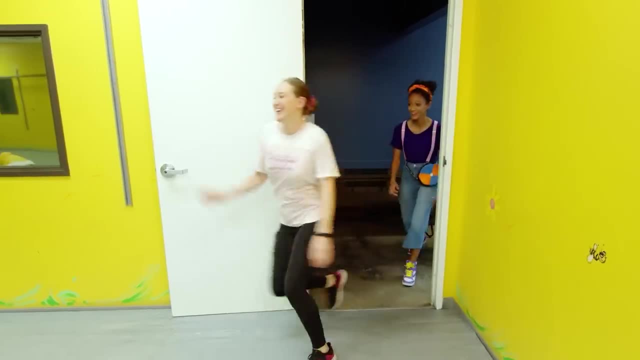 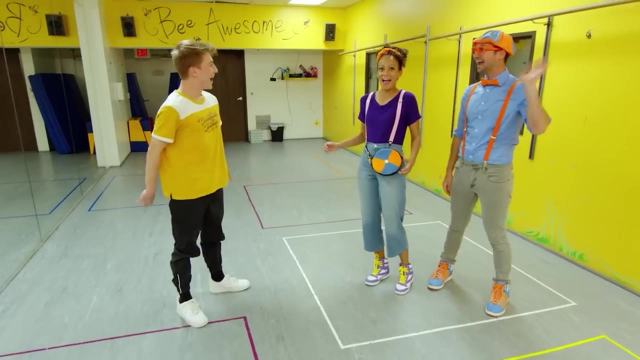 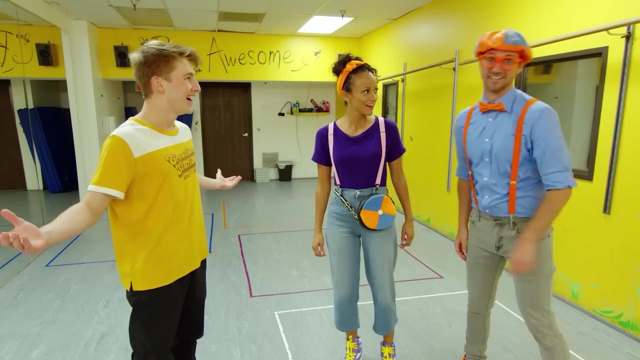 All right, Yeah, Ooh, Wow, Whoa Cool. Hi friends, Hey, I'm Mika And I'm Blippi. I'm Mr Kaden. I'm a hip-hop instructor here at Creation Station. Wow, that was really cool. 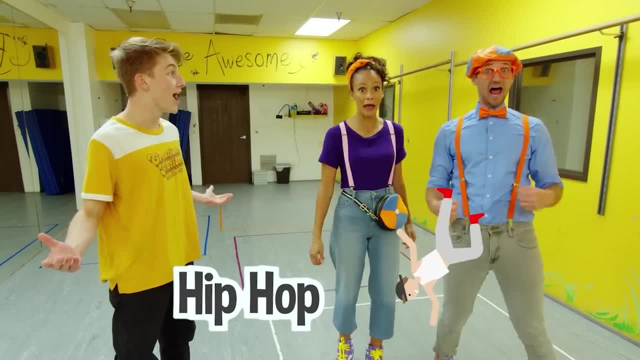 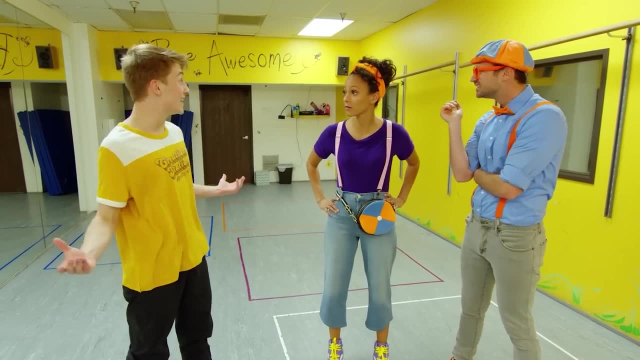 Thank you. Do you guys want to learn some hip-hop moves? Yeah, Okay, well, first, do you guys know what hip-hop is? A type of dance? Yes, it is a type of dance, But it's like all types of dance. 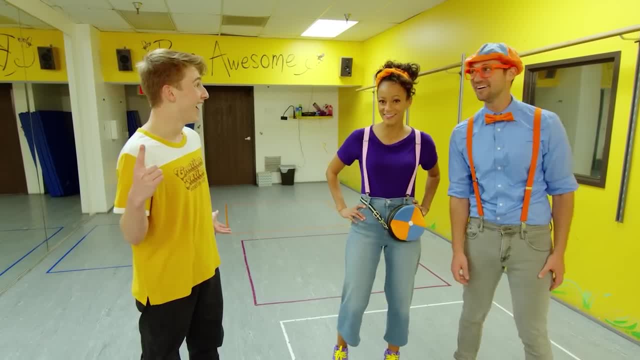 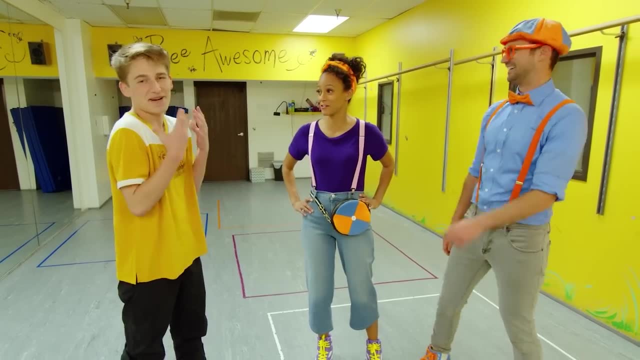 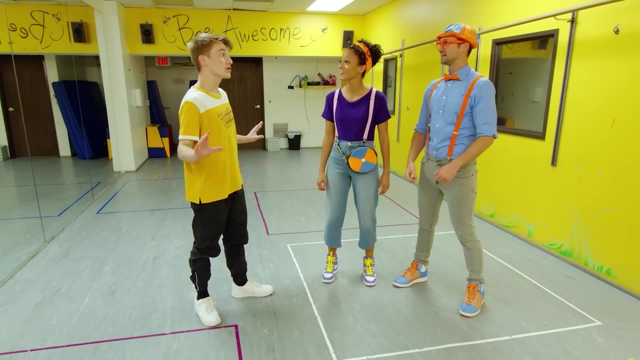 mixed together into one, Wow, Cool. Yeah, it's like ballet dancing and tap dancing and jazz dancing all put together And there we have hip-hop. Yeah, Yeah, Okay. do you want to learn some moves? Yeah, Okay, Ready. 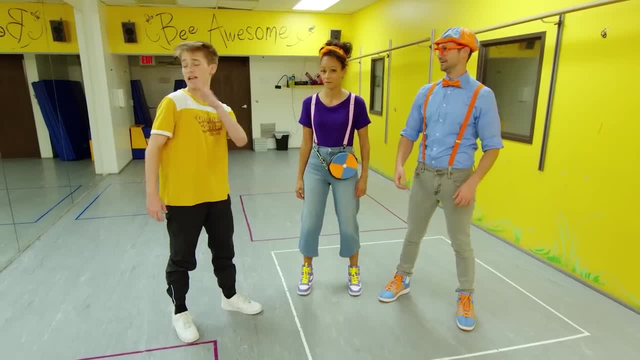 First we're gonna dust off our shoulders- Ready. We're gonna take our left hand and we're gonna dust off our shoulder- Oh, like it's dirty, Yeah, Ready. And then we're gonna do it to the other side. 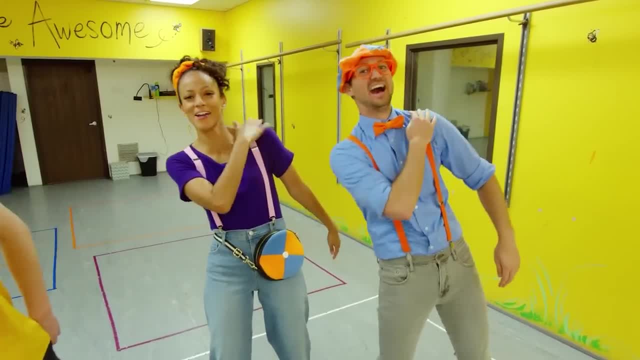 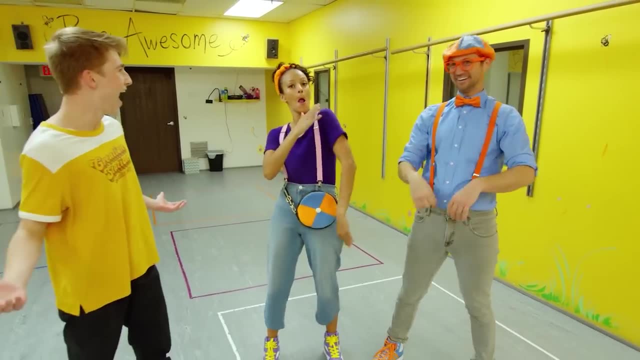 Okay, Dust it off. Yeah, Wow, You guys are so good at that. Oh, thank you, You too. Aw, thank you. Okay, ready. Do you want to learn another move? Yeah, So we're gonna raise. 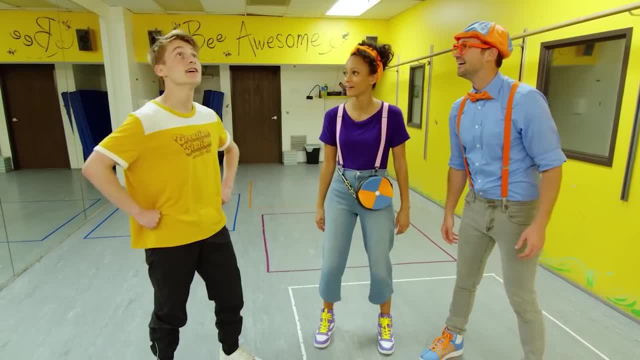 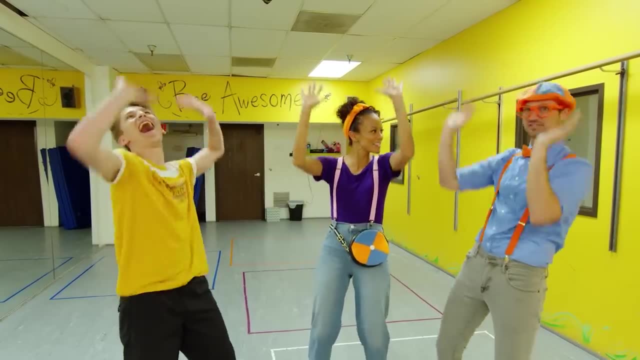 the roof Ready. You're gonna take your hands, you're gonna place them up like they're on the ceiling, like that, And then you're gonna push the ceiling up. It's really heavy, Right, Yeah, Wow, Raise the roof. 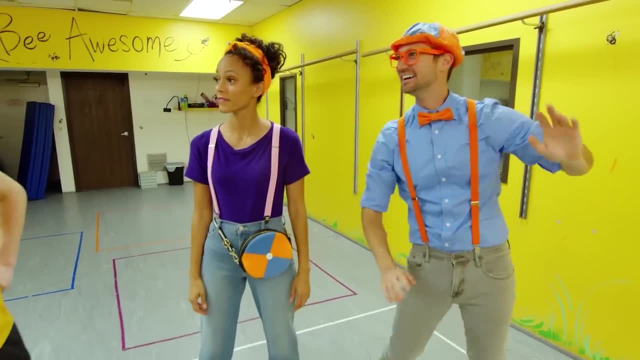 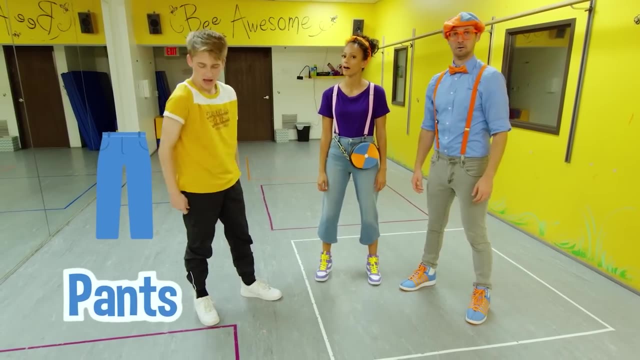 Raise the roof, Perfect. Wow, You guys are really good at hip-hop. Oh, thank you, Ready. Another move. We're gonna put our pants on, Ready. What we're gonna do is we're gonna grab it and put it up. 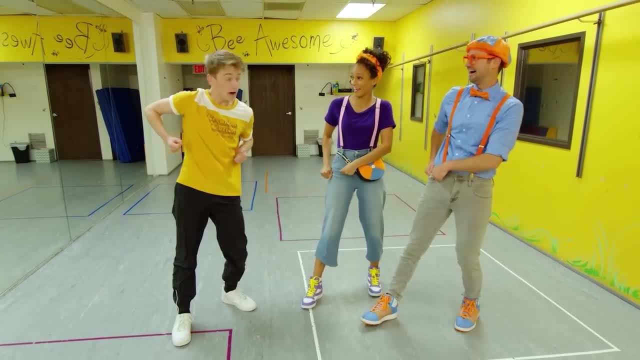 Whoa, So ready. Grab your pants and put them on. Okay, We're gonna do it to the other side. Ready, Grab your pants and put them on. Yeah, Let's try it one more time. Ready. 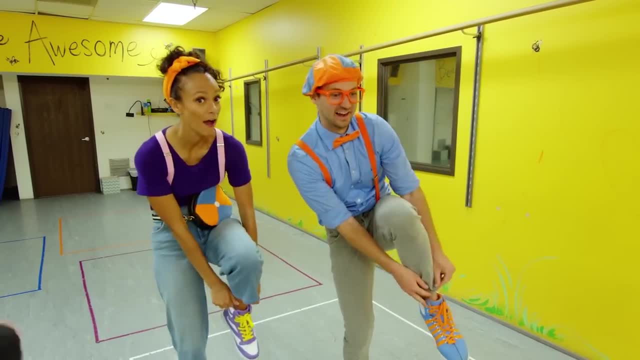 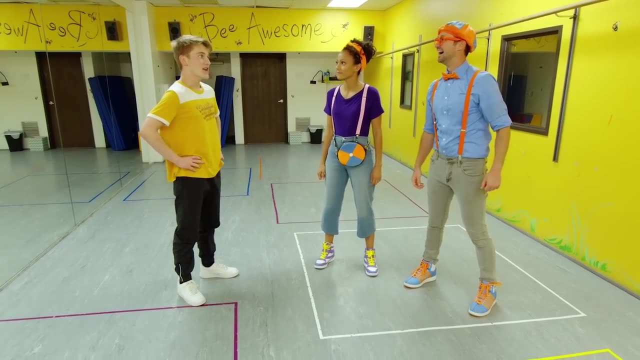 Grab your pants, put them on Other side. Grab your pants, put them on. Yeah, Woo, Okay, Ready, Huh, We're gonna learn another hip-hop move. Whoa, So many moves. Ready, We're gonna do a hip-hop. 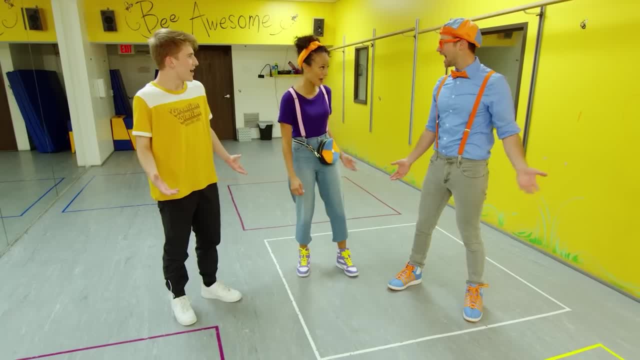 slide. Do you guys like water slides or anything like that? Yeah, We love going down slides. So much fun. Well, ready, We're gonna learn a hip-hop slide. So, all you're gonna do, you're gonna take your hand. 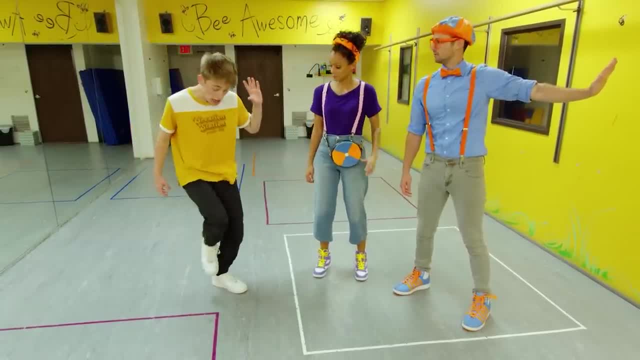 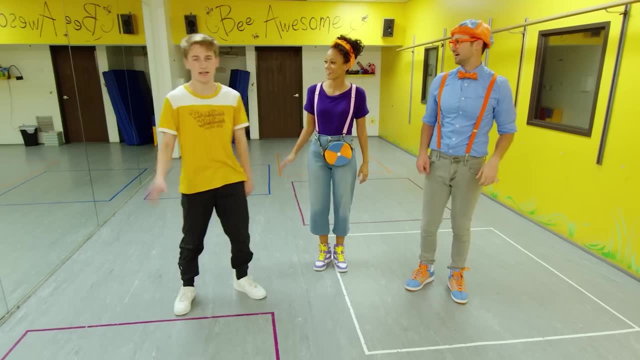 and push it away At the same time, you're gonna slide your feet over to the right side. Oh Okay, You do the exact same thing on the other side. Take your right hand, push it away, left foot slide. 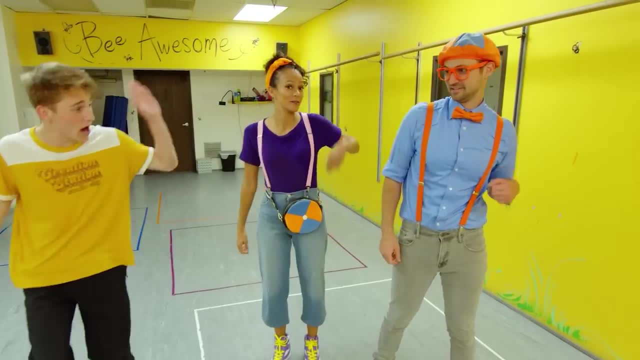 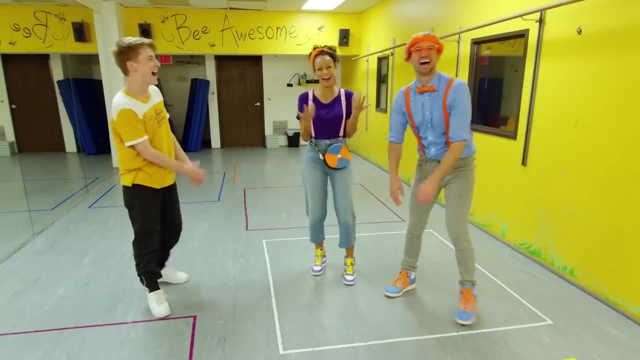 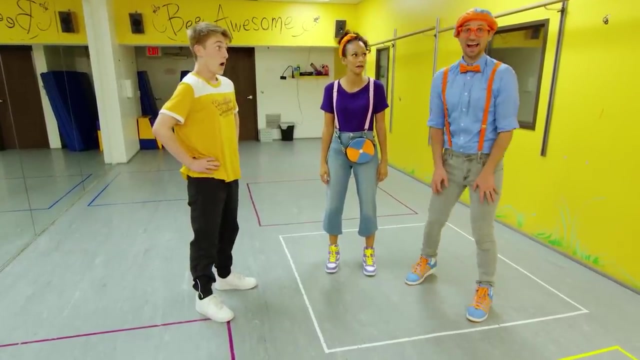 Whoa Ready. Let's try it one more time, Ready. Slide to the right, Whoa, And slide to the left, Whoa Tonya. okay, Yeah, Ready, We're gonna learn a super cool move, Yay, Okay. 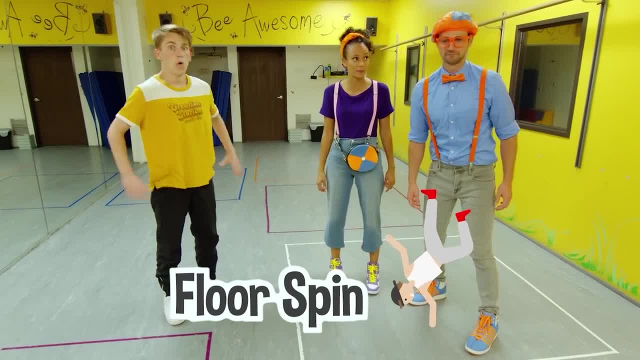 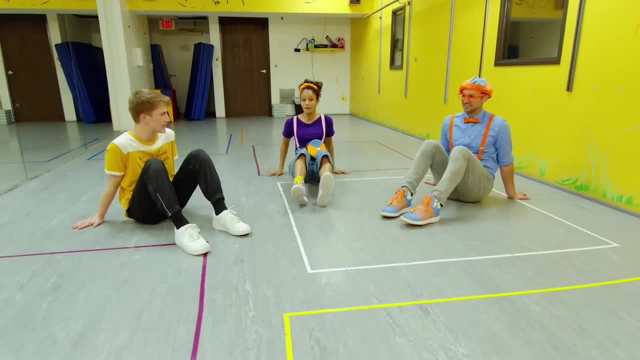 This is called a floor spin. Floor spin, What, Whoa? Okay, all you're gonna do. you're gonna stay on the floor, Ready. Let's stay on the floor Ready. We're gonna sit with our feet, Just like this. All you're gonna do. 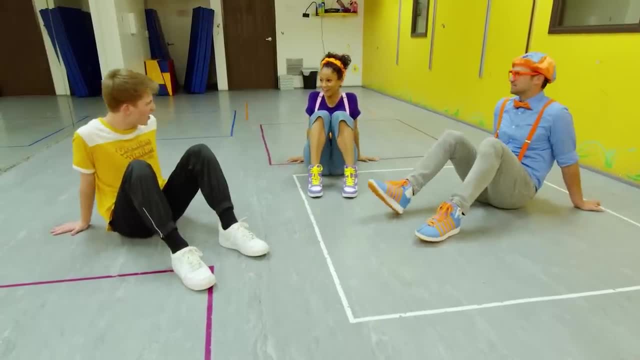 make sure you have all your weight on your hands behind you. Okay, Is all your weight on your hands? Yep, I think so Ready. All you're gonna do is you're gonna push your hands around and then strike a pose. 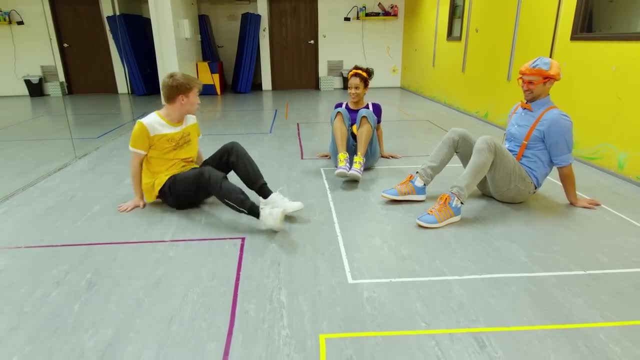 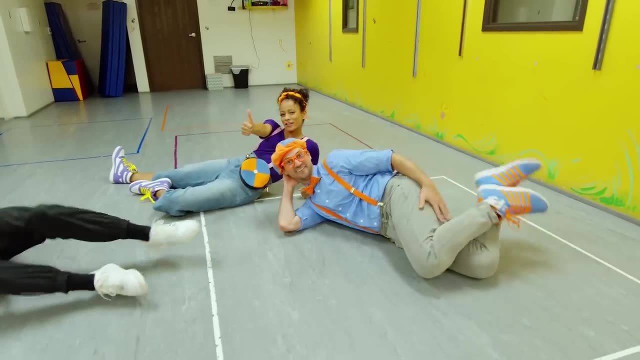 Whoa, Yeah Ready. Do you guys wanna try it? Yeah, Ready, Let's go Ready And go. Whoa, Whoa And ready, Strike a pose, Strike a pose, Yeah, Yeah, Mika. 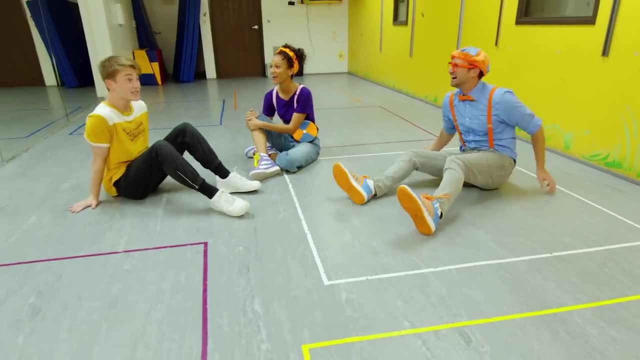 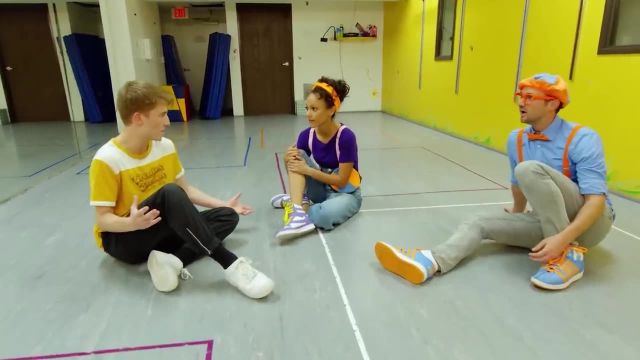 Okay, Flippy, That was awesome. That was awesome. You guys did so good, Thank you, Thank you. Okay, now that we've learned all those hip hop moves, do you wanna put it into a fun hip hop combo? Yeah, 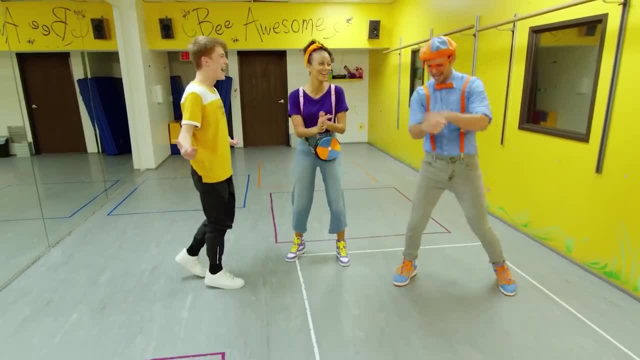 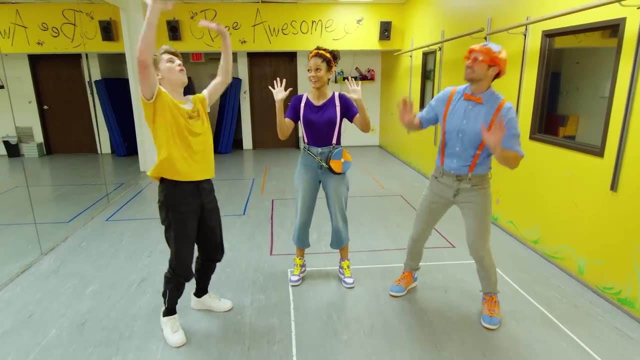 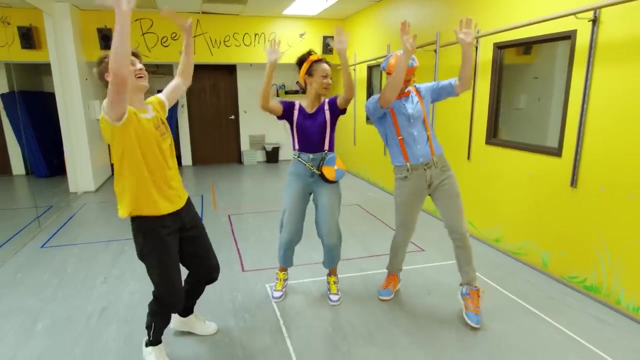 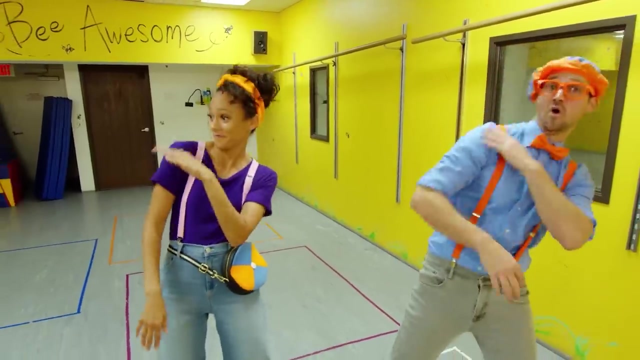 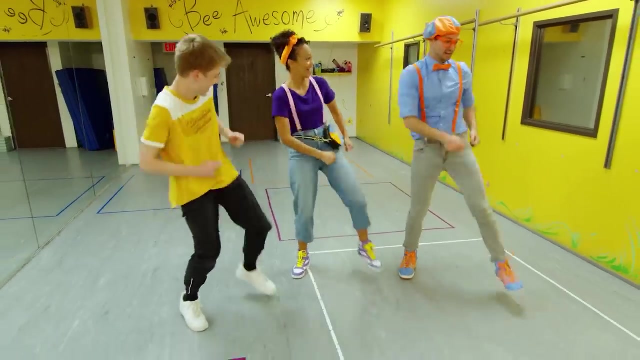 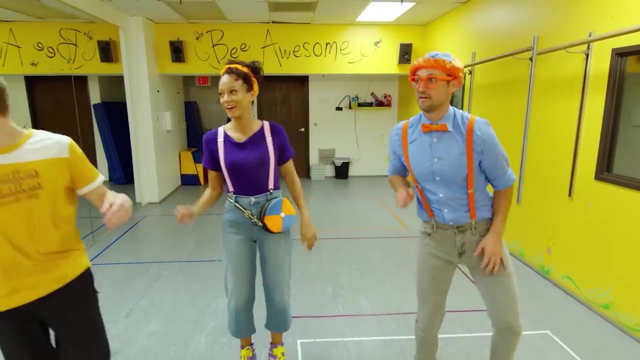 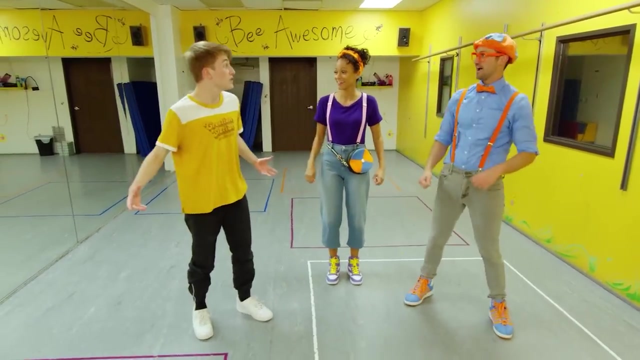 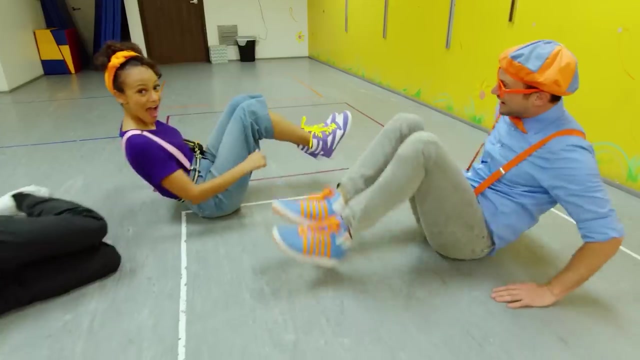 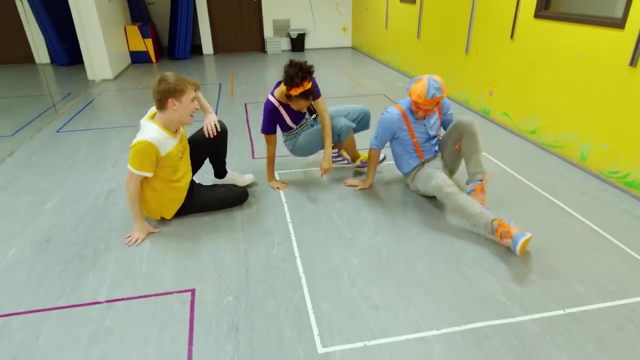 Okay, ready, Let's stand up and dance. Okay, Let's do it, Woo. So first we're gonna start with raising the roof. Let's go. Okay, Woo, money, money, dream, dream, dream, dream, dream dream. that was awesome. thank you so much for teaching us how to dance hip-hop style, of course. 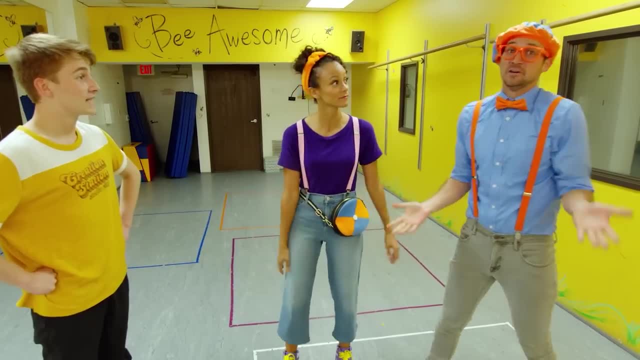 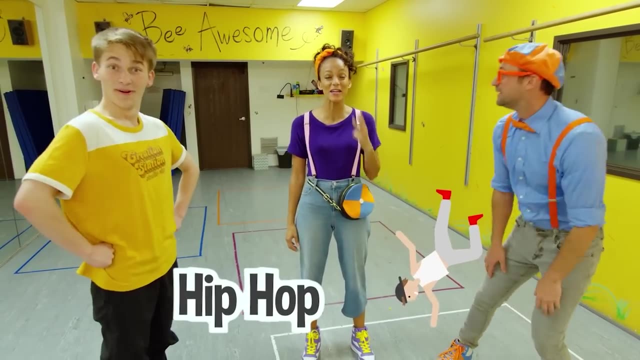 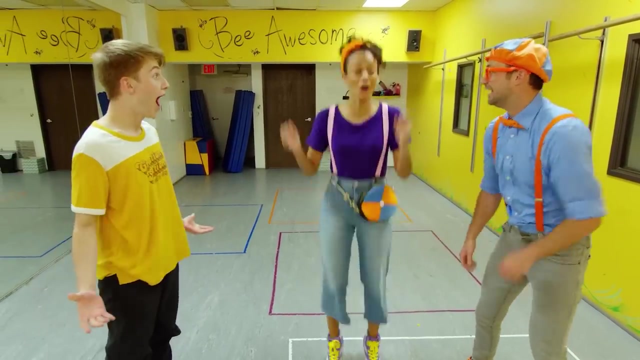 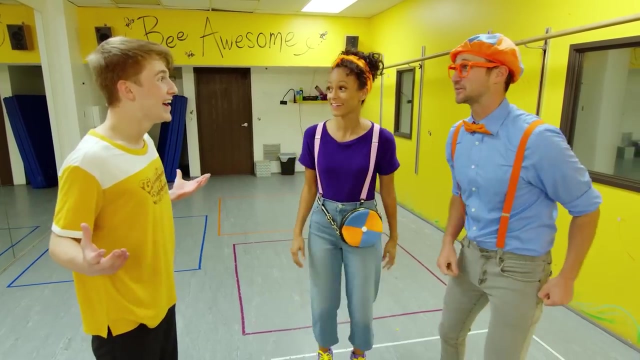 yeah, so so far we've learned how to do some ballet and tap and hip-hop- three different styles of dance. oh, maybe mika and i we should have a show. yeah, let's do it. you can be the blippy and mika dance recital. yeah, do you want to come to the show? yes, i'd love to come. all right, see you. 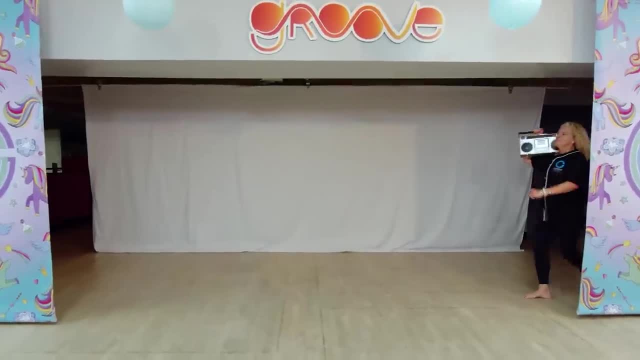 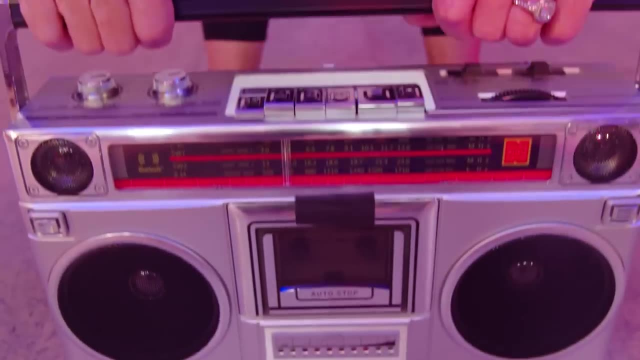 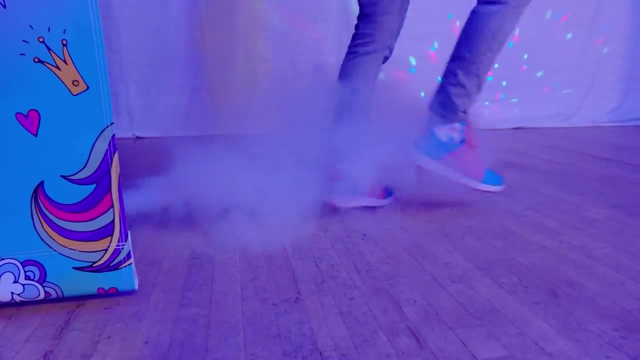 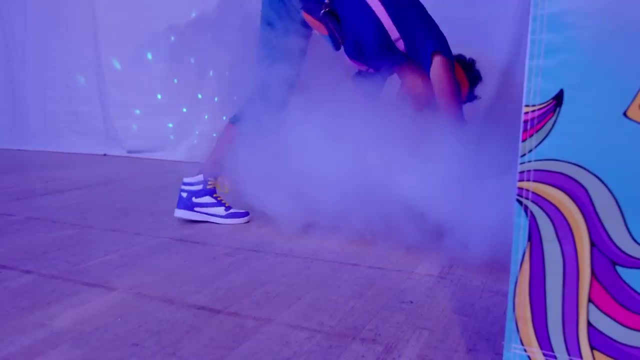 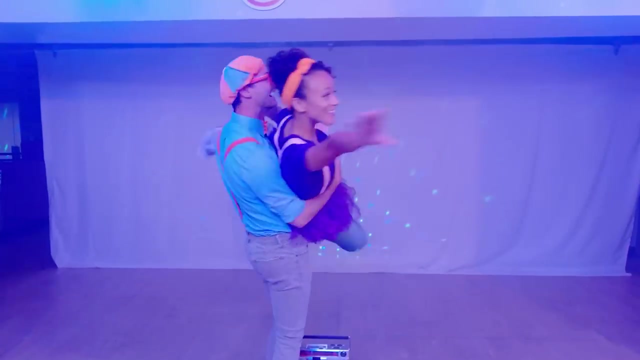 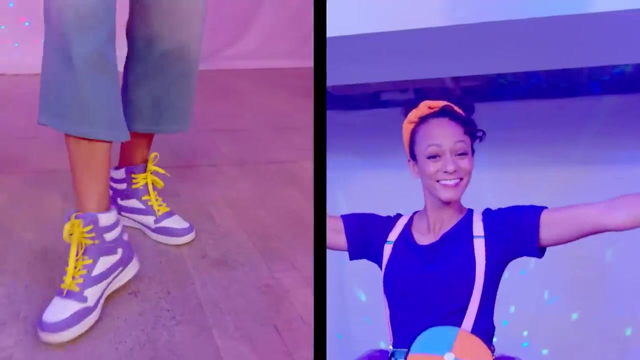 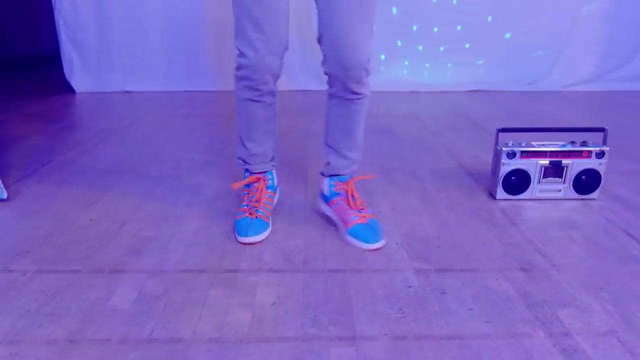 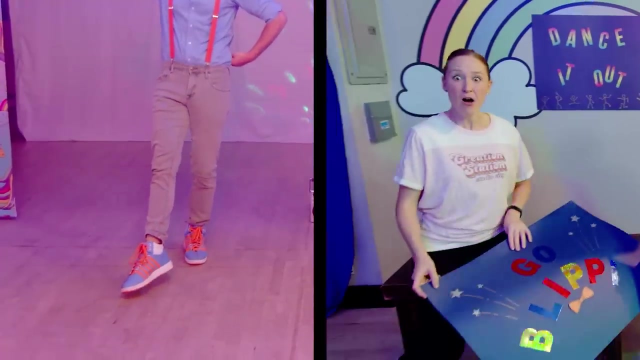 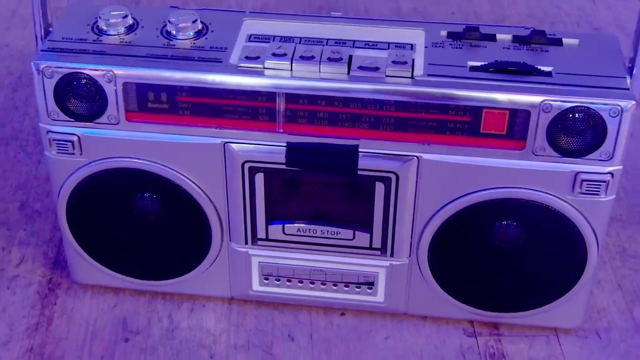 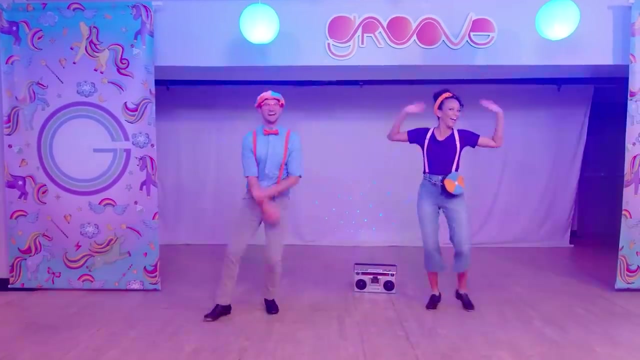 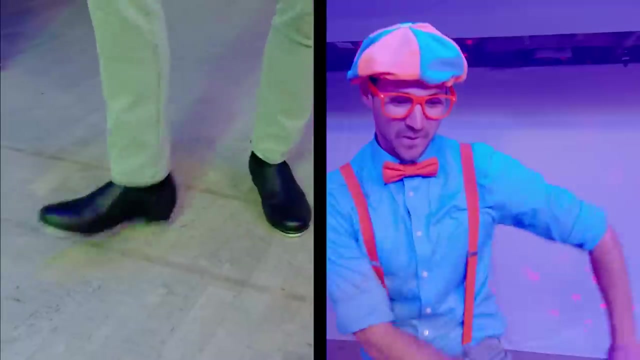 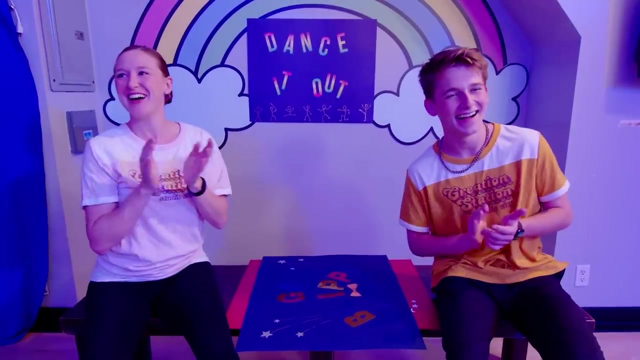 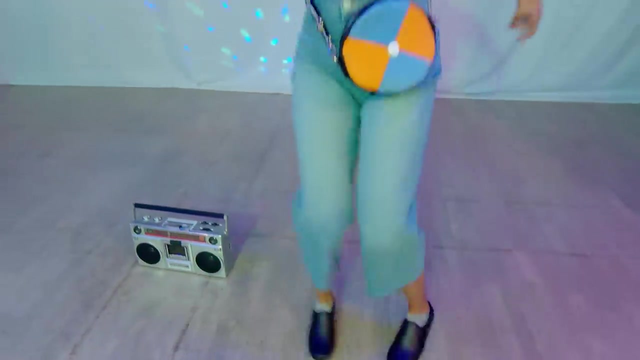 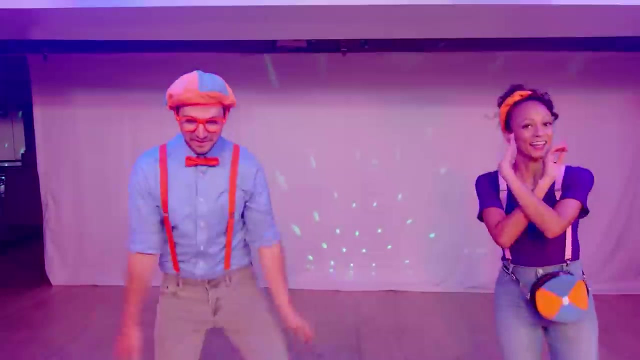 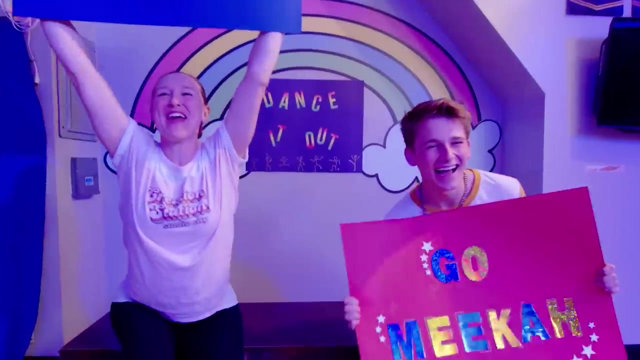 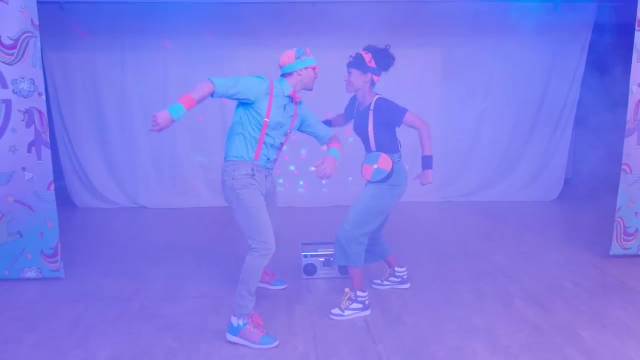 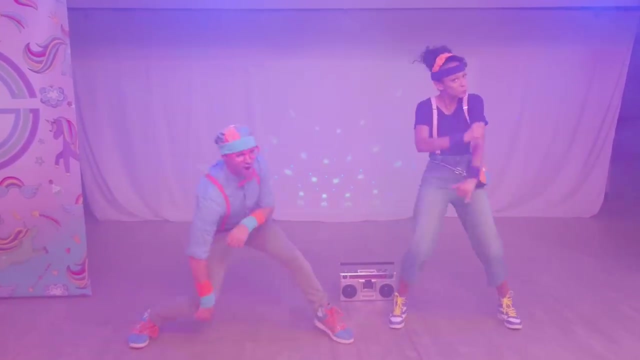 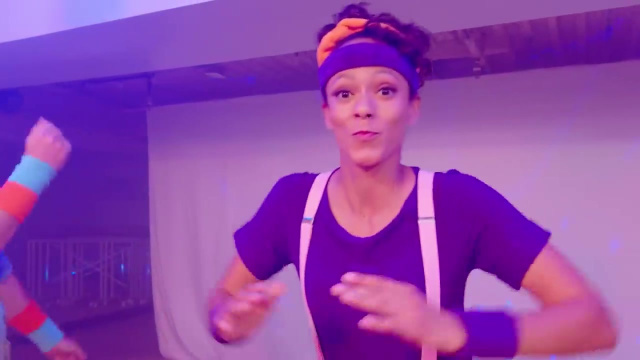 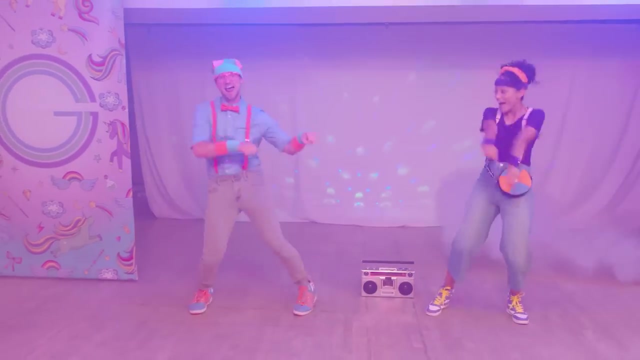 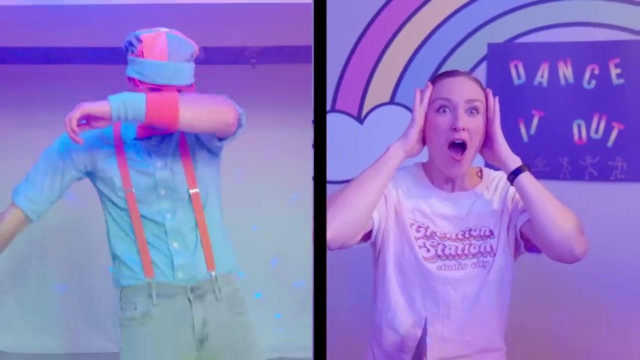 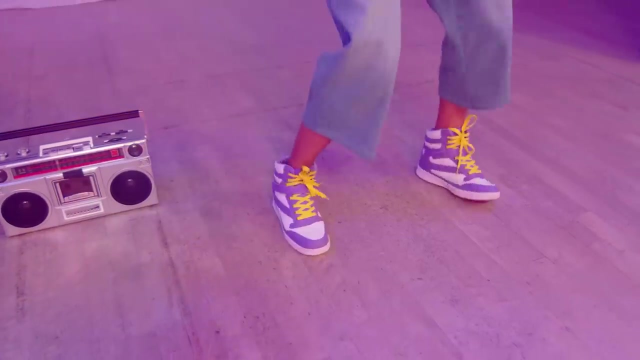 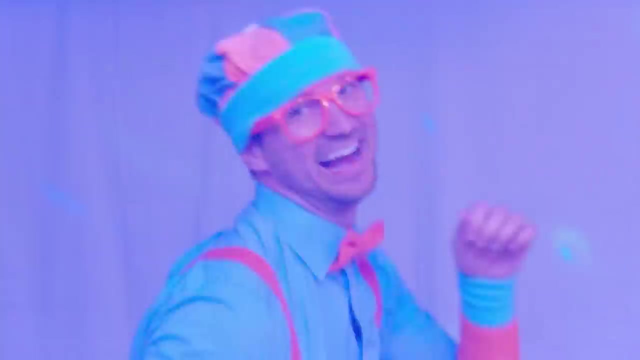 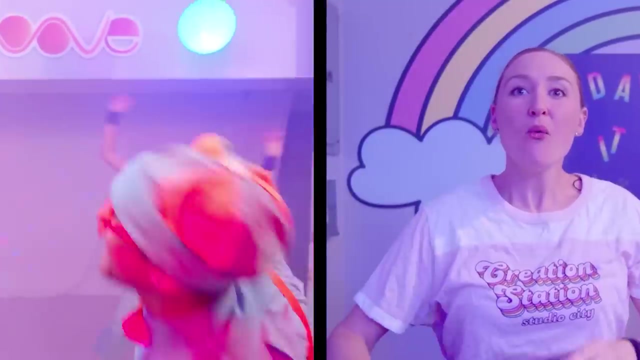 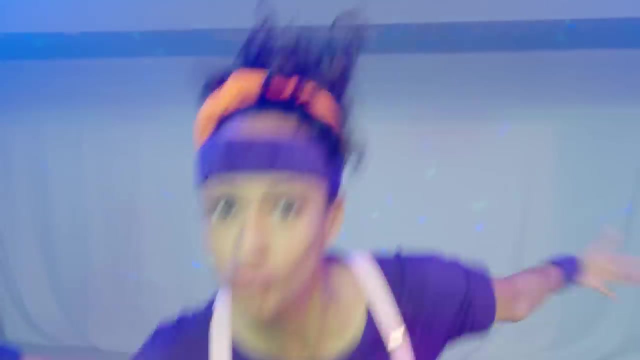 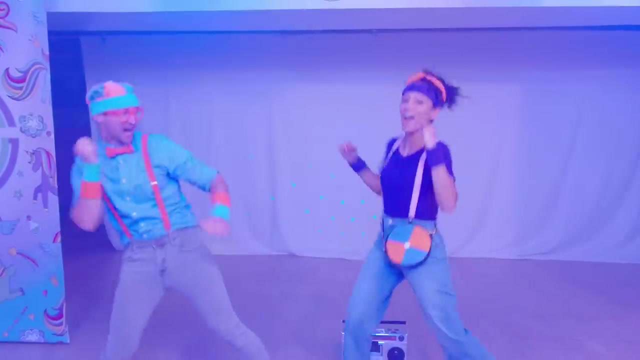 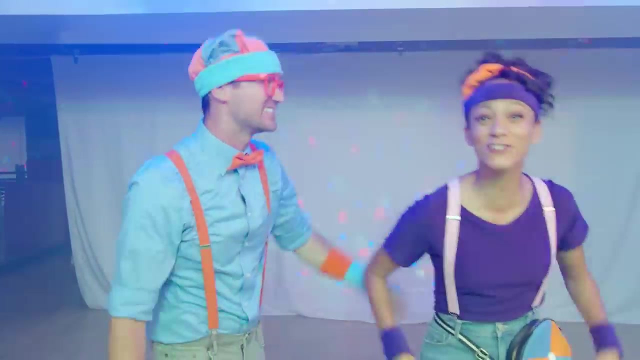 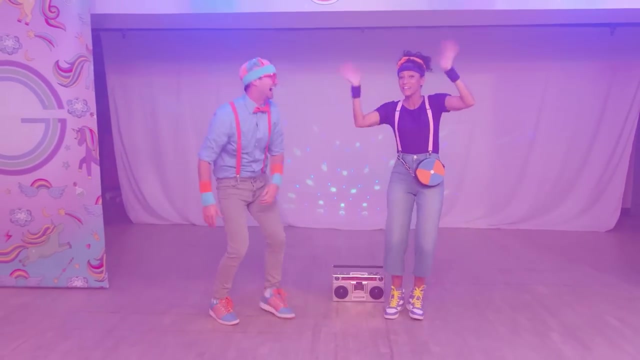